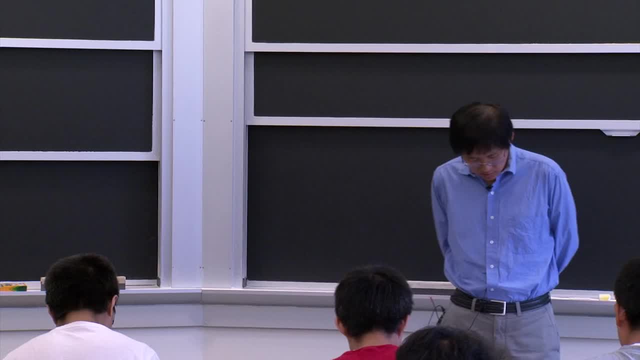 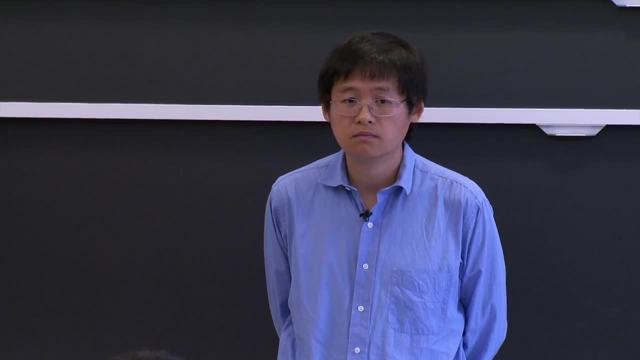 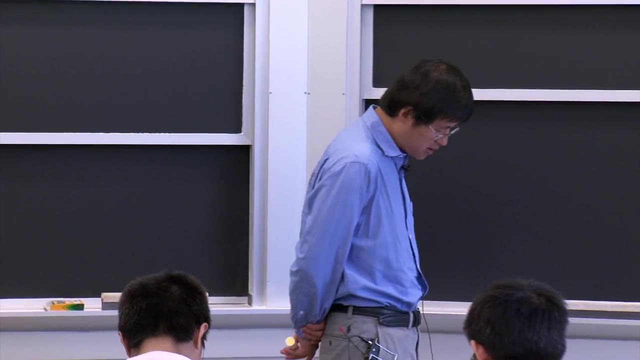 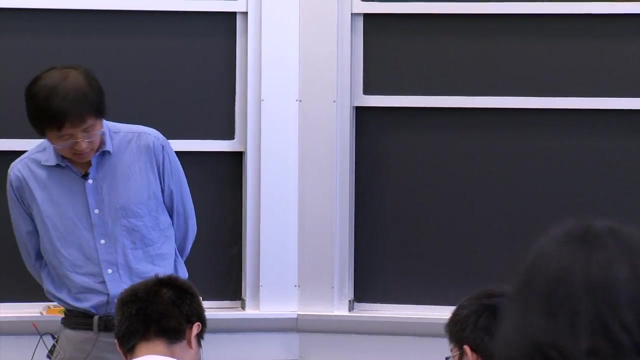 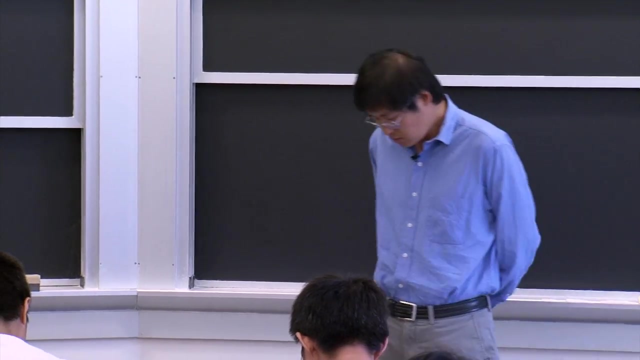 Good, So before we start, do you have any questions on what we did before? OK, So we have discussed that black hole can be considered as a thermal object and that actually black holes obeys the standard law of thermodynamics, And now we also mentioned that it's a natural question. 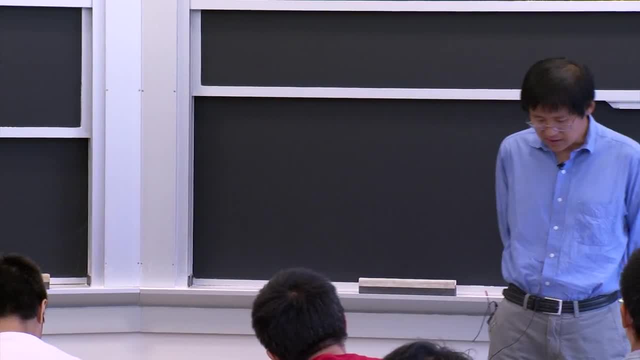 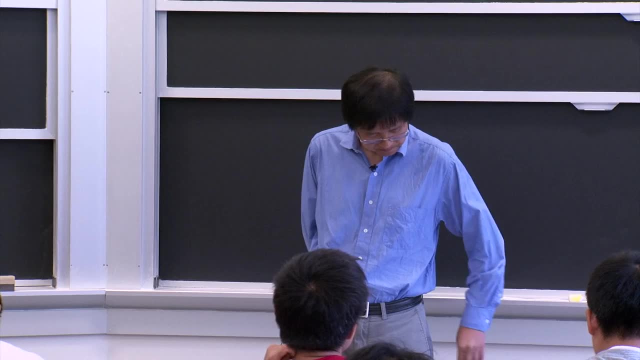 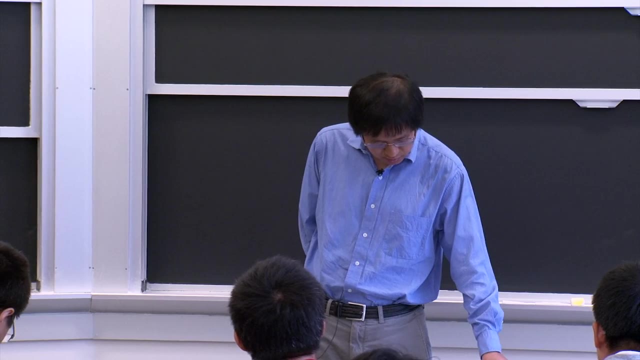 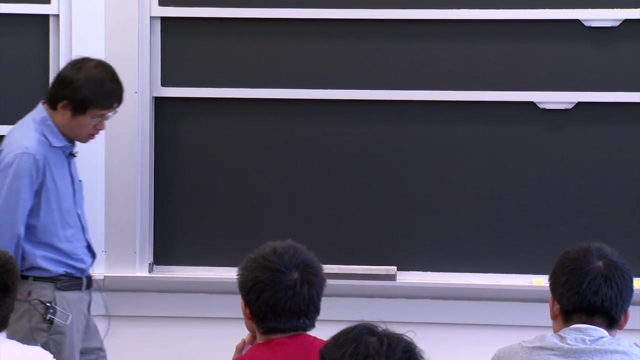 to ask Black hole should be considered as ordinary quantum mechanical objects, And so this is related to the issue of information paradox. But if one disregards this information paradox, which I think now have a very good in principle, have a reasonable resolution, which we will talk about later. 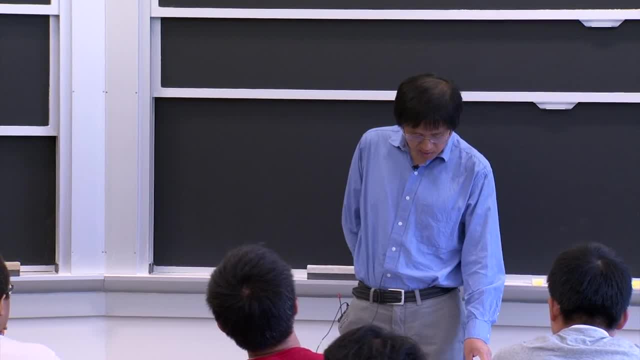 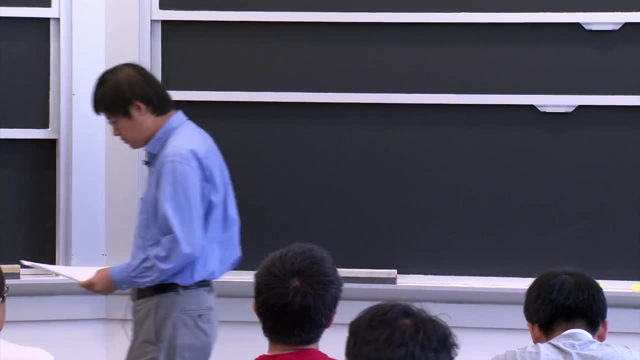 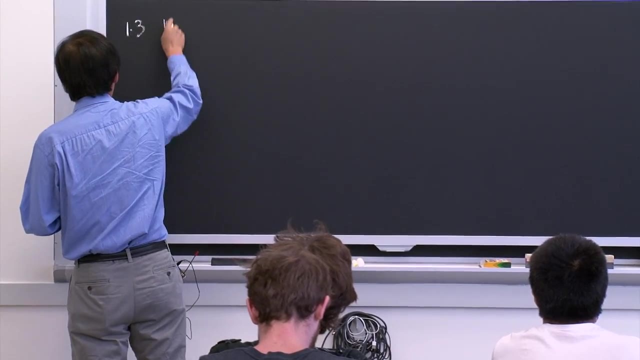 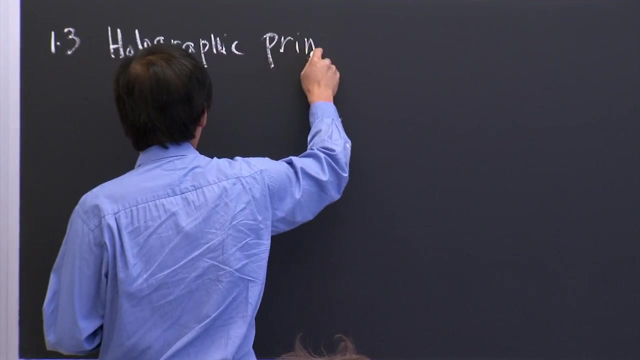 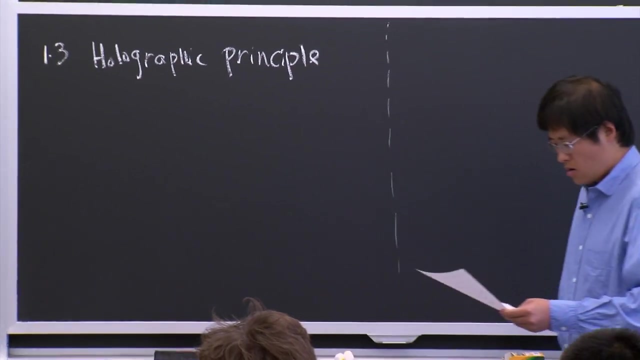 But if we do treat the black hole as ordinary quantum mechanical object, then there are actually very important implications. So one implication is this called the holographic principle. So holographic principle, by the way, is a very important one. It's a very important principle by itself. 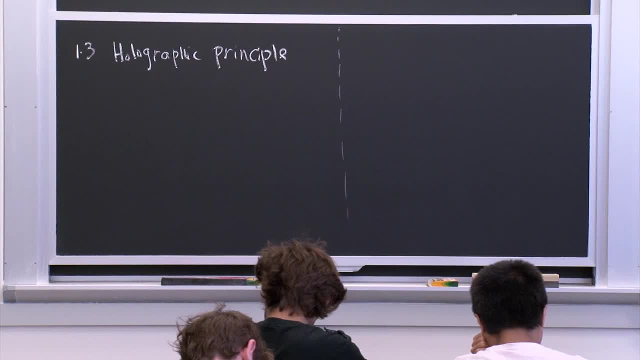 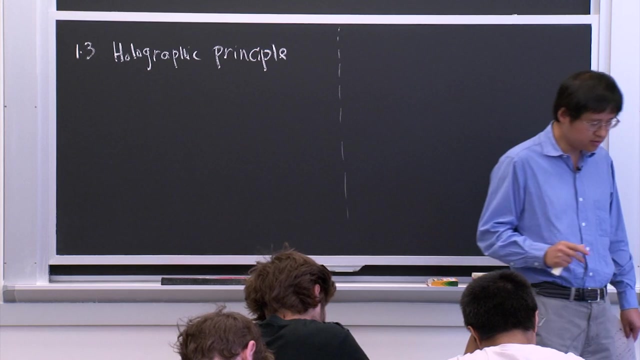 It's in some sense a rather heuristic concept at the moment And I will also only give you a very heuristic discussion, And it's possible to make it a little bit more rigorous, But I will do it at a rather heuristic level just. 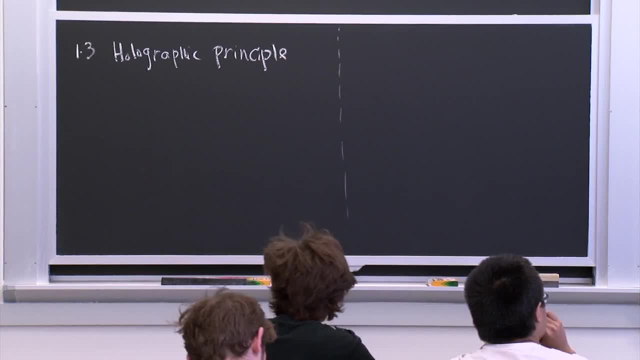 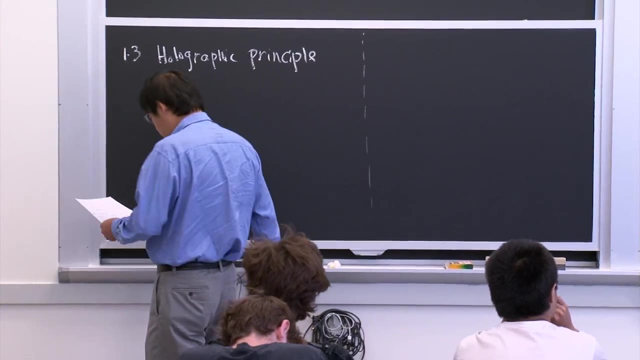 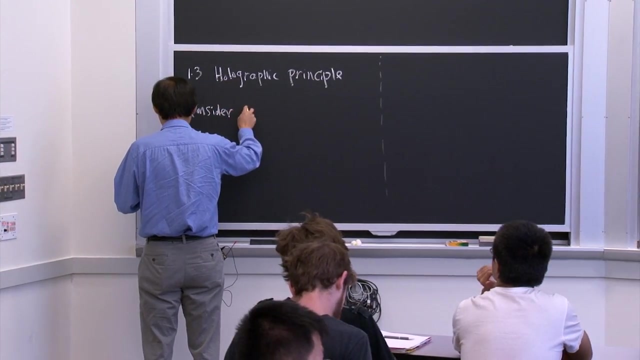 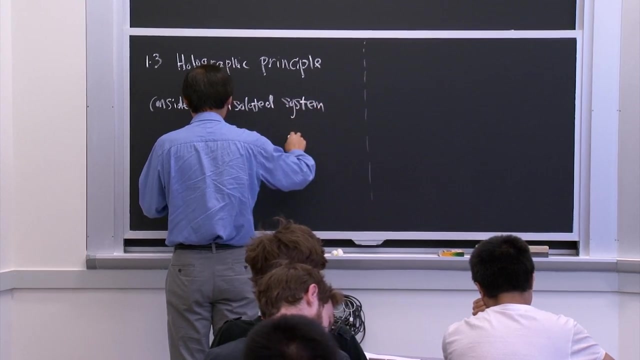 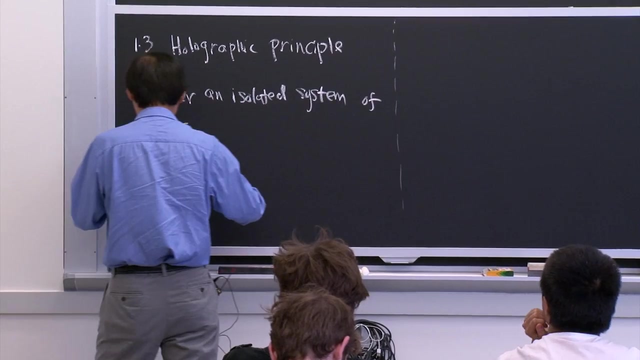 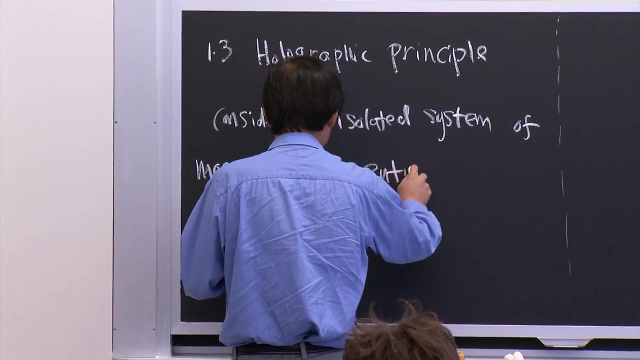 to give you a feeling. So let's consider that there's something profound going on in quantum gravity because of the black holes, because of black holes. So let's consider an isolated system. Let's say we have a mass of mass, say E and say entropy S0,. 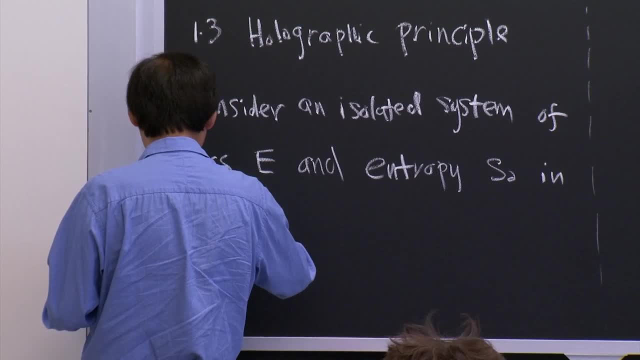 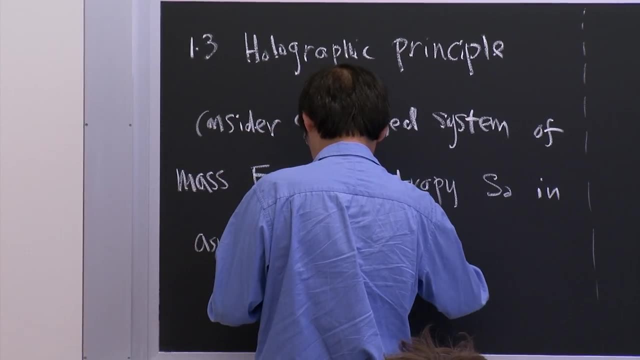 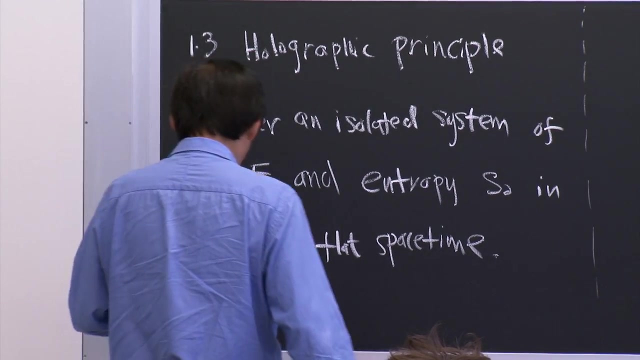 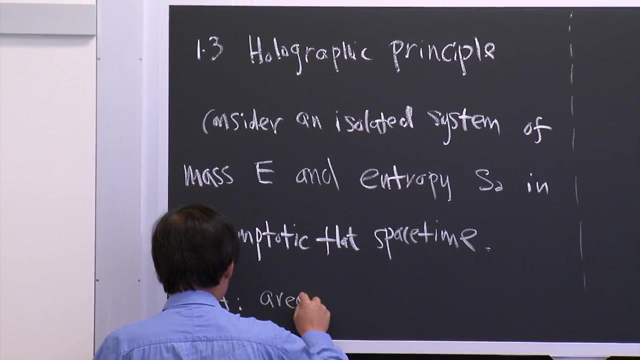 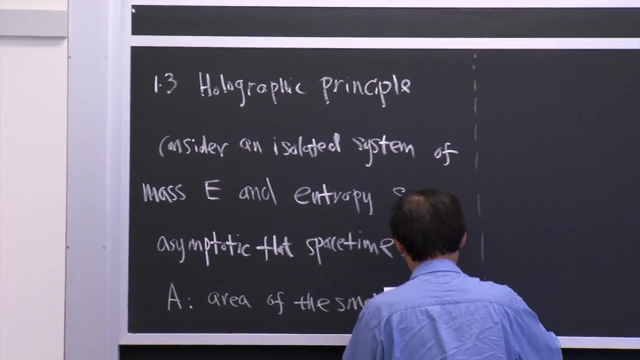 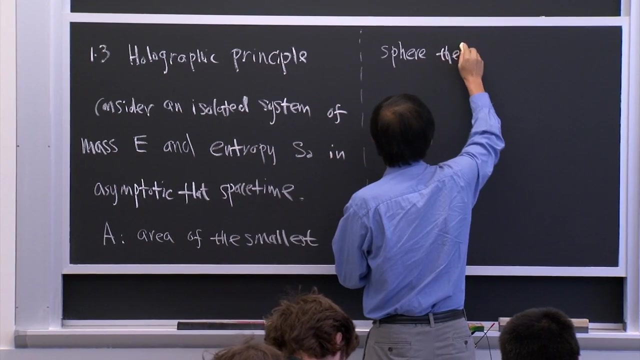 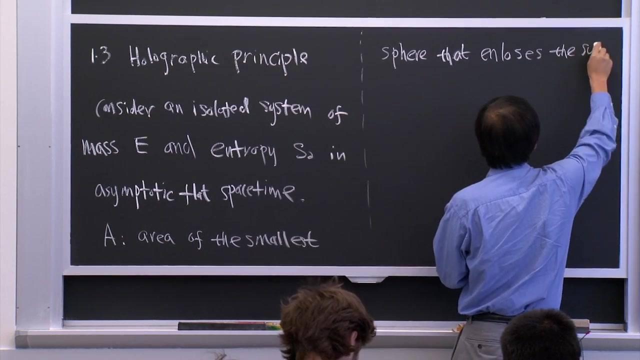 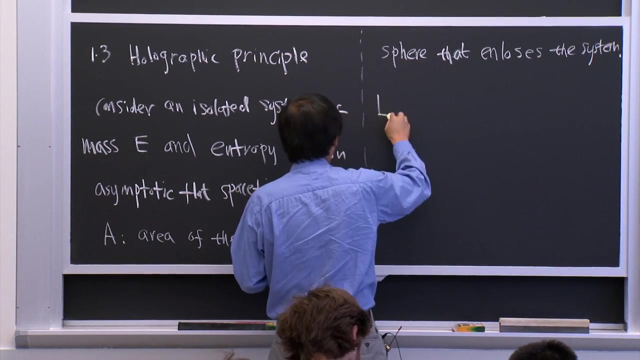 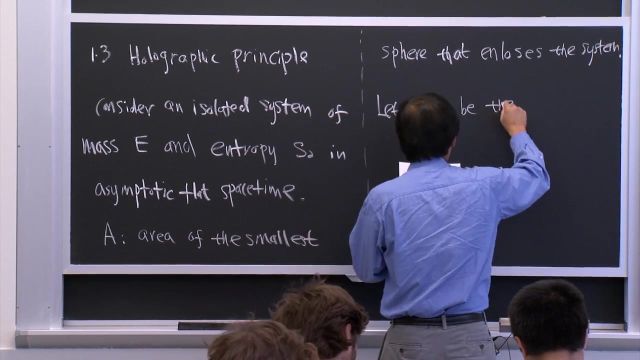 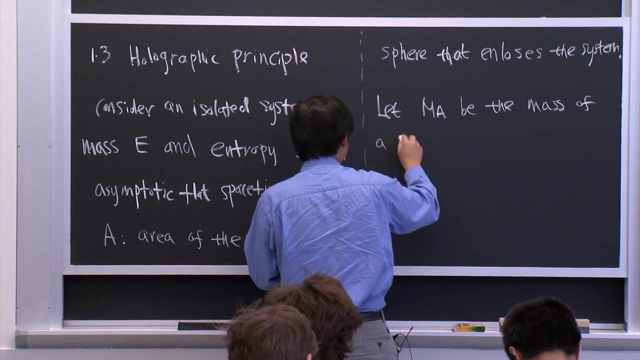 say in asymptotic flat space time, OK. And then we also denote A as the area of the smallest sphere, that say encloses the system, OK. And also let me introduce: let M A be the mass of the black hole. 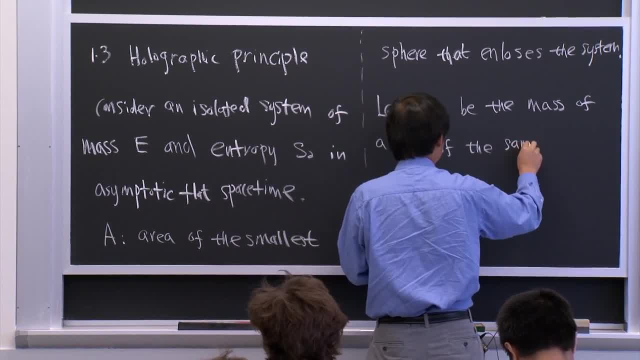 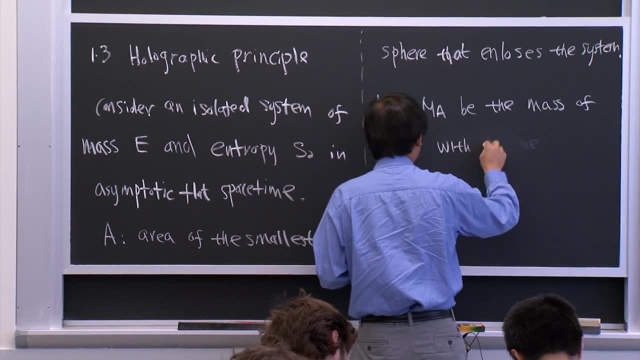 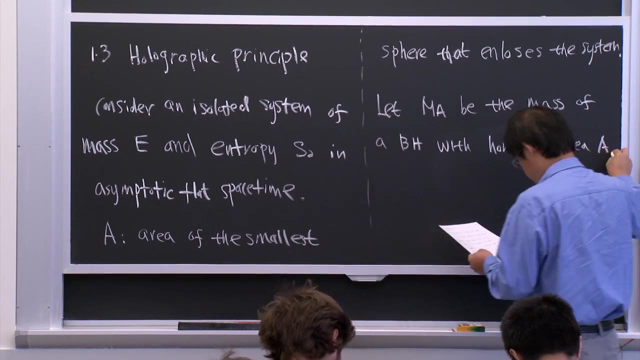 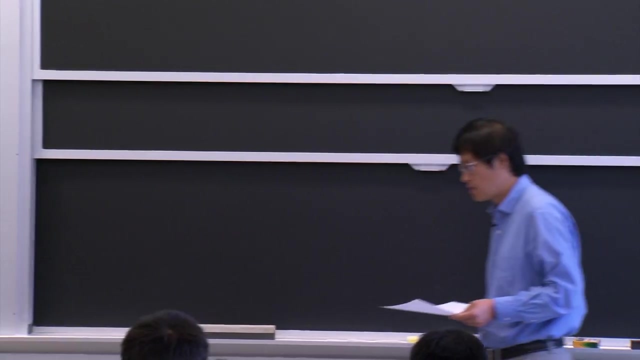 of the same horizon area. OK, OK, OK, OK, OK, OK, OK. Yeah, Say with black hole with horizon area A: OK, So in GR, anything which is sufficiently massive will eventually collapse to form a black hole. 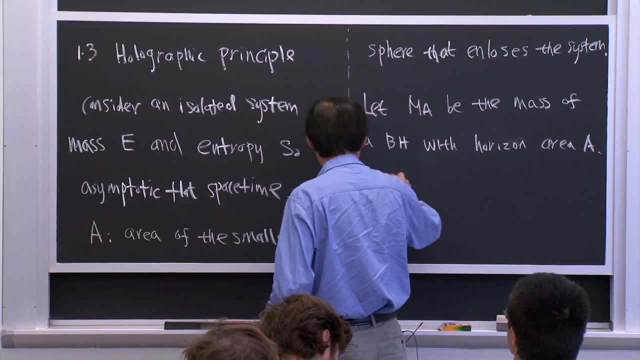 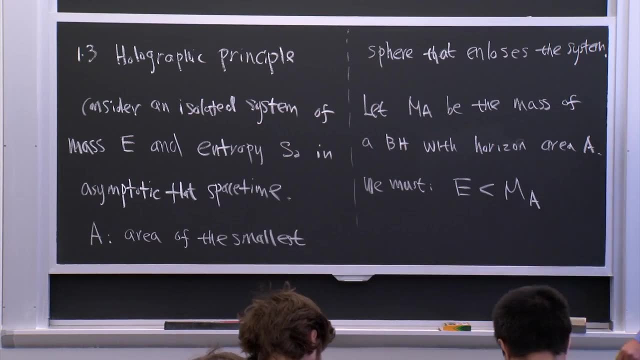 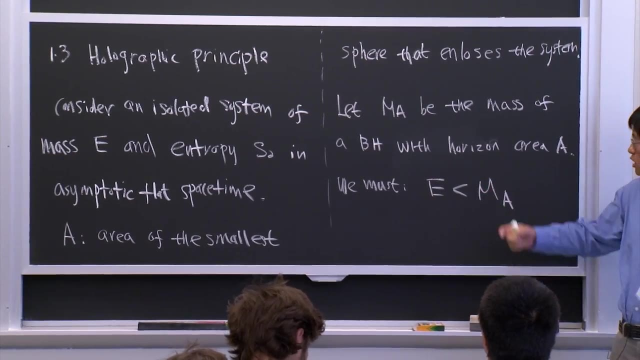 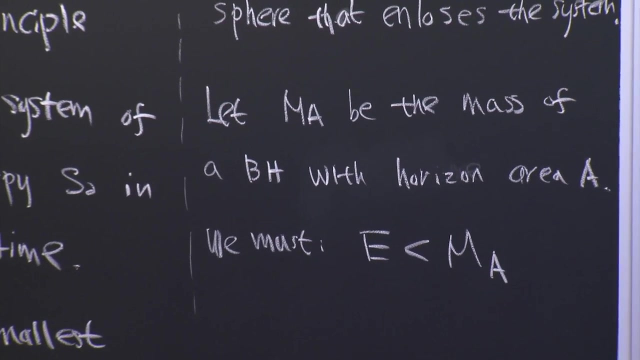 Because of that. OK, So we must have E. is smaller than M A. OK, So we must have E. So whatever energy you can put in this region surrounded by area A must be smaller than the mass of a black hole which you can put in that region. 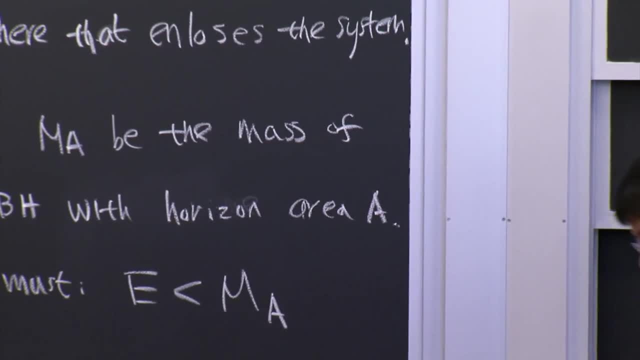 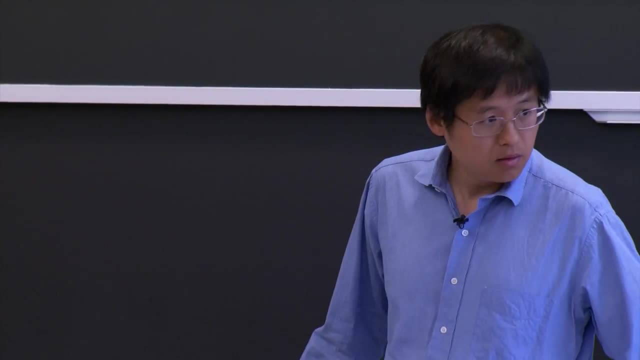 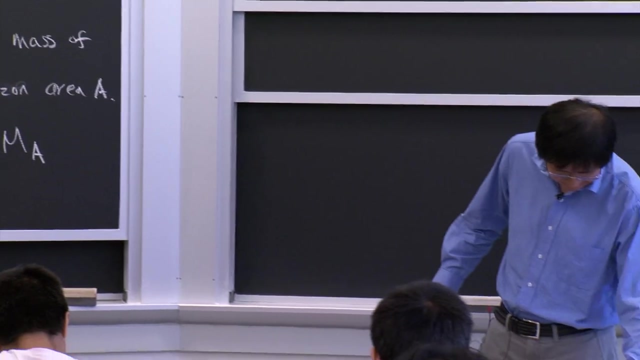 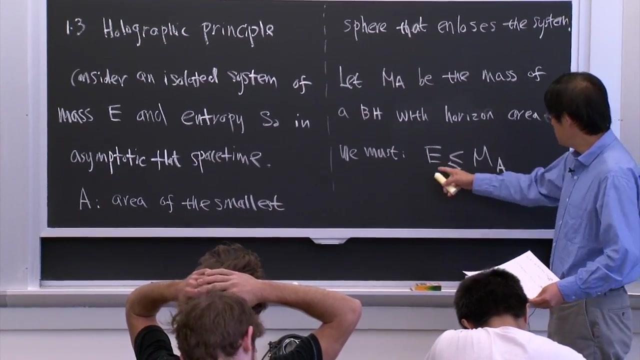 OK, OK, OK, OK, OK, OK, OK, Because otherwise, if we have more mass, then we would already be a black hole. OK, Could that be equal. Could that be equal? Yeah, Say equal. So now let's suppose E is smaller than M, A, So we can now. 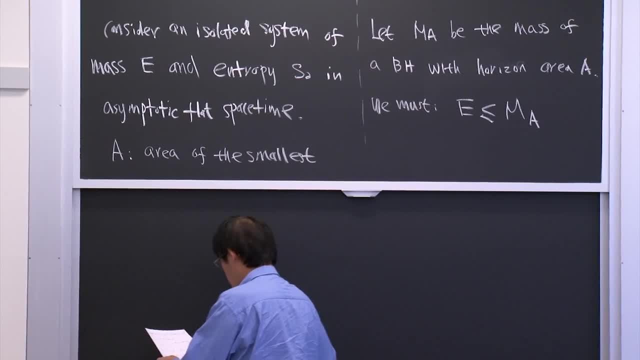 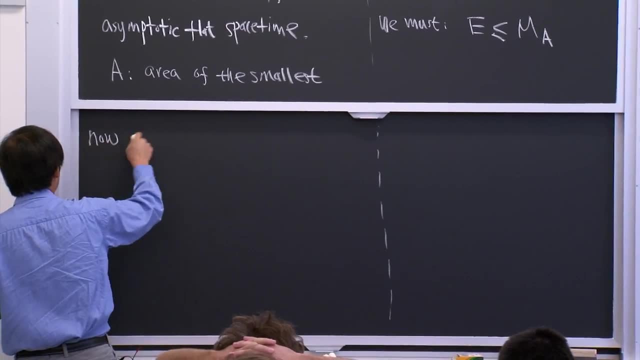 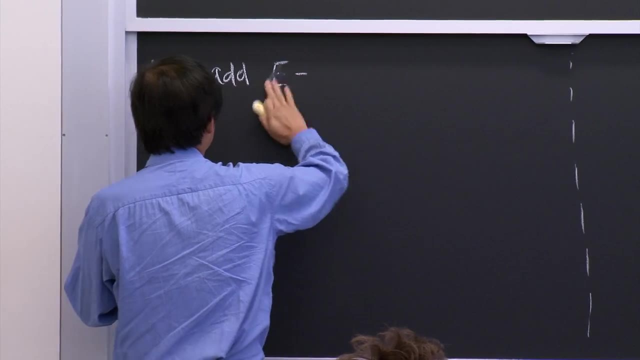 let's suppose E is smaller than M A. So we can now, if we put So we can. now. let's suppose E is smaller than M A. So we can now Now suppose E is smaller than ma. Now we can add this amount of energy, say ma minus E. 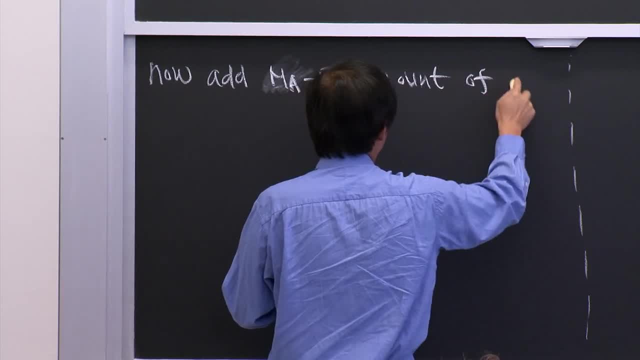 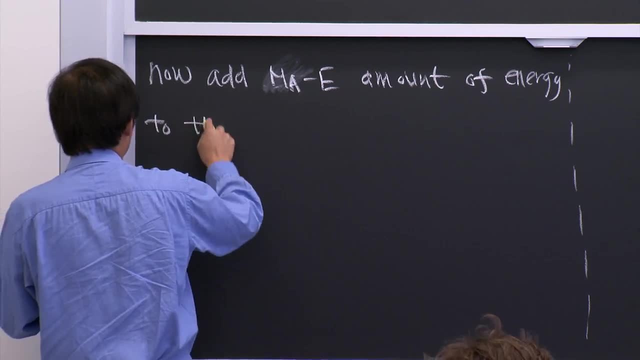 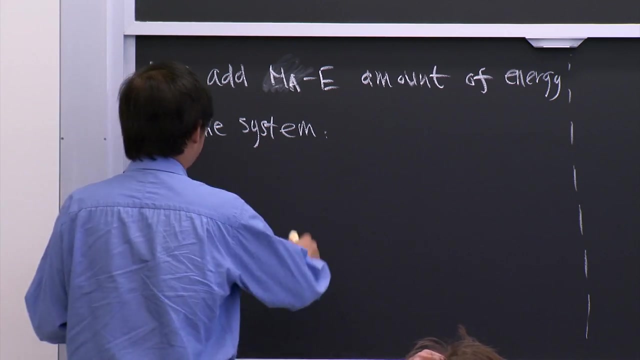 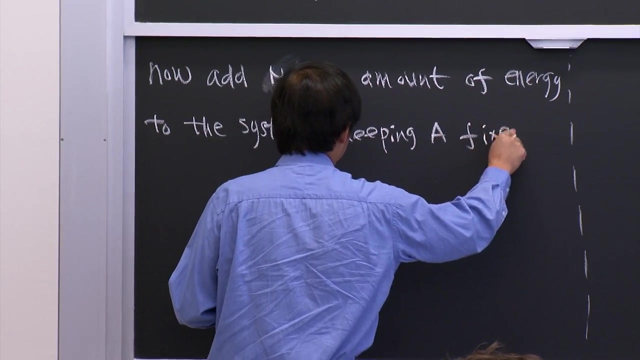 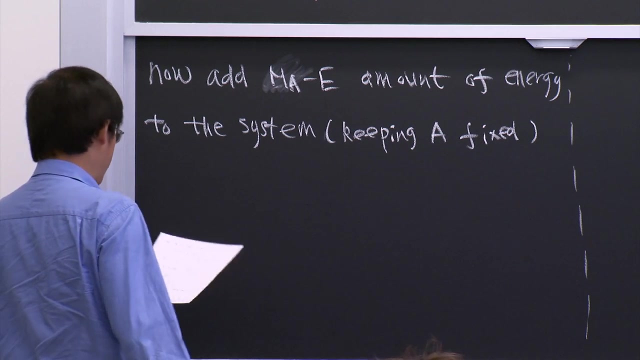 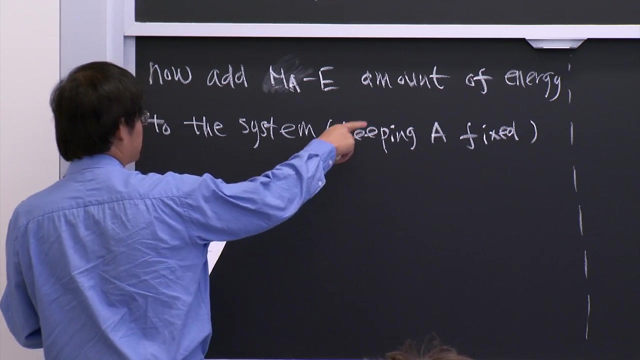 amount of energy to the system. OK, Suppose we can do that, keep A fixed. OK, Suppose we can do that, keep A fixed. And then this will reach a black hole mass, Then the final system will have a black hole. 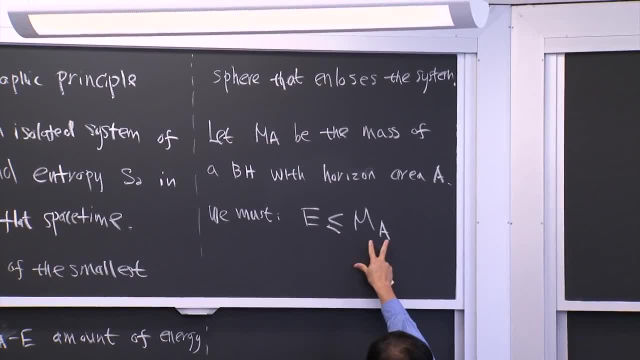 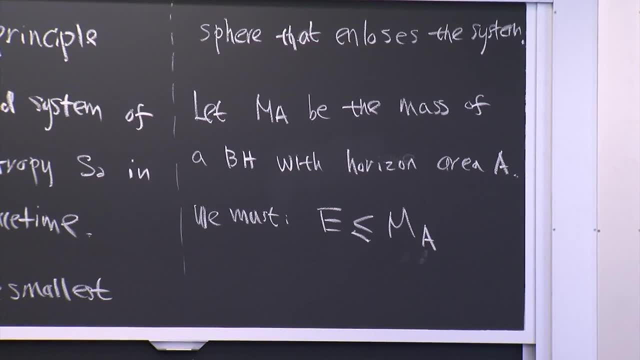 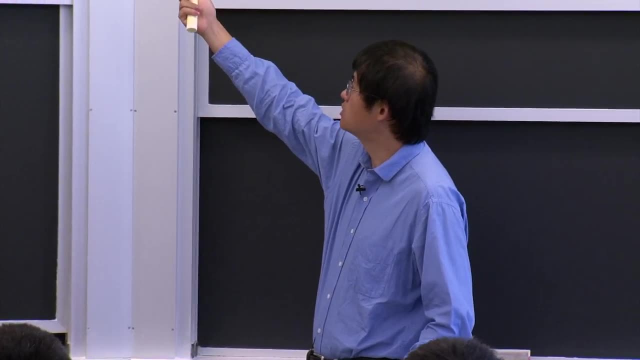 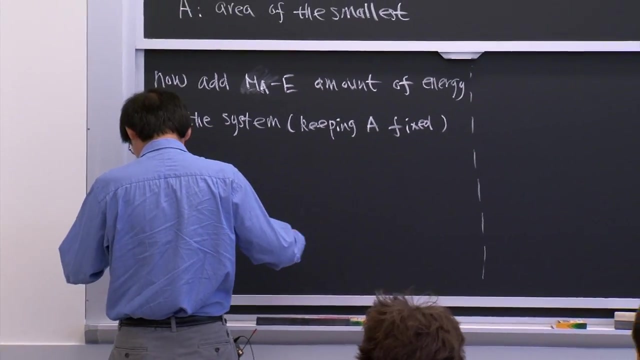 So we'll have the black hole, We'll have the energy given by ma and that object must be a black hole because that's the black hole with the same horizon area. OK, So that's because of this process also tells us. 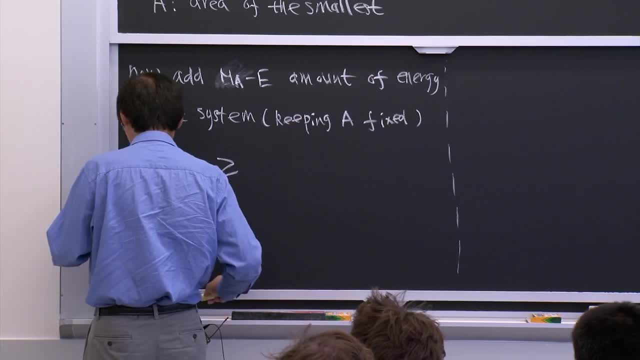 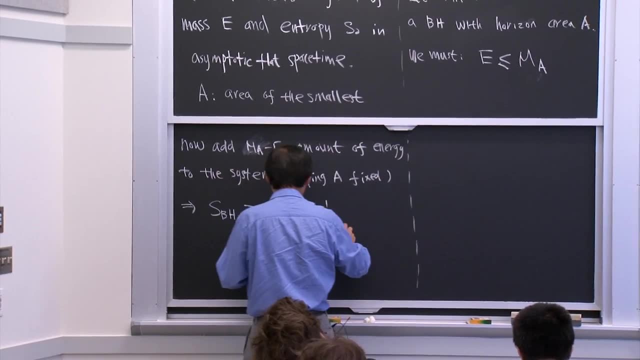 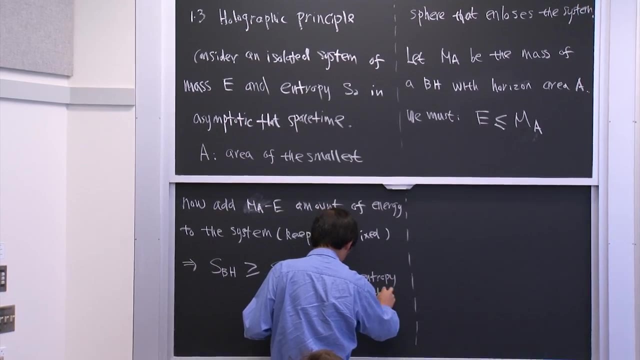 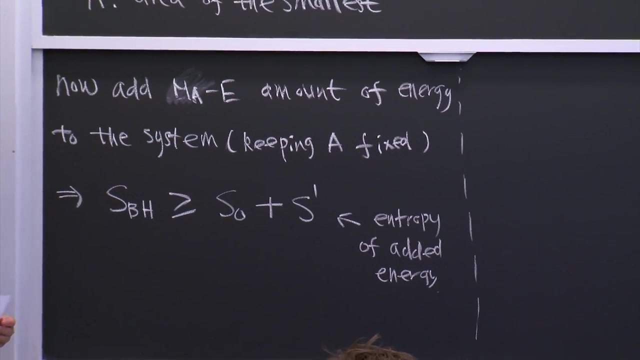 It tells you that the black hole entropy must greater than the S0, the initial entropy of this system, plus the S prime. S prime is the entropy of added energy. OK, So just because of the second law of thermodynamics, your entropy should not decrease. 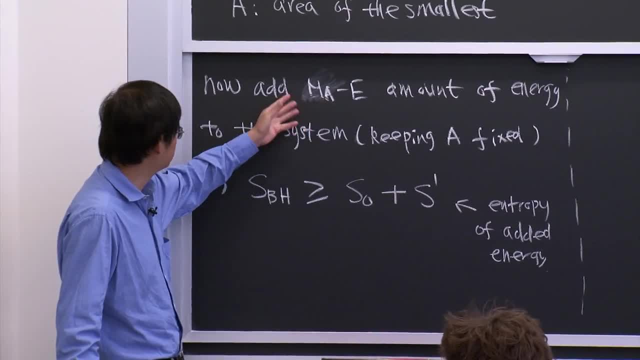 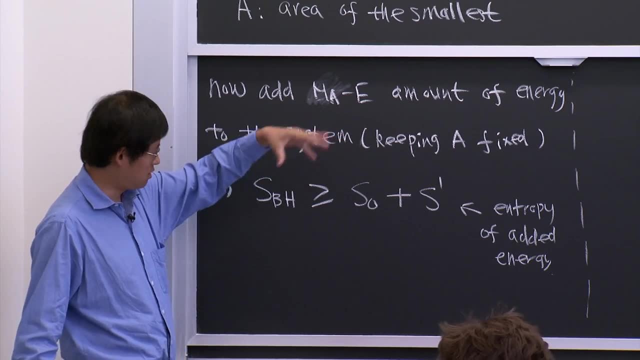 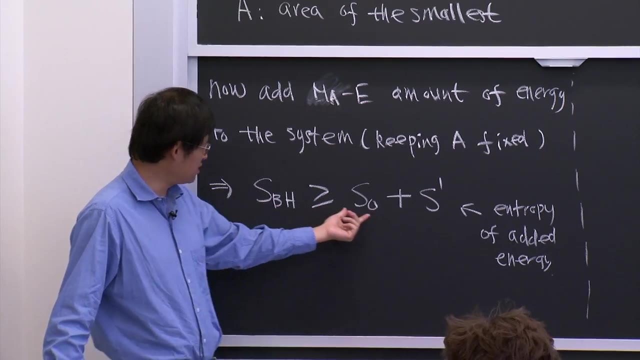 So the final. So you add this amount of energy to ma. so then you will precisely form a black hole of the mass ma and with the horizon area A. But this black hole entropy should be greater than S0, plus the entropy you added. 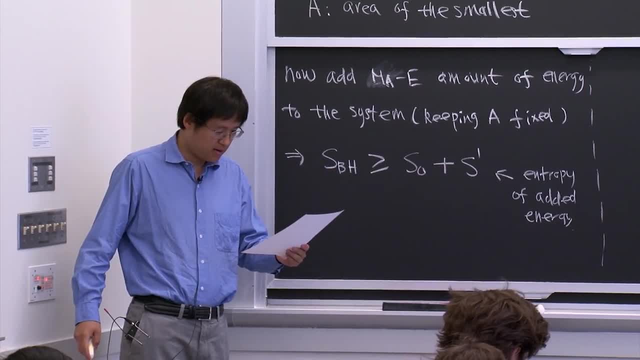 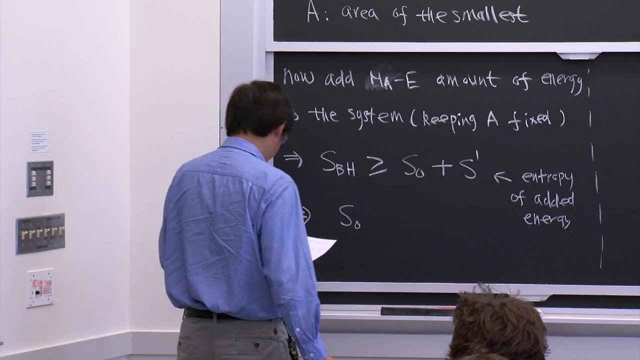 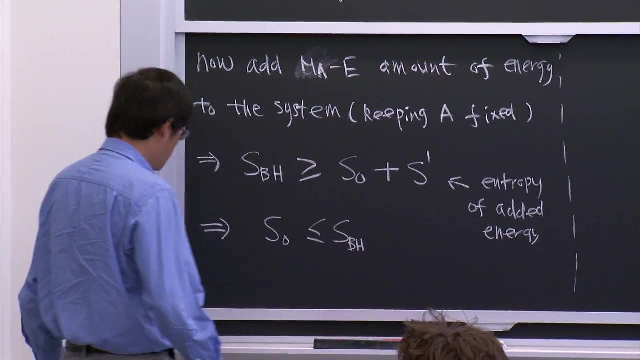 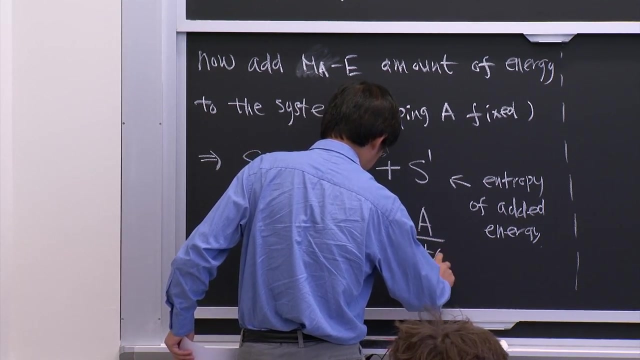 from the second law of thermodynamics. OK, So then that means the initial energy. your initial entropy must be smaller than the black hole entropy. OK, Must be smaller than a divided by 4 h bar g, newton. OK, 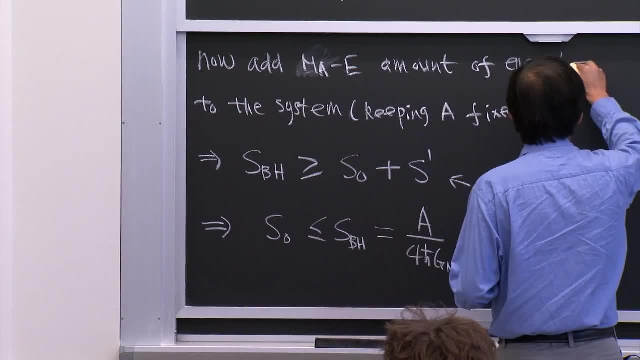 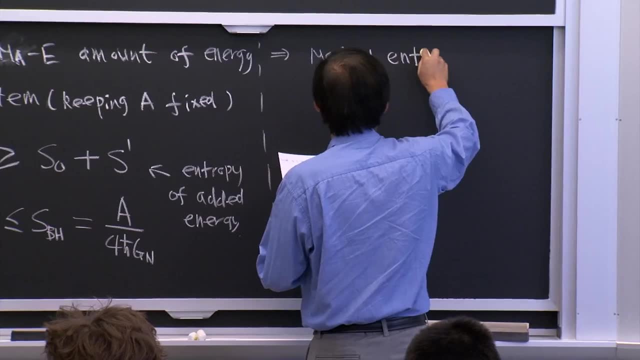 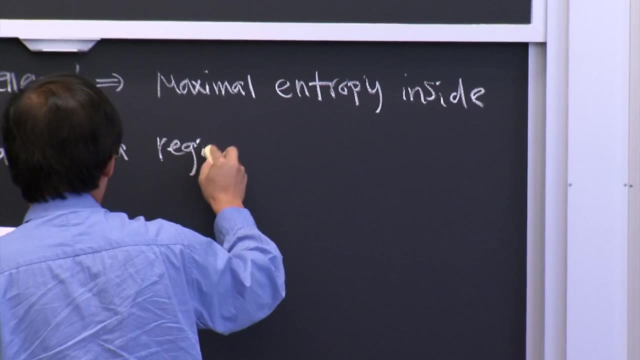 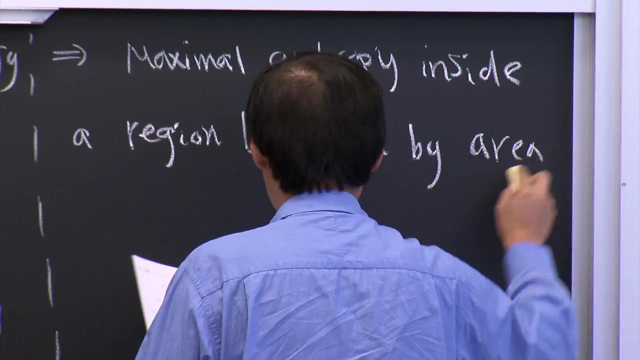 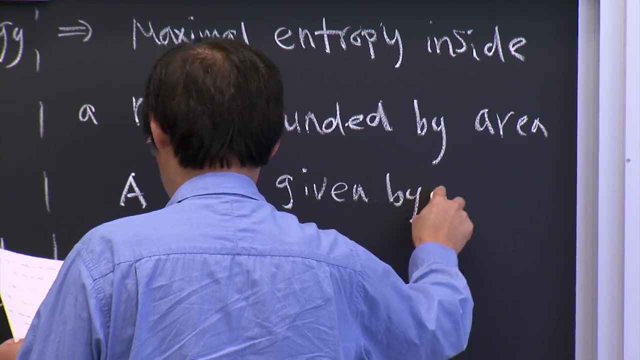 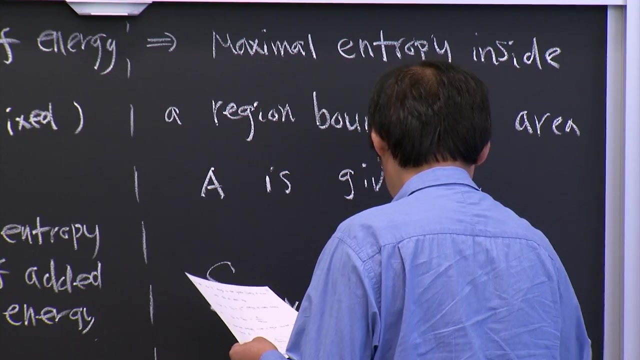 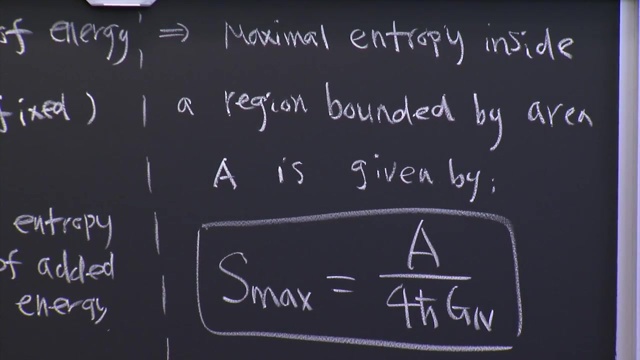 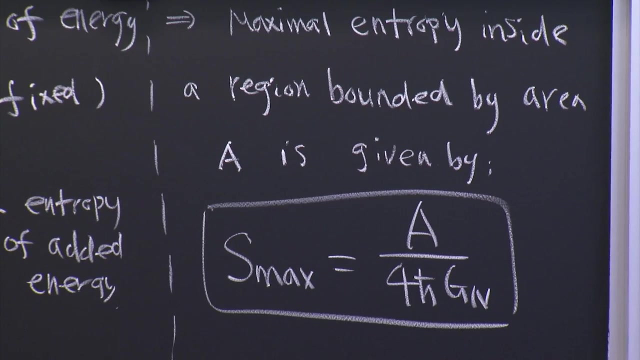 So this argument tells you that the maximal entropy inside a region bounded by area A is given by: OK, Yes, So will keeping A fixed add extra entropy to the system? Yeah, So in that case, why we don't have such a term? 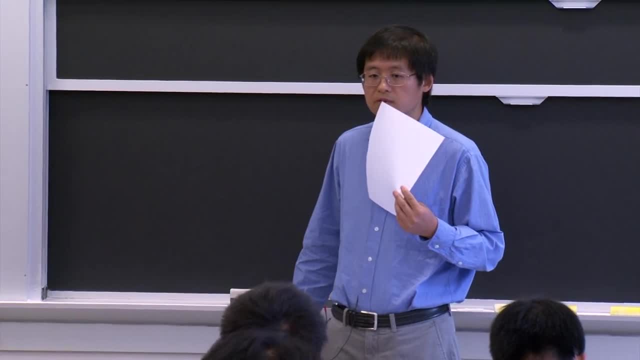 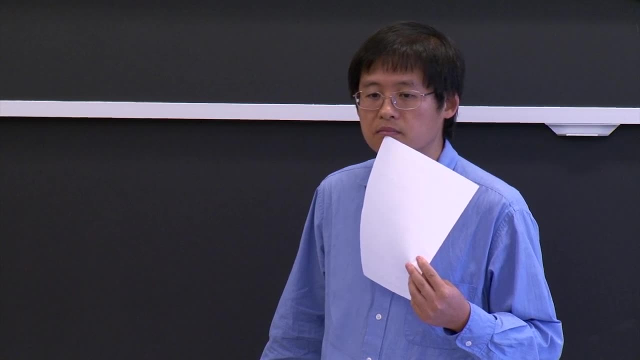 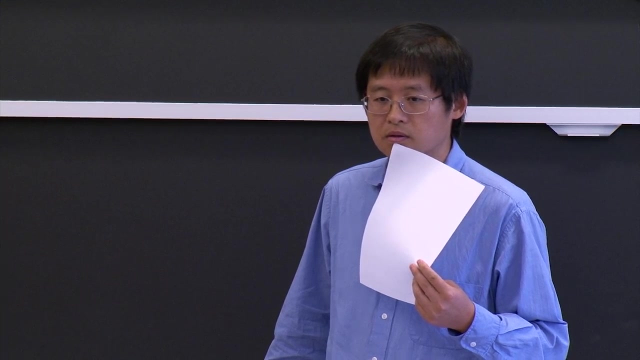 Sorry. So you said: well, we want to keep A fixed. Will that add extra entropy to the system? Yes, So according to the second law of thermodynamics, why will we claim that the entropy of black hole is greater than or equal than S0, plus S0?? 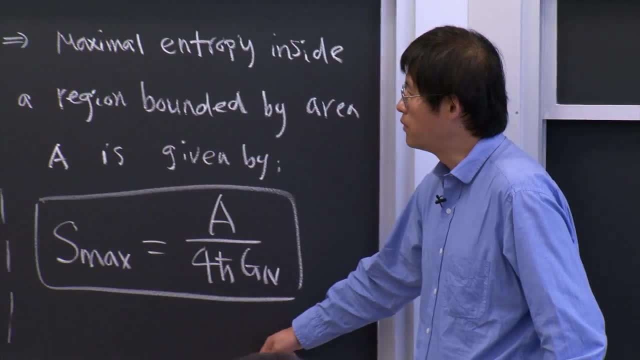 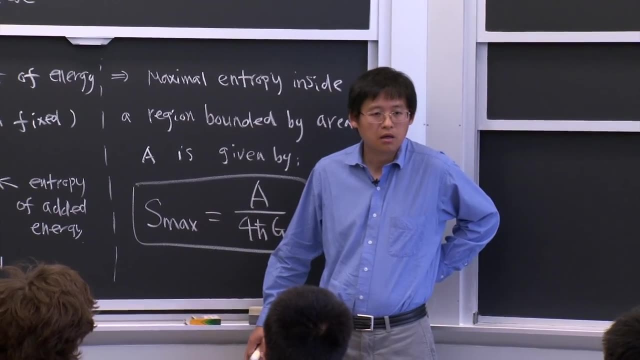 Yeah, Oh, OK, It's added energy. Yeah, because this is the energy of what I added. How about the extra energy that might be introduced by keeping A fixed? Because it's not a? Yeah, whatever it is. Whatever it is. 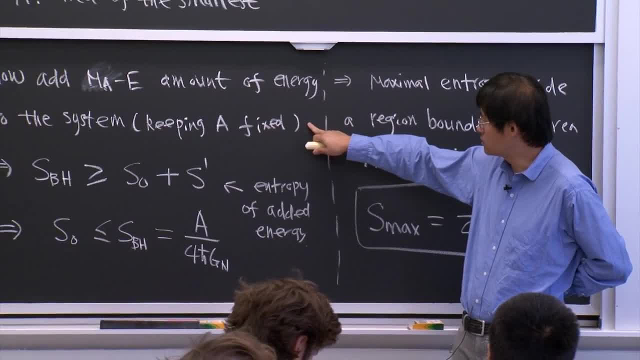 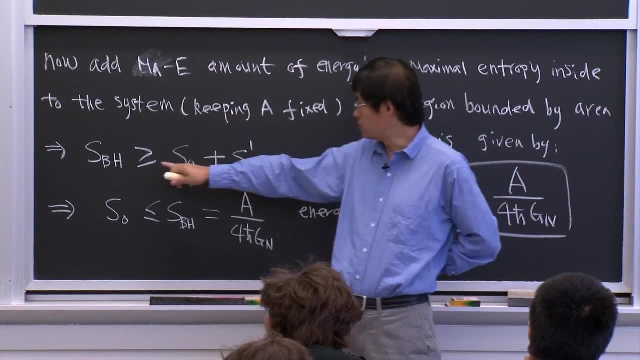 Suppose you can keep A fixed. Suppose you can keep A fixed, OK. OK Then whatever things you added to that, that total entropy must be smaller than the black entropy, because black hole is a phallal state. You said it's an isolated system. 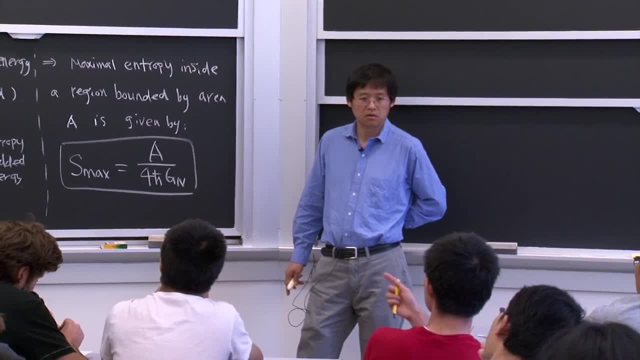 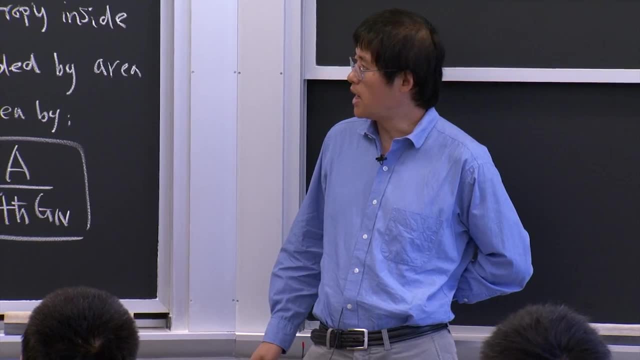 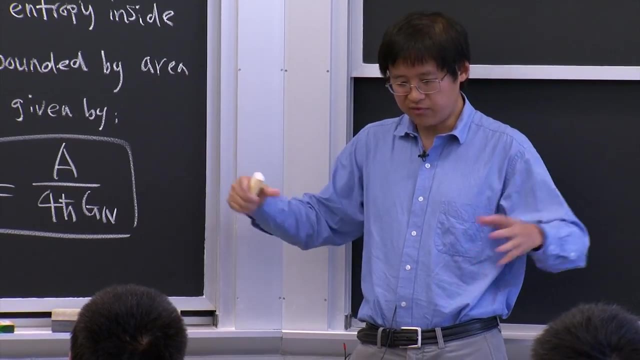 So with that, how can you make sure that A is fixed? Why is it not? Oh yeah, I'm just saying, we are doing a thought experiment. Imagine you can do this by keeping A fixed. Yeah, just say, you just put stuff in. 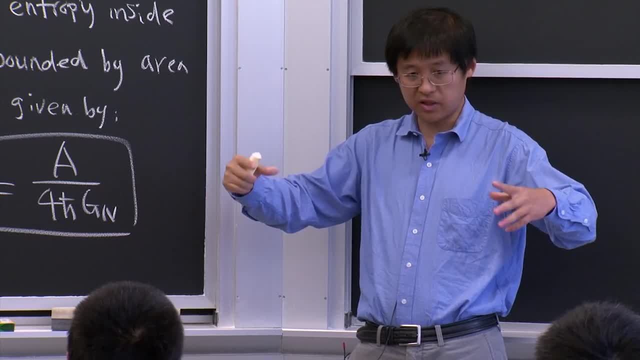 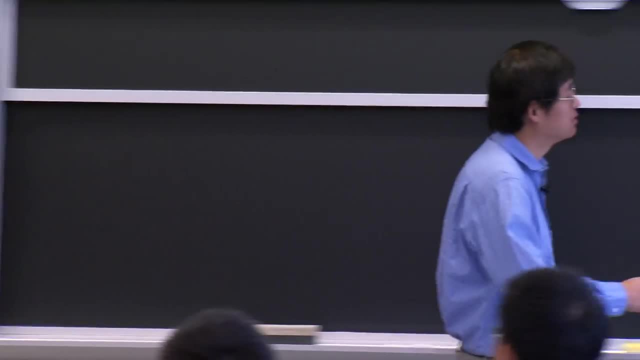 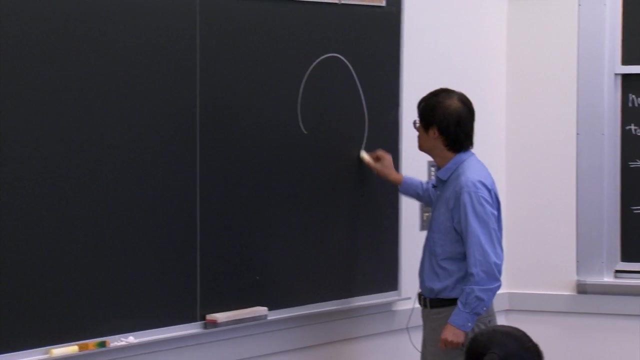 Into this region so that stuff does not come out. Yeah, just, you have some region A, Maybe let me do it here. You have some region A, And then there's some mass inside here, There's some energy stuff inside here. 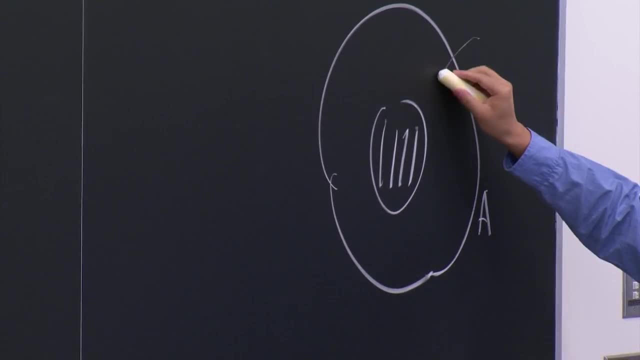 So this is region A, And then you just keep putting stuff in, Just keep putting stuff in. So this is the region A, And then you just keep putting stuff in So that those things don't come out of A. They don't come out. 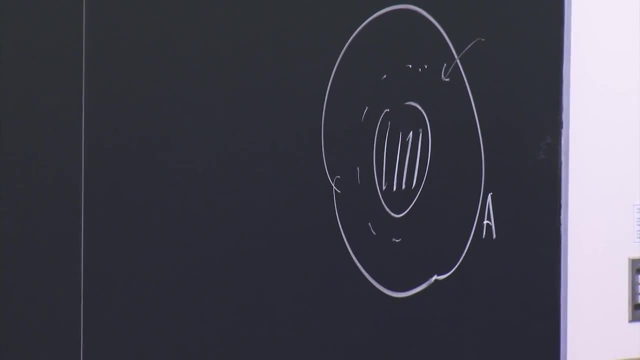 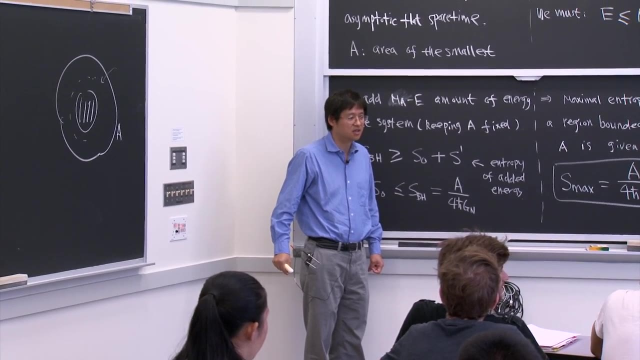 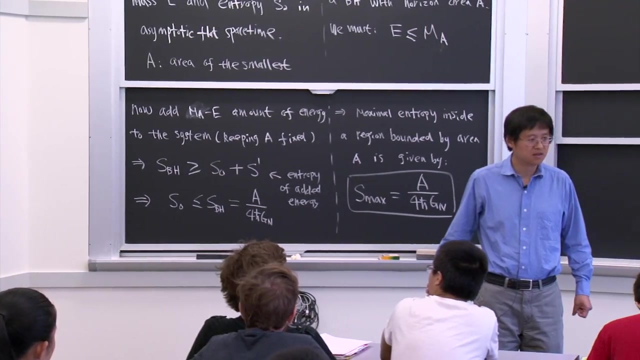 of this region. That's what this means. Then A is not the smallest sphere, Then A is not the smallest sphere at all. A is what? Not the smallest sphere that you close the system. So that's required, It's not required. 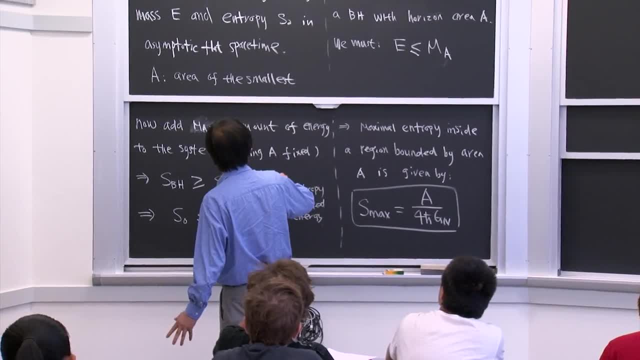 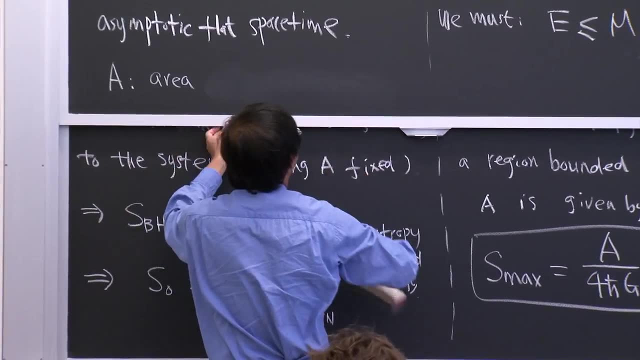 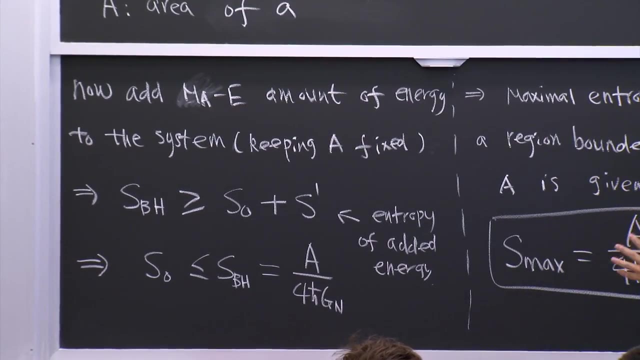 No, A is not the smallest sphere. increase system A. just yeah, maybe I should call it just A. It's the area of a sphere. Sorry, Yeah, Thanks. So just enough A to be a sphere that encloses the system. 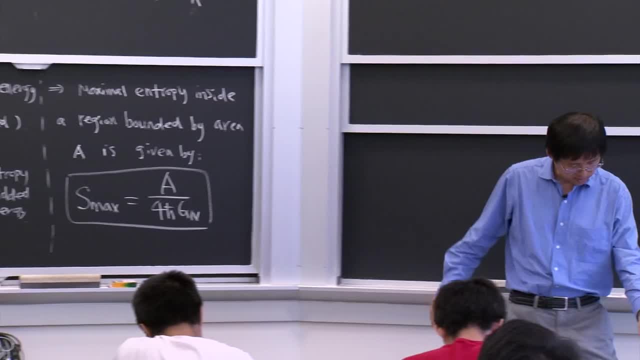 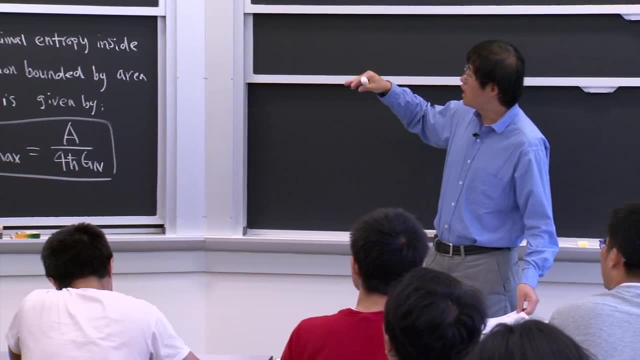 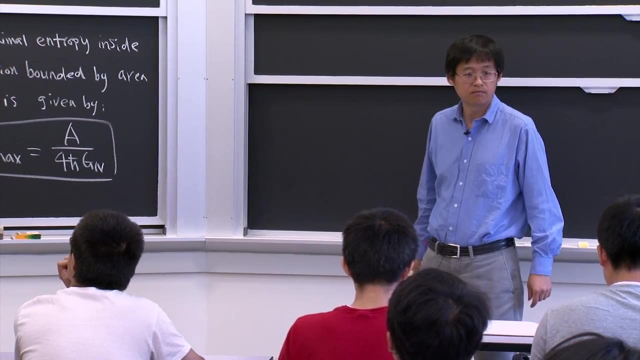 Yeah, So I should not put the smallest there for some reason. Yeah, no, no, no. Yeah, it should not be smallest, Just A. is any sphere? Yeah, Some sphere which encloses the region? OK, Yes. 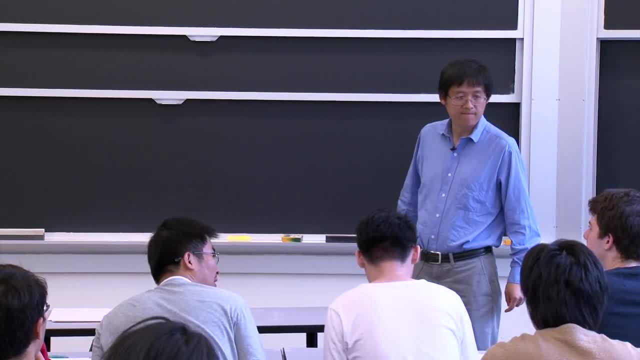 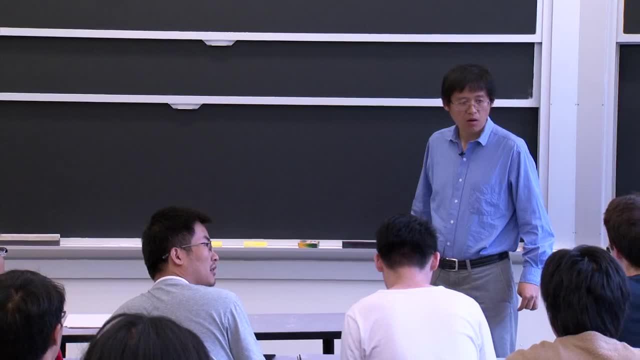 So it seems that this argument implicitly assumes that, in order to add entropy, that sort of corresponds to adding some amount of energy. But is it possible to add entropy to the system without adding energy to the system? Oh, you can. You can then just make it even more. 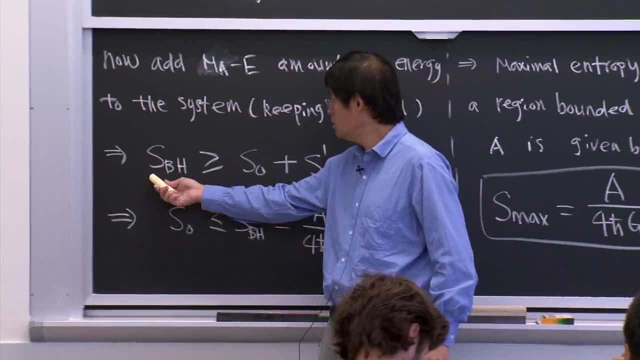 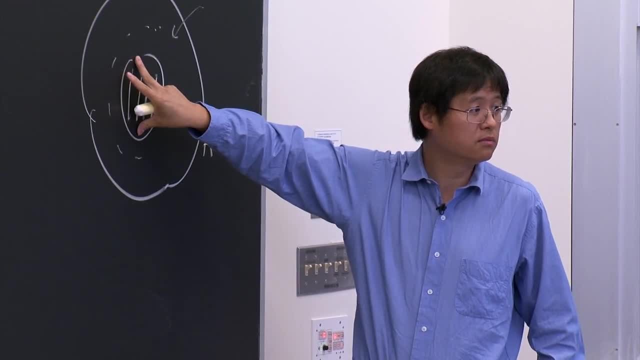 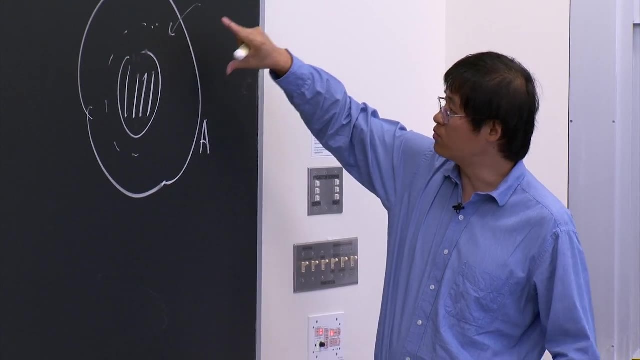 Whatever it is, this is a final state. So the basic assumption of this is that if you can put stuff inside this region, Yeah, Yeah, Whatever is inside, Yeah. The assumption is that the maximal stuff you can put inside the region is a black hole. 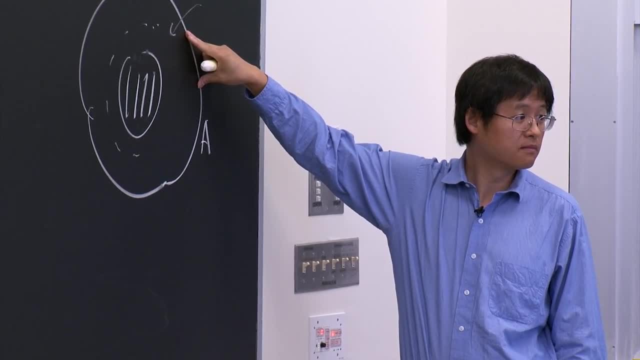 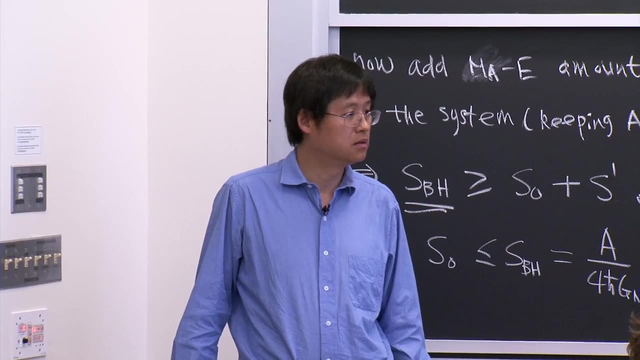 It's the horizon area. Well, I guess what I'm confused about is that it seems that I certainly believe when you say that you can't have a certain amount of energy in an area, But I'm not sure why you can't have a certain amount of entropy in an area. 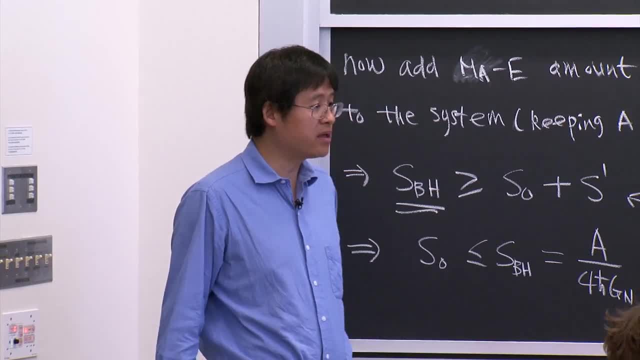 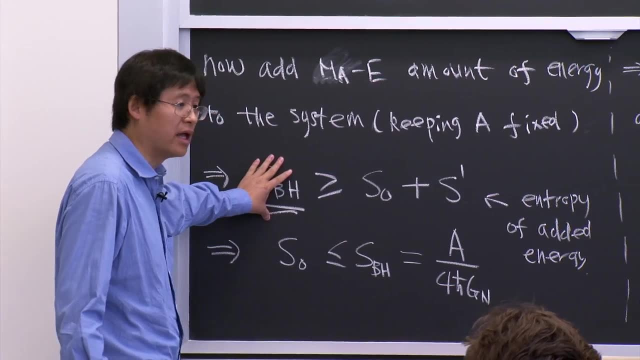 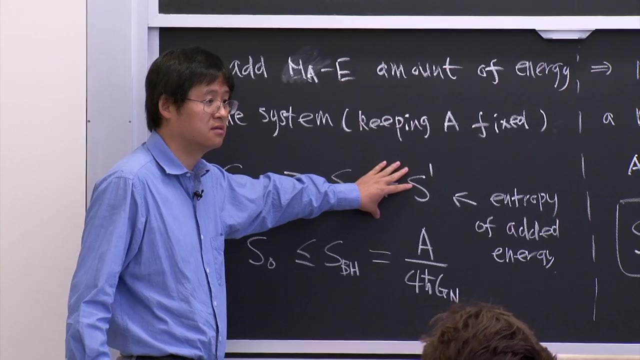 If energy and entropy are not. No, I'm not making that assumption. The entropy is just a consequence. It's a consequence of that. This is a final state entropy. The final state entropy is always larger than the entropy of your initial state. 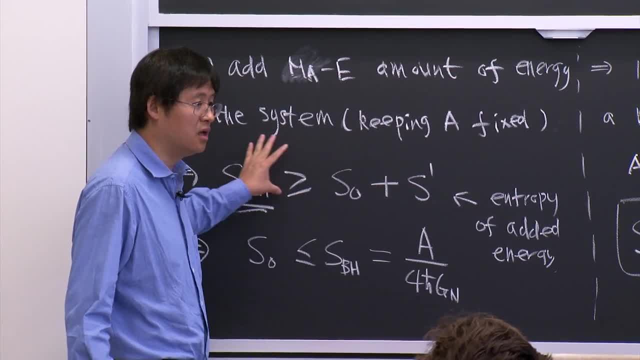 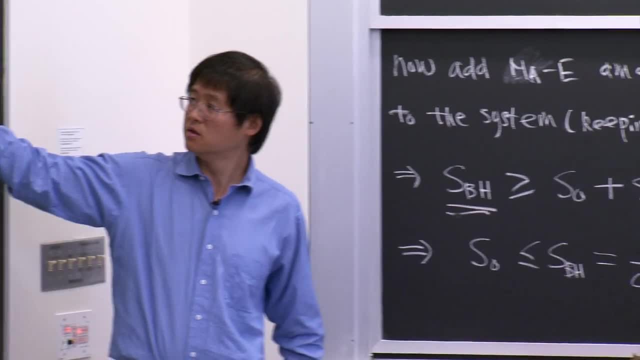 OK, Sure, Yeah. Yeah, Entropy is a derived. This equation is not an assumption, It's a derived. Yeah, The assumption is that the black hole is the maximal. It's the most massive object you can put inside this region. 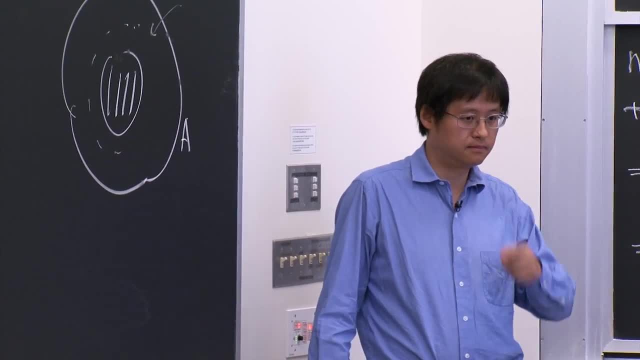 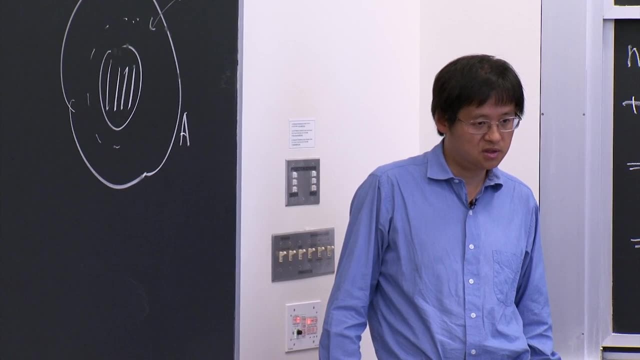 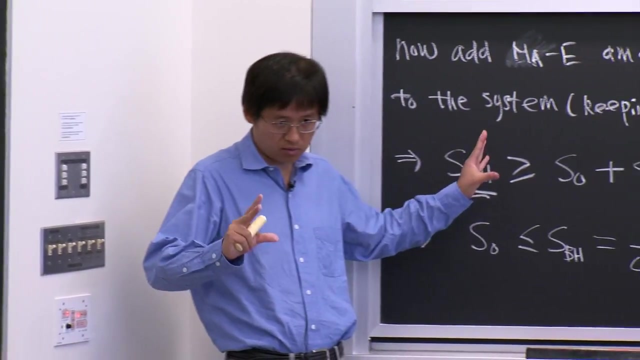 Sure, I understand. Yeah, But you can't have a less massive object with more than that entropy. You can't have a less massive object with entropy that is more than that value inside the same region. This is ruled out by this. Once you get this equation, then you don't ask about the mass. 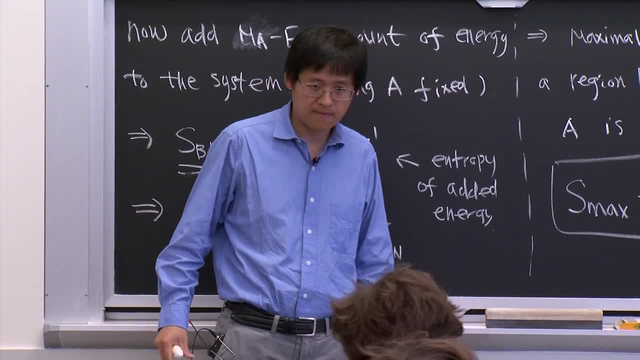 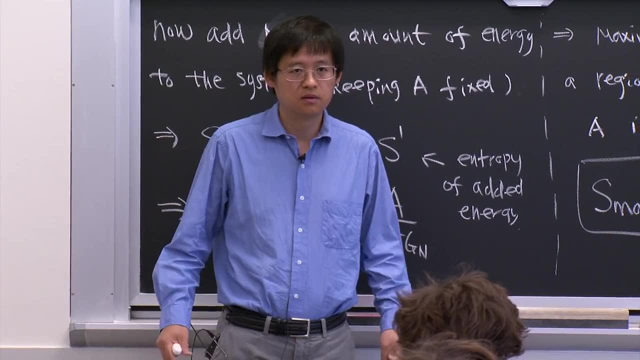 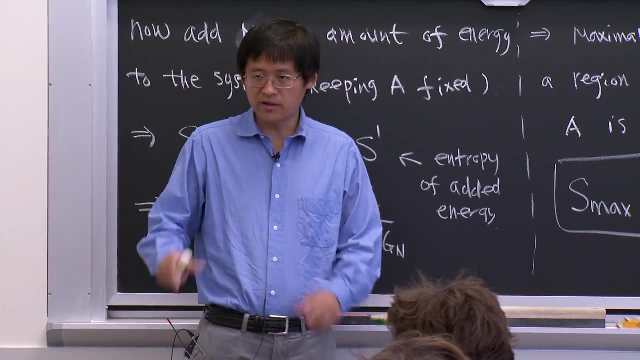 Any entropy must be smaller than this value. Any other questions? Yes, How do we keep track of the area? I mean, doesn't space between them work, the way that the horizon approaches, Right? So that's why I say this is a little bit. 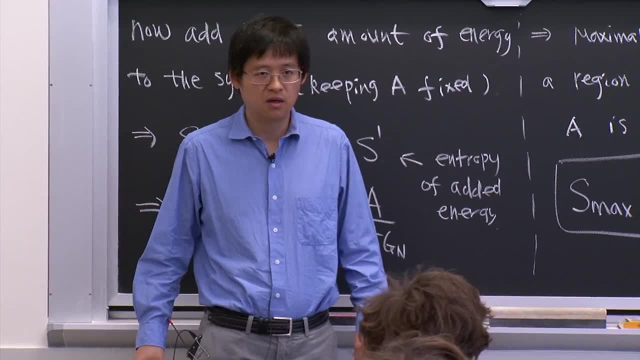 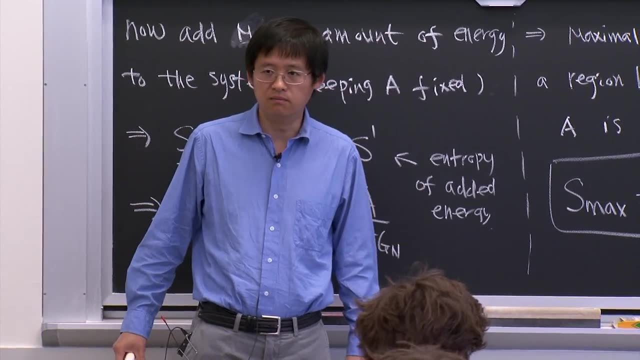 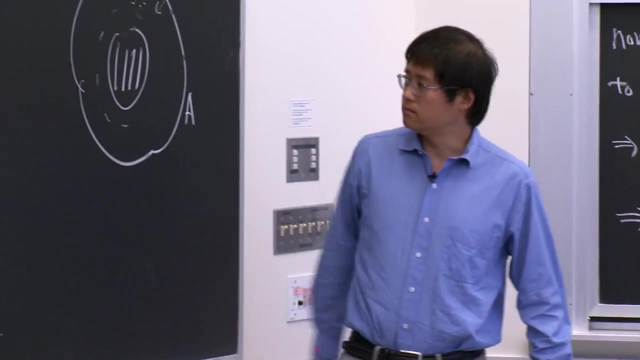 of a heuristic argument, And that's why I say this is a heuristic argument. Yeah, Indeed, you have to be a little bit more careful about that. Yeah, But say, if you are: Yeah, The key thing is about the area. 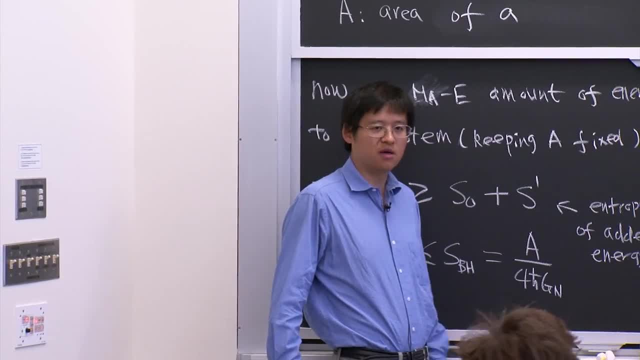 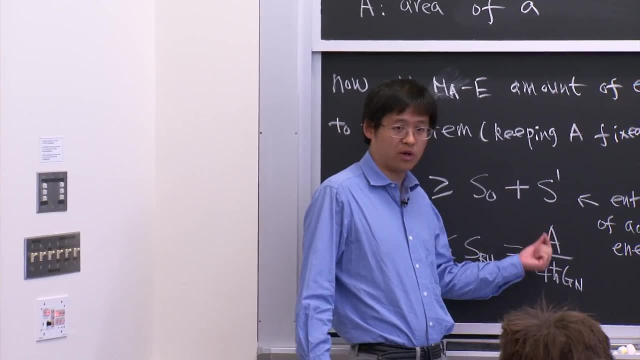 And this all the one cautions one maybe have to think about it when you include the quantum corrections et cetera, the back reaction et cetera. Yeah, But the key thing is the area. The black hole must be proportioned to the area. 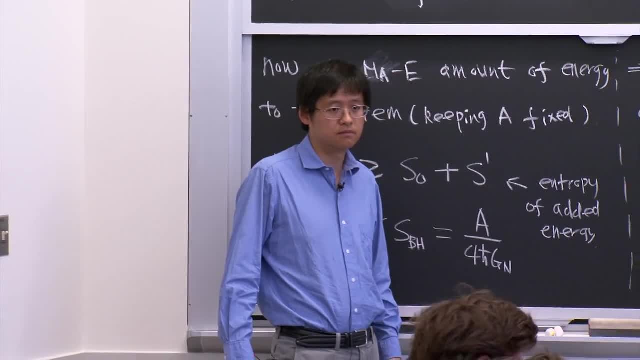 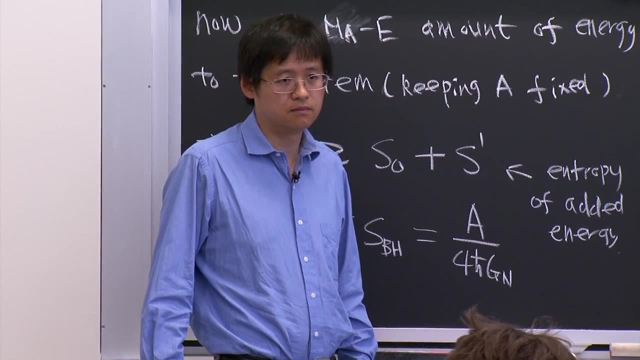 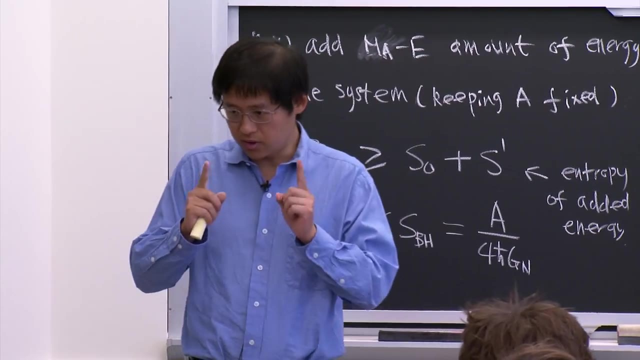 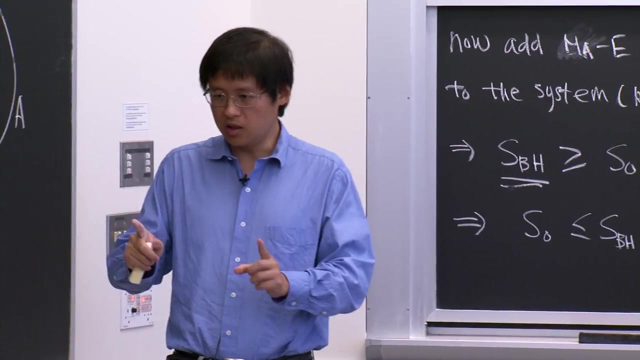 Well, this is derivation based on the assumption that the area of the horizon of the black hole is only based on the mass. Oh yeah, yeah, yeah. So let me say again: there's a true nature of this argument. The first nature of the argument is the maximal energy. 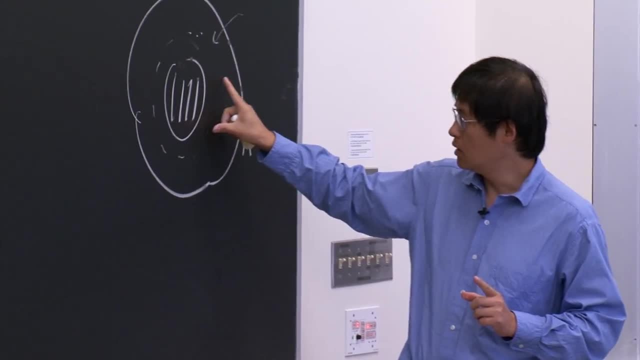 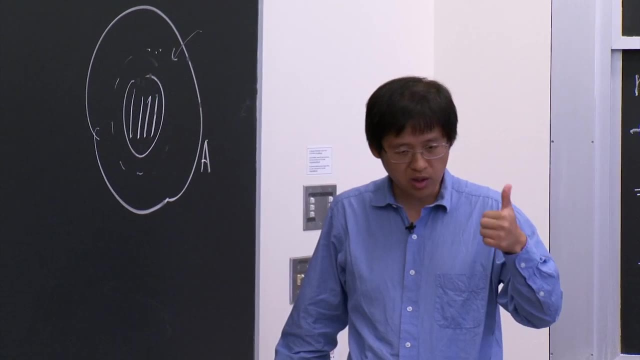 you can put inside the region is a black hole whose horizon area is given by the area of this region. This is assumption Yeah. this is assumption Yeah, because we know in the GR, any sufficiently massive thing will collapse to form a black hole. 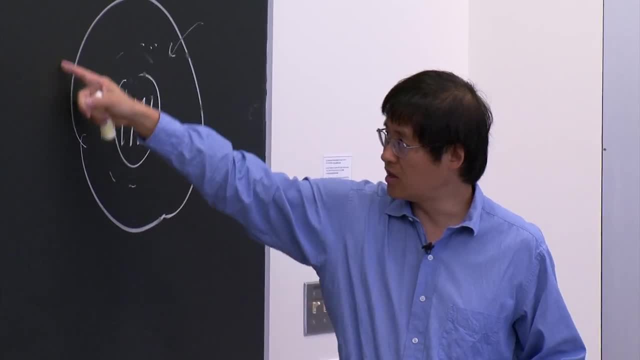 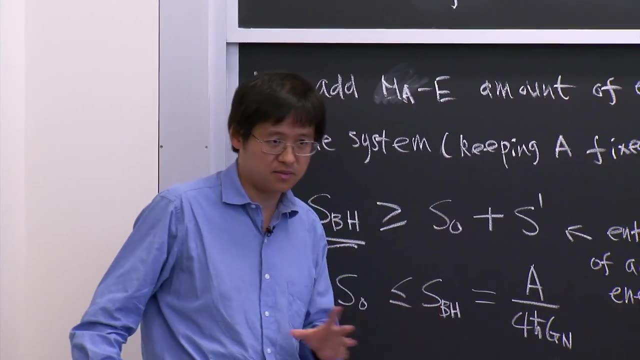 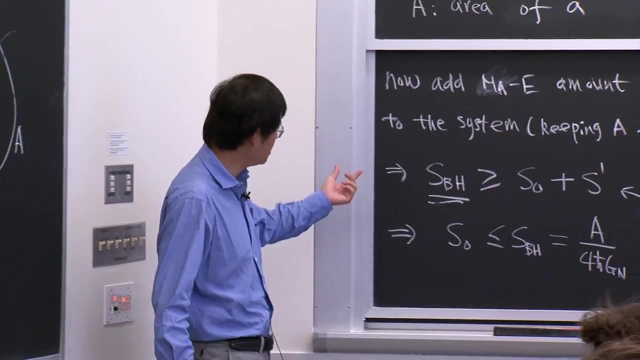 Yeah, OK, And if you have more mass, then the horizon area will be outside, And then you will be outside this area. You can no longer keep this fixed. Yeah, So that's the first assumption. So with that assumption, then just: 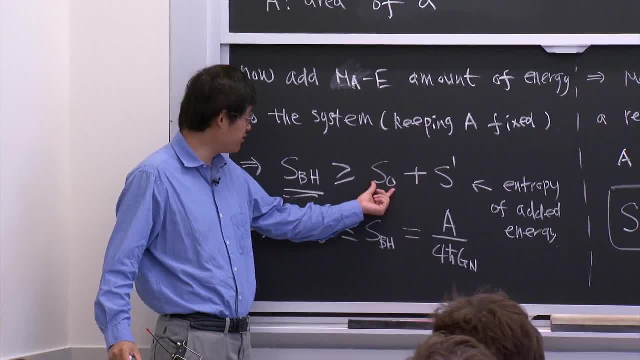 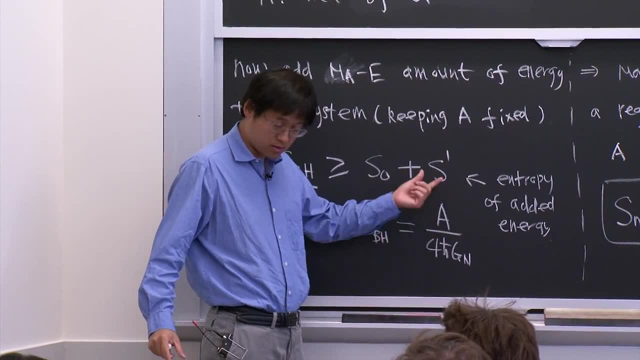 follows from the second law of thermodynamics, Because this is whatever the entropy of the matter inside, Then this is whatever the initial entropy of the energy you need to put it in to make it into a black hole, And then that must be smaller than the entropy. 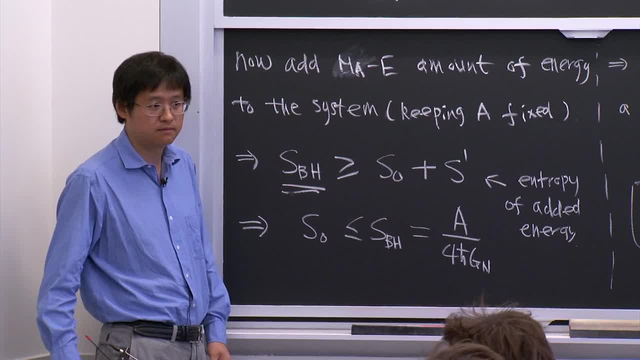 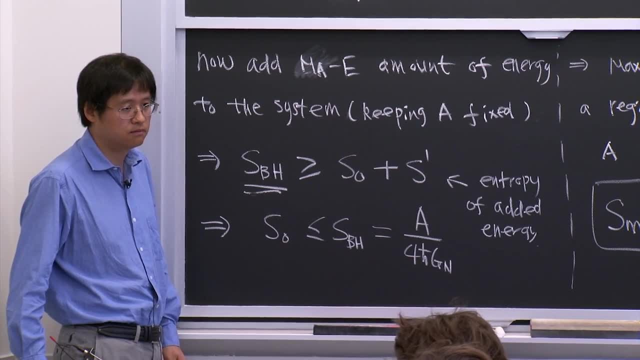 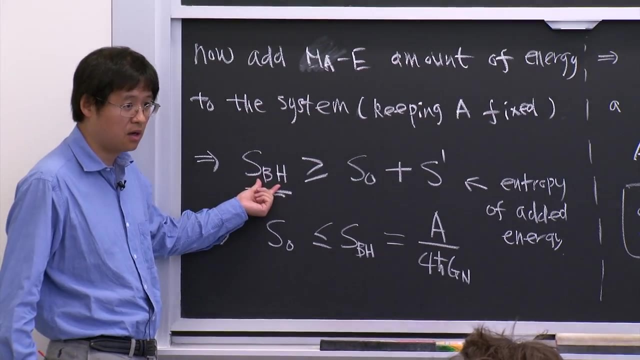 of the final state, which is the entropy of the black hole. But my question is that by keeping A fixed, you might introduce the actual entropy into the system. Yeah, It doesn't matter as far as the black hole is a final entropy state. 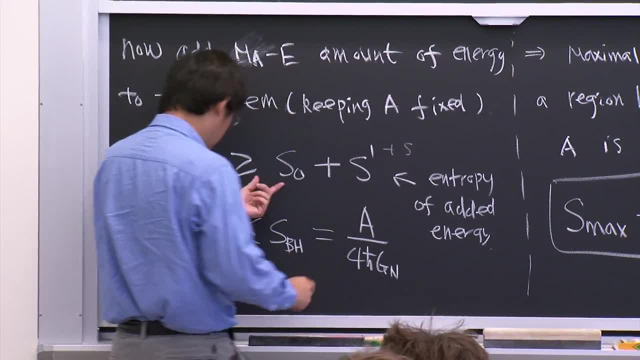 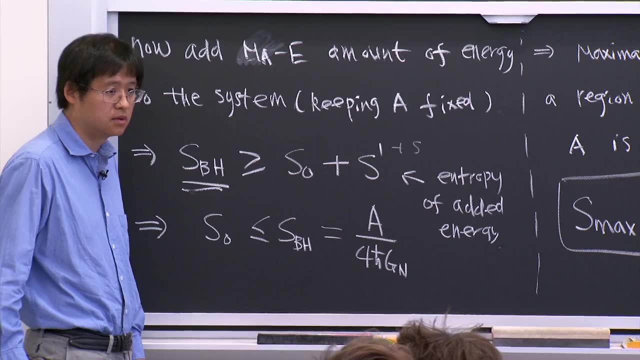 What you are saying is that there might be some other things here. It's fine That does not change the direction of this Entropy might be negative, Yeah, But I'm not sure to just do it. No, Whatever it is, this is my initial. 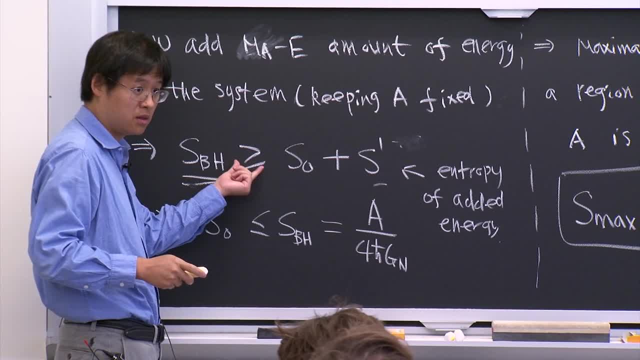 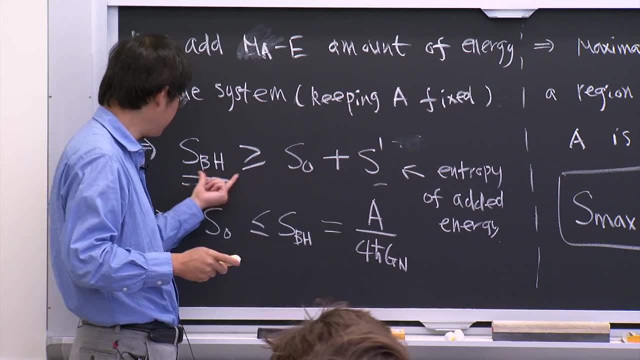 So that's why this is inequality here. This is not equality, Inequality, And we are just using the second law of thermodynamics. This is your initial state entropy. This is my final state entropy. This must be greater than that. We are not asking the specific process. 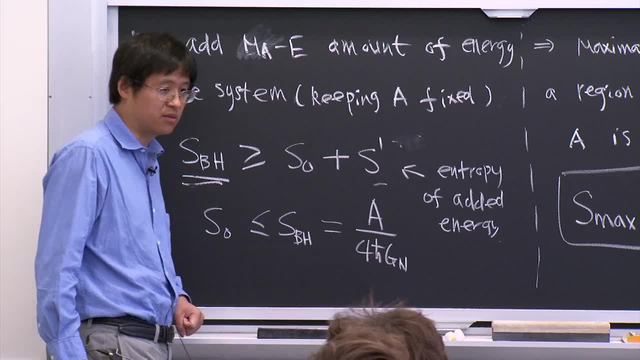 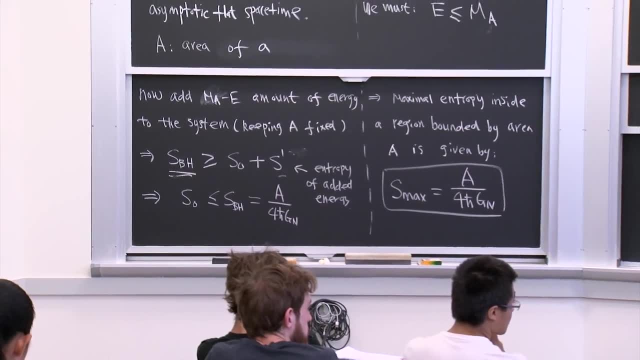 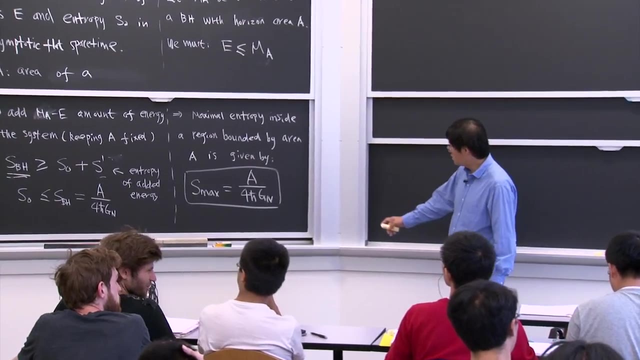 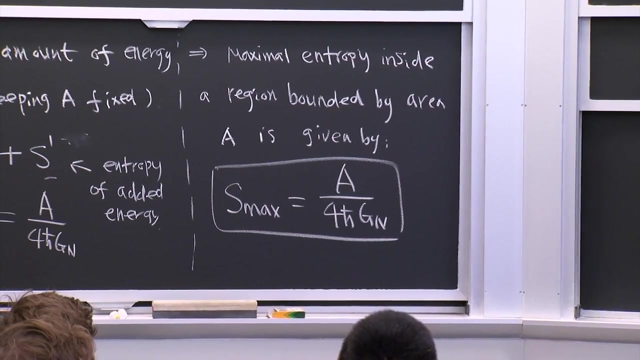 We are not asking the specific process. Yeah, Just the final state has to be greater than the initial state. Good, OK, So now let's see what we can try to go a little bit further from here. So now let's recall: 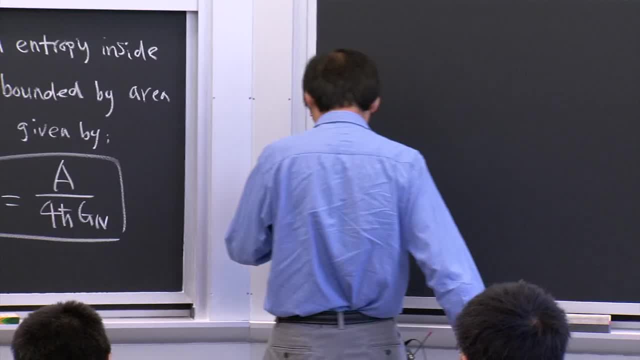 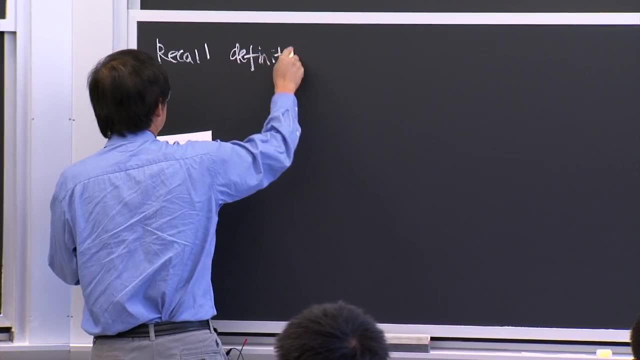 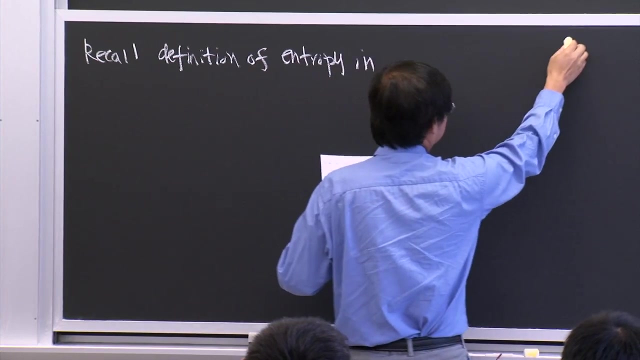 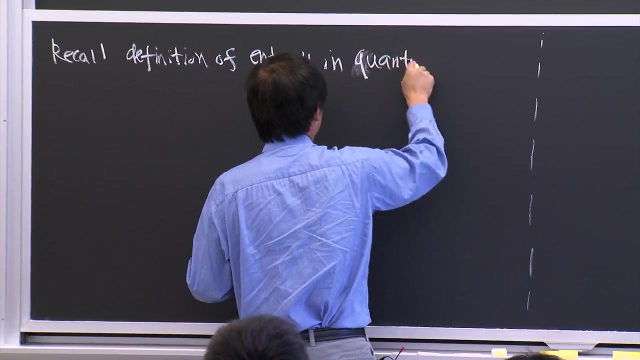 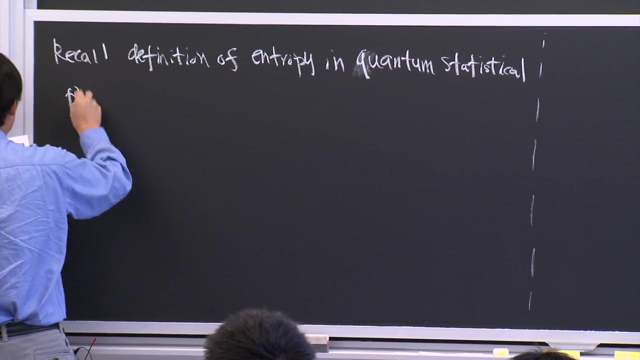 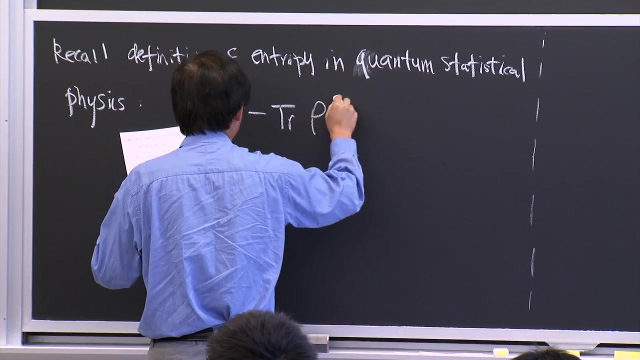 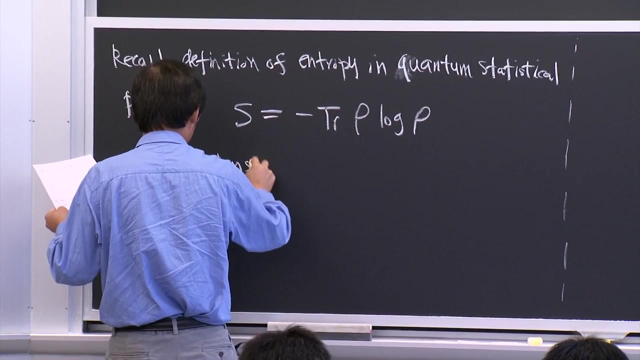 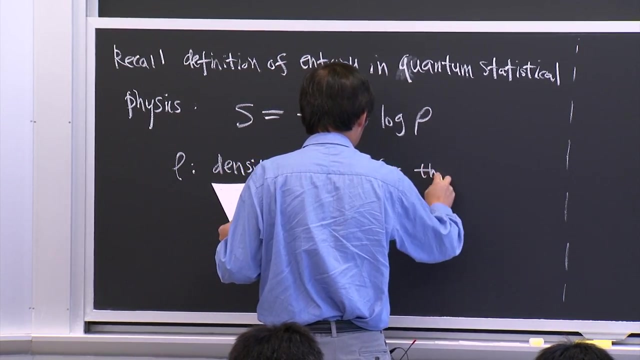 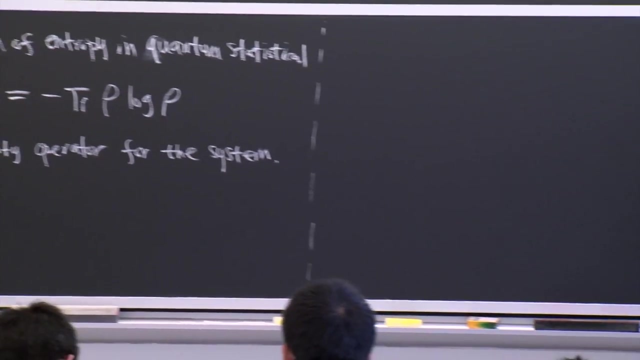 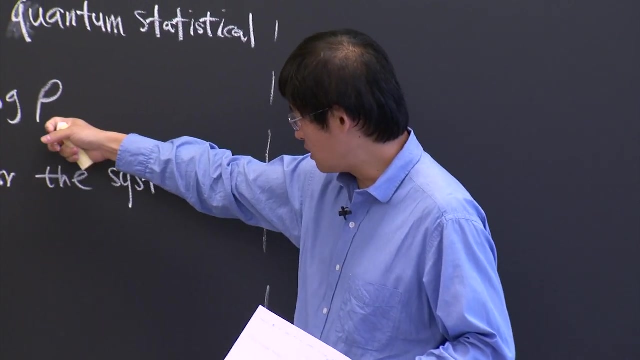 So now we really treat the black hole. We treat the black hole as a quantum statistical object. So now we recall definition of entropy in quantum statistical physics. OK, So if you say have some system and the state of that system is described by some density, 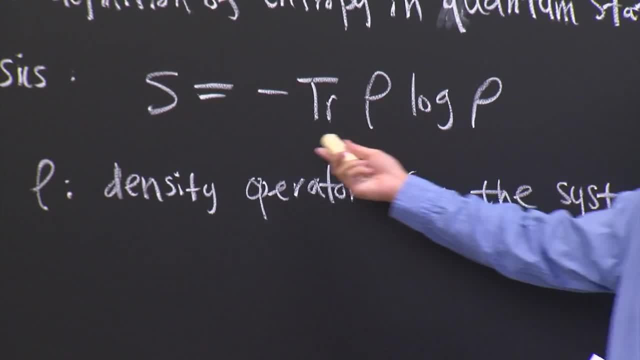 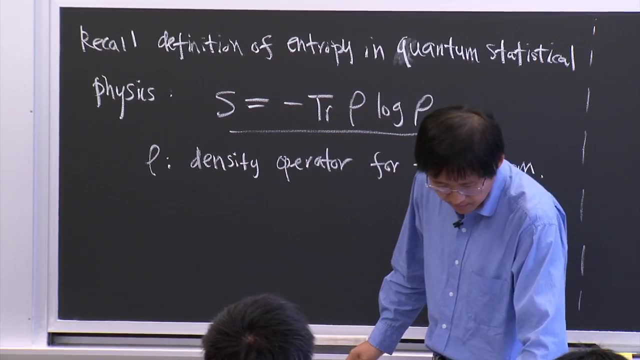 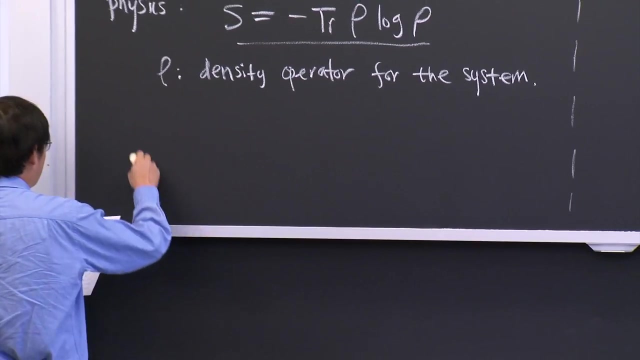 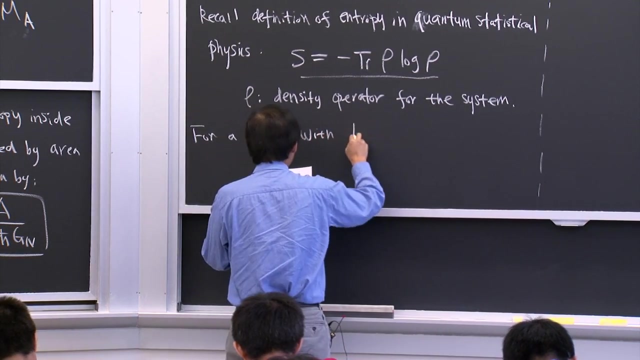 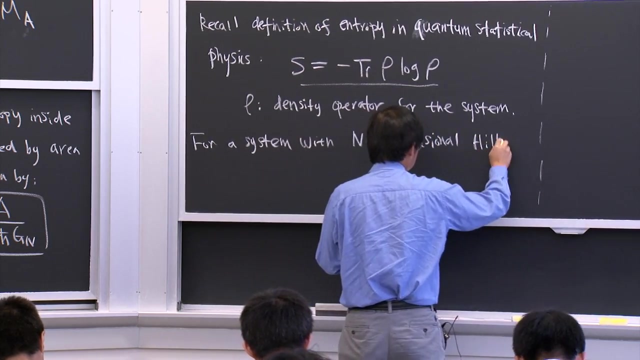 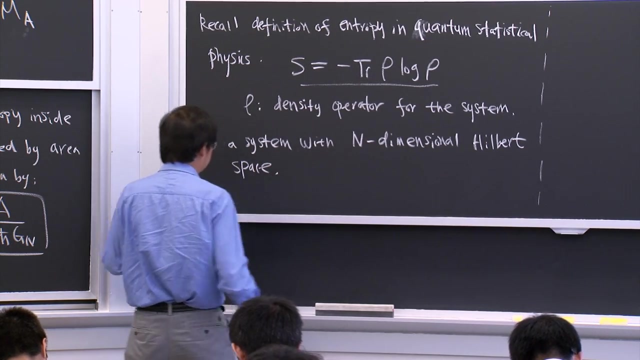 operator or density matrix, and then the entropy of that system is just given by this formula, Just given by this formula. OK, In particular, in particular for a system, it's given with n-dimensional Hilbert space. OK, So this is the n-dimensional Hilbert space. 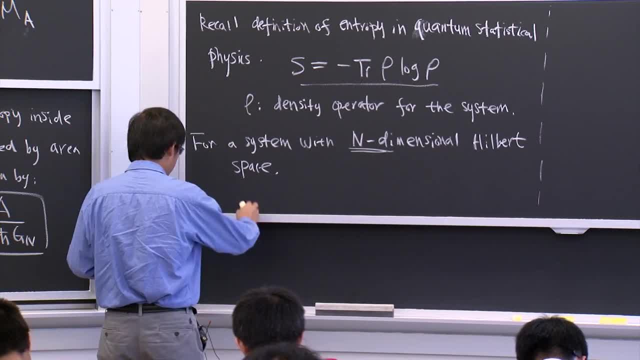 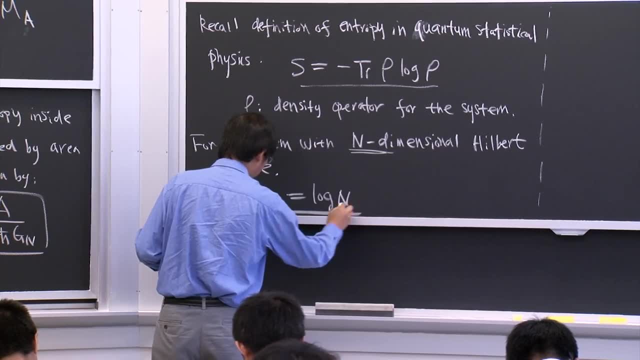 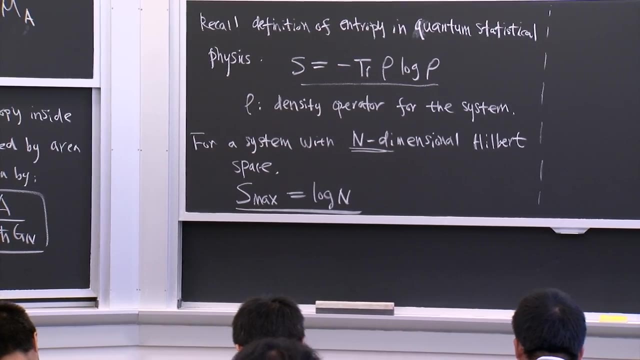 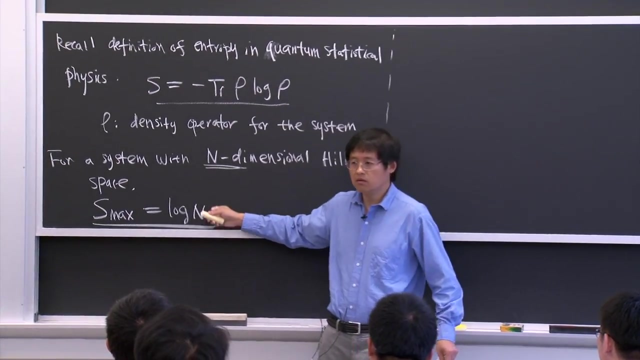 OK. This is a dimension of the Hilbert space. That S max is log n OK. OK, So the maximum possible entropy you can have is log n OK. Is this fact familiar to you So you can convince yourself? the maximal entropy? 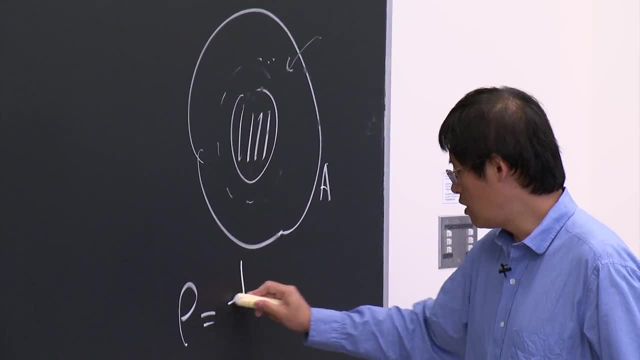 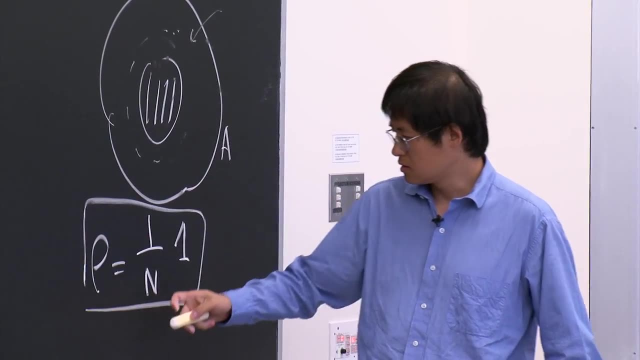 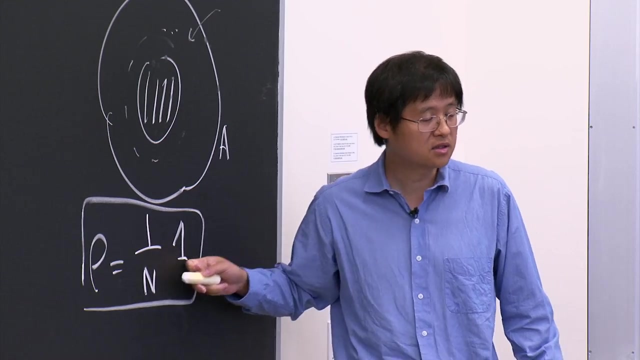 is realized when rho is just given by 1 over n times the identity matrix. OK And so? So this is the density matrix, which have low information, because every state plays the same role And this state. then you can plug in here and give you log n. 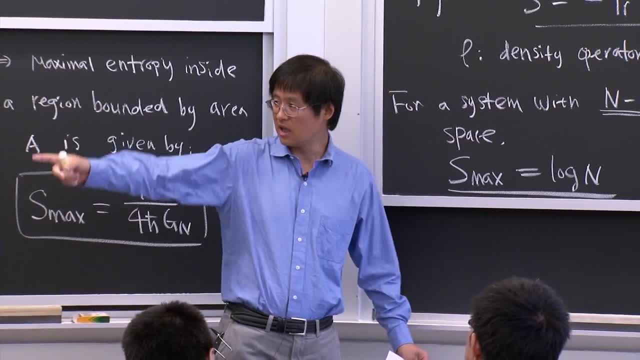 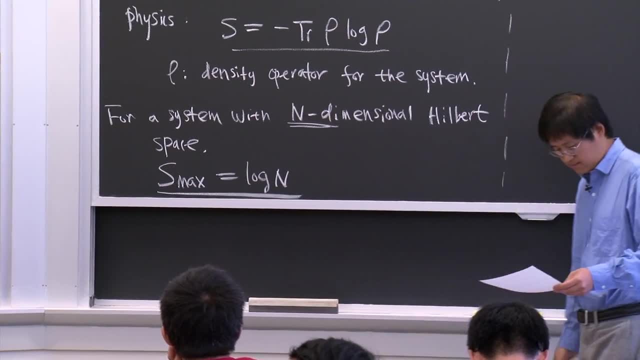 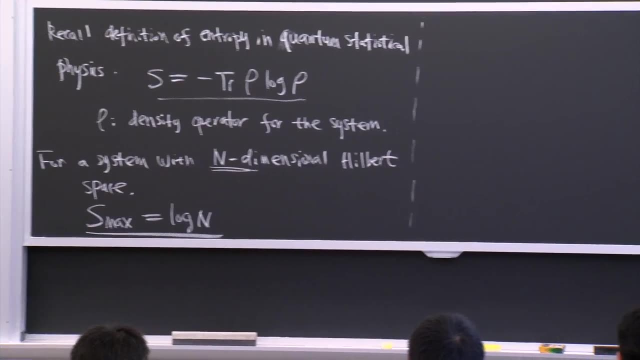 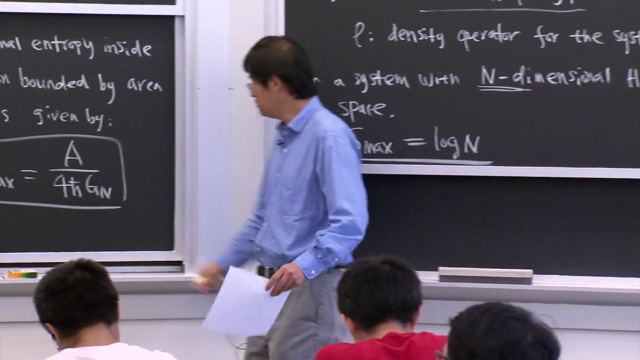 And the maximal entropy means you have minimal information. OK, And that is the state with the minimal information. And you can also just prove yourself using some algebra. But this is a physics, A physical argument for this. So now, if you compare with these two formulas, 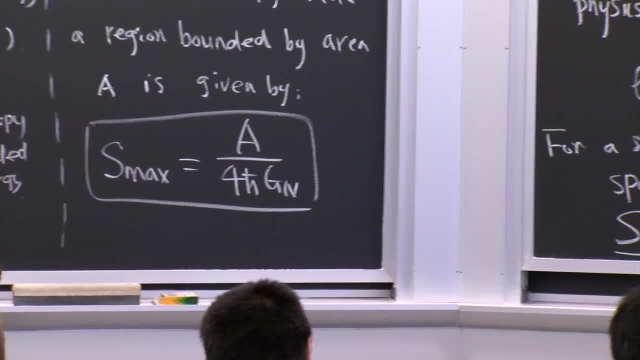 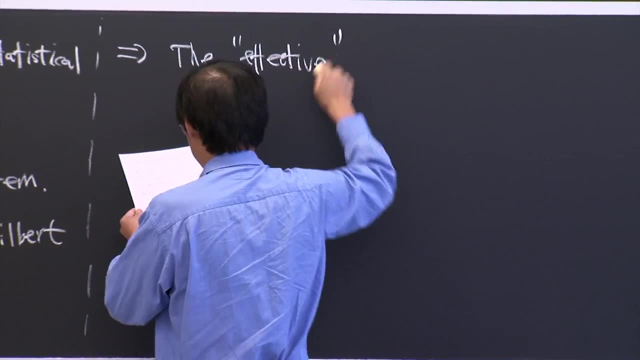 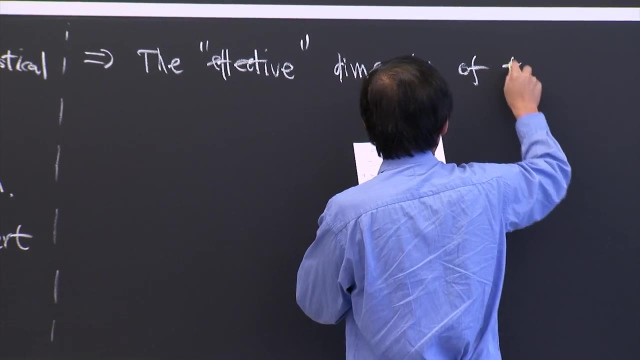 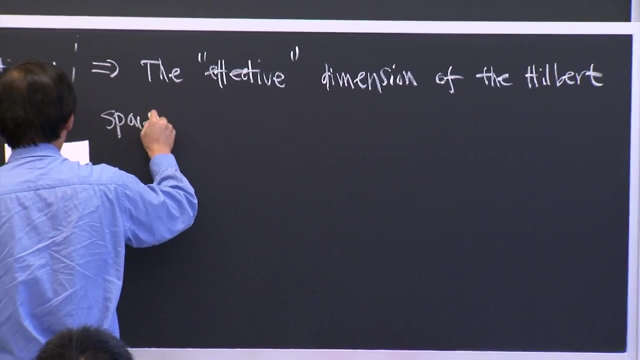 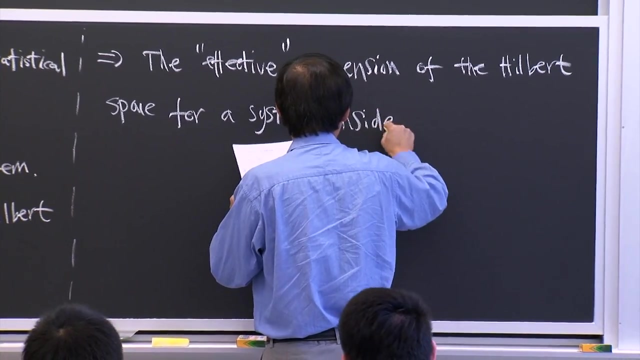 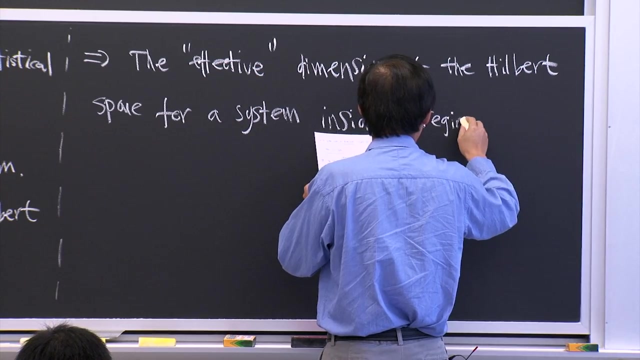 then we can draw a conclusion. It's that the, so let me add a word called effective. Effective dimension of the Hilbert space. OK, It's for a system inside a region of area A is bounded by: OK, OK, 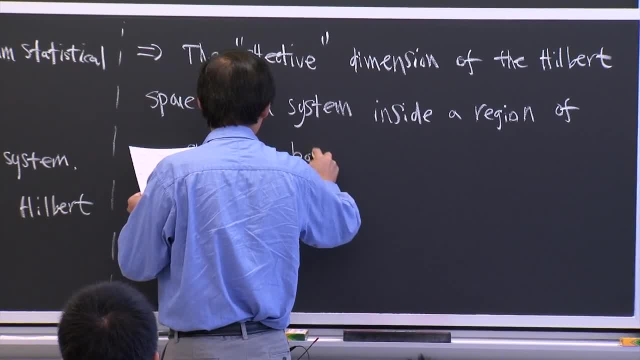 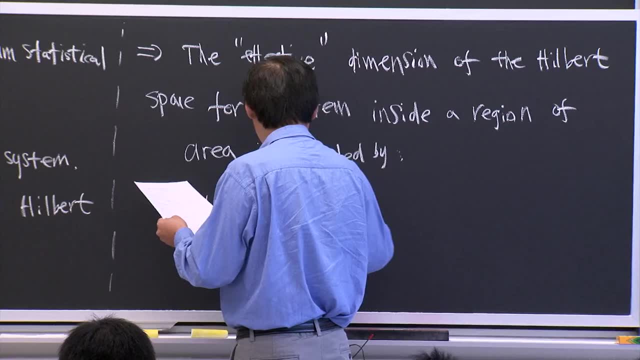 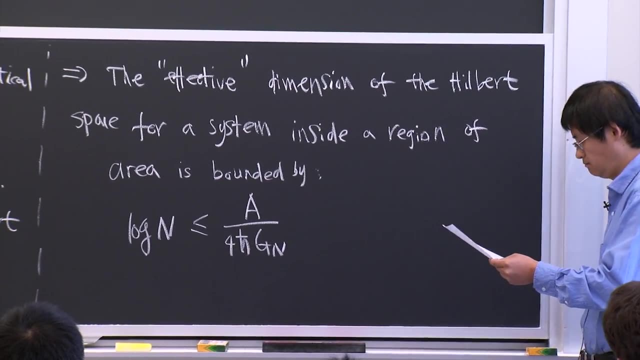 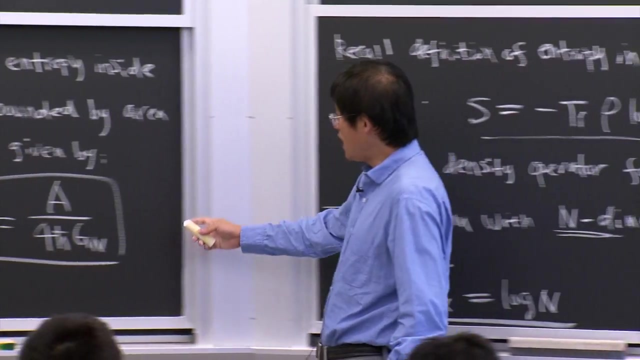 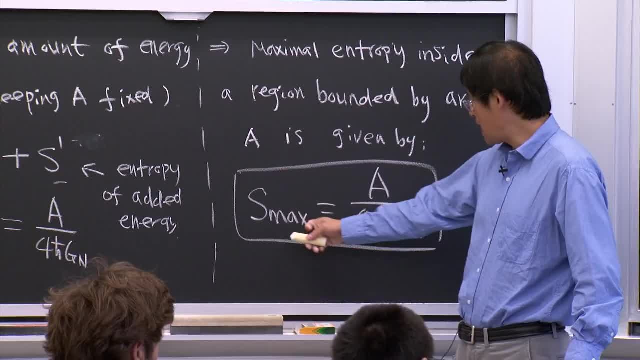 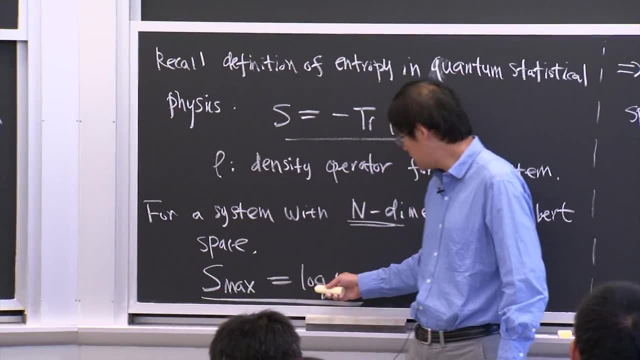 can put inside of this region of area A. that's the maximal entropy you can have. And if you have n degreed freedom, then the maximum entropy you can have for this n degrees, which is log n, then that tells you that log n must be smaller than this. OK. 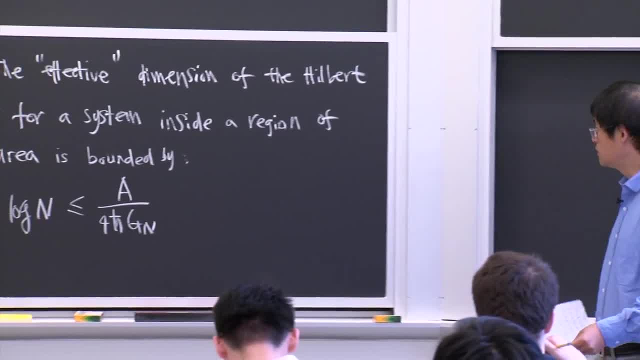 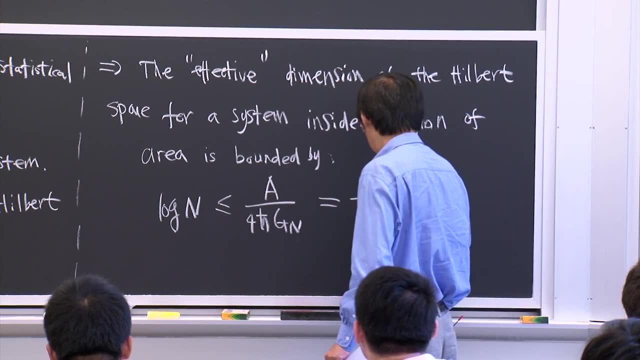 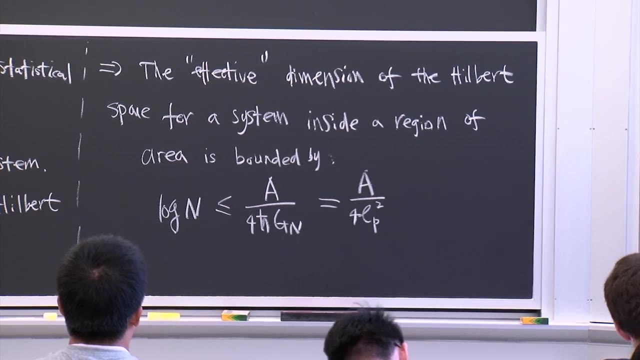 Smaller or equal to that, And so let me write this in terms of the. so this can also 4h. bar n is also Planck length squared, So it's also 4 times the Planck length squared. So for this part, usually, 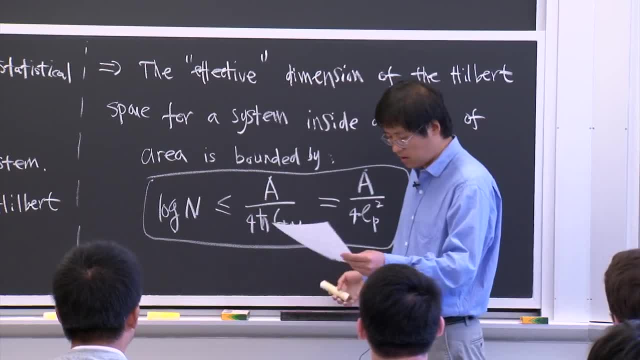 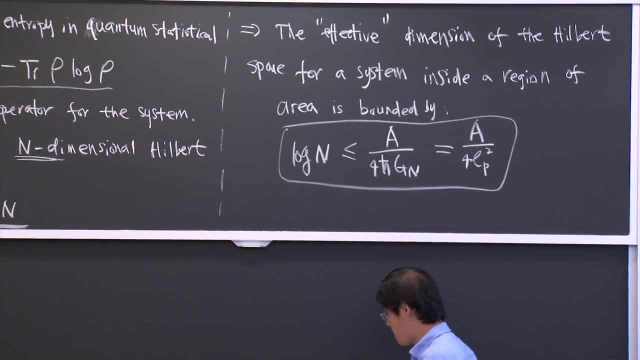 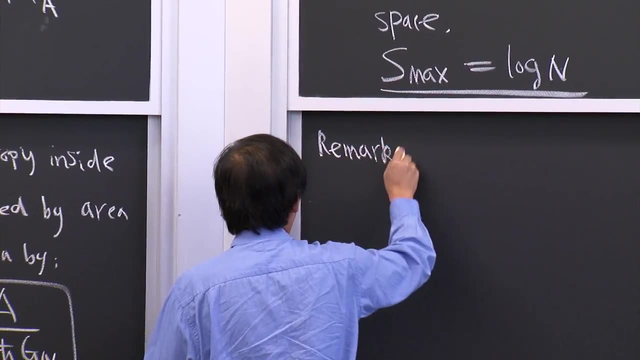 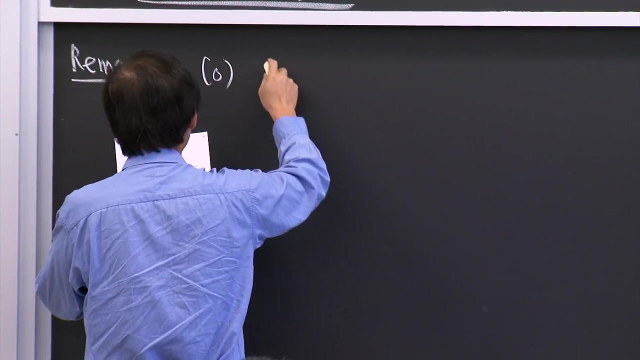 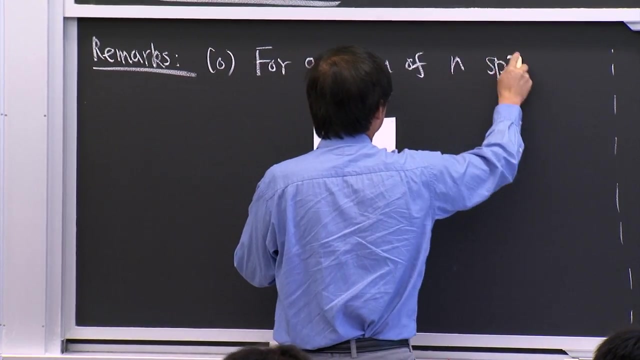 cube of space can be even infinite. Yeah, and let me say that. So that's why we need effective. So now let me make some remarks. So zero remarks. is that for a system of n spins, say n spinning off particle? 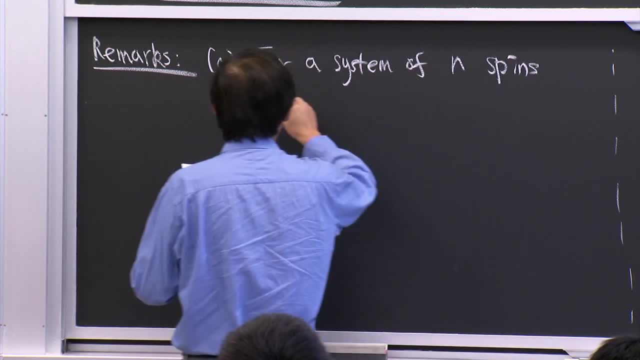 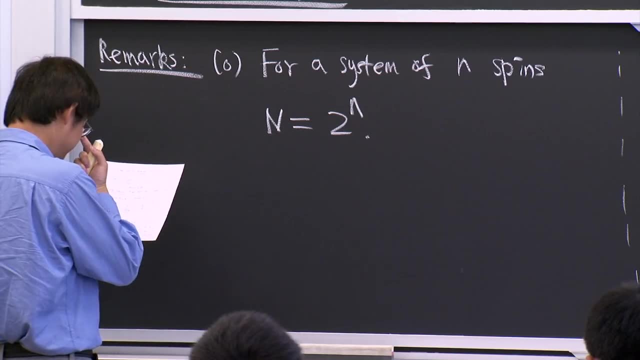 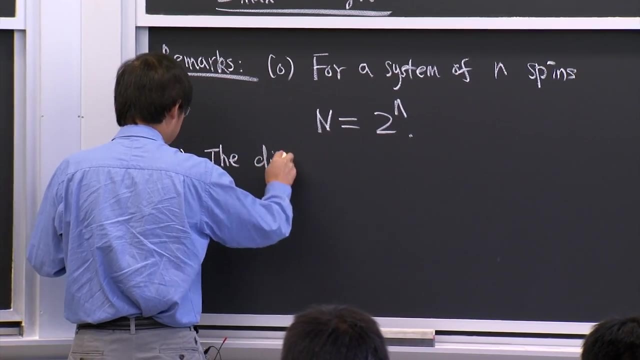 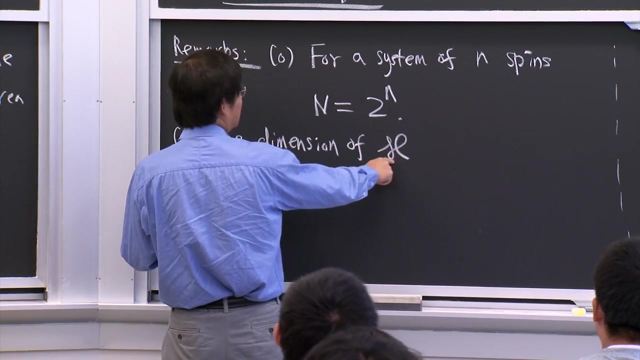 So when I say spins, I always mean spin half. Then the dimension of the helper space is 2 to the power of n, OK, Just to remind you, But the dimension of H, the herbose space. so normally I'd 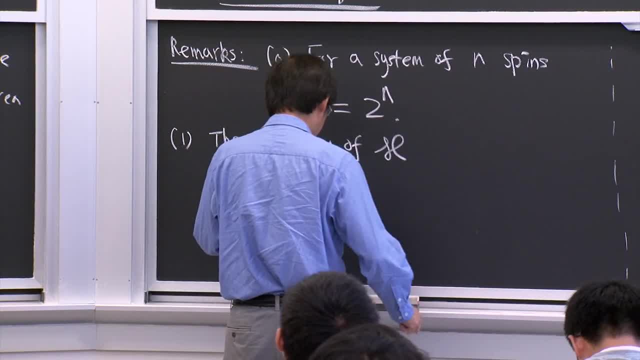 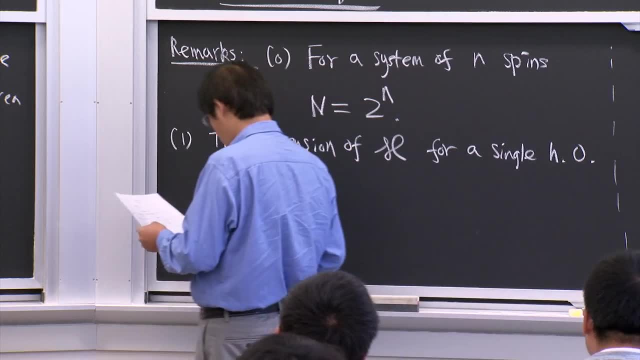 asked: how have these? How have these Thirty n times 1? 03.. Why do I have just 30 n times n? use script H to denote the Hilbert space for a single harmonic oscillator. So the next, so the simplest system is spin. 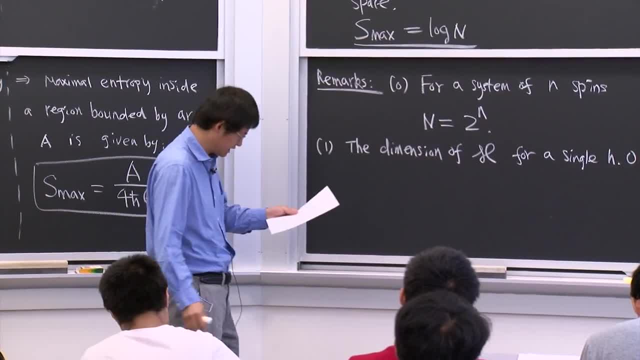 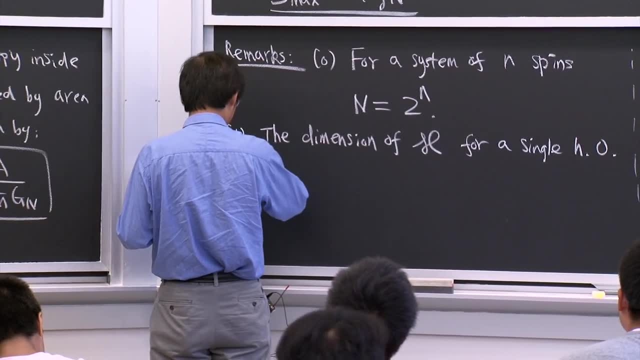 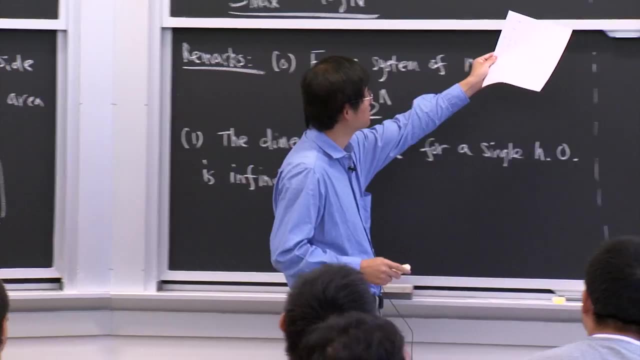 Then the next simplest system is essentially a harmonic oscillator, And even for a single harmonic oscillator, and the dimension of H is infinite. And then you ask what I'm talking about here, Because here I say the Hilbert space should be smaller than that. 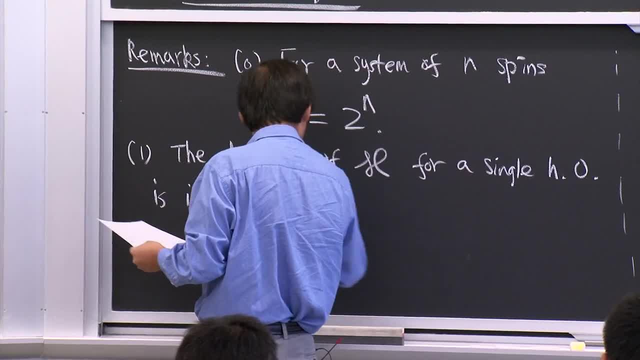 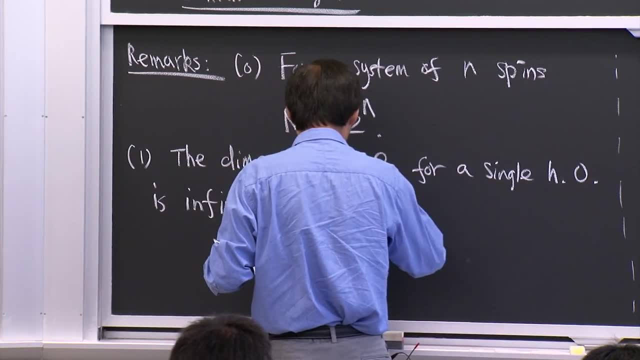 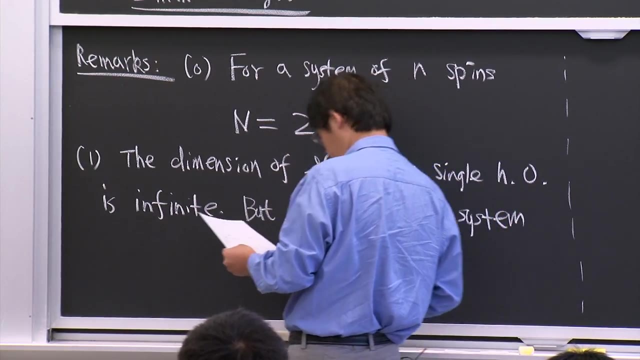 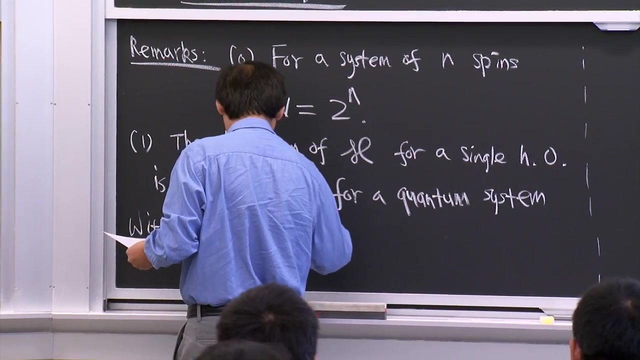 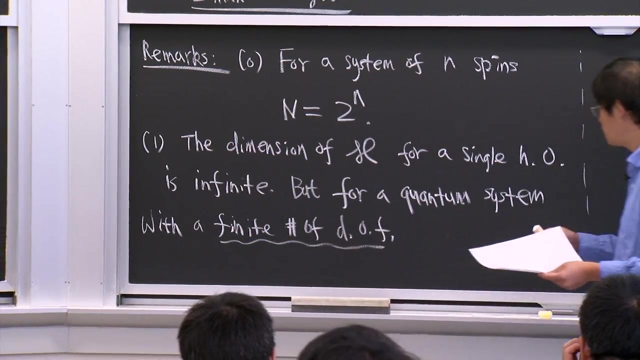 But OK. so even for a single harmonic oscillator the Hilbert space is infinite. But for a quantum mechanical system, for a quantum system with a finite number of degrees of freedom, by finite number of degrees of freedom, for example, you can interpret as, for example: 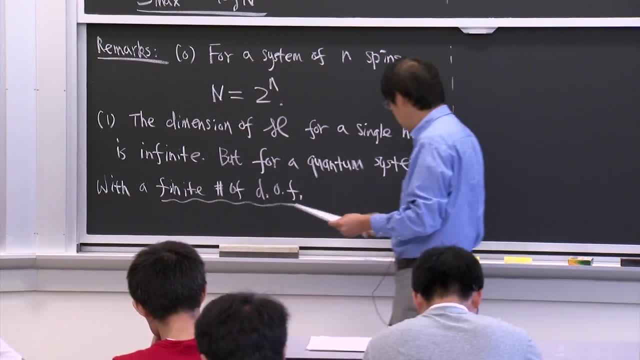 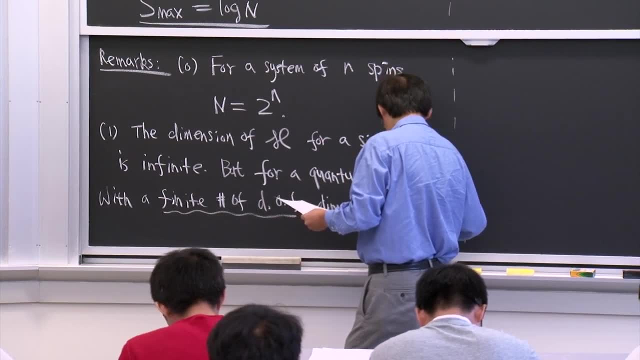 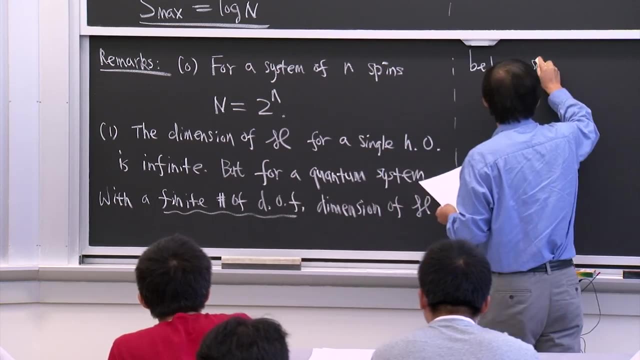 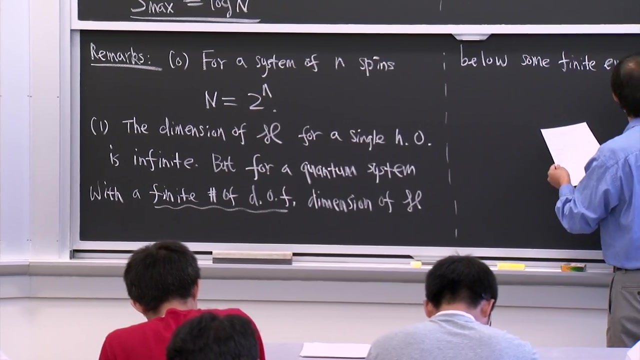 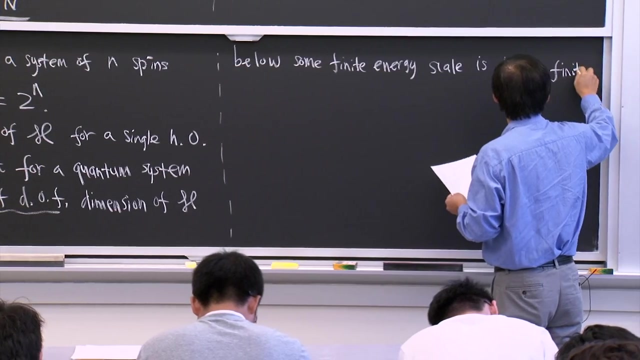 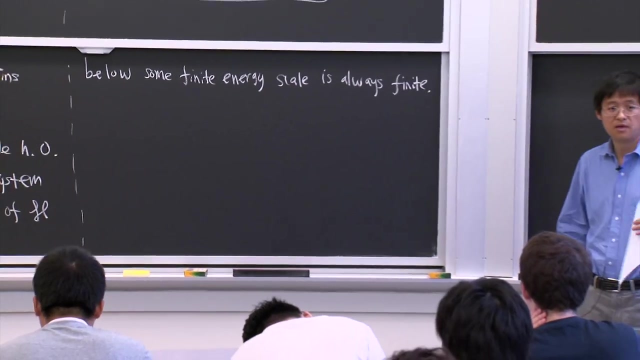 finite number of harmonic oscillators? OK, The dimension of the Hilbert space below, OK, Some finite energy scale. energy is always finite. OK, It's always finite, And so that's why I used the word effective there, And because normally we all consider the finite energy. 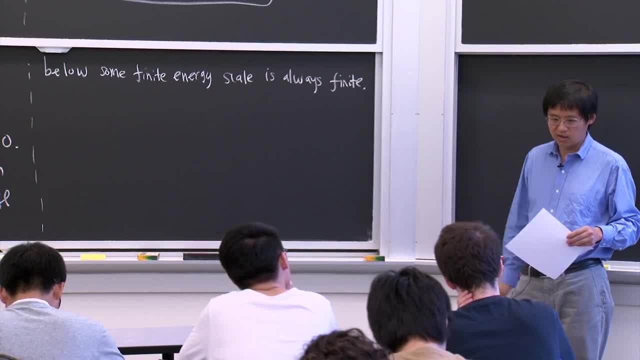 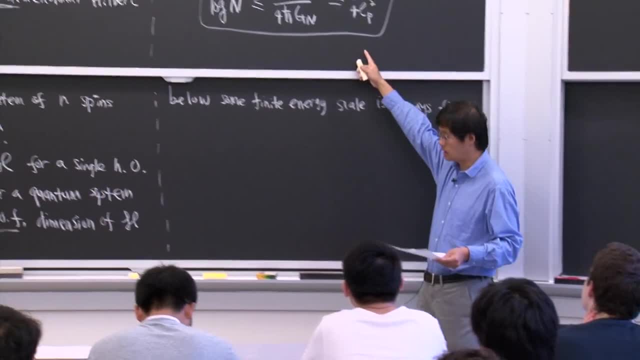 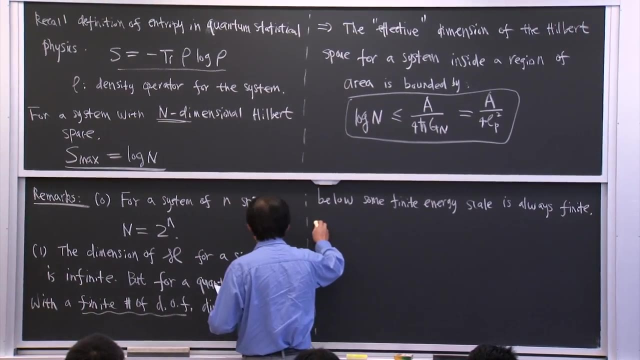 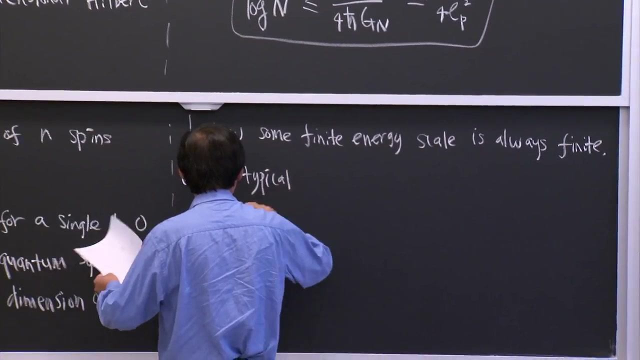 Yeah, Because the system will have finite energy And then you have, in fact you have, a finite dimension of Hilbert space. OK, So this equation is not that crazy. So actually, in typical physical systems, even for harmonic oscillators, both for spin, 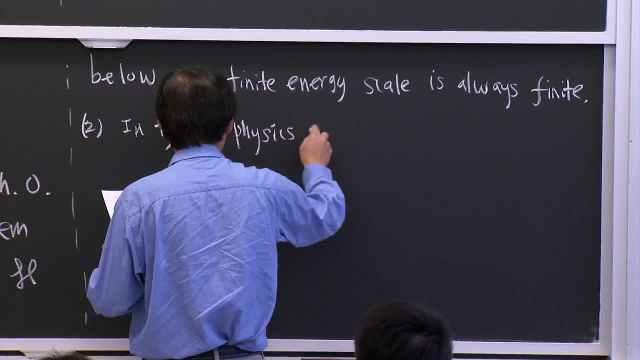 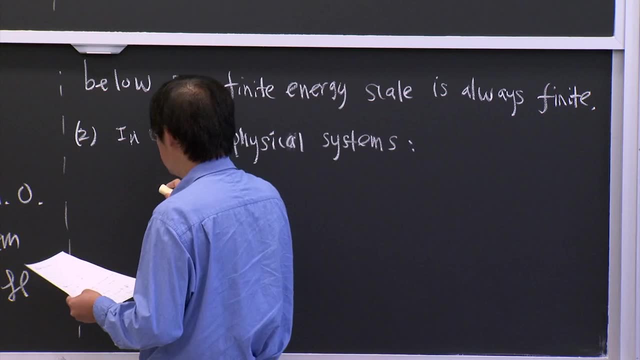 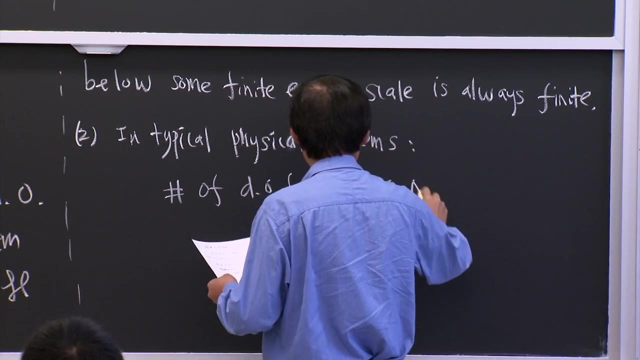 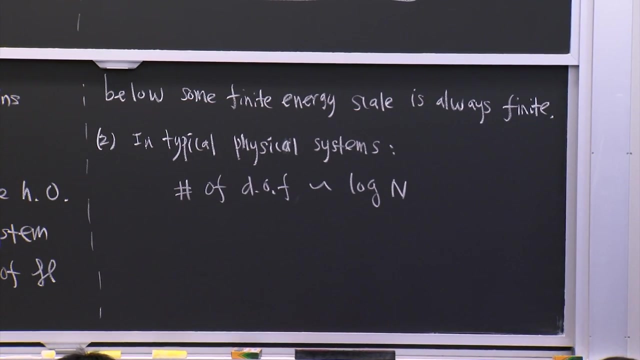 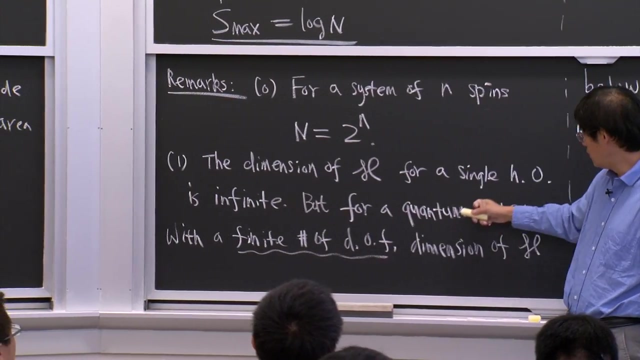 or harmonic oscillators. OK, Essentially, number of degrees of freedom is, of all the log n, Yeah, n is the effective dimension of your Hilbert space. OK, Yeah, this is obvious from the spin. OK, This is also obvious if you have a harmonic oscillator. 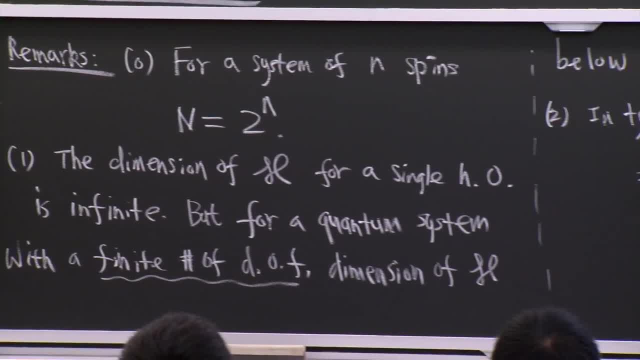 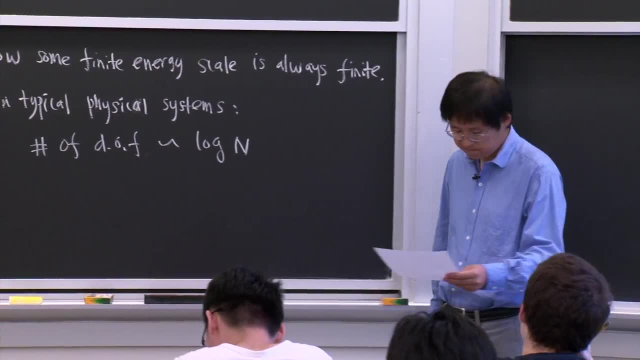 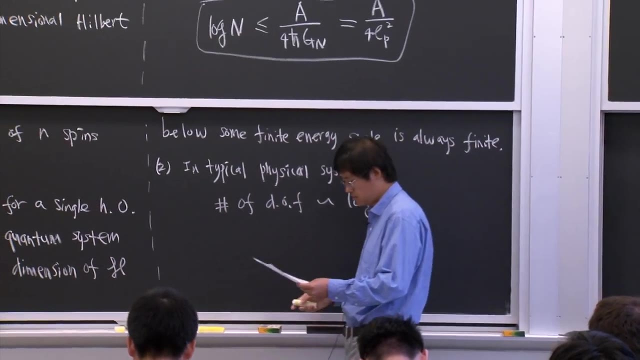 So we each harmonic oscillator. Harmonic oscillator is finitely excited, And then again roughly. the log n is the number of harmonic oscillators. OK, So because of this we can also write this equation as the number of degrees of freedom. 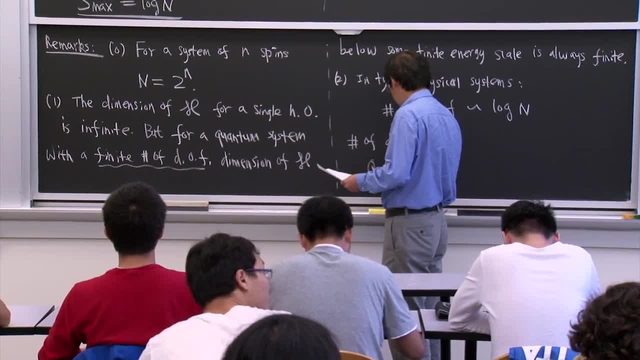 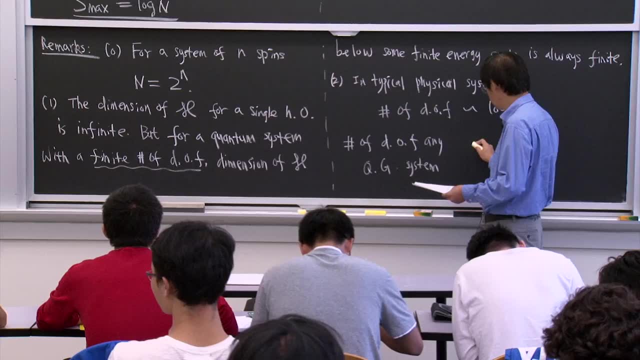 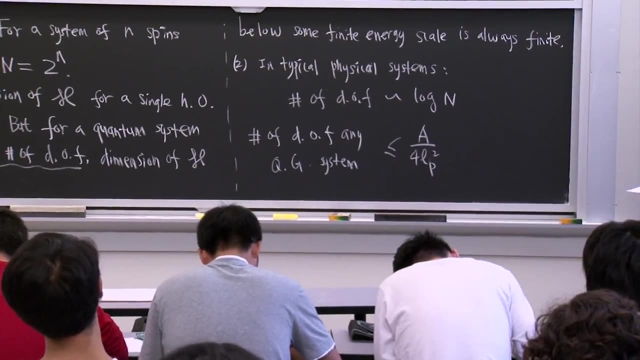 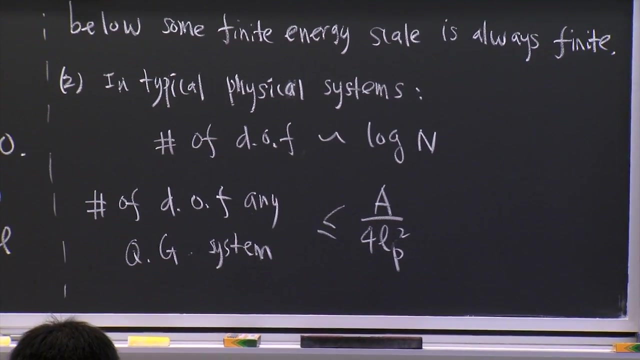 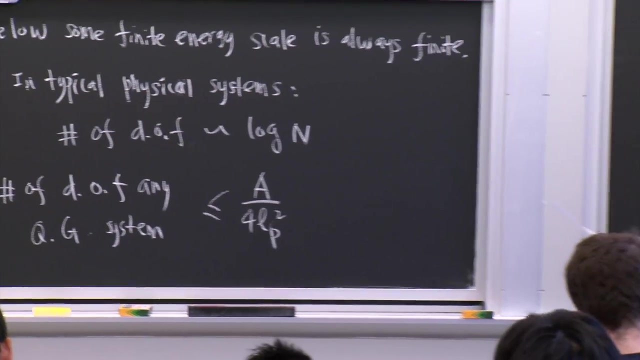 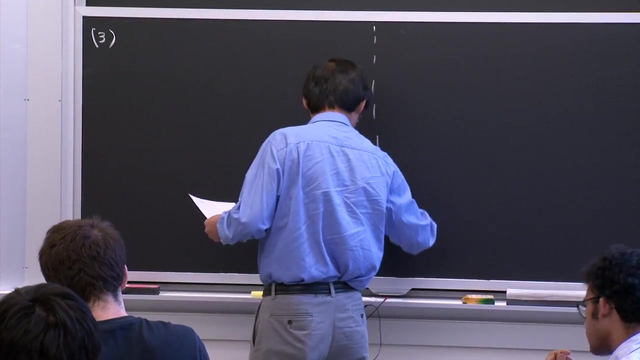 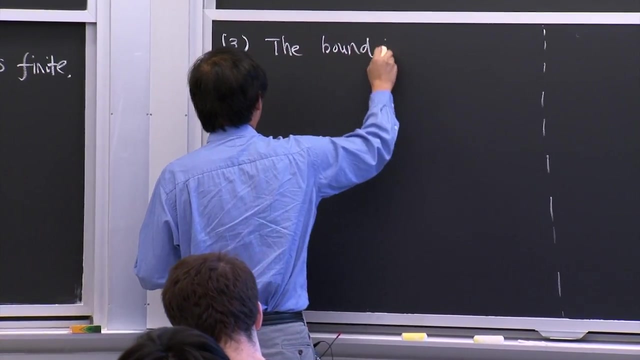 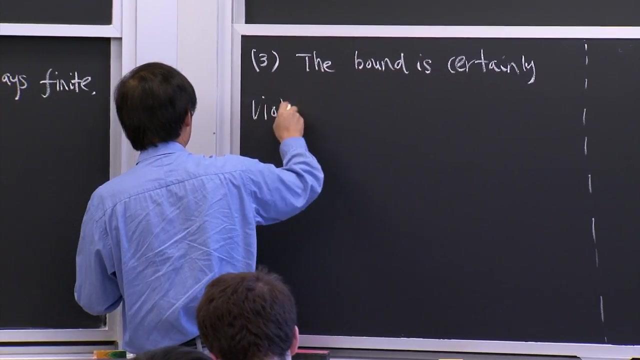 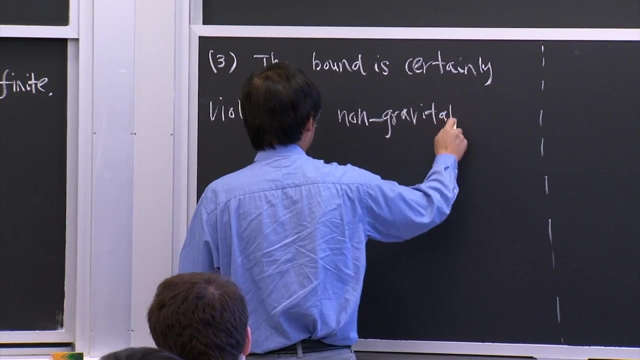 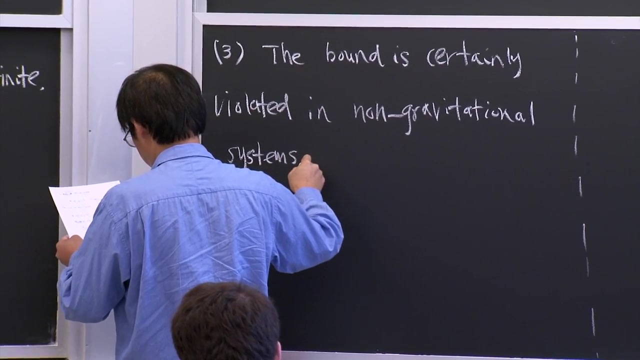 over any quantum gravity system. OK, Inside the region A can be. should be smaller than should be bounded by the area of that region. OK, So this bound is certainly violated in non-gravitational systems. OK, Because in non-gravitational systems 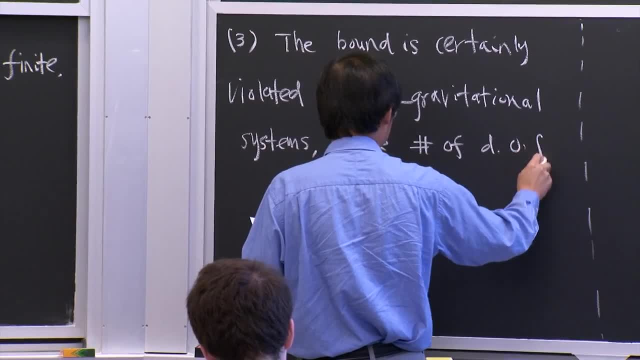 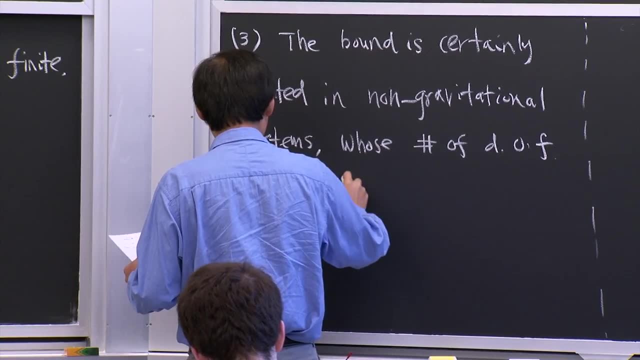 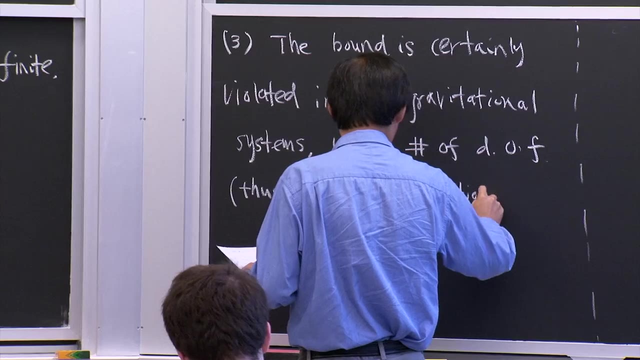 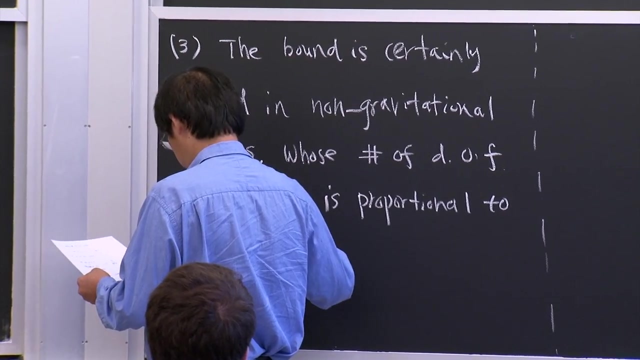 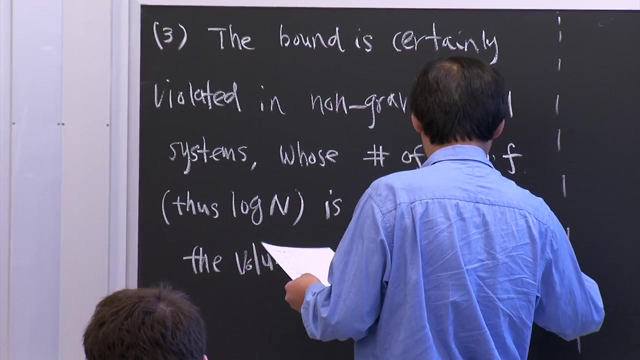 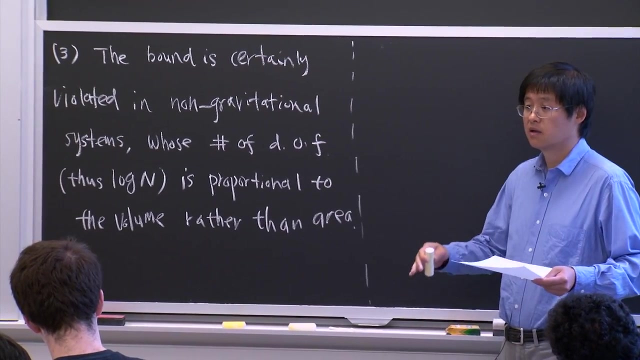 whose number of degrees of freedom and the sus, the log n, the log of your dimension, of your Hilbert space, is proportional to the volume rather than area. OK, So when the region is big enough, then you are guaranteed to violate this bound. 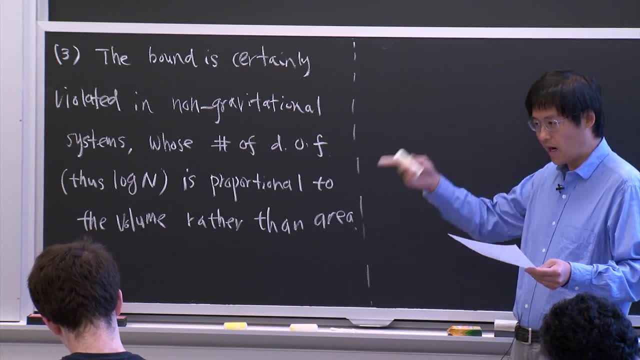 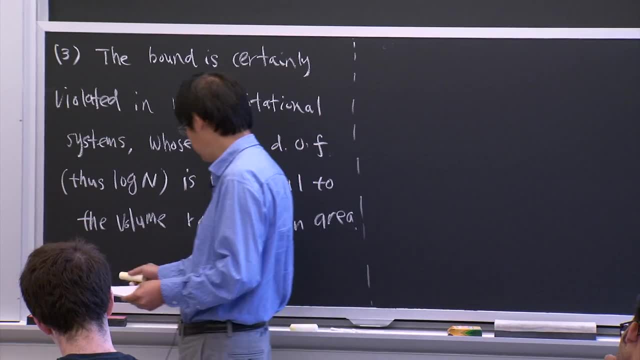 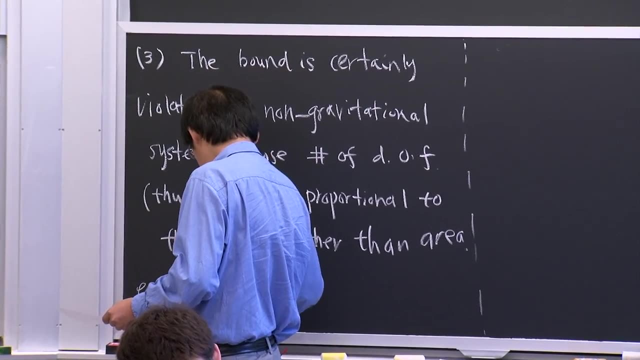 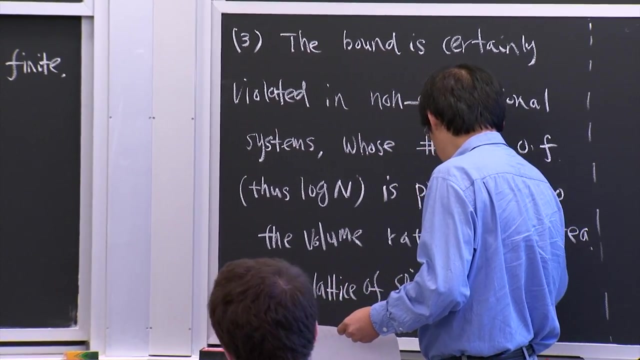 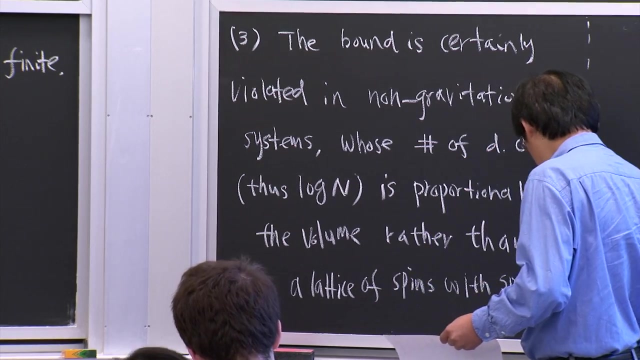 Because of course, the volume grows faster than the area if you have a sufficiently larger region. So, for example, consider just a lattice of spins, Say three-dimensional lattice of spins, of lattice spacing A Say of lattice spacing A. OK. 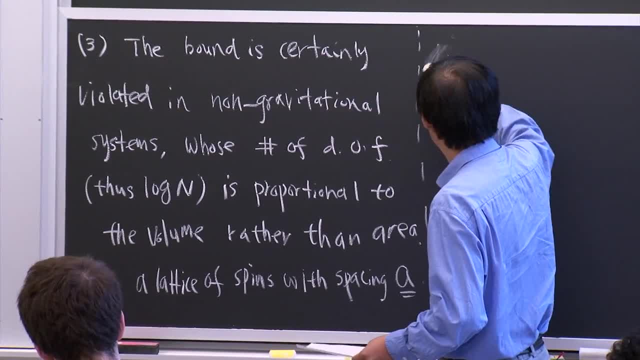 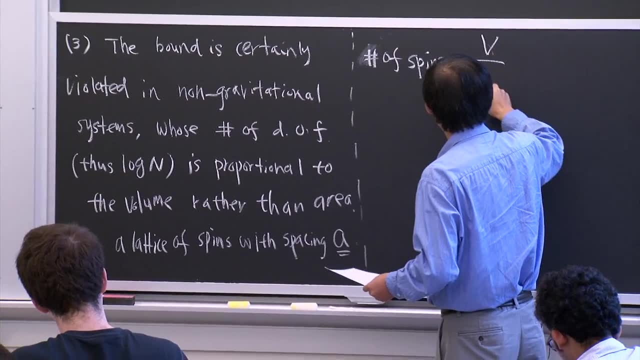 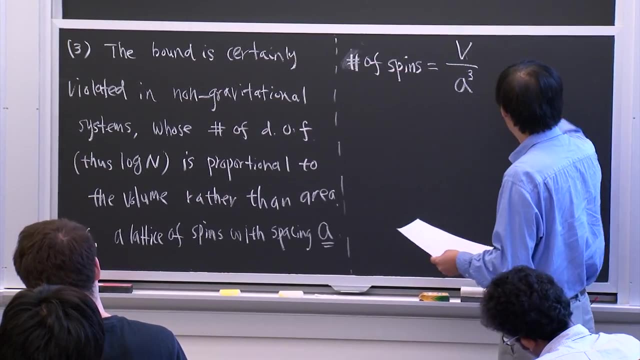 Then the total number of spins, then the total number of spins, then it's given by volume divided by a squared. OK, OK, OK, OK, OK, Cube, OK, So this is essentially the number of degrees of freedom, And then this is given by A, the area. 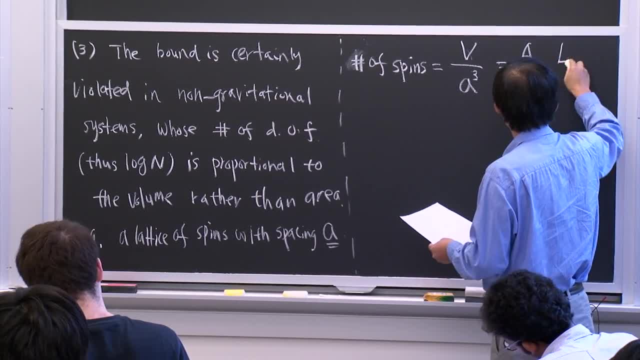 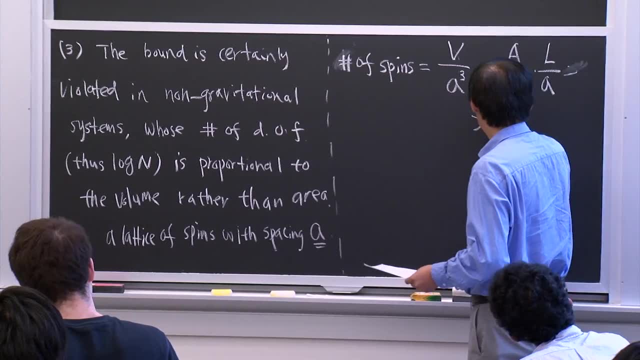 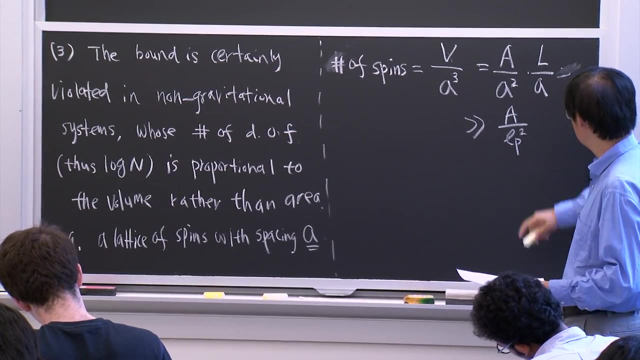 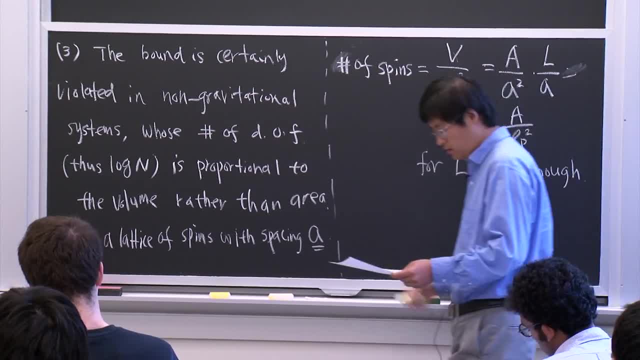 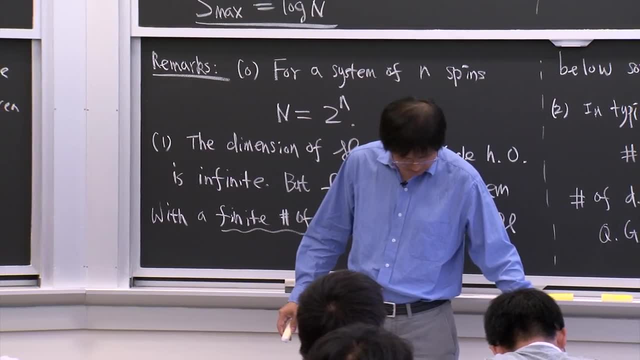 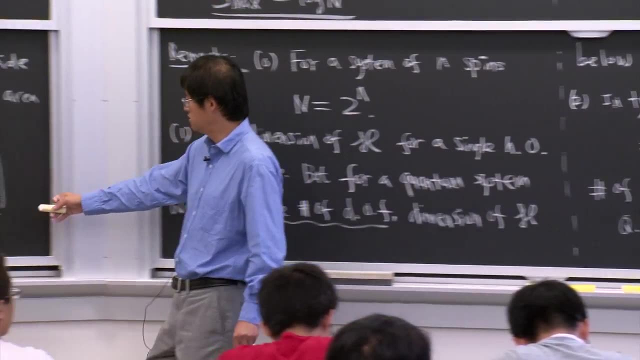 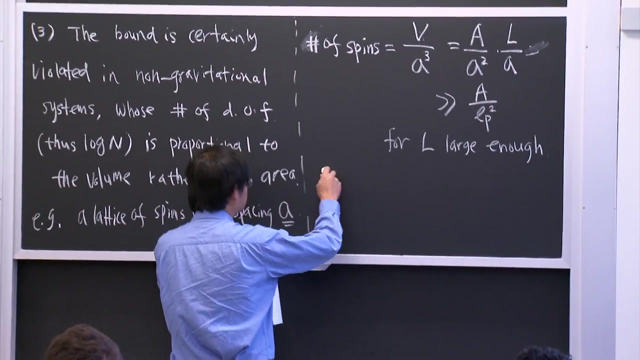 They are large enough. So if you have a long gravitational system, then this bound can be easily violated. In particular, this equation can also be violated because of the dimension of the Hilbert space. Then in this case it would be 2 to the power a cubed. 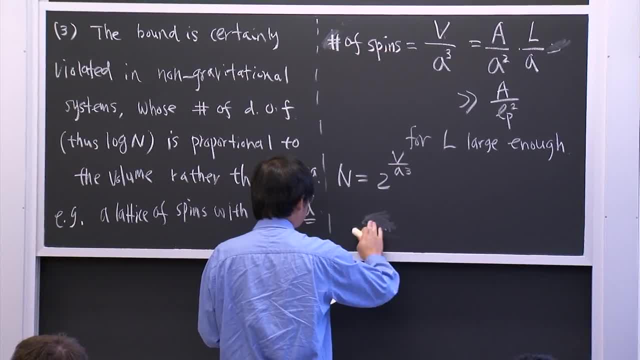 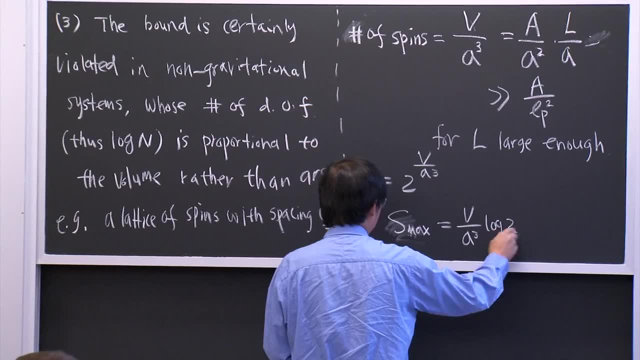 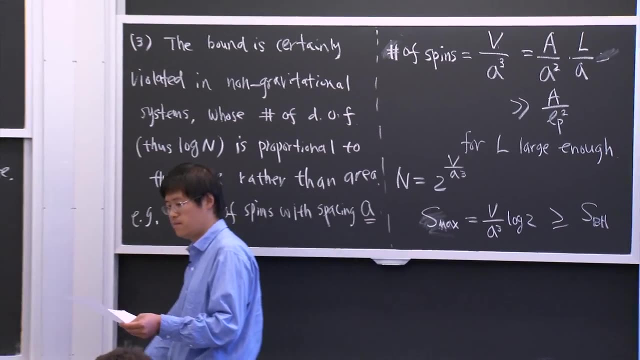 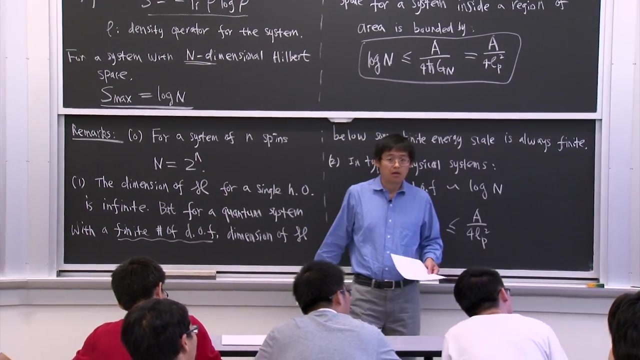 And similarly. so the maximum entropy would be, say, v divided by a cubed, log 2.. Log 2 because it's a spin half system, So this can be larger than the entropy of a black hole. So it's key that we can see the gravitational systems. 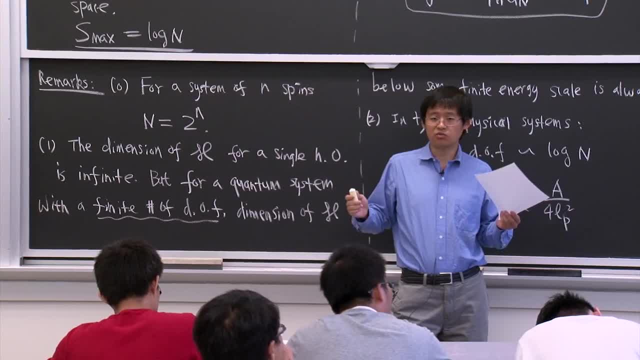 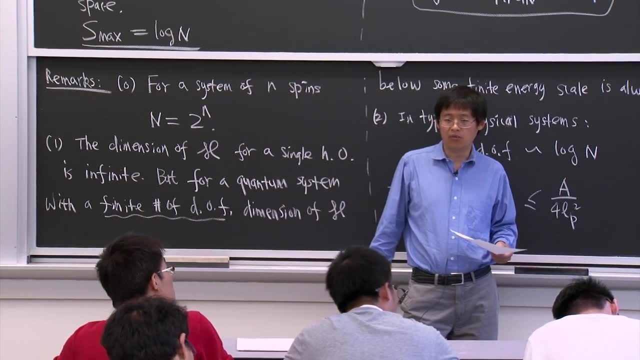 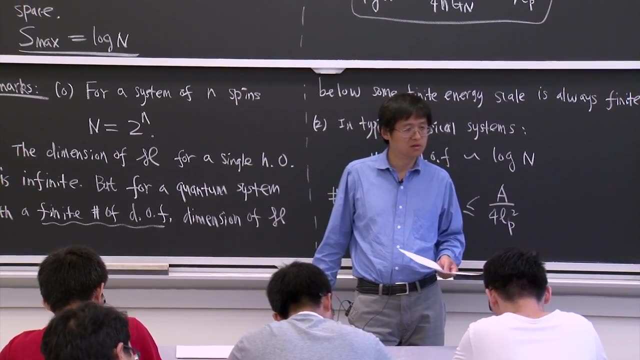 OK, Only in gravitational systems. you have this remarkable feature that things will collapse. OK, Things will collapse, will collapse, And then you will have this upper limit provided by the black hole. Yes, So in the real world, every system is a gravitational system. 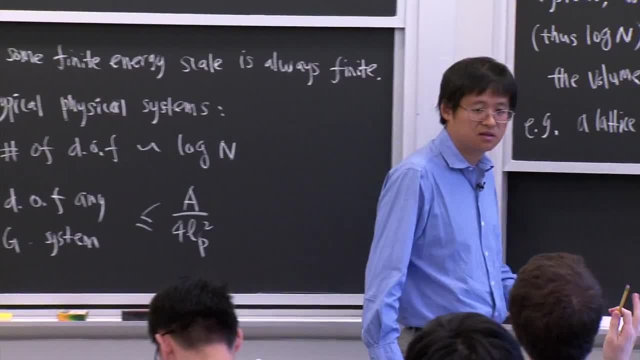 HONG LIU- Yeah, So, But this is just, in some sense, this is not actually correct in the real world. HONG LIU- Yeah, but you need this L to be not enough. I see, HONG LIU- Yeah. 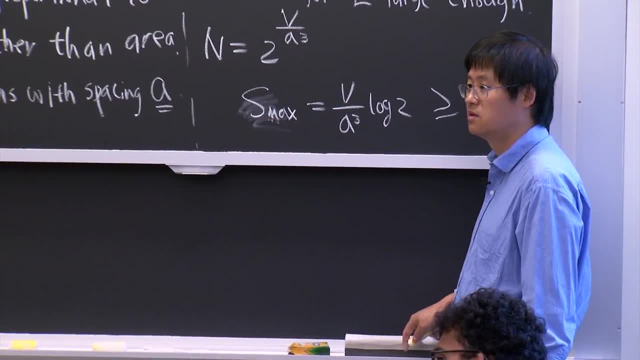 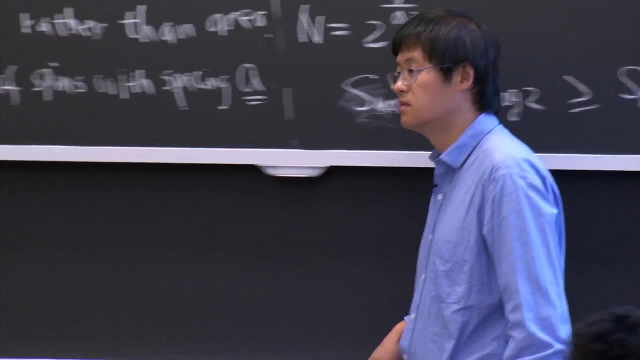 Yes, So right in the real world, this bound has to be obeyed by a system. So does that put some bounds on QFT UV completions? So in the real world, this bound has to be obeyed by everything. 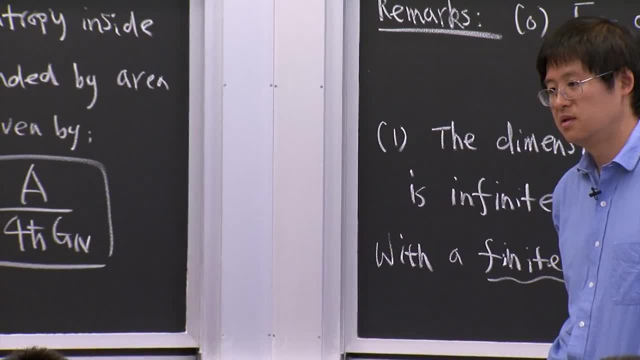 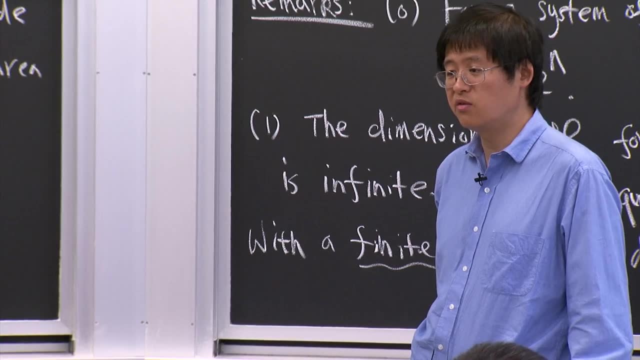 HONG LIU- Yeah, So does that put some kind of restrictions on QFT UV completions, Because we usually say it's you know infinite density of degrees of freedom? HONG LIU- No, because the UV completion of a QFT. 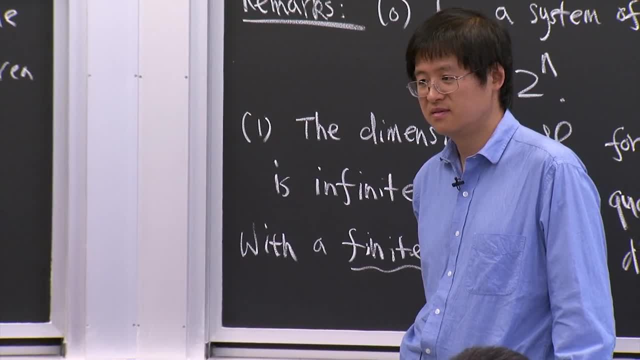 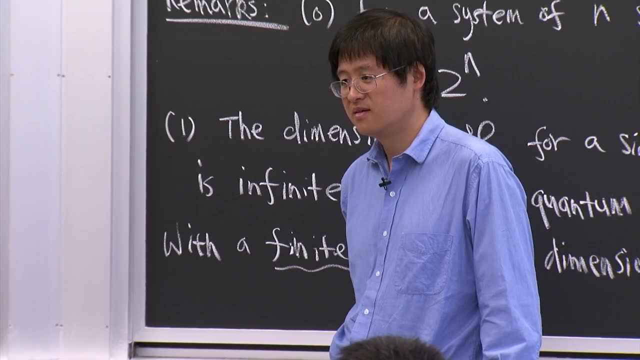 is provided by gravity For any QFT. I just mean, like a scalar field, HONG LIU-, Then that's not a theory of gravity, Right. but if you have a scalar field in a spacetime which has GR in it, what is otherwise flat? 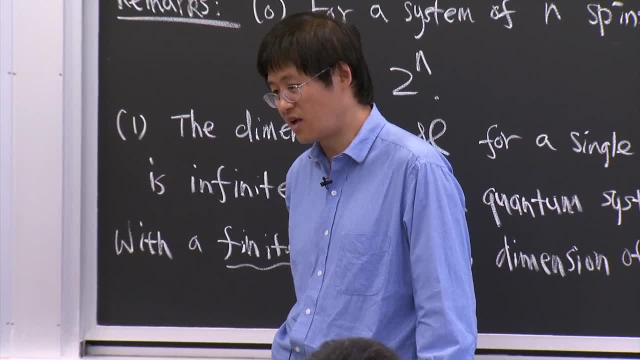 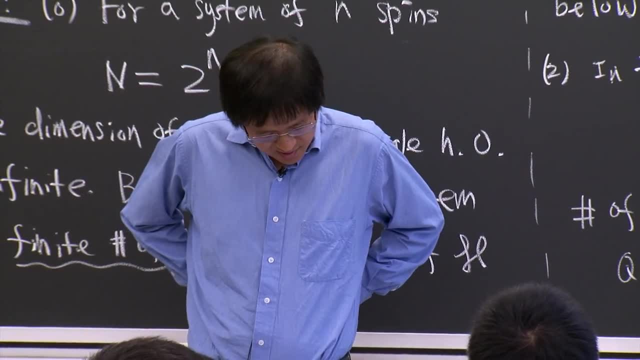 HONG LIU- Yeah, then the GR, then the gravity will provide the UV completion of that scalar field. OK, OK, HONG LIU- Yeah, Yeah, Right, I was going to say something else, but I forgot. 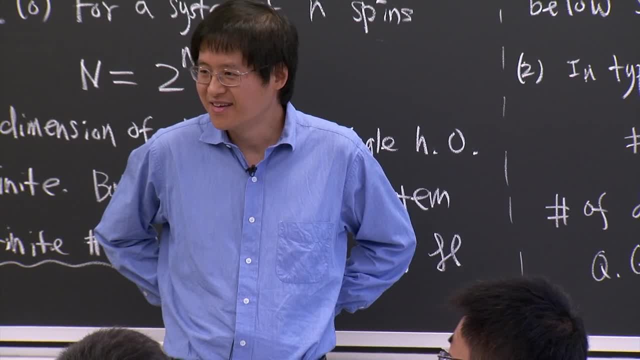 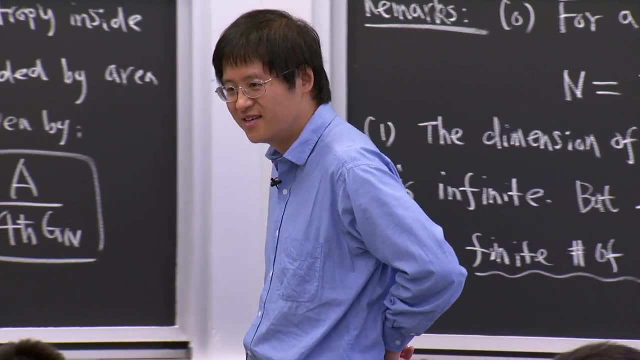 What about the ones that are UV complete? HONG LIU- Hm. What about the theories that are UV complete, at least formally? HONG LIU- Sorry, say it again. The QFTs that are UV complete, HONG LIU- Yeah, they are still limited by gravity. 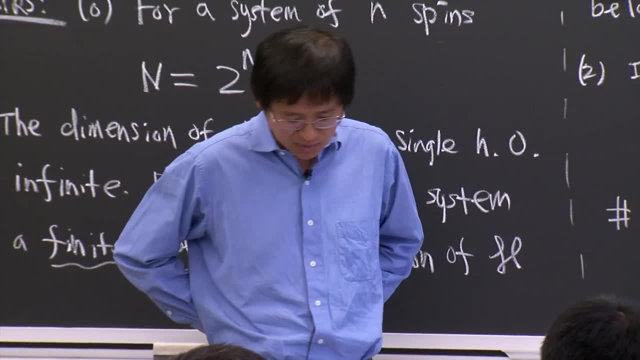 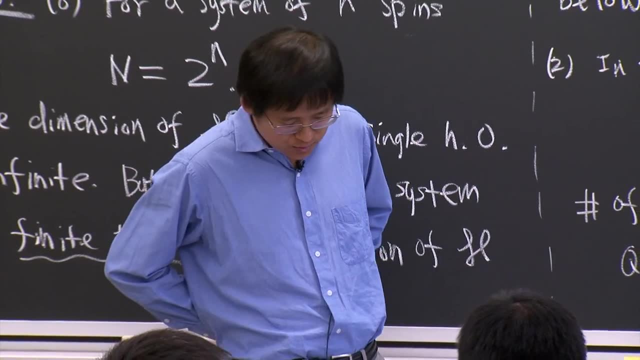 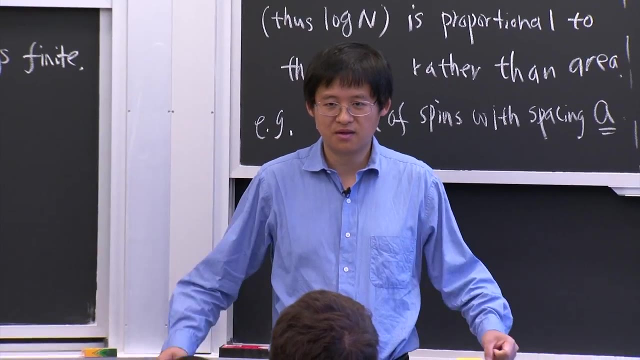 Yeah, the gravity will still provide something, Because QFT have infinite number degrees of freedom. OK, HONG LIU- Yeah, so example of this: for example, you can think a classroom, say, full of photons, and then you can calculate entropy. 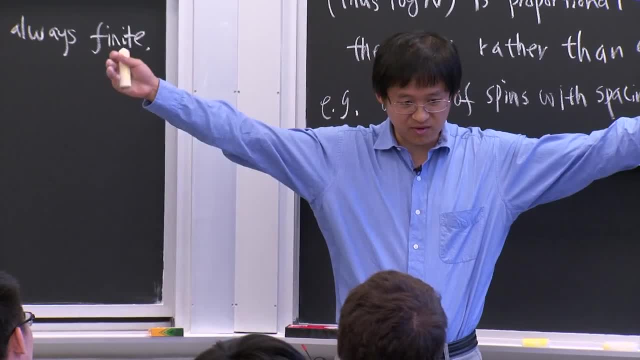 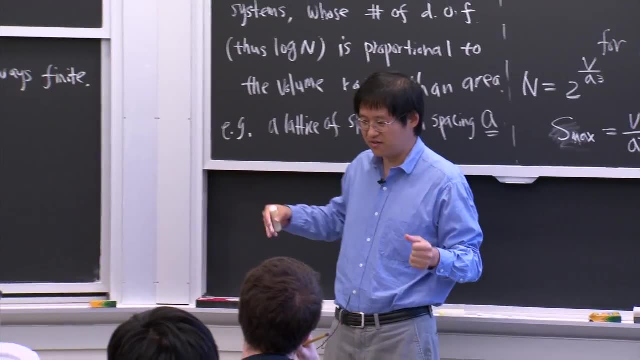 Again, that entropy will proportion to the volume. So if you make the classroom big enough then that will violate this bound. But it's a simple exercise for you to do yourself that if you put a classroom at the finite temperature photon, then when the room is big enough, 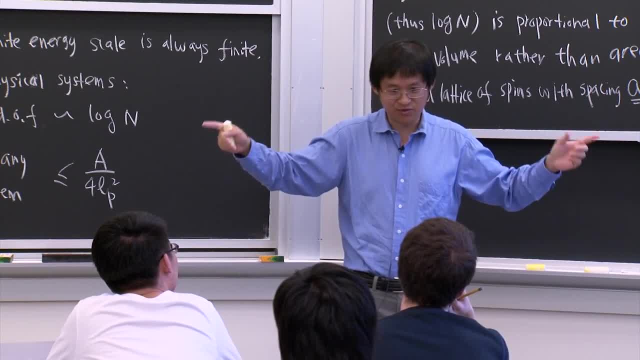 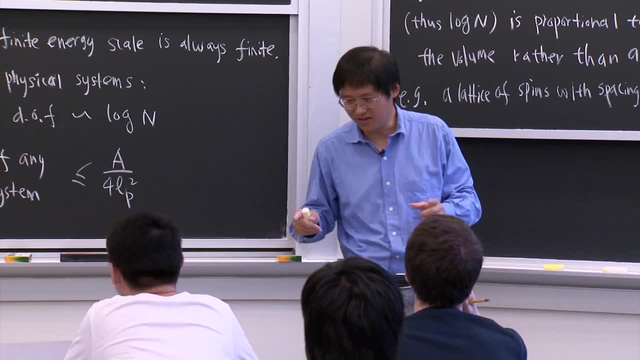 there's always a radius that will collapse, form a black hole, before this bound is violated. OK, I think maybe I have this problem in the piece. I forgot whether I have it or not. Yeah, you can do this simple exercise yourself. 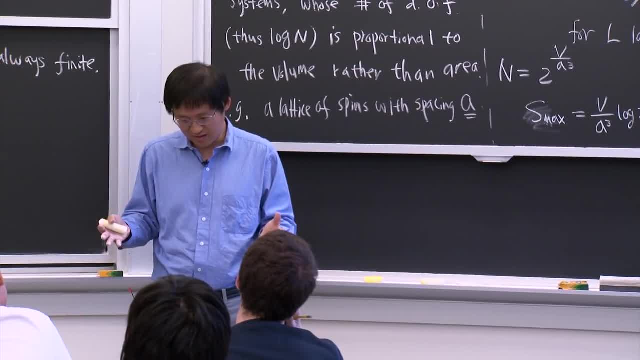 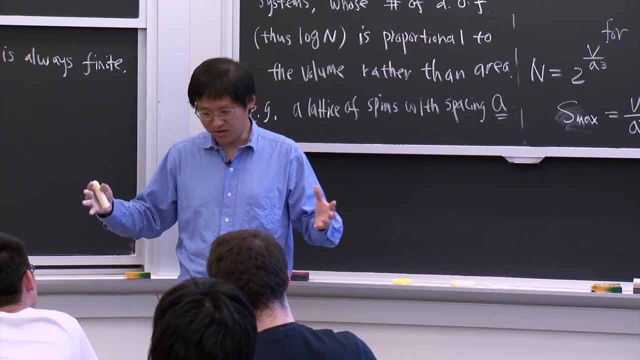 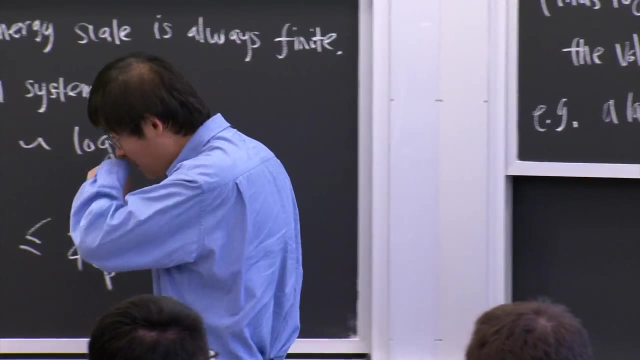 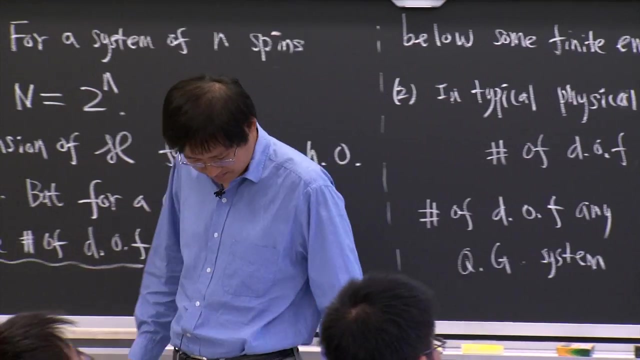 Yeah, just imagine you have a box of photons at any non-zero temperature, T, and then, when you put the box big enough, then at a certain point this whole box of photons will collapse, form a black hole, And that's to make this bound to be satisfied. 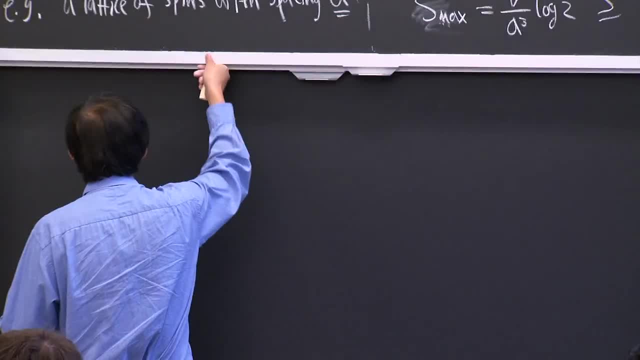 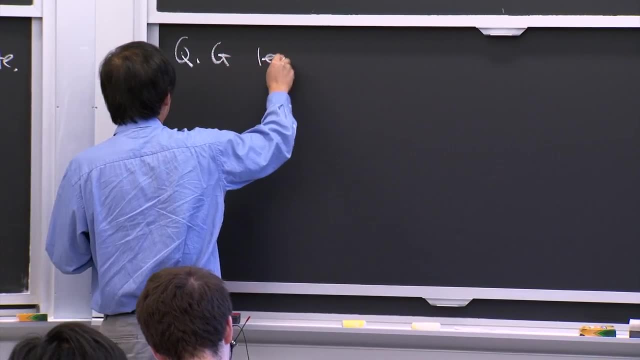 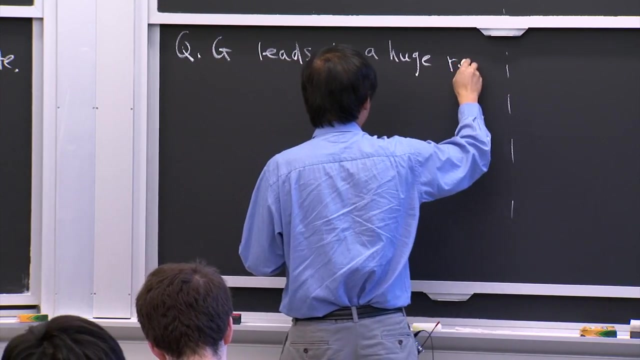 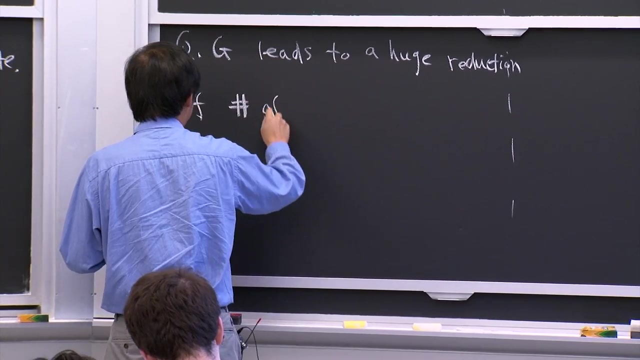 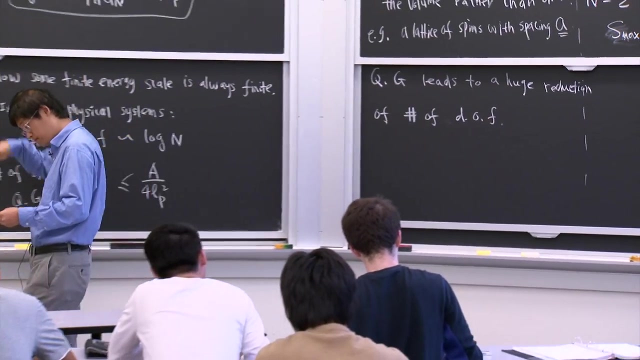 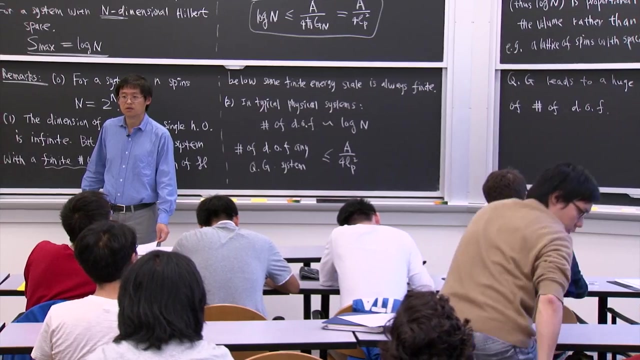 So what this means is that if you have gravity, the quantum gravity leads to a huge reduction. OK, It leads to reduction of lambda degrees. freedom- OK, It's really bounded by your area. Now, your previous answer was that you have a conformal field theory. 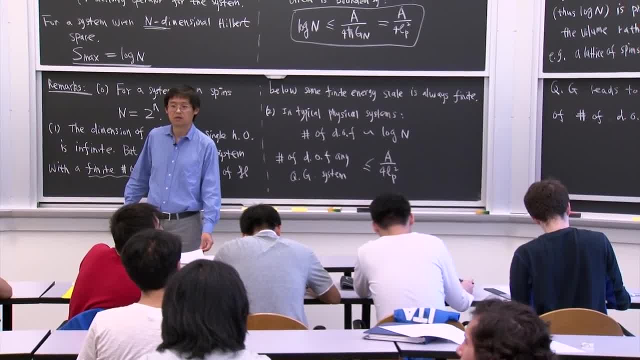 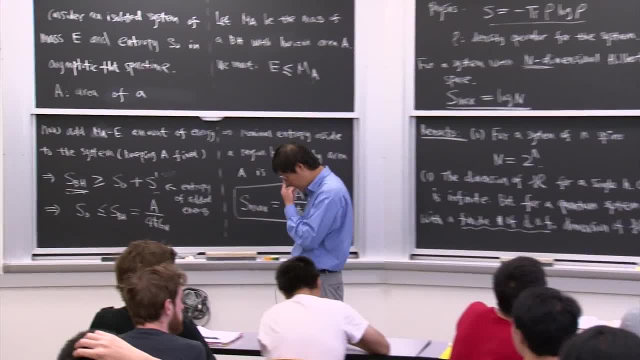 And so this bound also applies to conformal field theory, But we don't need to have any new combination. No, Yeah, as I was answering Pawel before, if you have a conformal field theory just by itself, then there's no bound. 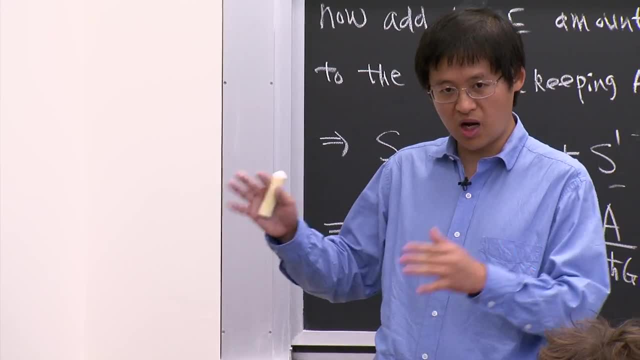 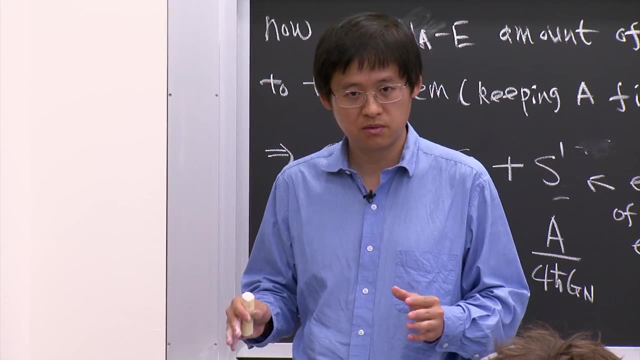 Then there's no bound. But if you couple this conformal field theory to gravity, then at sufficiently high energy, and then the degrees freedom of this conformal field theory must be reduced. No, but if you just have a conformal filter, 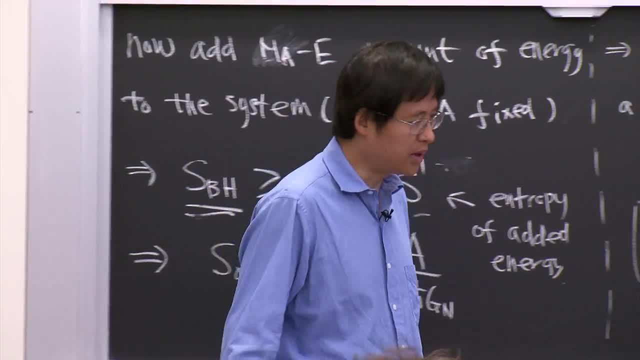 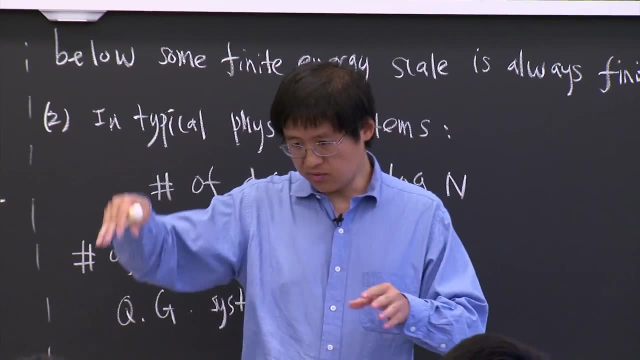 then there's no bound. No bound, Yeah Yeah. But you can ask what happens if we couple conformal field theory to gravity? Not even conformal field theory, just any quantum field theory, Because any quantum field theory have infinite lambda degrees freedom. 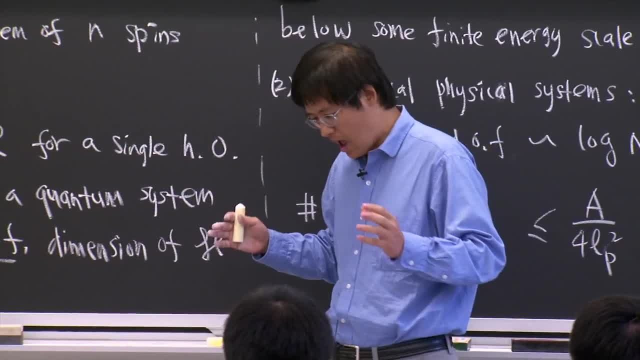 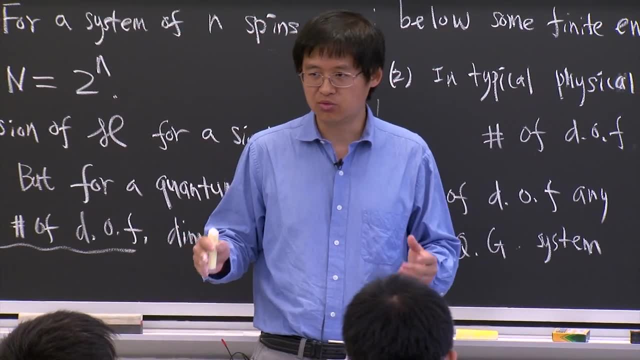 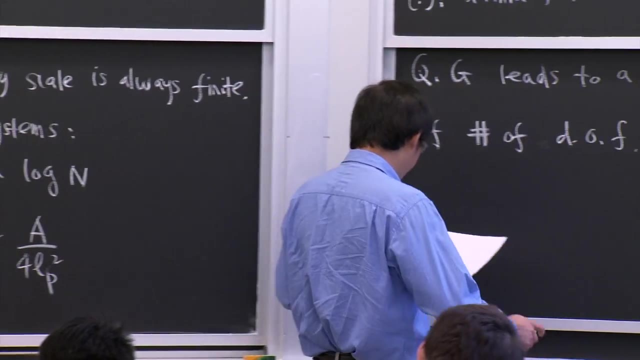 And the lambda degrees. freedom is also proportional to the volume, And if you couple it to gravity, then this reduction must happen. This reduction must happen, OK, So now, if we take a small leap of phase- so we already have taken some leap of phase- 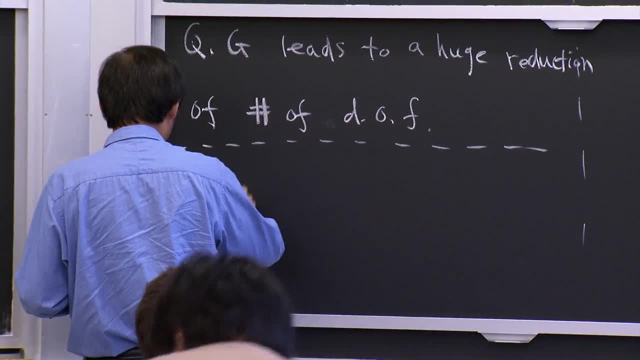 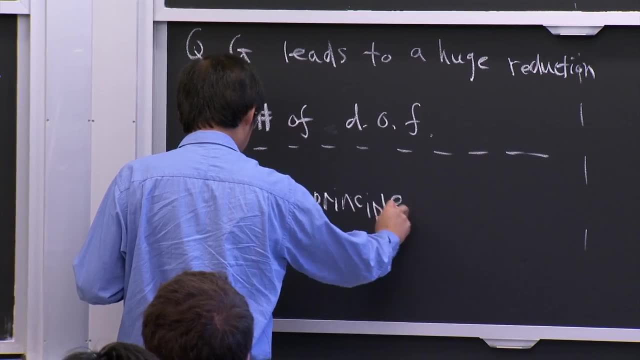 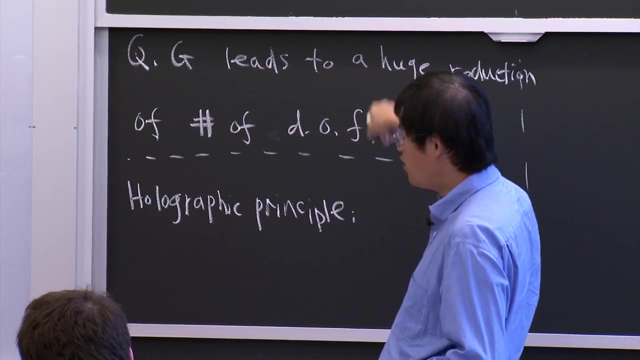 But let's take one more step of leap of phase. Then you can formulate something called a holographic principle. So, given that the lambda degrees freedom inside the region is always bounded by the area, and this area actually has a very nice way, this area in the unit of Planck's 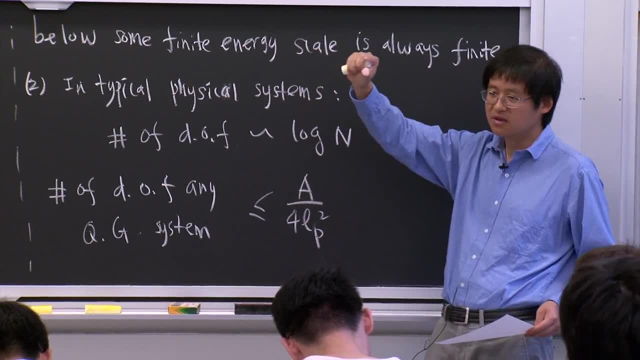 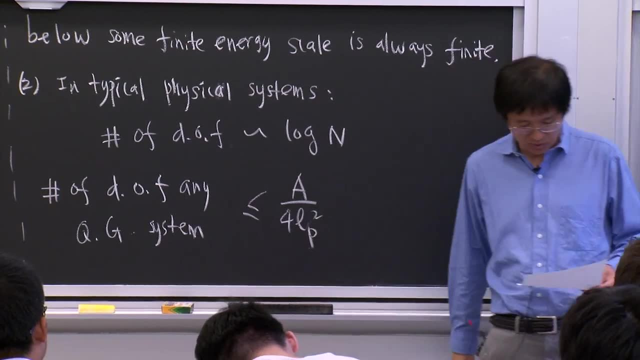 length. it looks like you have a minimal length, minimal area, which is a Planck square length, And just the area divided by that. give you the total lambda degrees freedom. OK, So if you try to extrapolate a little bit further, 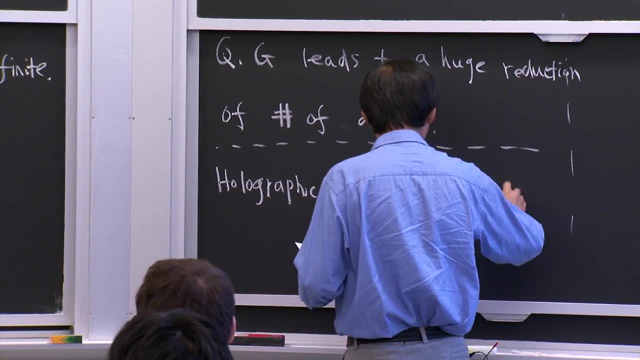 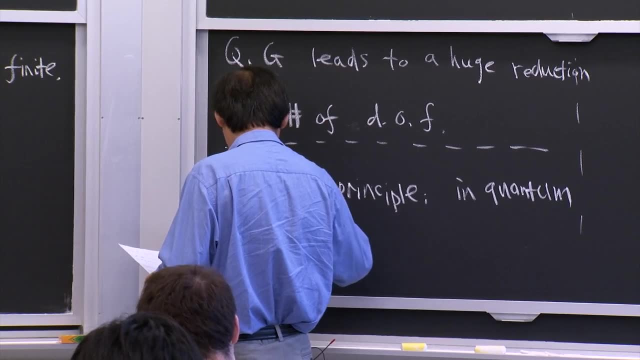 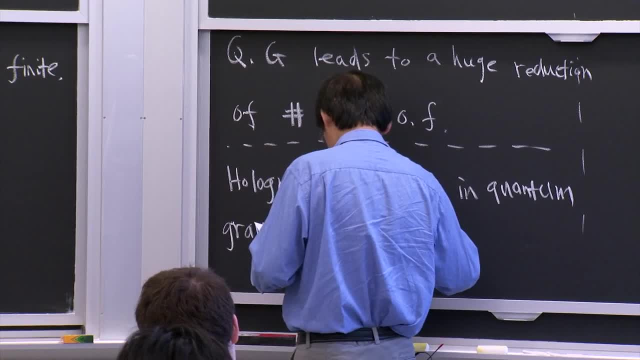 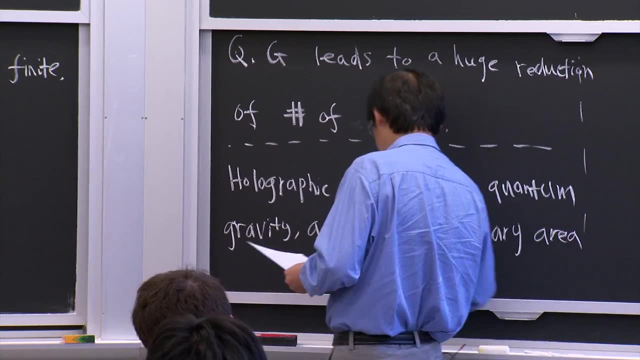 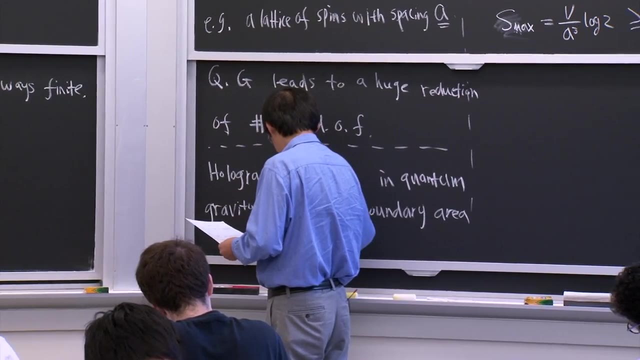 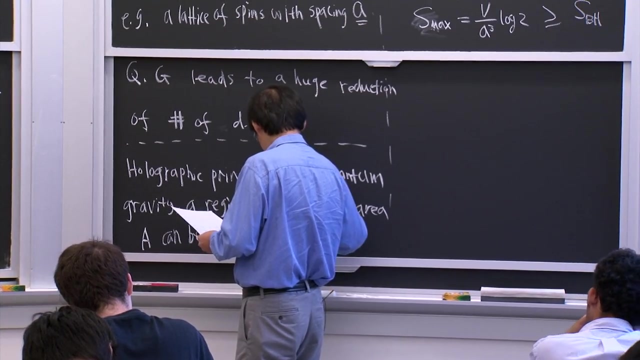 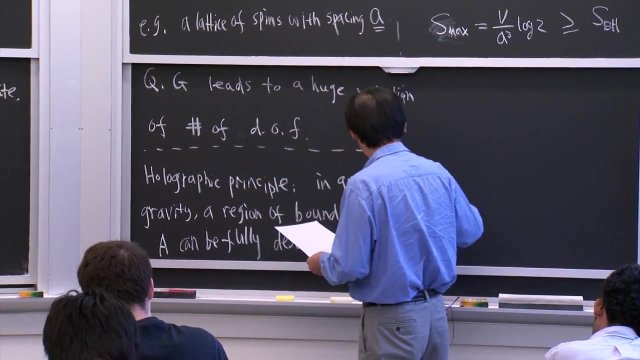 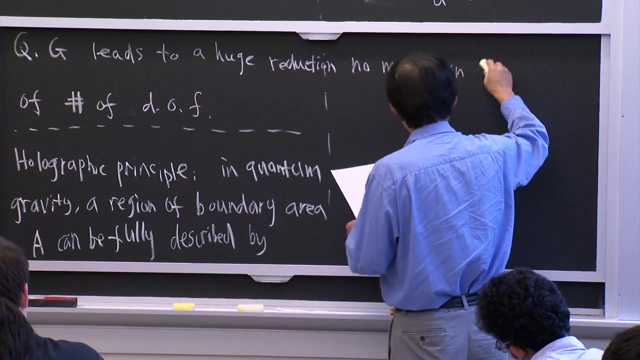 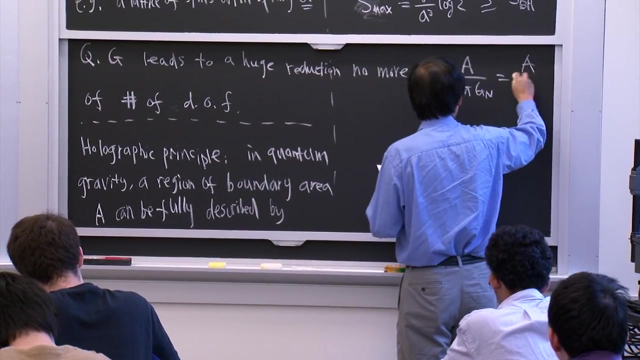 We have a holographic. We have a holographic. We have a holographic Of boundary area. A can be fully described. Can be fully described by No more than So. essentially, it just varies. A, h, bar, h n is a square. 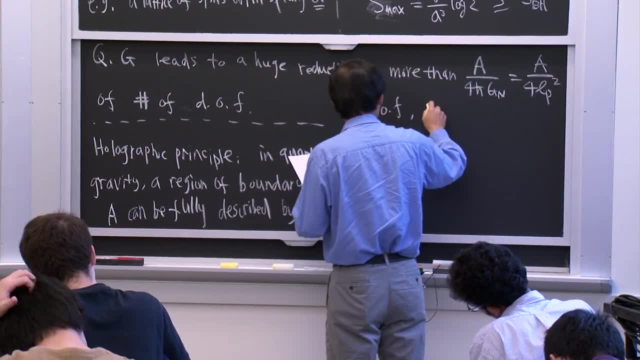 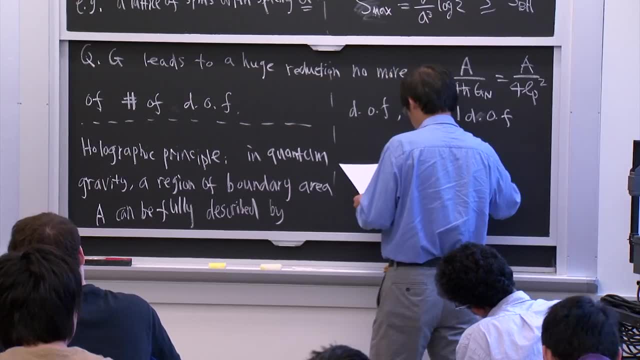 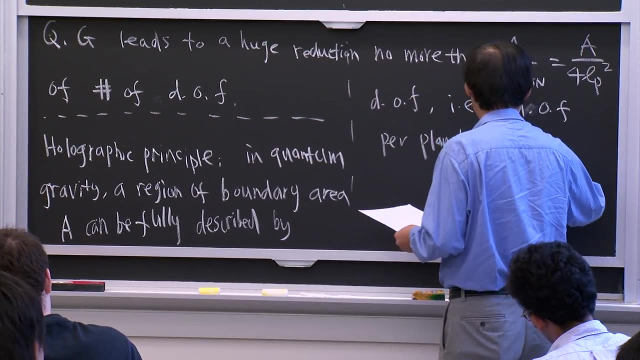 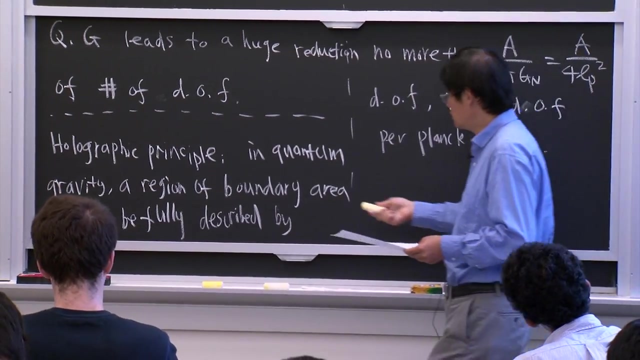 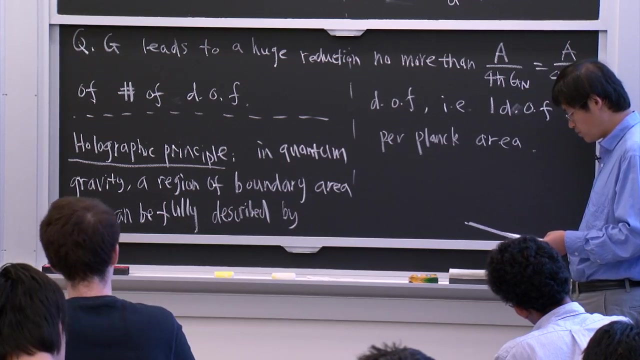 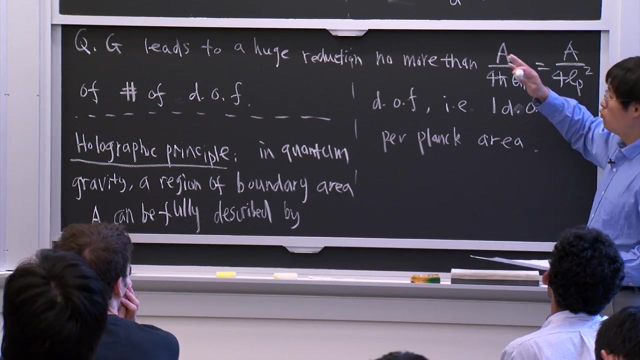 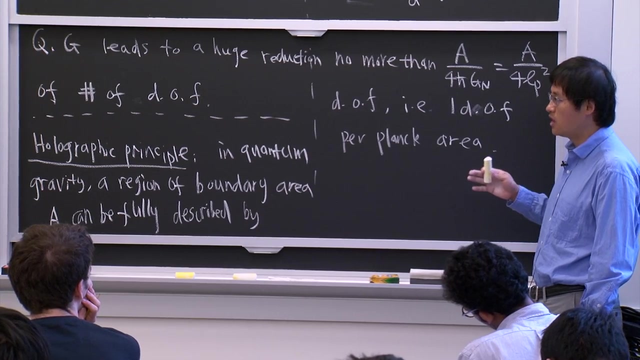 Give you this freedom, In other words, one degree of freedom per Planck area. OK, So this is just a rough formulation of the holographic principle. So what we just said- it just highlights A point we made earlier- is that, even though laively, 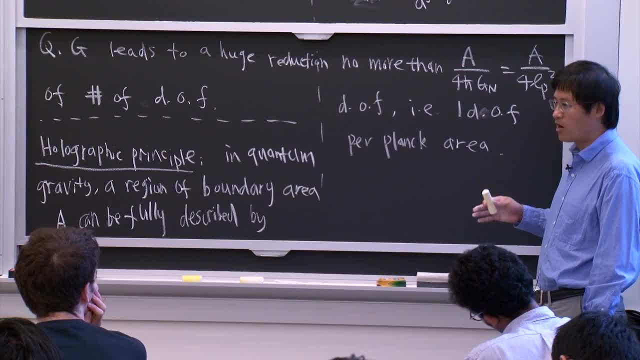 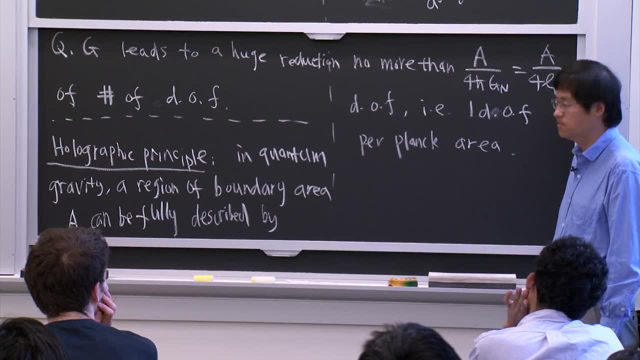 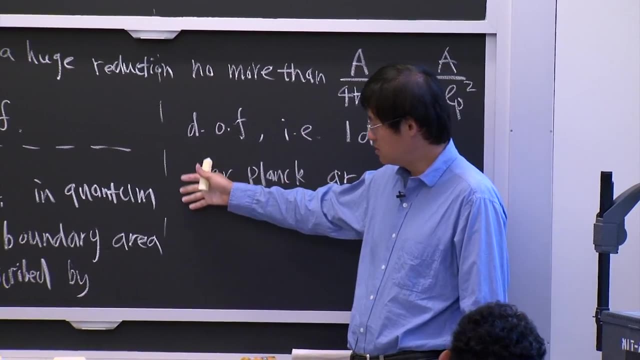 from dimensional analysis that the quantum gravity is only operating, say, at Planck scale, Say at the Planck mass or Planck mass et cetera. But we see that the black hole actually brings the quantum gravity really to microscopic level. 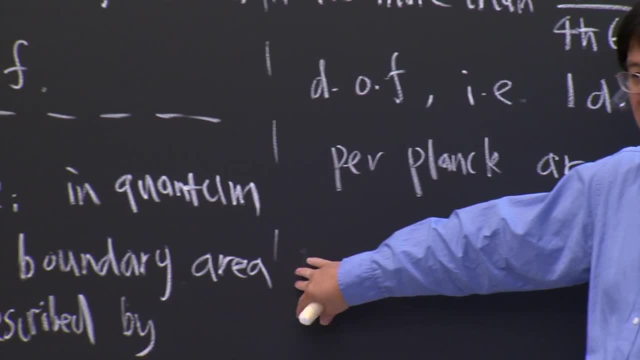 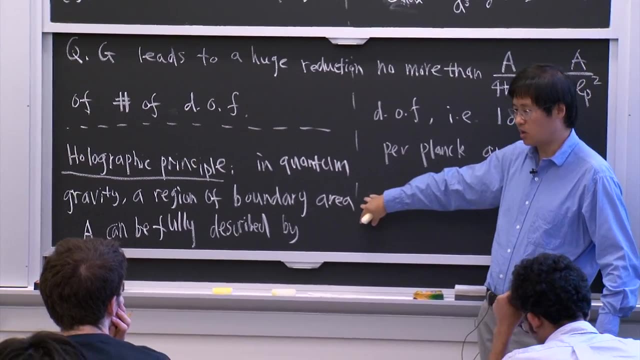 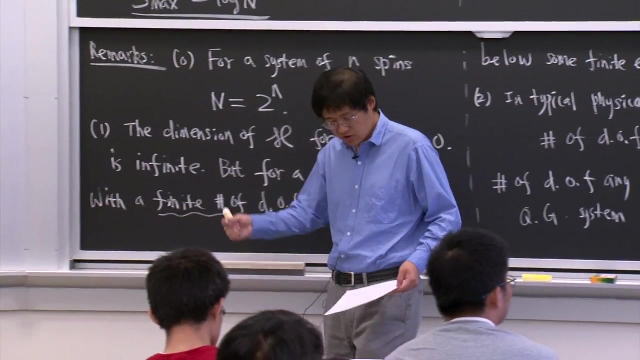 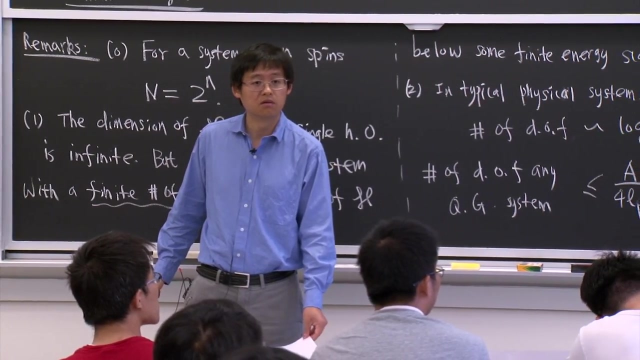 OK, So these are the really macroscopic statements can apply to regions of arbitrary sides, But somehow they are limited by constraint of quantum gravity. OK, So this is a remarkable manifestation of the quantum effect. Any questions on this? Yes, What's so special about dimensional surfaces? 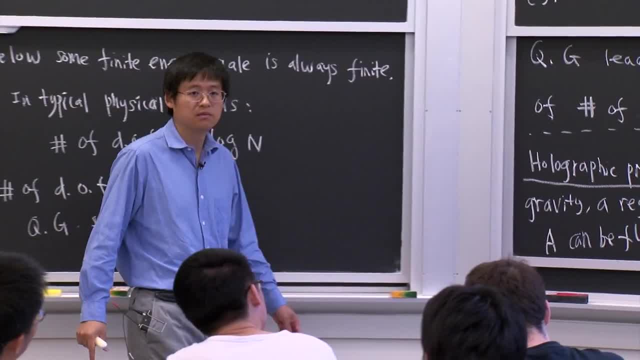 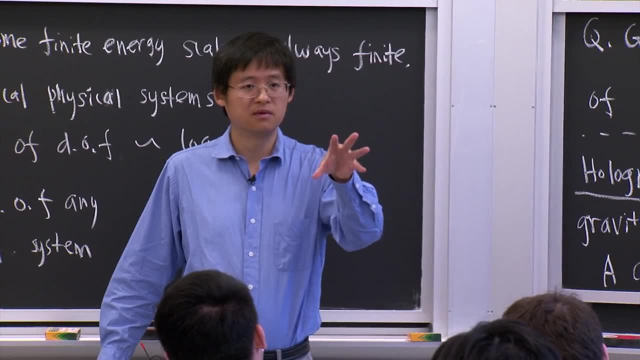 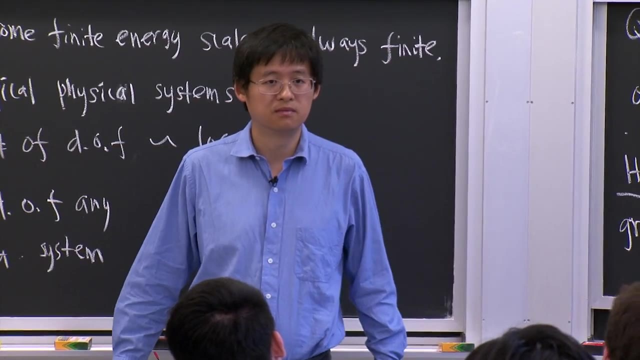 Can it be generalized to? Oh yeah, Yeah, This you can generalize to any dimension. There's always core dimension too. So if you live in five dimension, then become three dimensions. Yeah, it's always core dimension one in the spatial region. 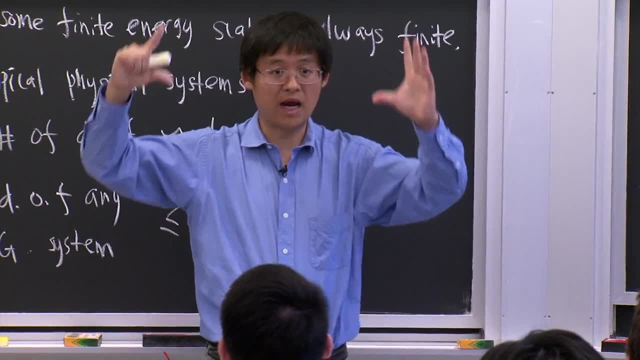 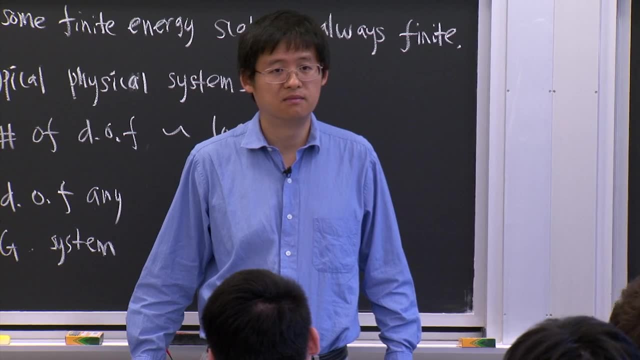 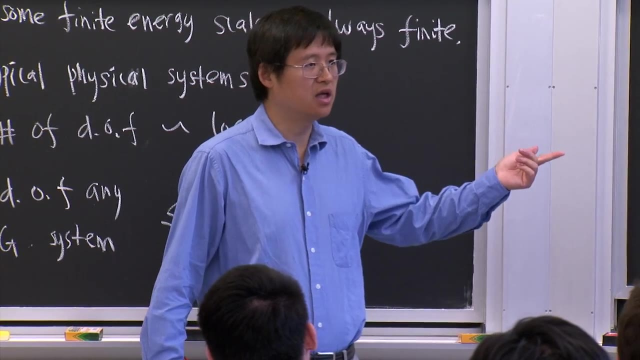 Because the black hole, yeah, black hole, just area of the black hole, is always core dimension, one in terms of spatial. Yeah, Can't you just say, and then I should space some trees here, and then it's Yeah, 10-dimensional space, then naively. 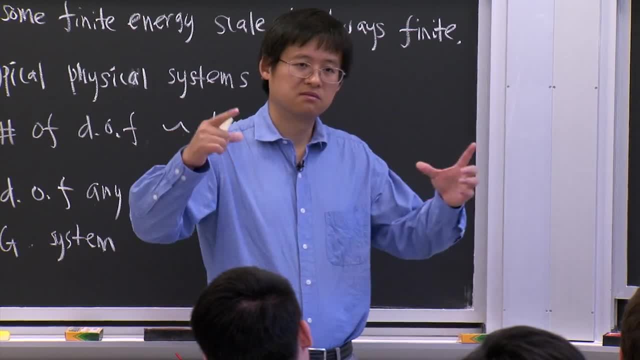 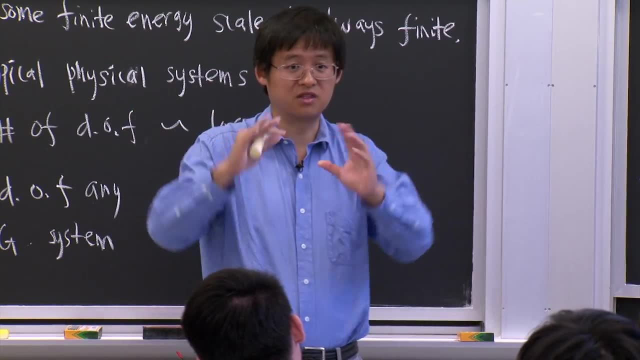 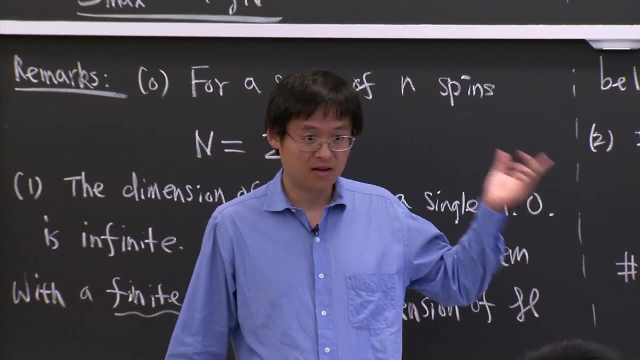 this would be constrained by 8-dimensional surface. Yeah, Yeah, just, no matter what dimension, it's always constrained by the surface, not constrained by the volume, no matter in what dimension. Other questions? I just have a question back in there. 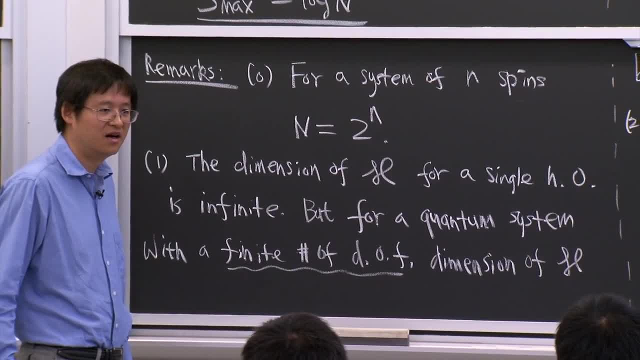 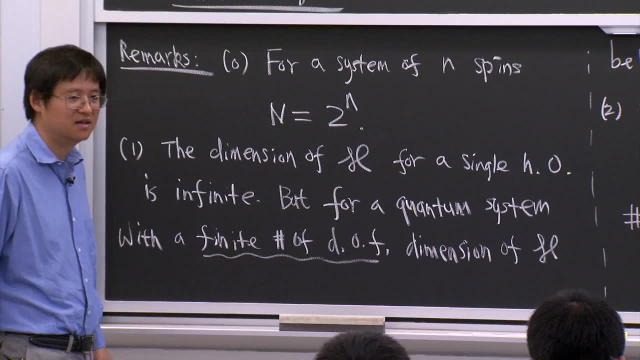 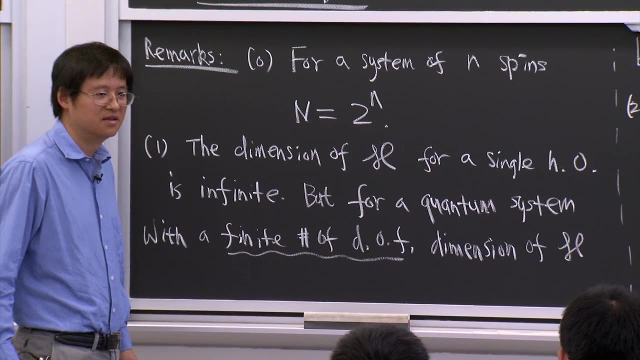 Yeah, So it seems like we must. we are like constraining a system, a quantum theory, And that its number of states for a given energy must grow slower than some. It must be lower than some finite energy. right Yeah, The number of states must be low. so 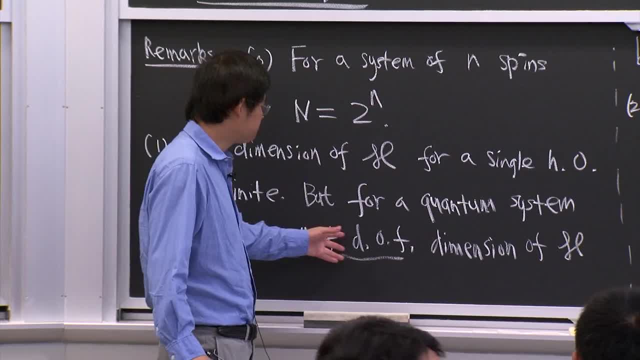 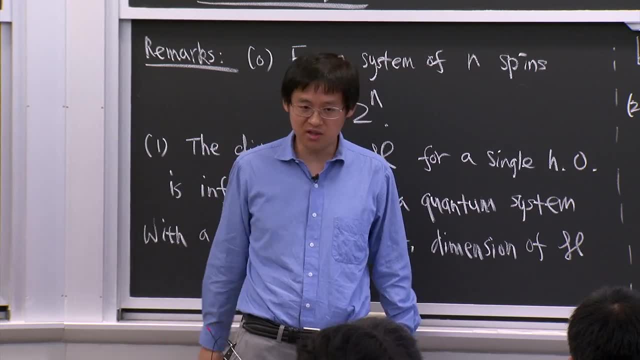 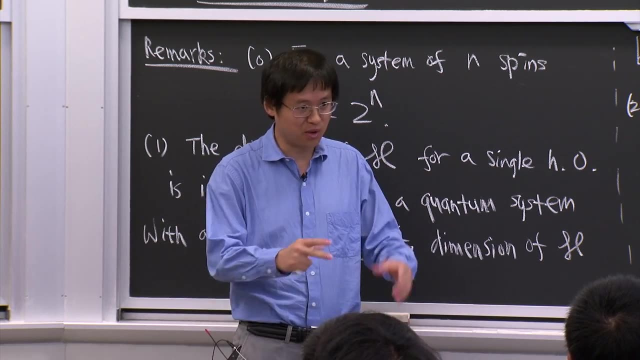 Yeah, just say essentially what we said earlier is that if you are in the theory of quantum gravity, there's a cutoff on the maximum energy you can have, And there's a cutoff also on the maximum energy you can have, because otherwise you form a black hole. 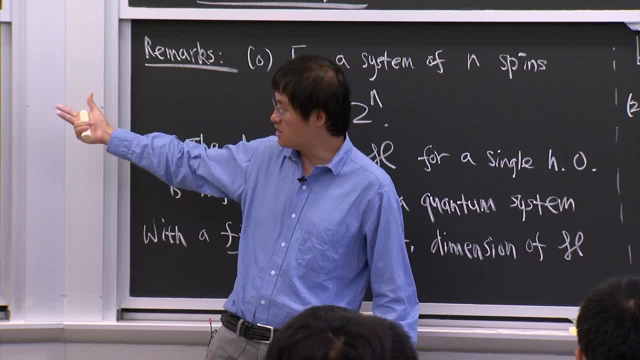 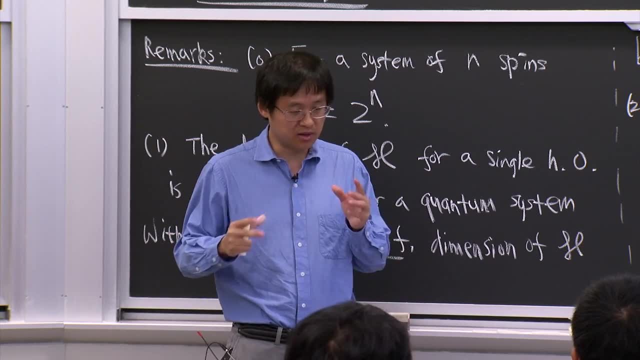 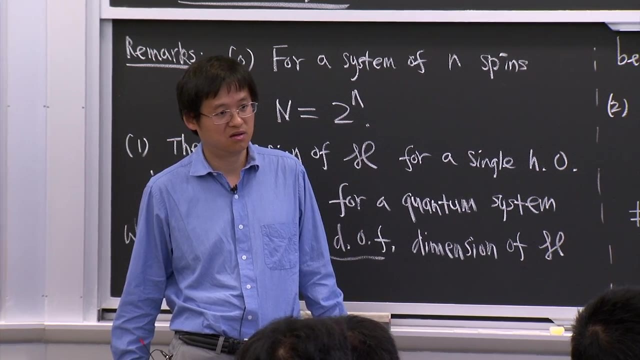 And then that cutoff translates into the state of the entropy and into the number of degrees of freedom. Yes, I mean Because much easier, yeah, yeah, For example, first we start with a simple theory, then maybe we, for example, we add, for example: 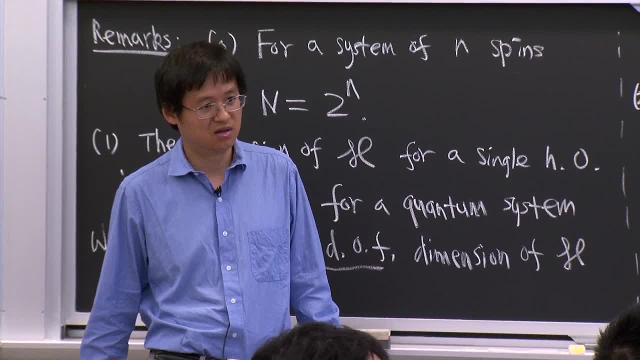 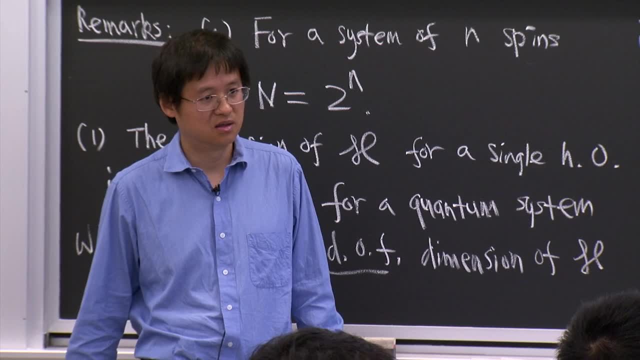 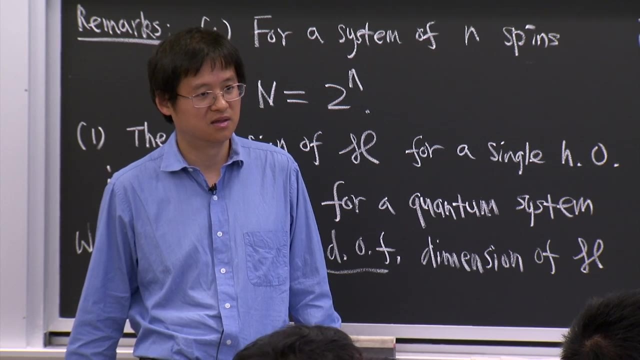 standard model. then we add supersymmetry, Then the energy spectrum, the limiting energy spectrum, the energy that is there, but the number of Hilbert states is more. And we can keep doing things like that. Yeah, But we can't, because it must be below this value. 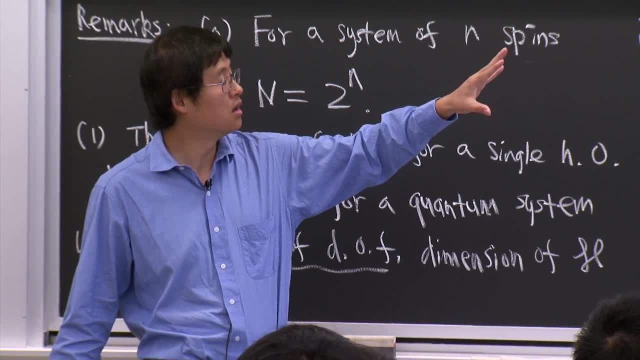 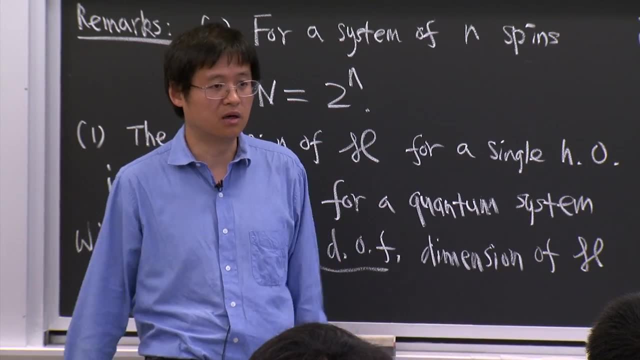 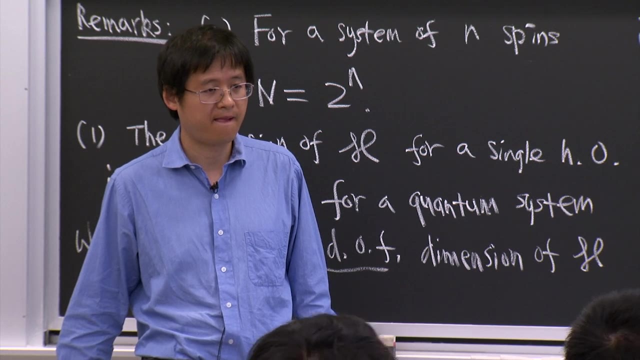 Yeah, but you see, there's something about the volume here You have to talk about within some region. Of course, abstractly, you can put some degree. Yeah, maybe I'm not getting your question. I was just saying now, if we overthink, we can just. 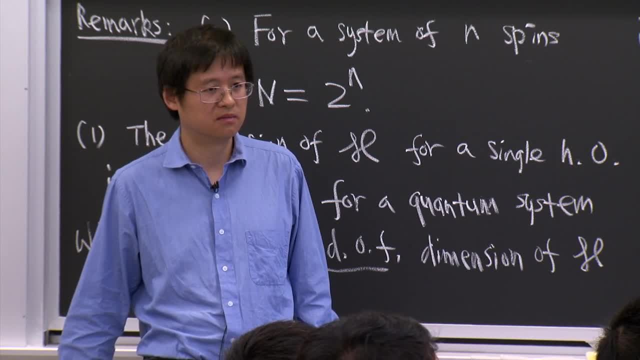 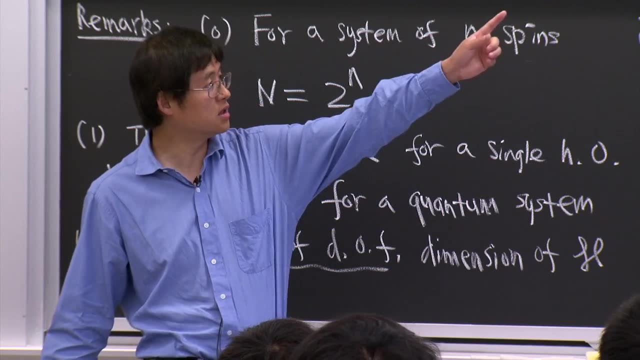 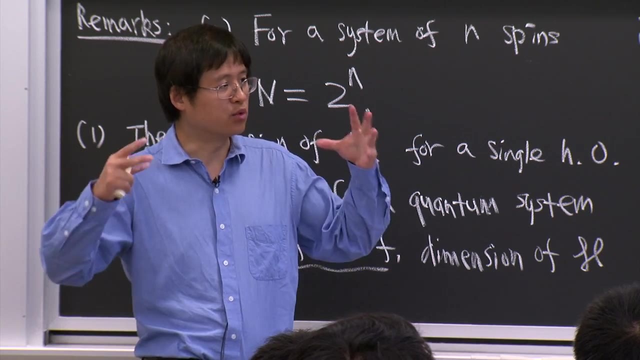 for example, say, the energy bound is here and below this, how many states we could have? No, no, no. This is not the direction in terms of the energy bound. This is, in the end, is the bound on the long body. 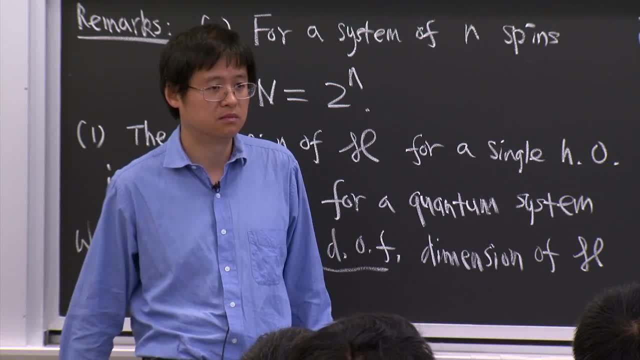 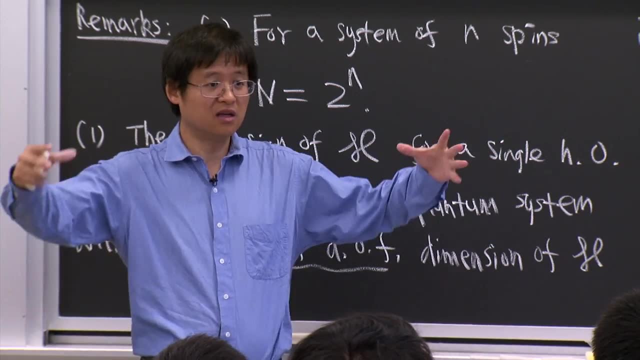 with freedom you can put inside a region. If you put too many degrees of freedom inside a region- Yeah, Inside the region- then you need to enlarge the region. Yeah, just say. it looks like the number of degrees is incompressible. 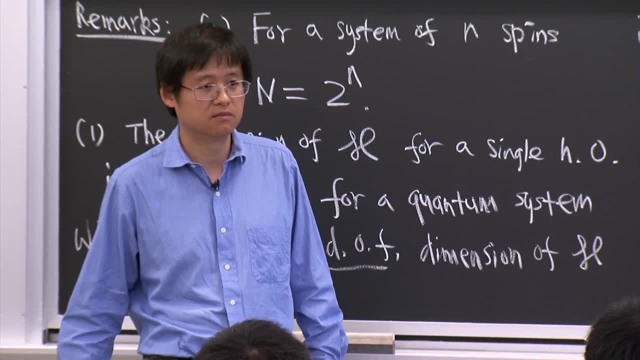 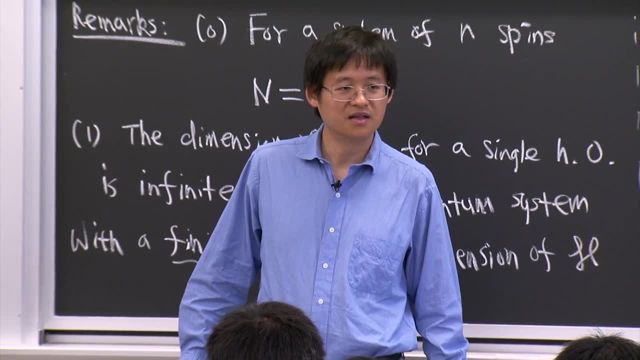 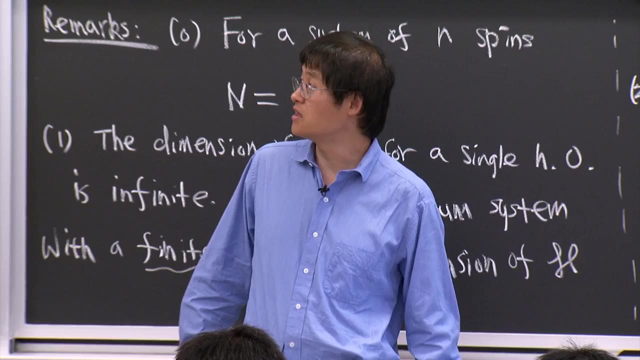 Something like that. OK, I have a question regarding back to your other. So I still don't understand. shouldn't the isolated system means also including the machinery to do these things? No, I'm just saying you start with the isolated system. 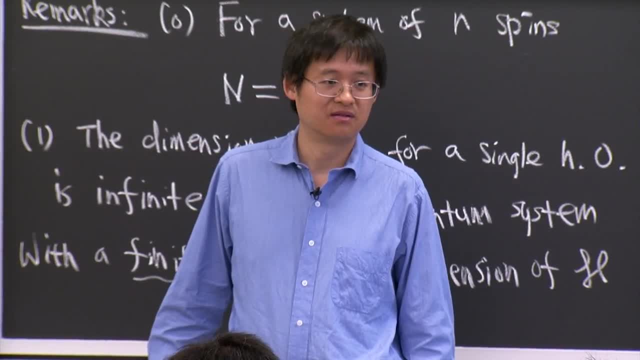 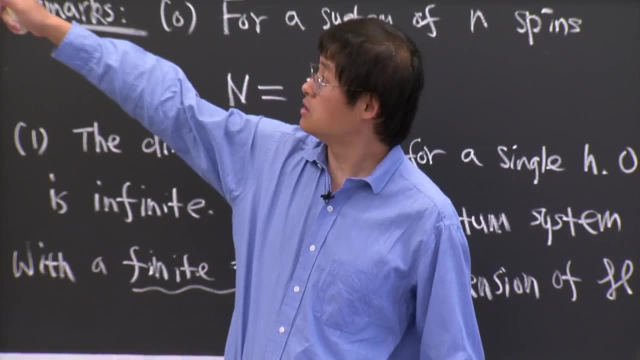 then you can add something to that isolated system. But what about we take matters out of the black hole? This equally will. No, no, you take it. No, that thing, that isolated thing, does not have to be a black hole. 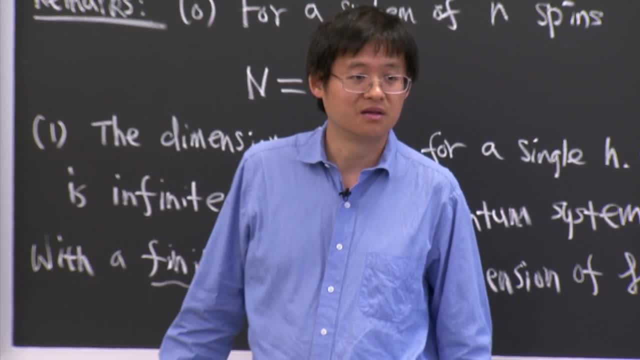 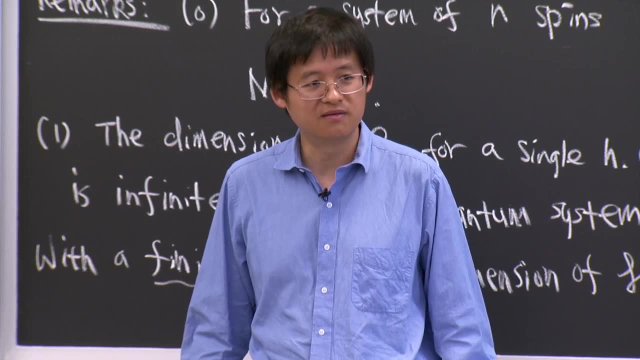 It can be anything. It just can be anything. So if we, instead putting energy inside, we take energy out- Yeah, you take it- Entropy will decrease. Yeah, just take entropy out. Yeah, Then this bound will be even more satisfied. 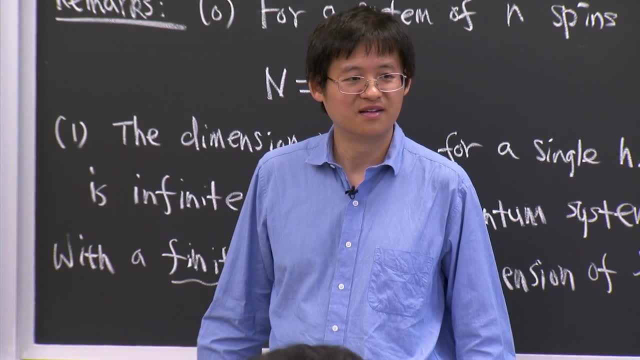 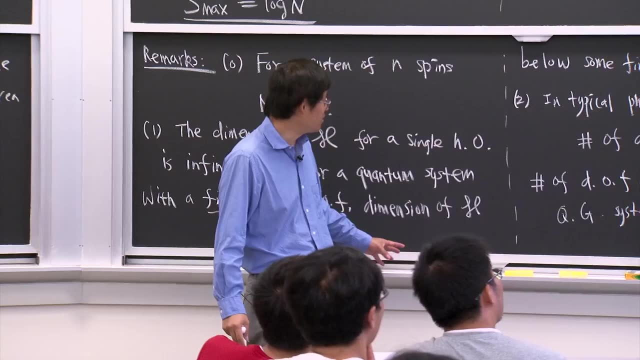 I have a question there: The grid, The degree of freedom, Yeah, I mean log of the degree of freedom. No, no, N is the dimension of the Hilbert space, N is the dimension of the Hilbert space. 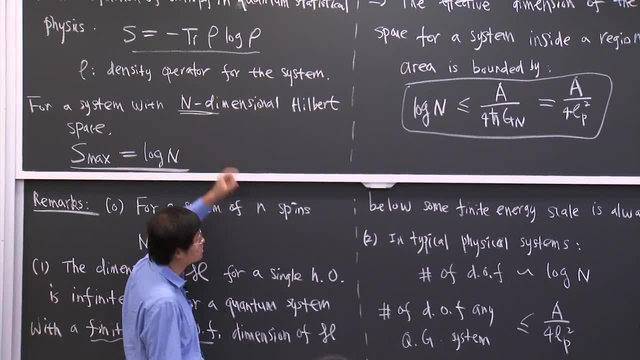 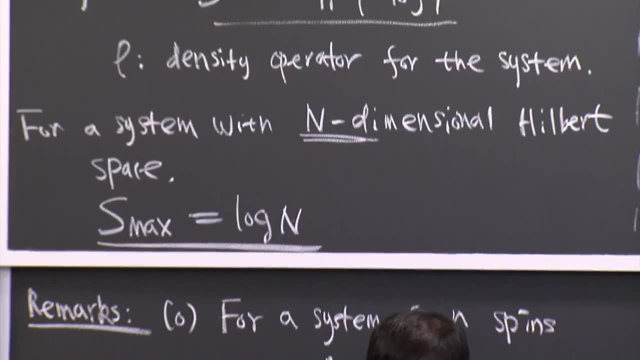 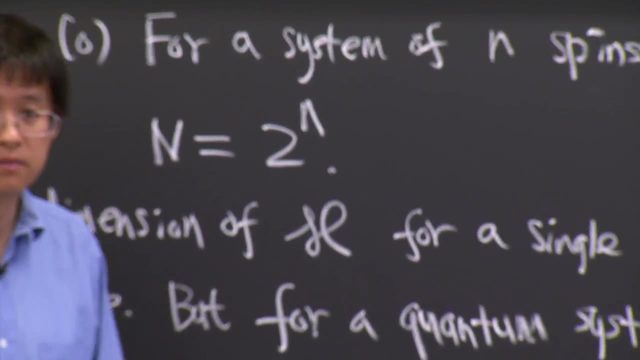 That's what I call the N here N- dimension of the Hilbert space. Typically, the dimension of the Hilbert space is exponential of the number of degrees of freedom. Just look at here. Just look at here. Yeah, Any other questions? No, OK, If we have a quantum field theory, it has a certain vacuum energy, right. And then if you now consider that to be the vacuum energy and you expand it at some point, it will actually collapse into a black hole. 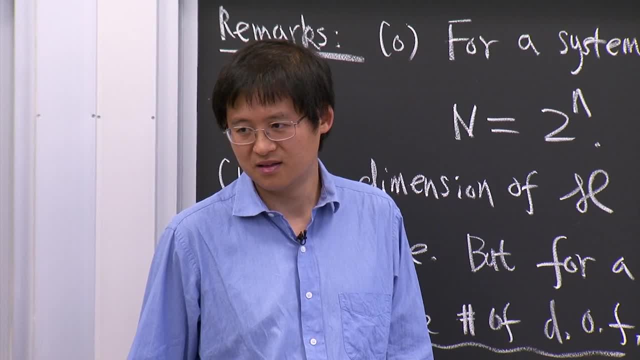 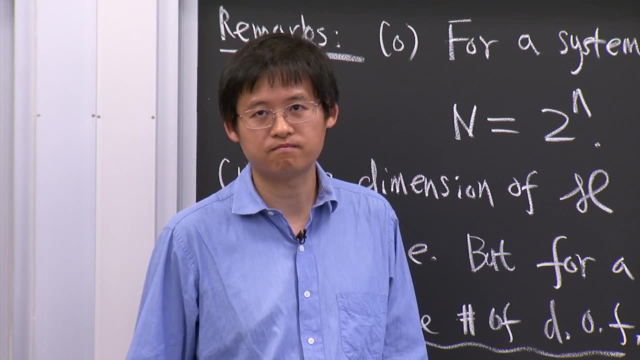 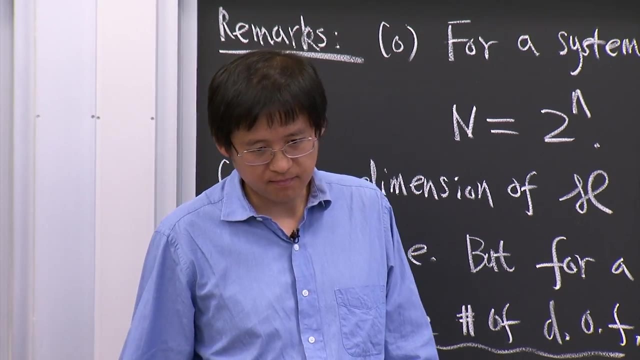 So if you take the vacuum energy to be that predicted by T of t, then for the universe it would not pour, Even theoretically. I mean, I know the cosmological constant is 120 orders, Not less. but Yeah, That's a little bit tricky because the vacuum energy will. 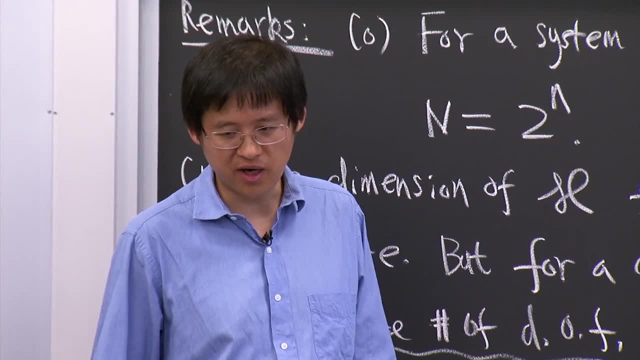 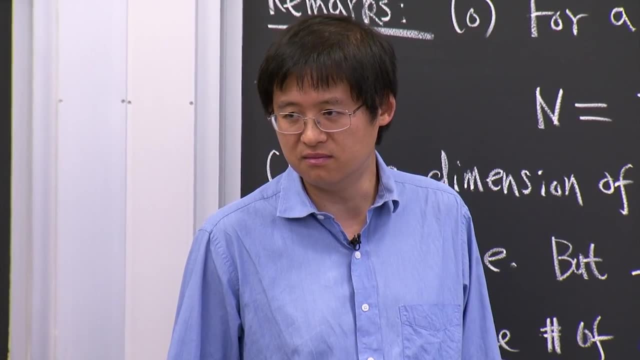 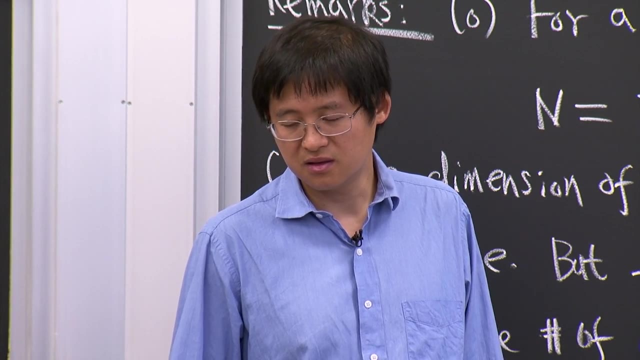 make it into, say, depending on whether the vacuum energy is positive or negative, make it into de-sitor, anti-de-sitor? Yeah, Then you try to see whether. yeah, It depends on details. But if you go big enough it's going to collapse. No, Not that. I'm just saying that you have to formulate a little bit differently. Are you talking About the particular state of certain energy to couple to gravity? Then you just take that state, couple to gravity to see what you get. 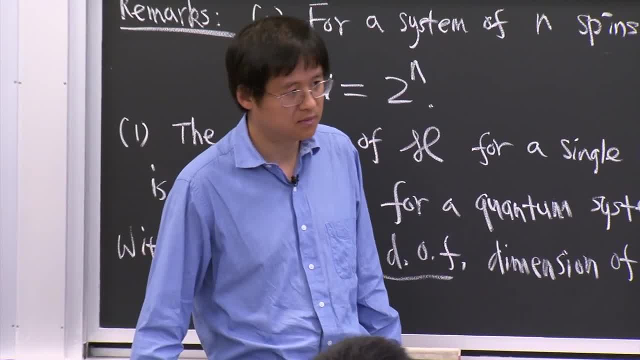 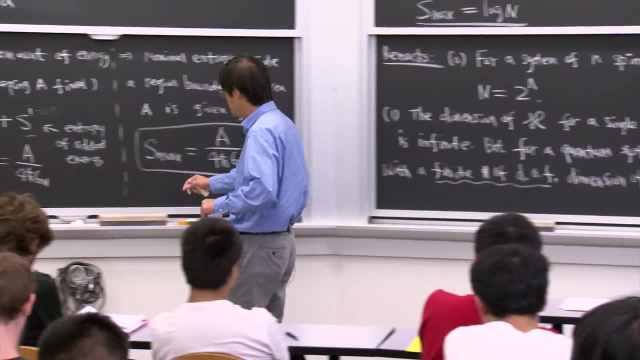 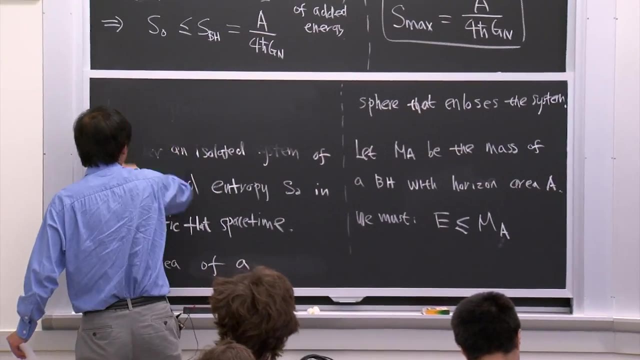 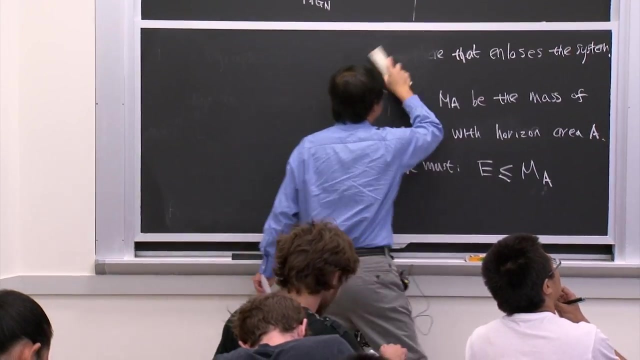 Yeah, Then ask questions from there. Good, So now let's move to a new topic. Still is in the preparation to go to the duality, But we need a lot of piece of importance, A piece of important intuition, in order to fully appreciate the duality. 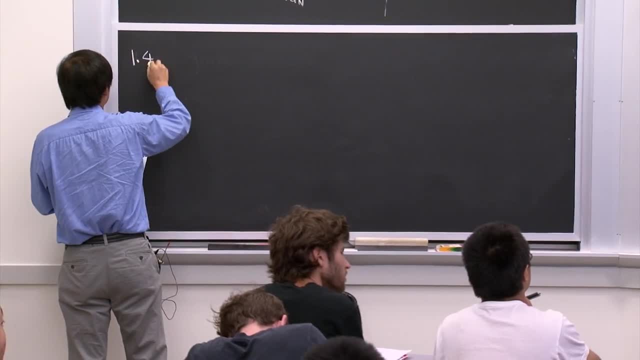 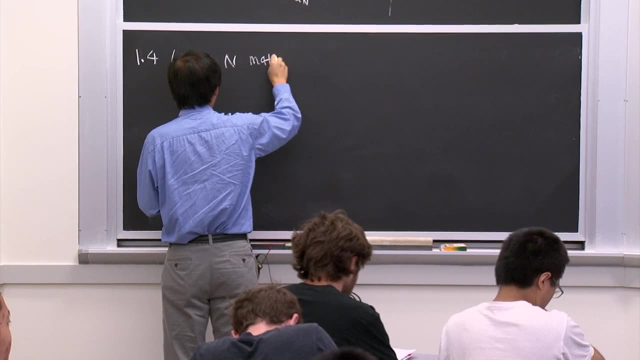 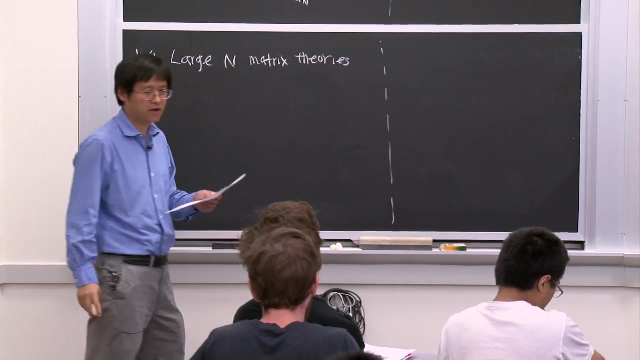 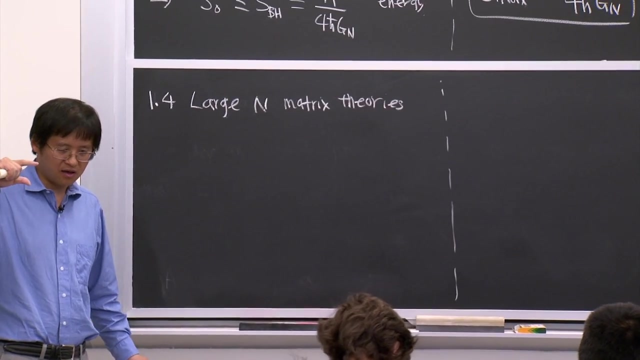 And this piece of intuition is Nagyian series, And let me call it Nagyian matrix series. OK, So now we want to look at the. now we try to look at the hints for holographic duality from the field theory side. 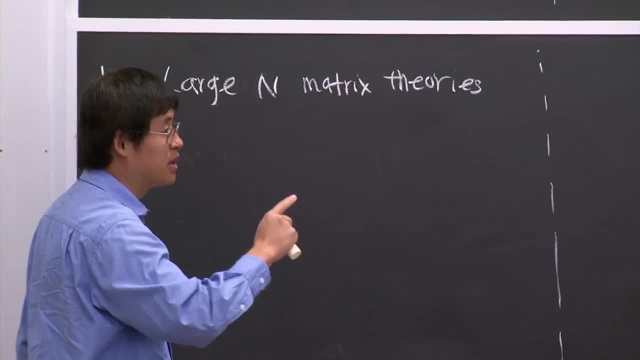 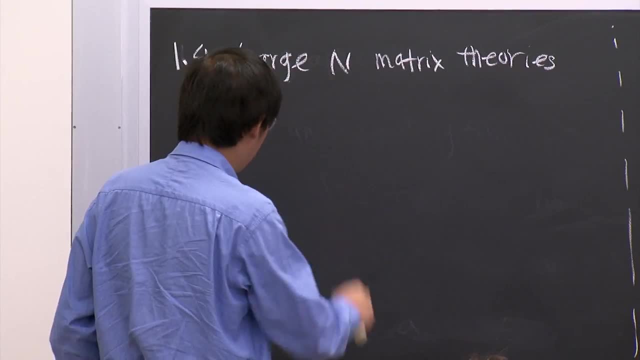 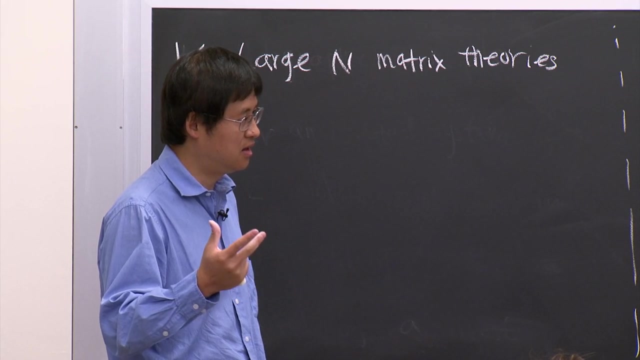 OK, From the field theory side. So far we have been talking about the hints for holography from the gravity side And now we look at it from the field theory side To see. actually from field theory side there's also some hints to relate a long gravity system. 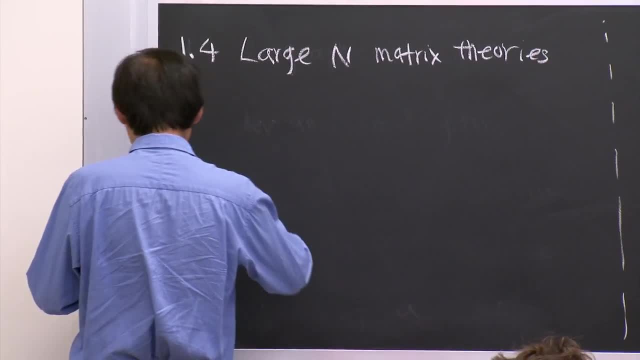 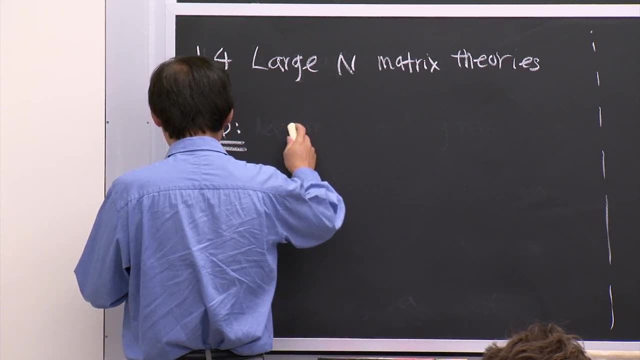 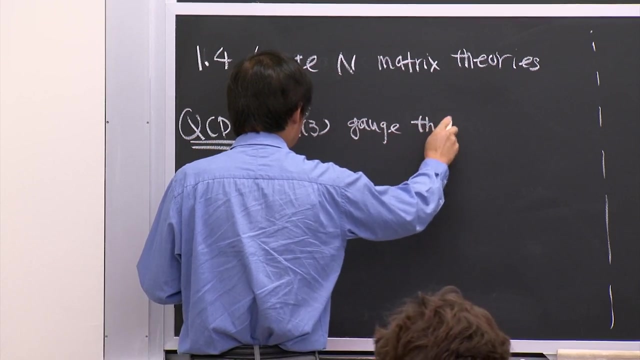 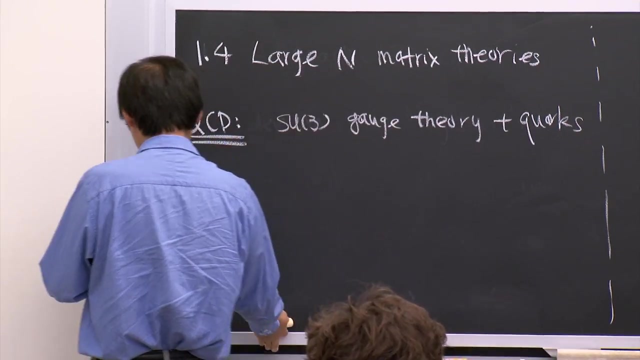 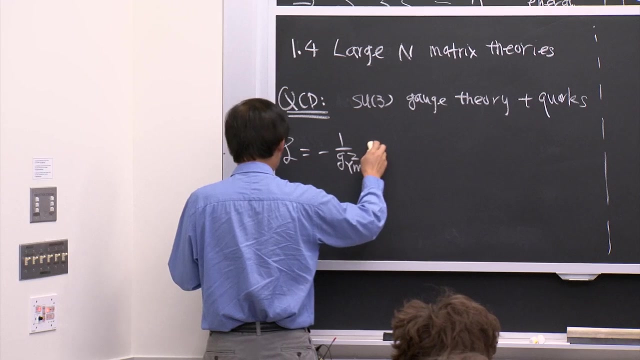 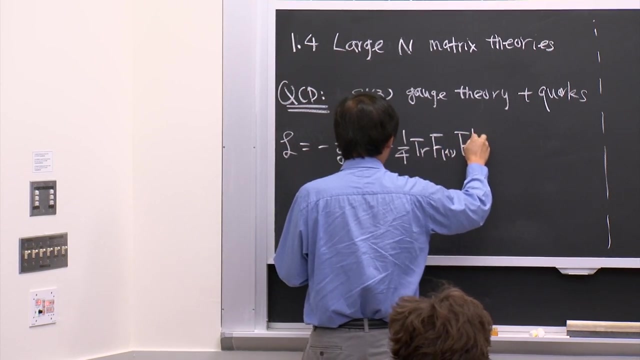 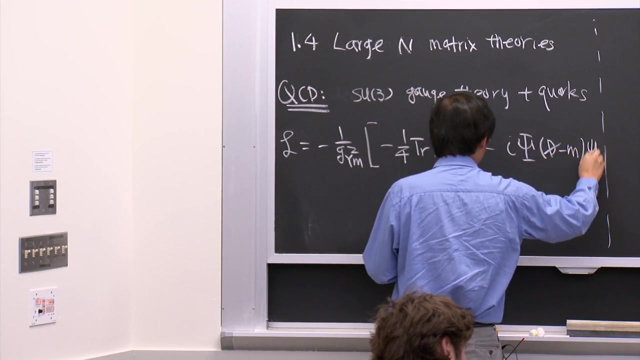 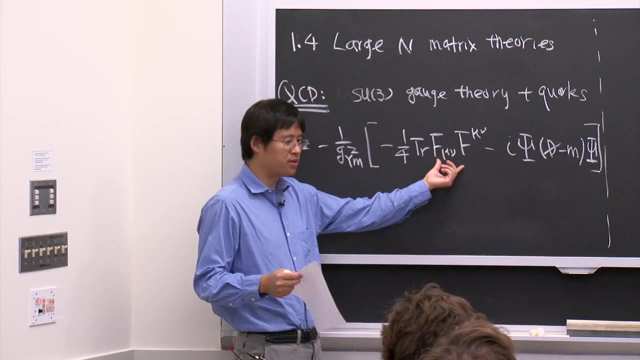 to a gravity system. OK, So let's start with QCD. So QCD is a SU gauge theory plus quarks. OK, So we can. so let me just write down: it's a Lagrangian. OK, So this F describes the gluon fields. 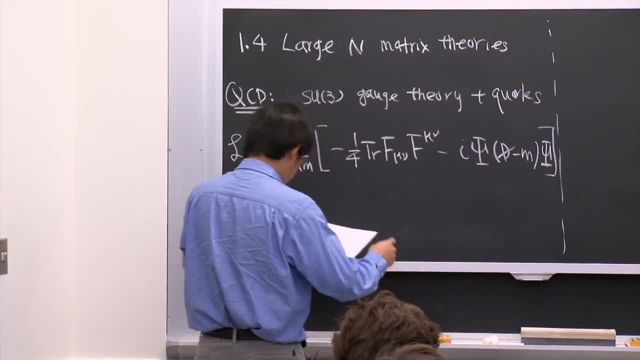 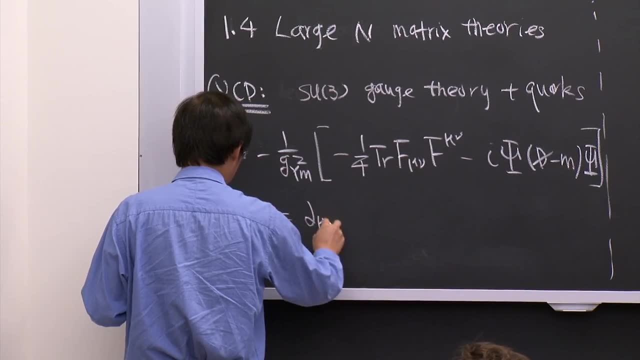 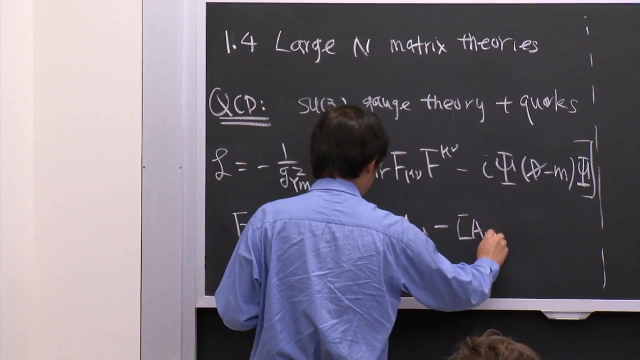 And this psi describes the quarks. OK, So this A, So this F, It's a Lagrangian. OK, So this F is built out of the standard partial mu A mu minus partial nu A mu minus A mu A mu. 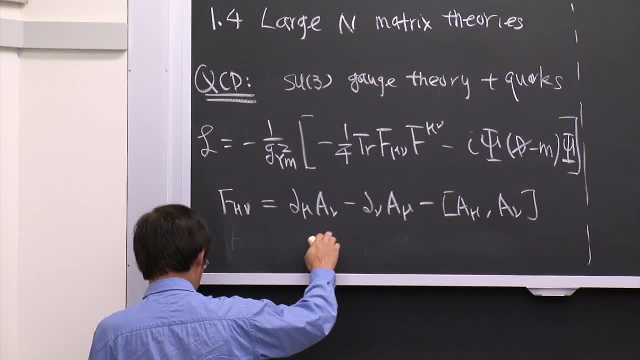 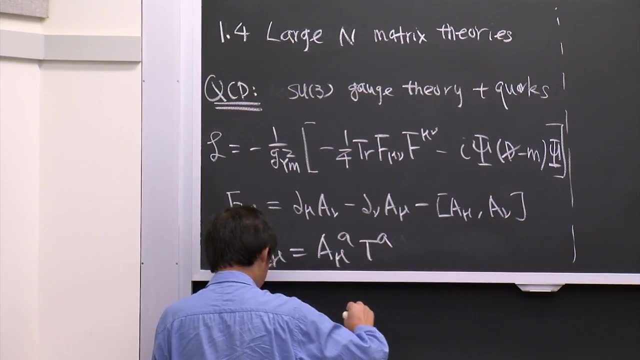 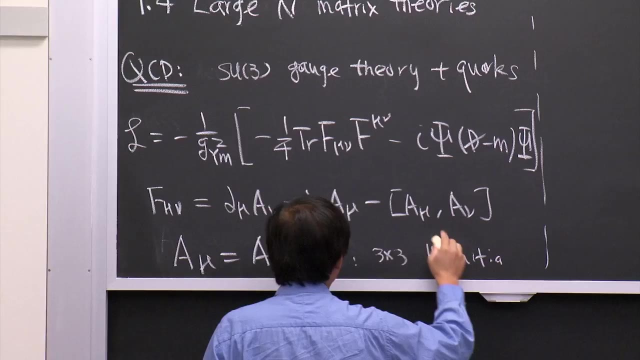 And A mu. each gauge field is a 3 by 3 Hermitian matrix. OK, So these are 3 times 3 Hermitian matrix. So this is using the matrix notation. So F is also a matrix. So there's a trace here. 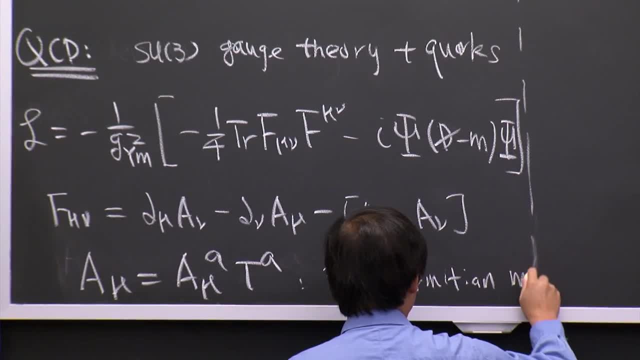 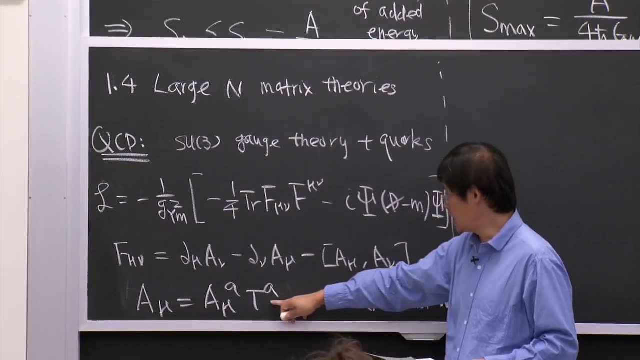 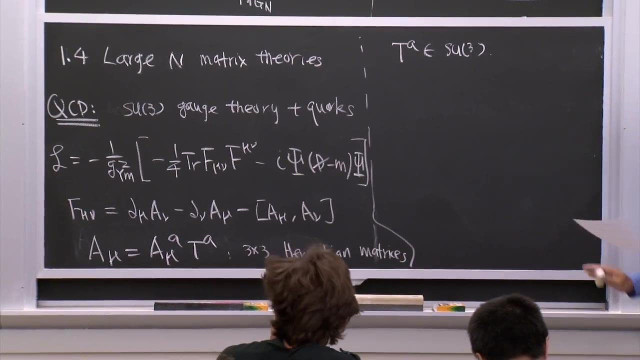 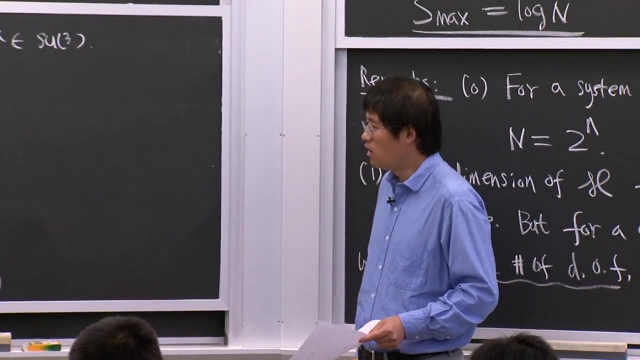 OK, Hermitian matrix And the TA is just the generators of SU3.. OK, So it doesn't matter if you don't know QCD, It doesn't matter if you have not seen QCD before, QCD before. The only thing matters is just to remember. 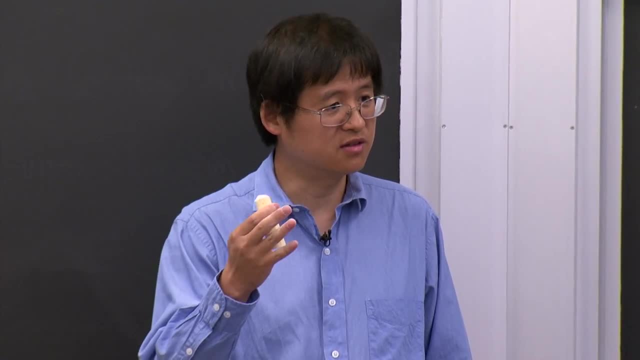 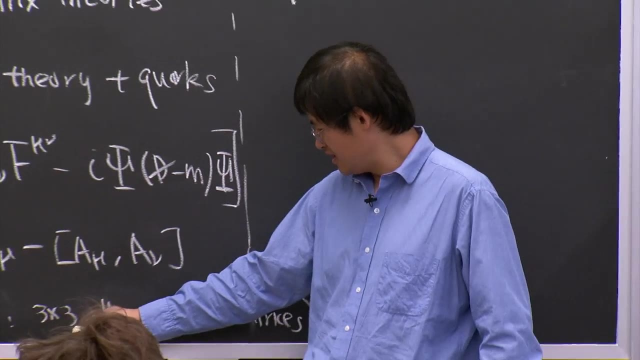 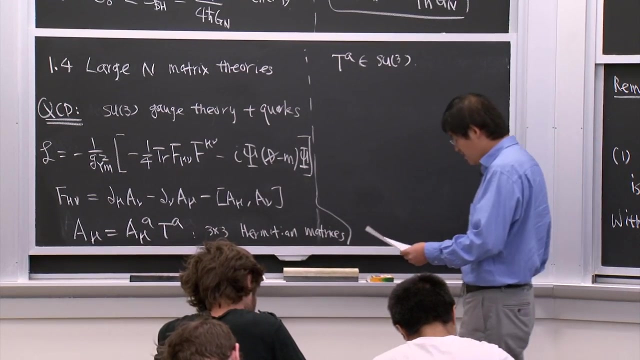 that QCD is a theory of matrices. QCD is a theory of 3 by 3 matrices. OK, So the gluon field is a 3 by 3 matrices. It's described by matrices. So, of course, one of the remarkable things about QCD- 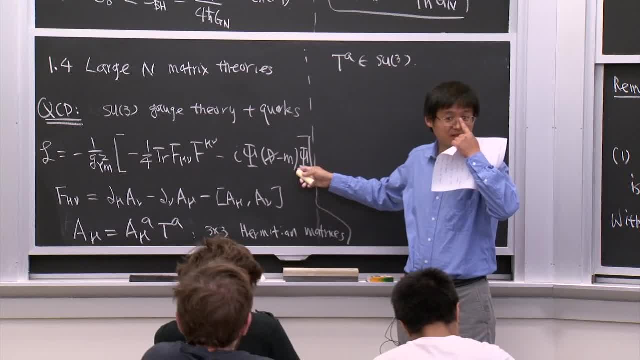 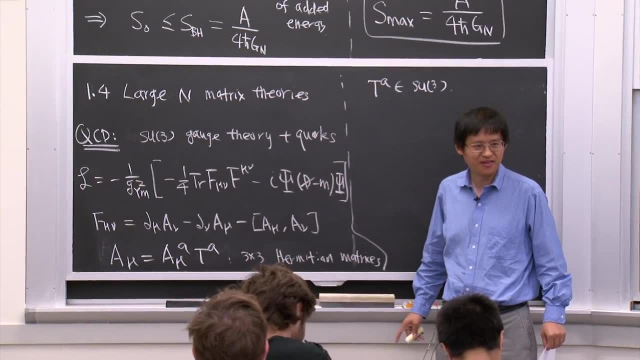 what's the most remarkable thing about QCD Do you know? Yeah, that's one. And what other remarkable thing about the QCD? Self-contained, Hm, Self-contained? Yeah, it's related to that Confinement. 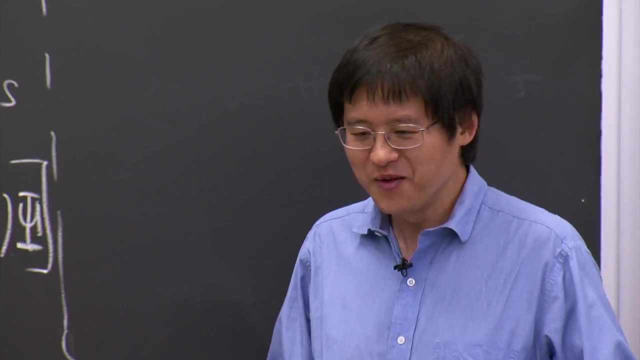 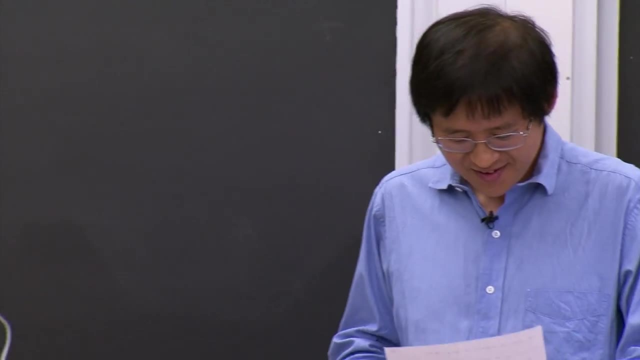 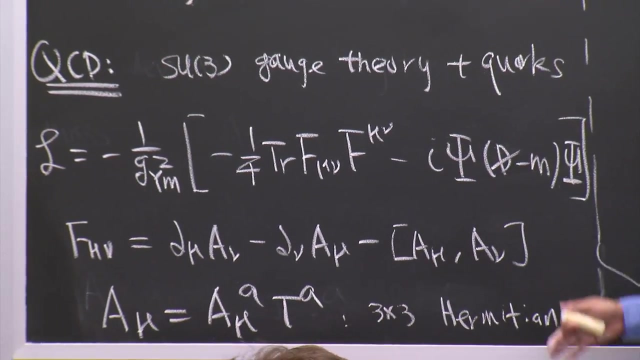 Yeah, confinement is also related to that. Yeah, one of the most remarkable things about QCD is still not solvable, And the reason for that is because QCD is not solvable- is because when you go to low energies, the coupling becomes strong. 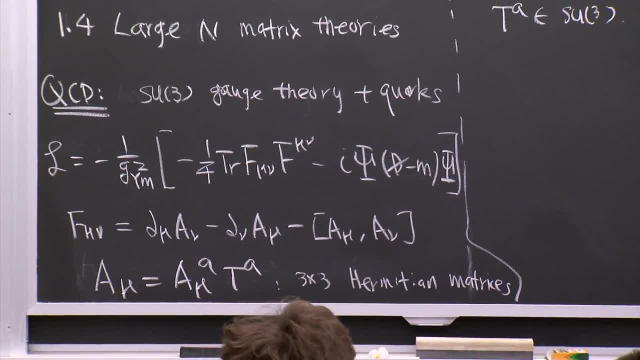 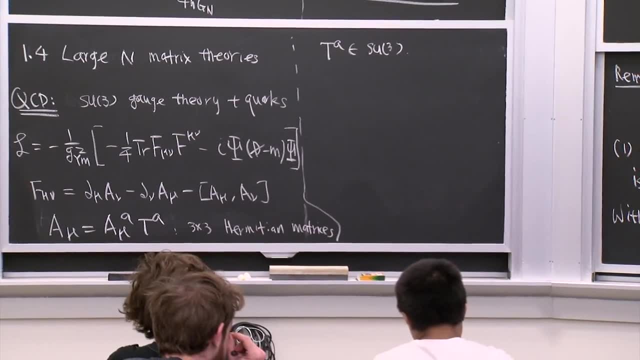 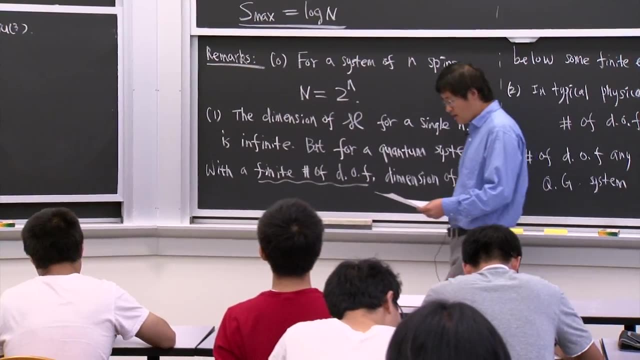 Then we don't know how to deal with it. OK, So we still don't know how to calculate it. from first principle, Of course we can put it on the computer, but just in terms of theoretical understanding it's hard. So in 1974, so this is an old problem. 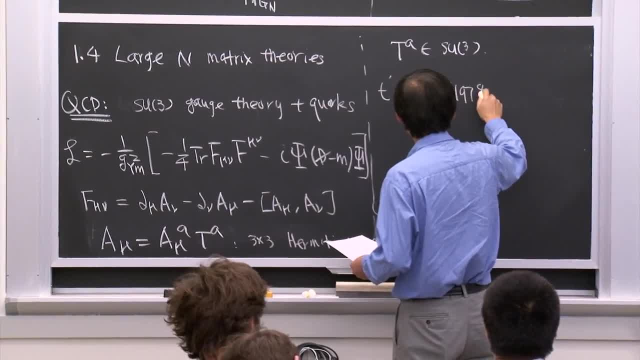 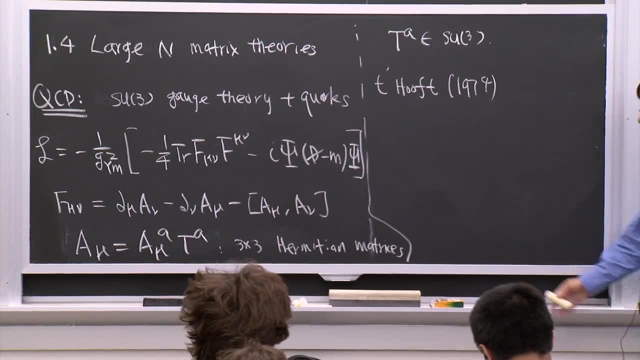 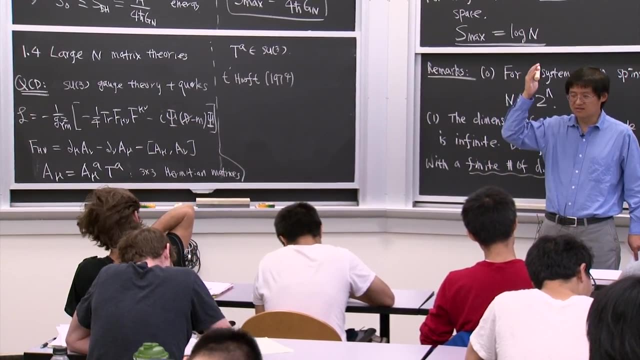 So starting in 1971, people already tried to solve it, So in 1974,. so the big problem with this thing is that in quantum field theory normally we do expansions. OK Say, we find some starting point. So in physics that we always do. 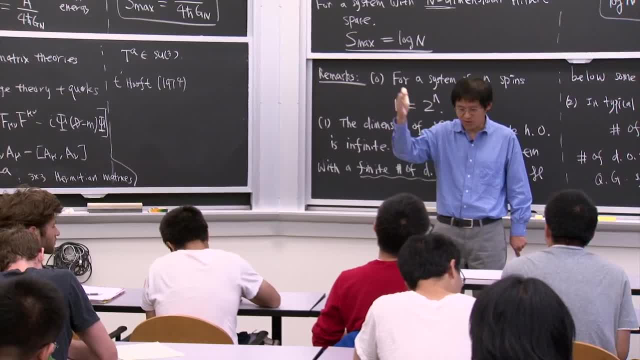 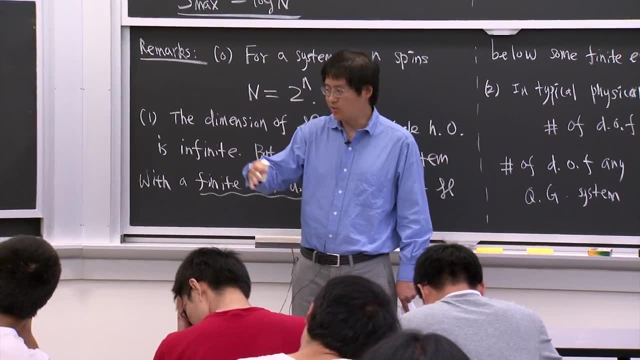 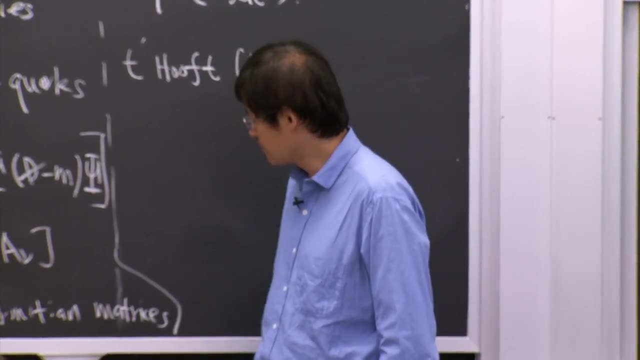 We find a starting point which can be solved, Then we expand around that starting point, And that starting point is often a free theory. OK Yeah, And then we expand around the free theory. So the difficult thing about this theory is that first it's hard when you go to low energies. 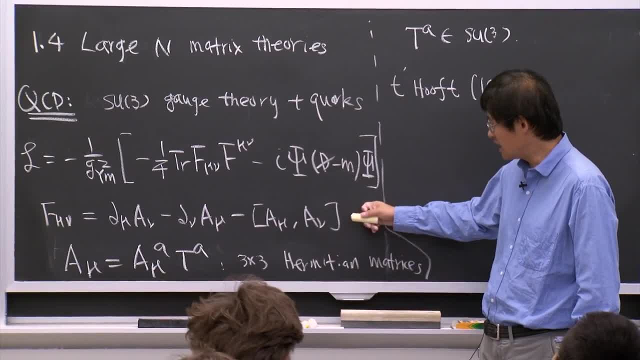 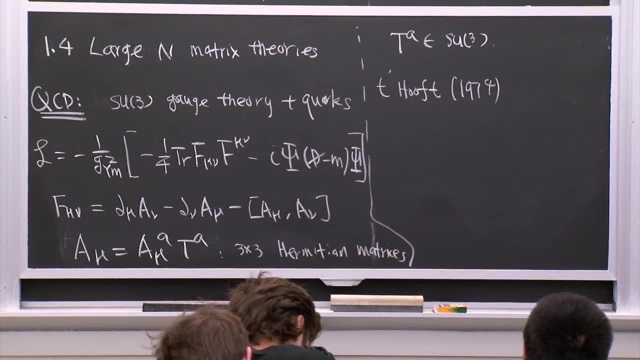 First, it's hard to find the starting point. And the second is that there's nothing to expand because there's no small parameters. OK, There's no small parameters. When you need to expand, you always need a small parameter. So in 1974, to come up with a 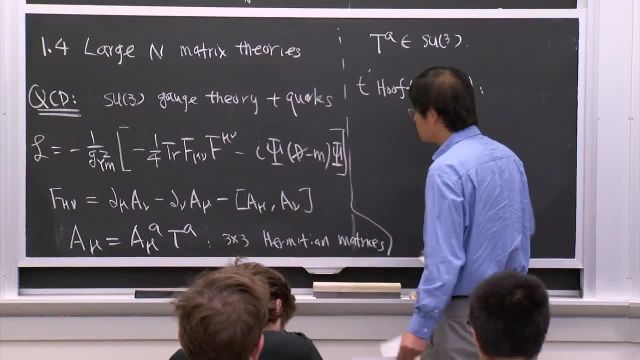 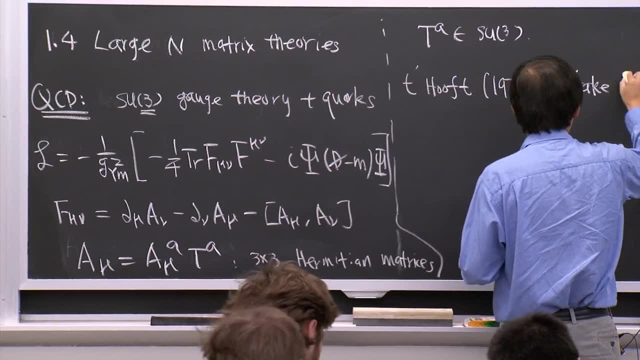 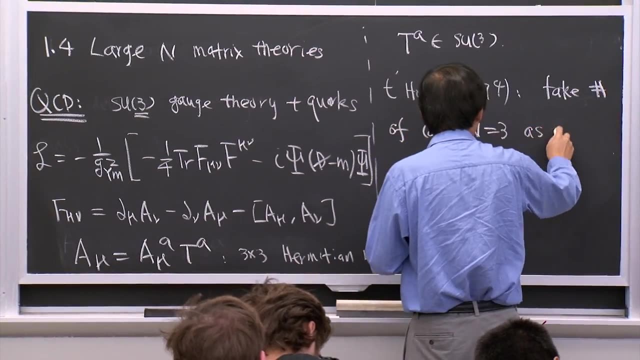 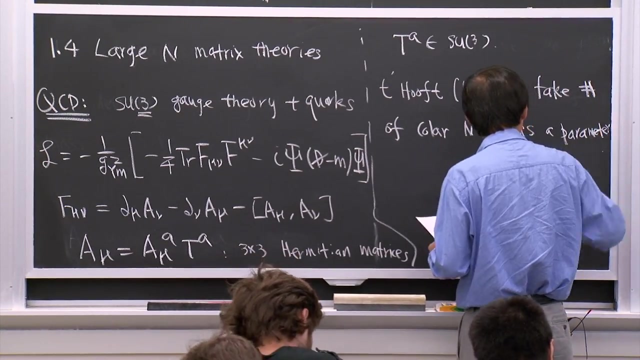 very nice idea. he said: this is SU3.. He said: let's just take the number of color, which is n, equal to 3, as a parameter. So even though in real life he said there's only three type of colors, 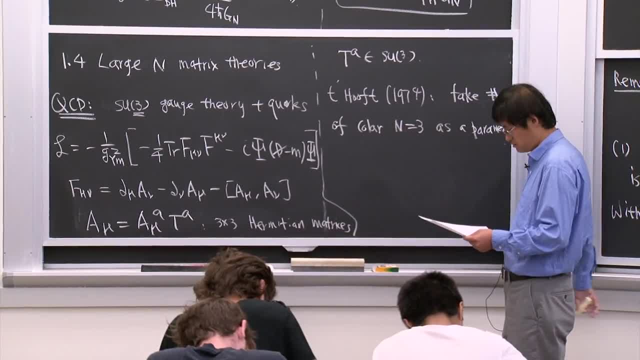 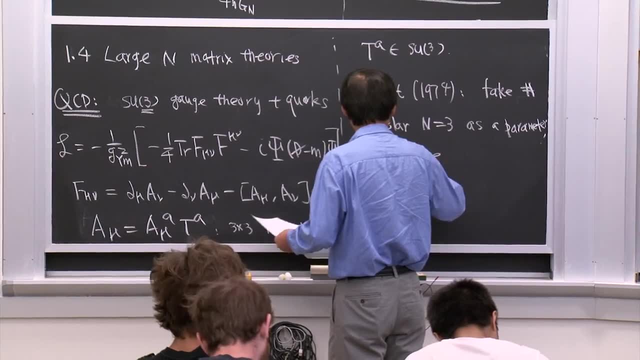 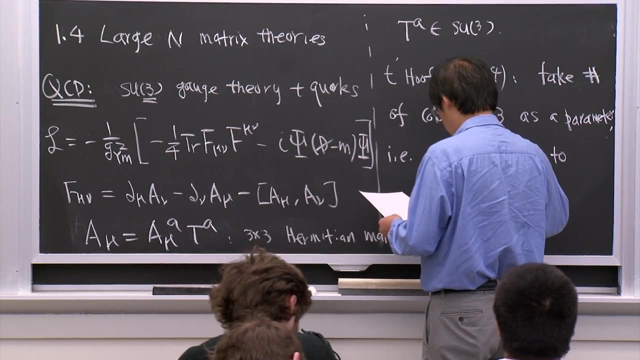 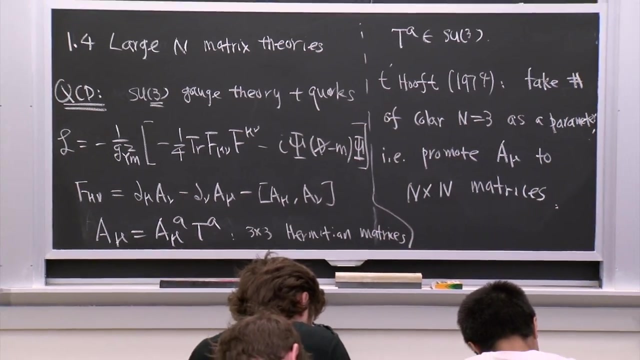 But let's imagine we treat it as a free parameter. OK, So this just implies, say you promote the gauge field to m by m matrices, m by m Hermitian matrices, OK, OK, He said let's just treat this in terms of m by m matrices. 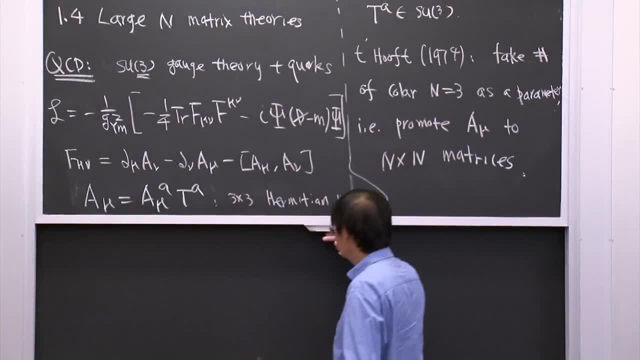 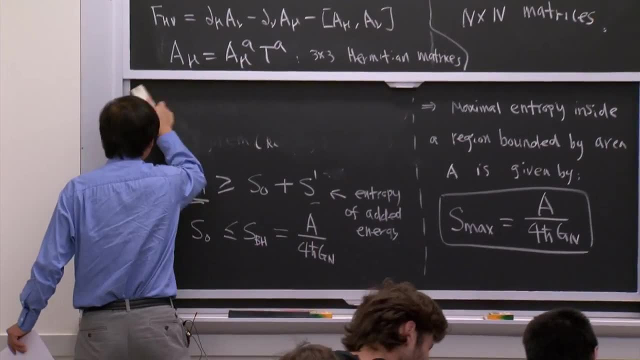 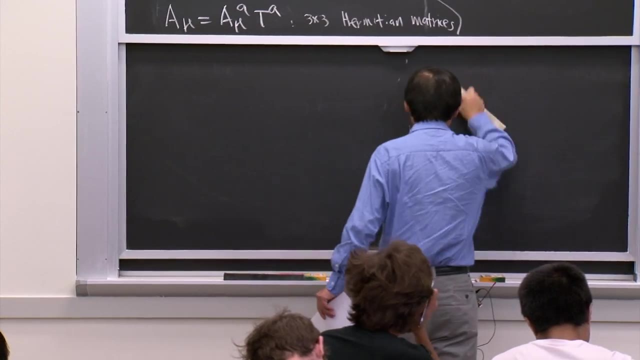 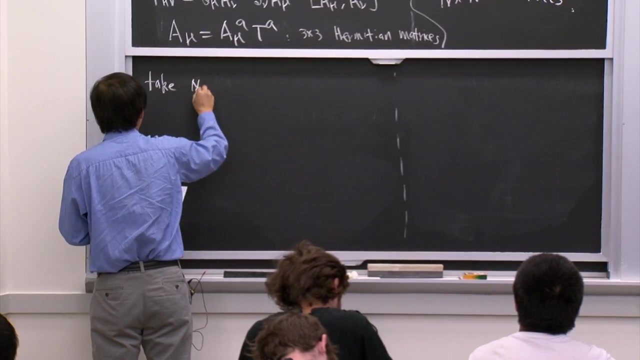 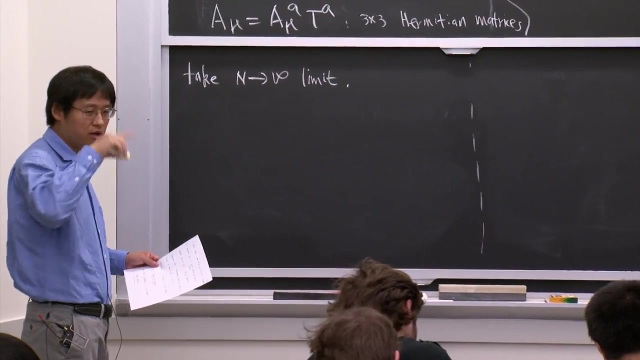 And then let's consider the angle to infinity. Let's consider the angle to infinity limit. OK, So let's consider the angle to infinity limit. Sorry, So he reasoned. If angle to infinity, If angle to infinity limit is sufficiently simple, 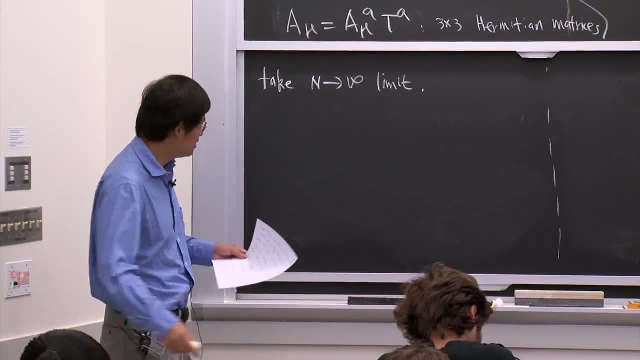 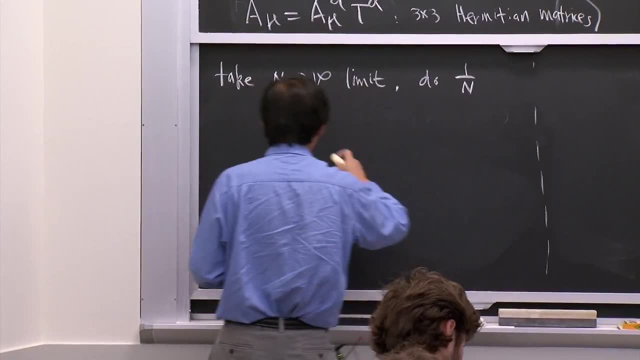 then maybe we can solve that limit And then do 1 over n expansion. 1 over n, then it's a small parameter. Then we can treat the 1 over n as a small parameter And then do 1 over n expansion. 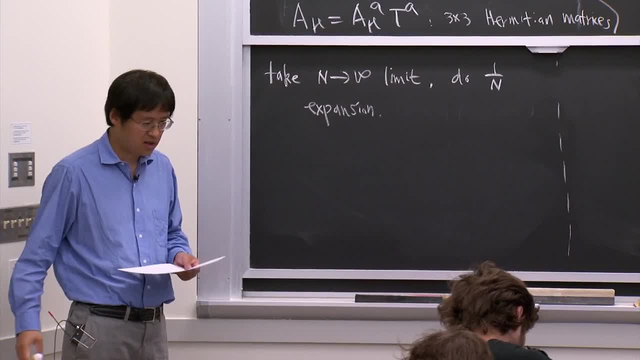 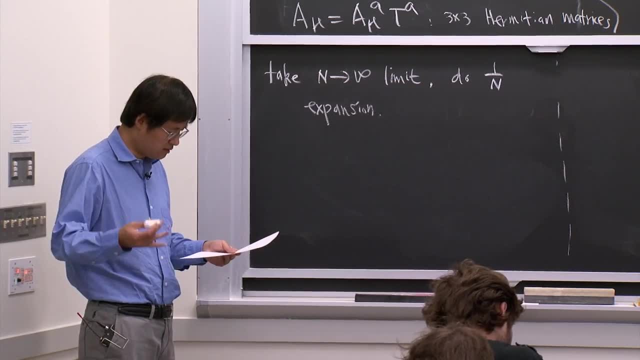 OK, So that's the rough idea. And then you get a small parameter with the 1 over n. So in real life n will be 3.. So 1 over 3. It's not the 1 over 3.. 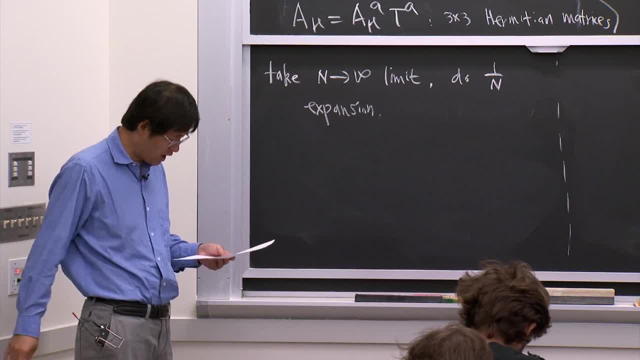 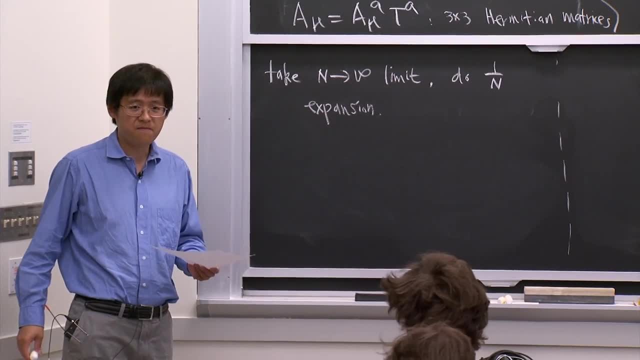 It's not the 1 over 3.. It's not very small, But it's at least smaller than 1.. OK, So this turns out to be an ingenious idea. Turns out to be an ingenious idea, But unfortunately, QCD still cannot be solved this way. 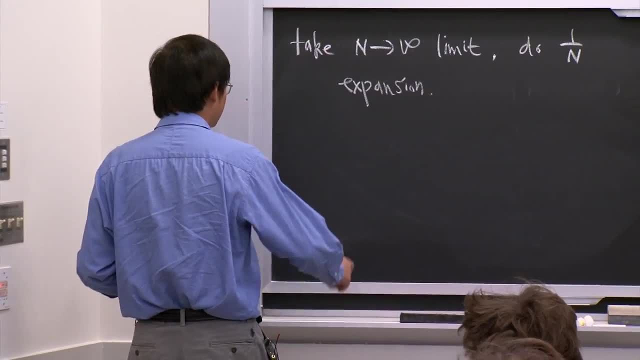 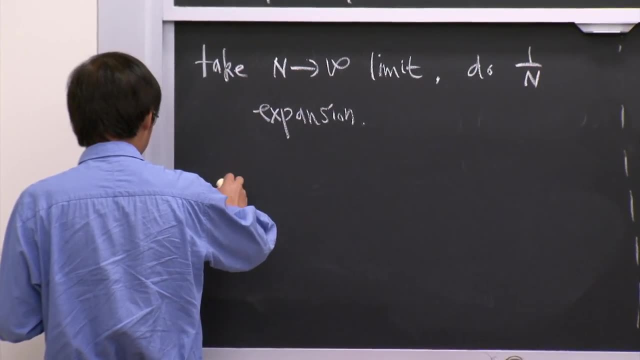 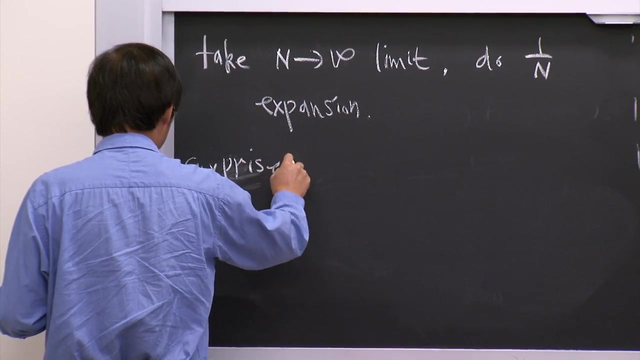 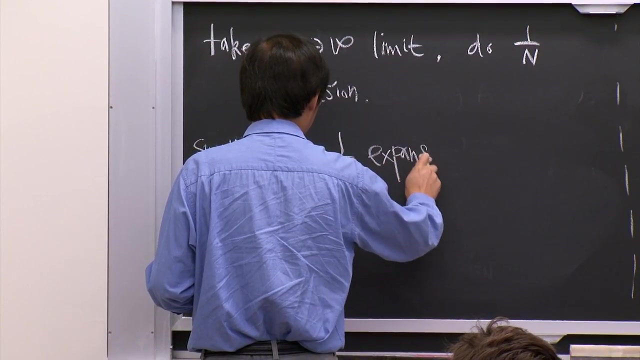 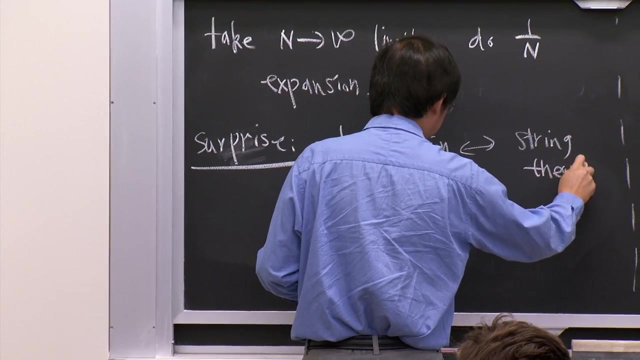 But there's a surprise. So still QCD. you cannot solve this way. Even angle to infinity limit turns out to be too hard. But there's a surprise, It turns out this 1 over n expansion gives you a string theory. OK. 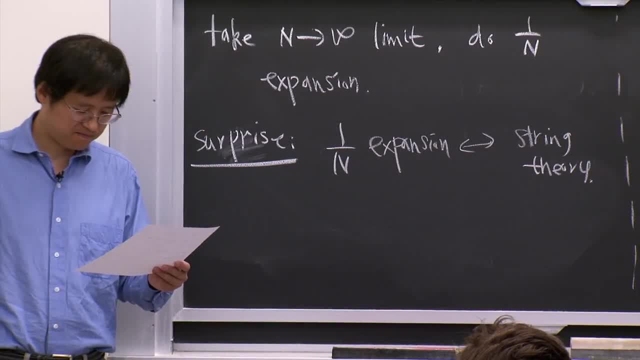 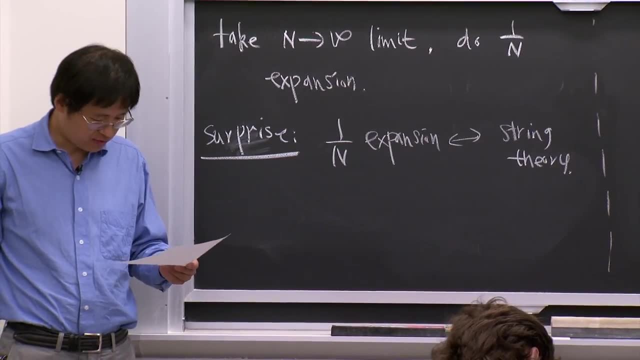 So I will now explain this. OK, So I will now explain this. OK, OK, OK, OK, OK, OK. So there's a byproduct of his large n expansion. He said: you find that this actually such a gauge theory. 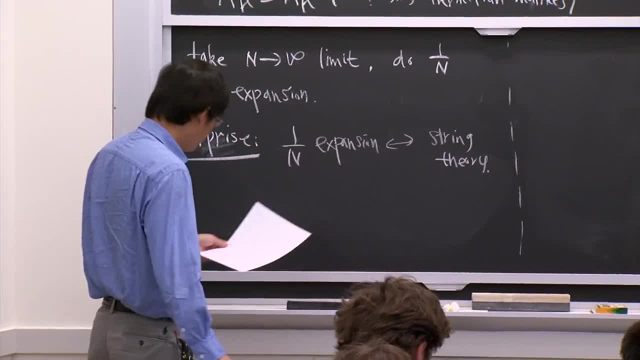 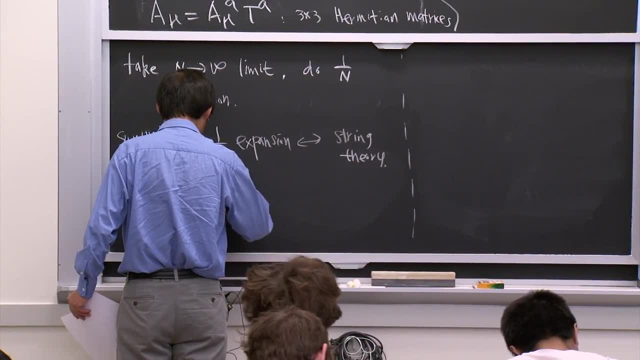 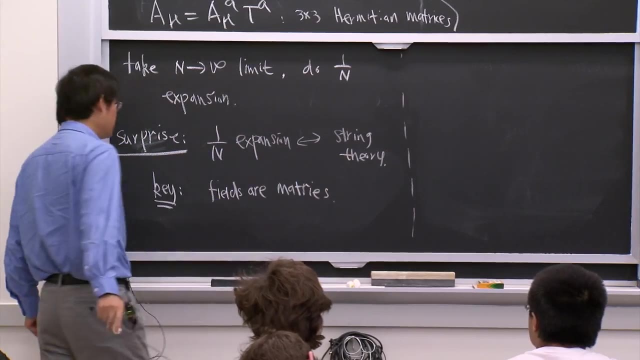 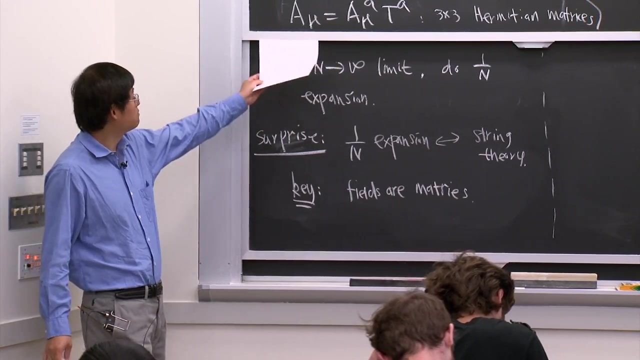 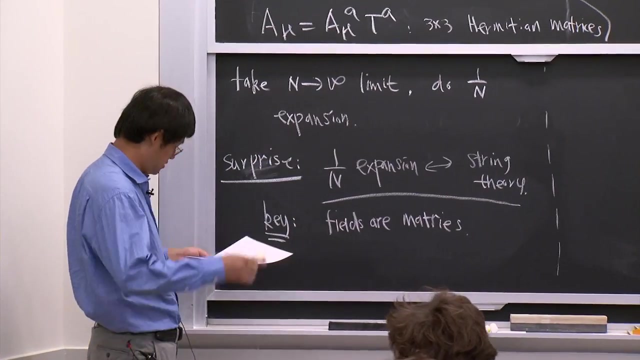 is actually, sequentially, a string theory. So the key is that these fields are matrices. OK, So the key reason this emerges is because we are working with fields which are matrices. So to illustrate this, I will not do the QCD, It's a little bit complicated. 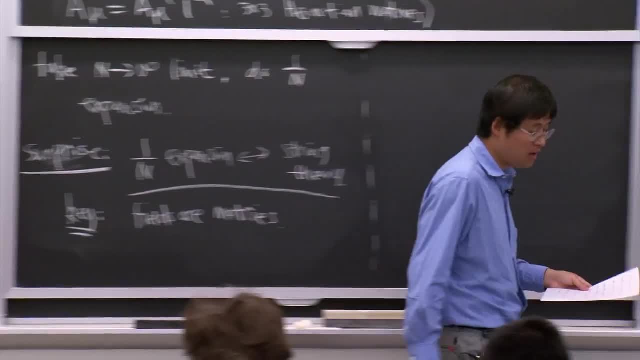 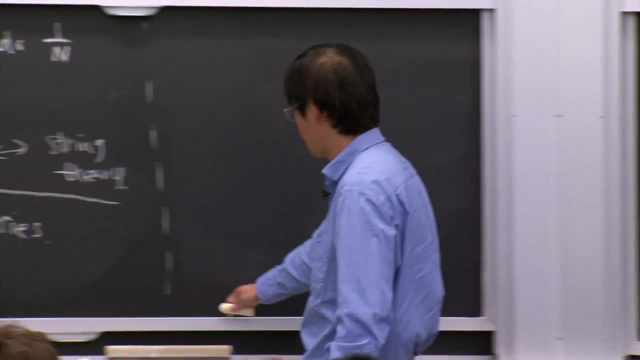 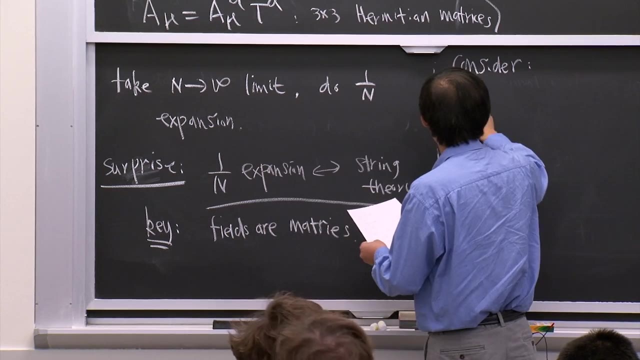 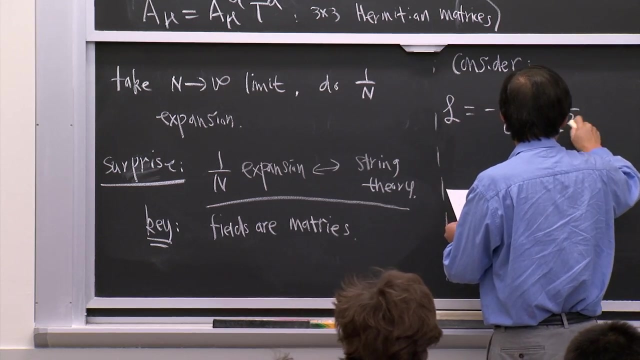 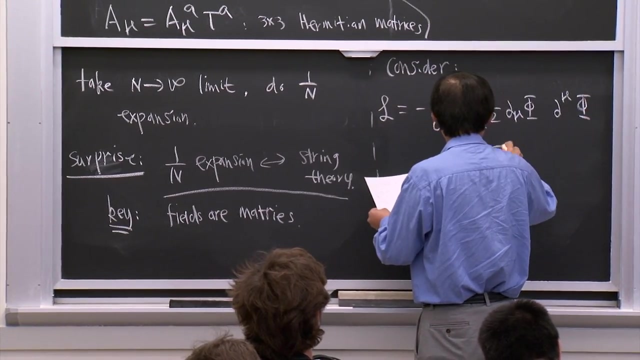 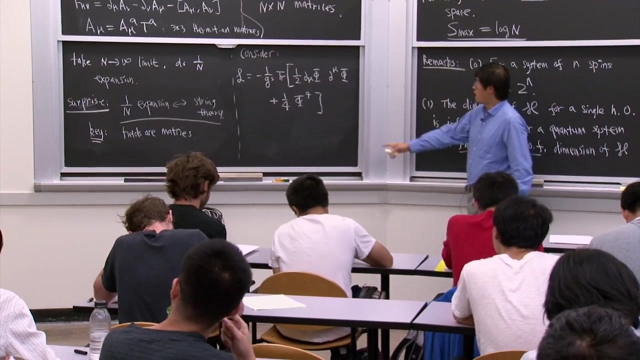 I will just do a simple scalar field theory. OK, So we'll just do a simple scalar field theory as an illustration. So let's consider the following theory: OK, So this G is still a coupling constant For what we do. it's actually convenient. 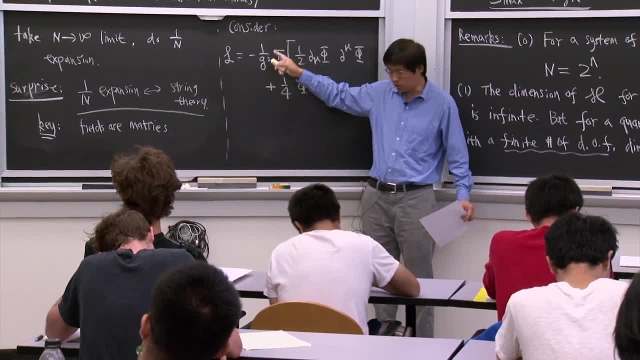 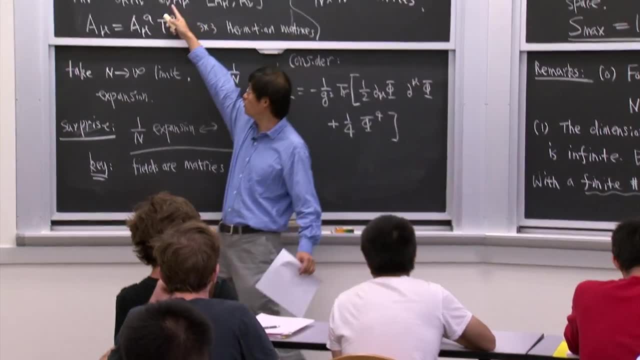 to put it in the front. Of course you can rescale it. I'm sure You can rescale it to put it here, which is a normal place, But I put it in the front, Just like what we normally do also for QCD. 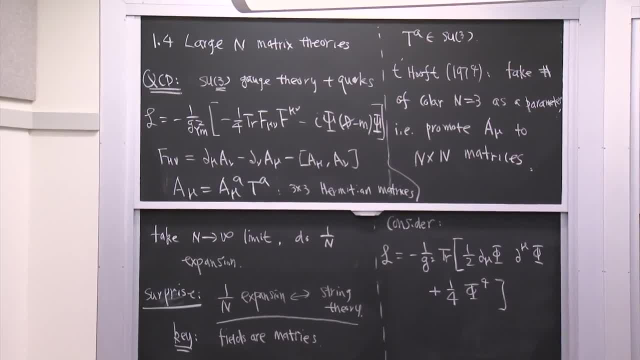 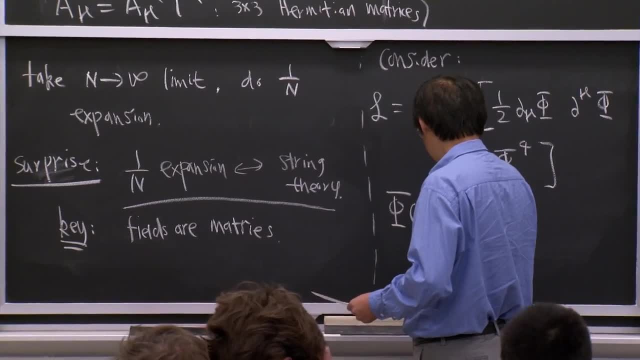 OK, So this G is a coupling constant which we put in the front, And then each phi. again, I take it to be a, n by n Hermitian matrix Phi x. each one is a matrix a- b. So I have two index. 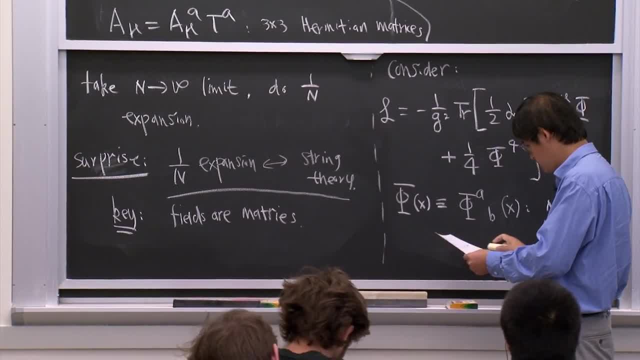 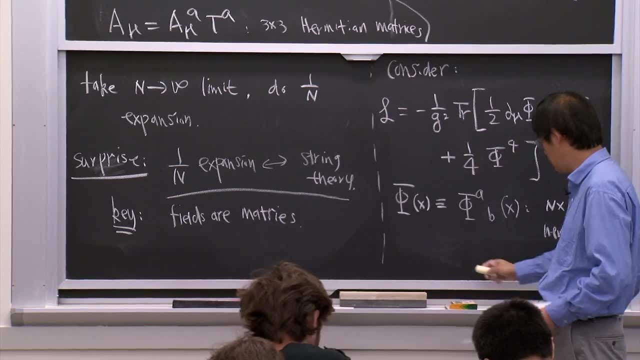 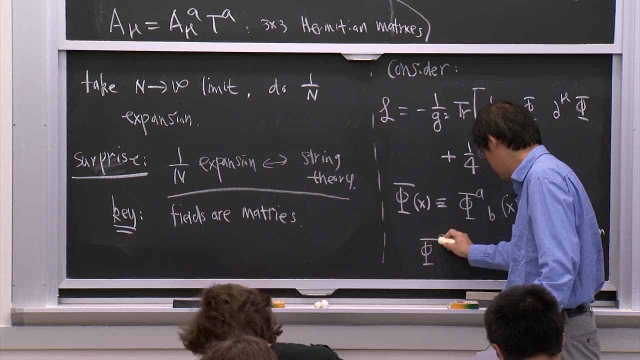 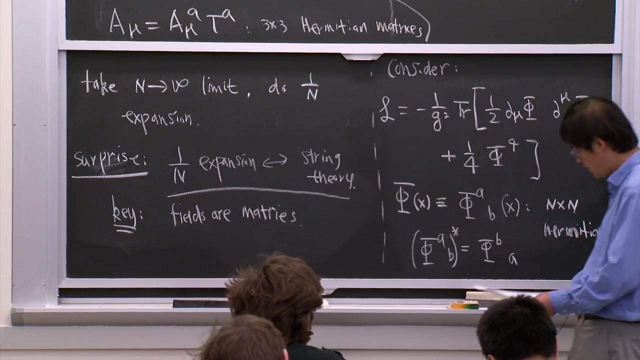 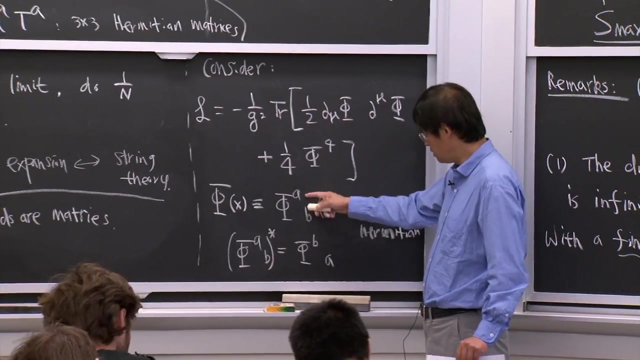 So this is n by n Hermitian matrix. Yeah, n by n Hermitian matrix. So which means that phi ab equal to star, equal to phi ba. OK, So there's a difference between the upper and lower indices, OK. 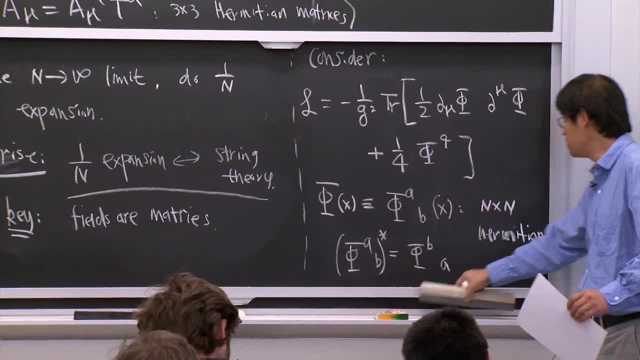 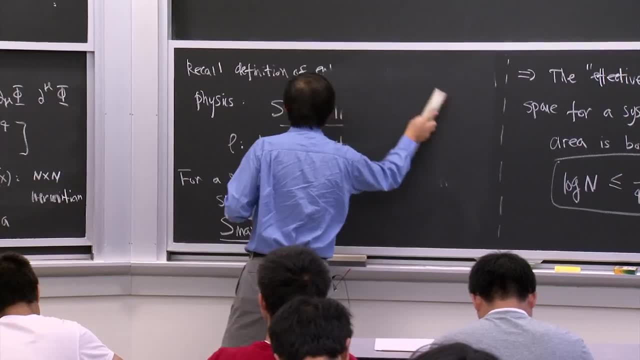 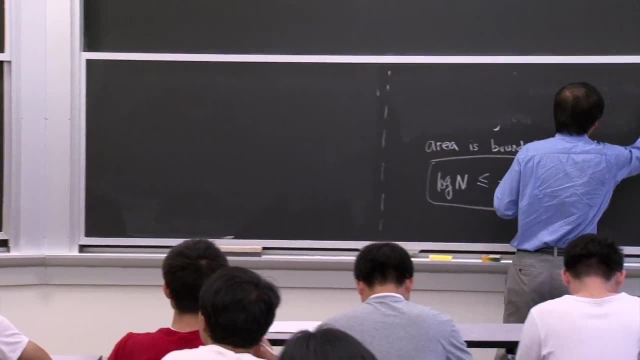 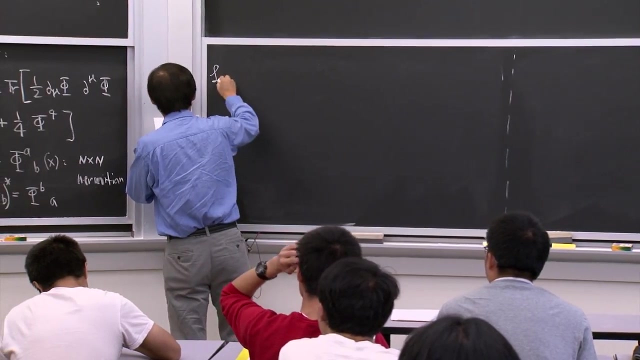 So I can write it more explicit in terms of components. So just to give you, in case some of you are not familiar with this kind of matrix kind of field theory, let me just also write it in terms of components. So writing it in terms of components, it's 1: half. 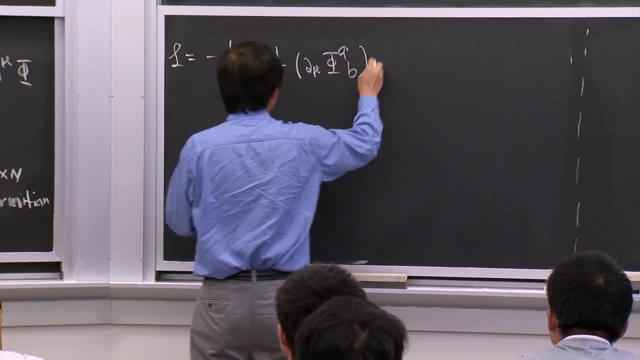 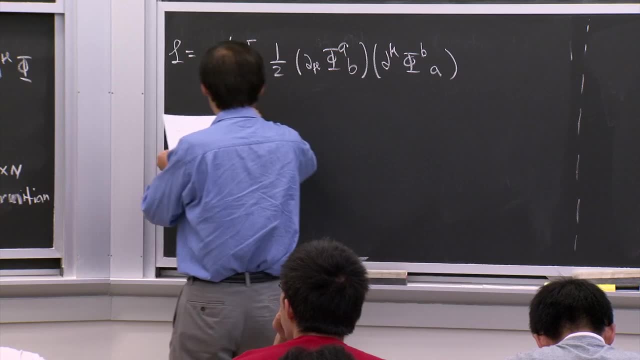 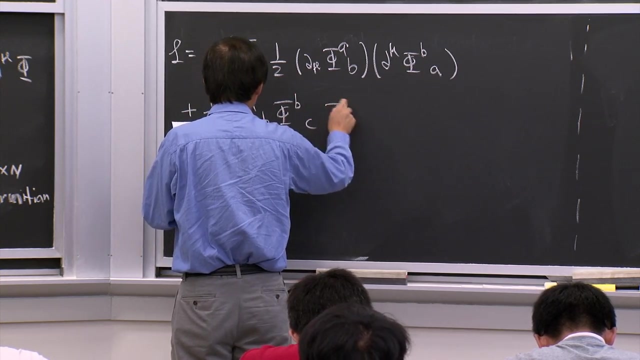 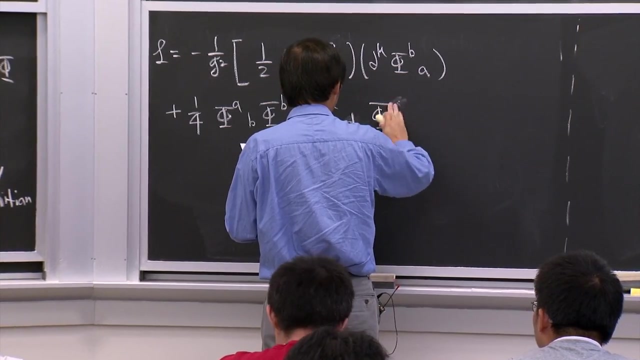 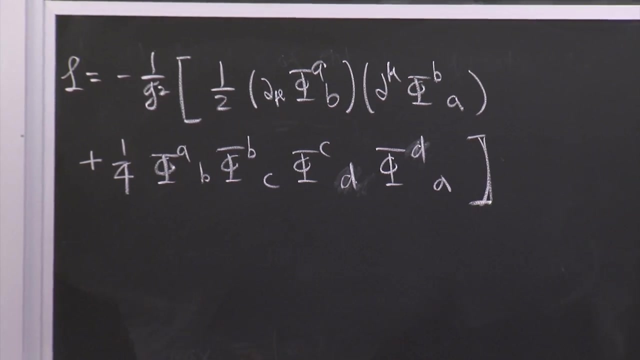 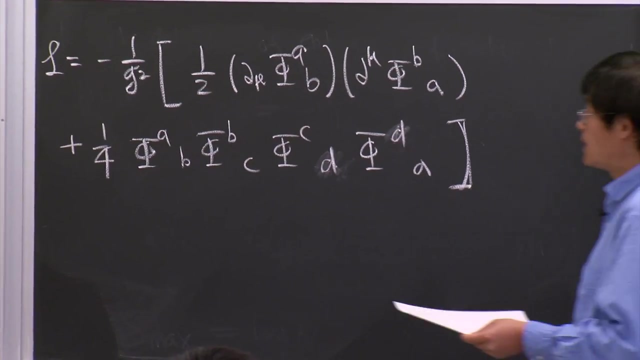 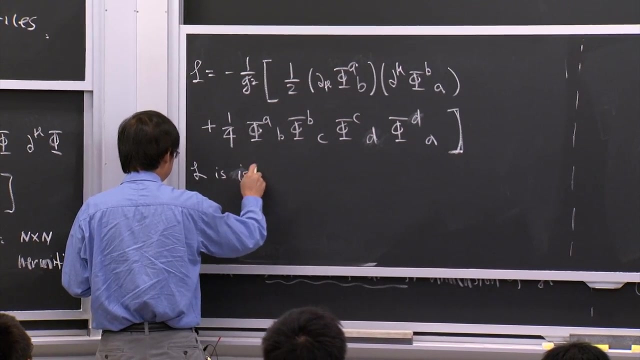 Partial mu phi ab, then partial mu phi ba, then plus 1 quarter phi ab, phi bc, phi ca, phi cd phi da. OK, OK, It's just having writing down the explicit union components. So this L by definition is invariant under. 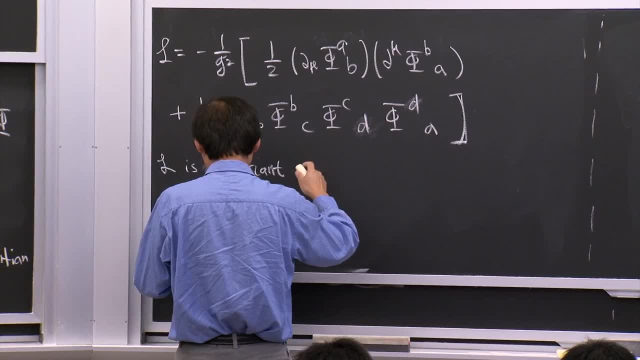 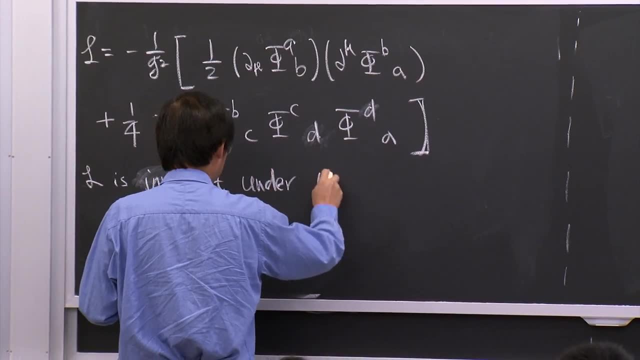 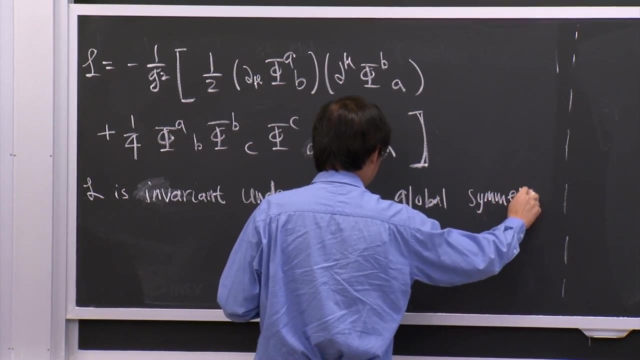 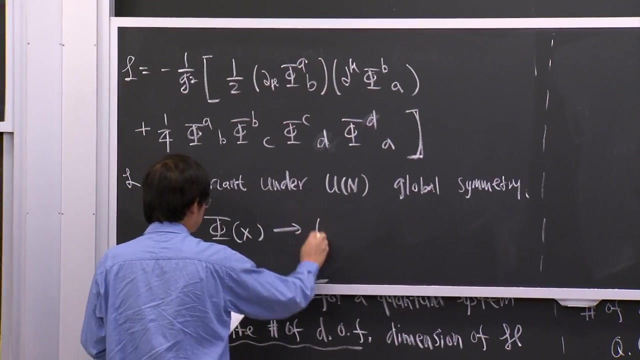 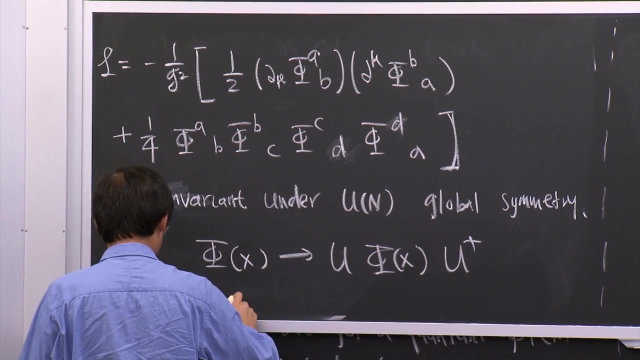 in addition to the usual translation, rotation, symmetries et cetera, has also internal symmetry. OK, It's under UN global symmetry. OK, So say phi x goes to u, phi x u dagger for any u. any constant is UN matrix. 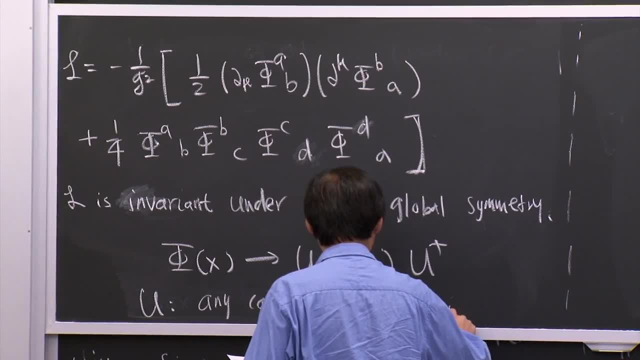 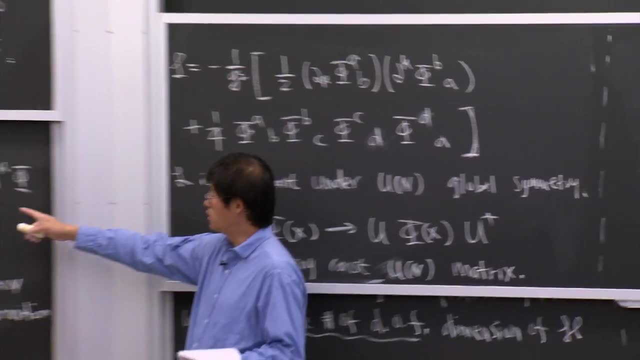 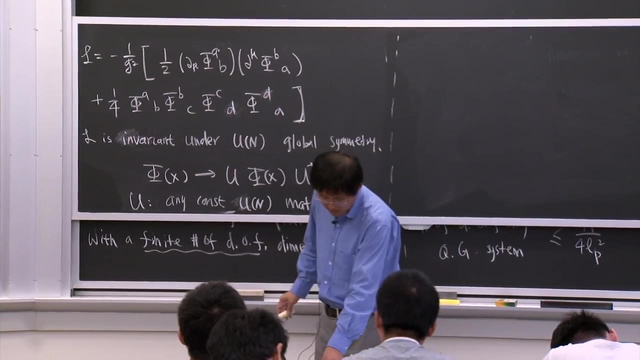 OK, So this series is invariant under: So this is obvious from here because of this trace. So this is invariant under this. OK, So let me just make some remarks before we proceed to talk about the features of this series. Let me just make some quick remarks. 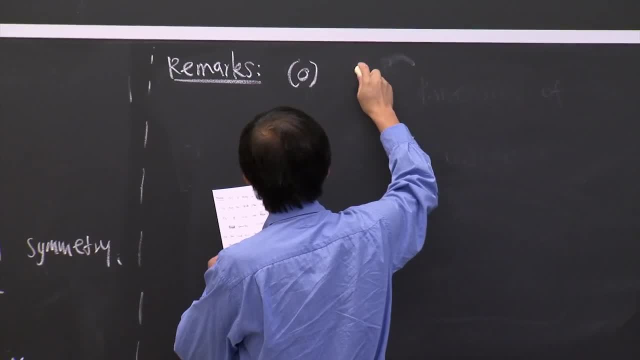 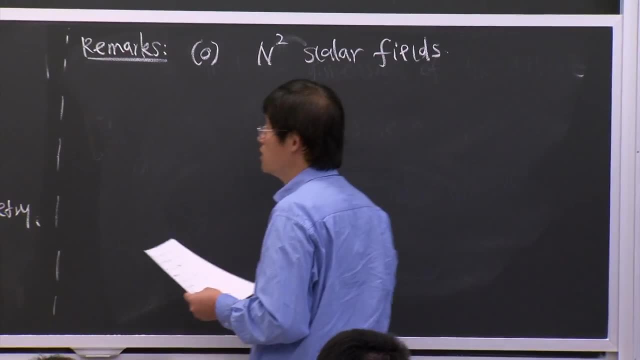 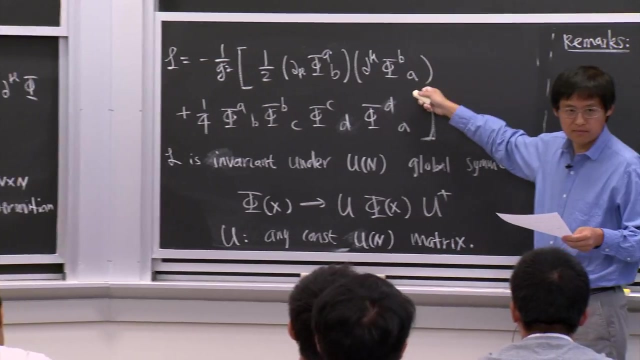 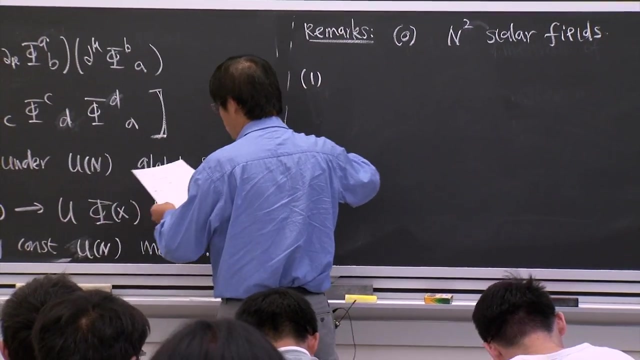 So this is 0.. You said this is a series of n squared scalar fields. OK, So if this is intuitive to you, then this just means you have many, many fields coupled together in some specific way. OK, And also we don't have to consider Hermitian matrices. 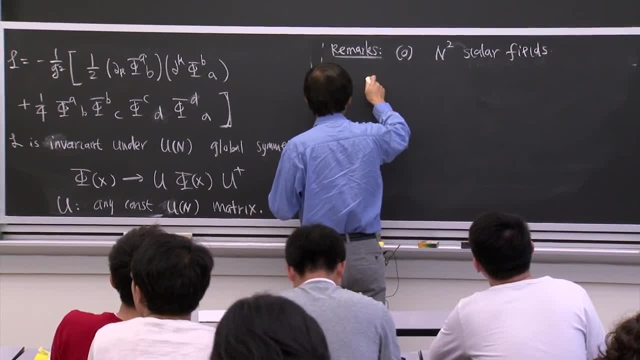 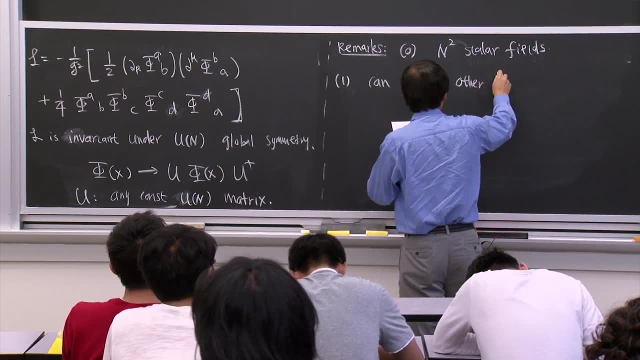 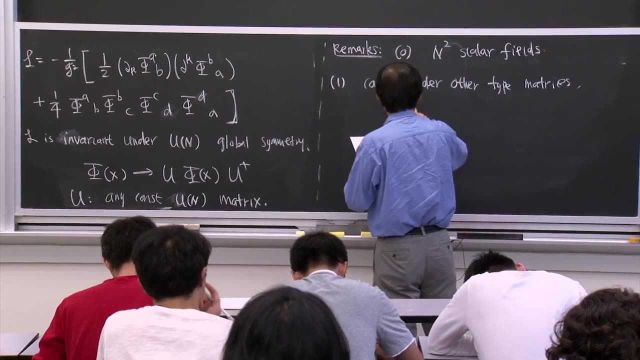 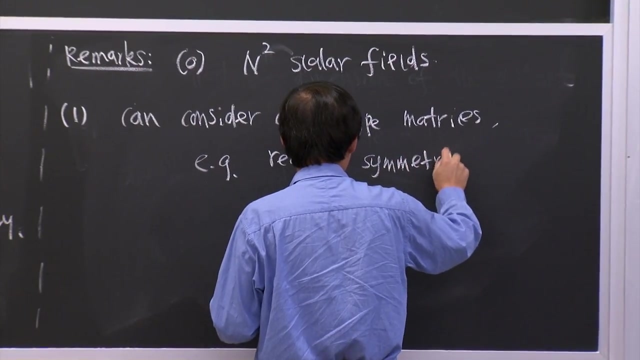 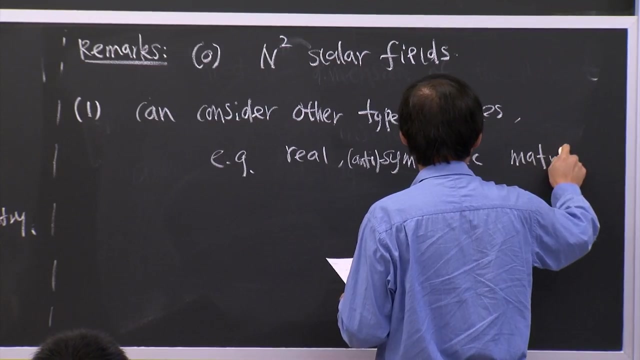 To consider Hermitian matrices, for simplicity one can also consider, One can consider other type of matrices, For example real, say symmetric matrices, Say real, symmetric or anti-symmetric matrices. So in those cases, If you consider, say, real matrices, 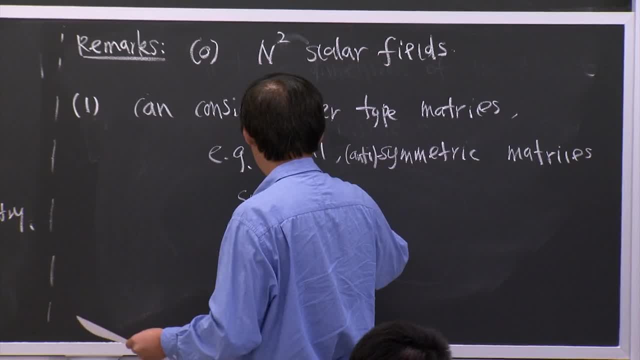 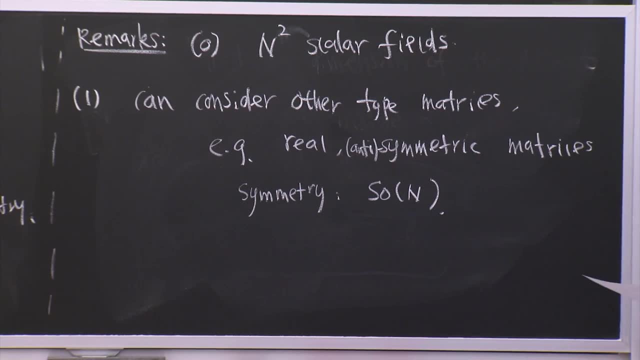 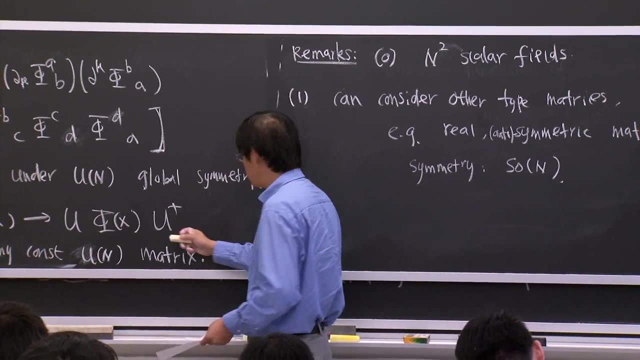 then symmetric or anti-symmetric matrices. In that case this global symmetry becomes S or n. OK, More than un. So in here this u is a global symmetry. Just u has become and cannot depend on x. You see it from here. 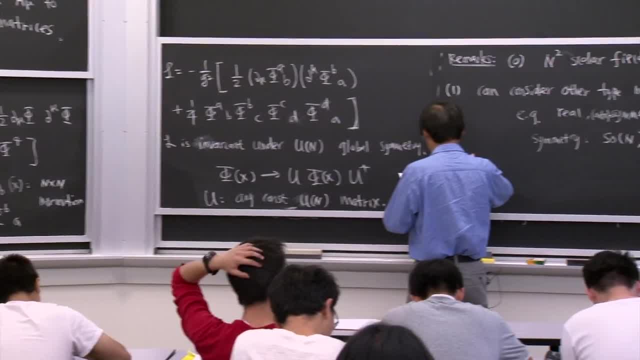 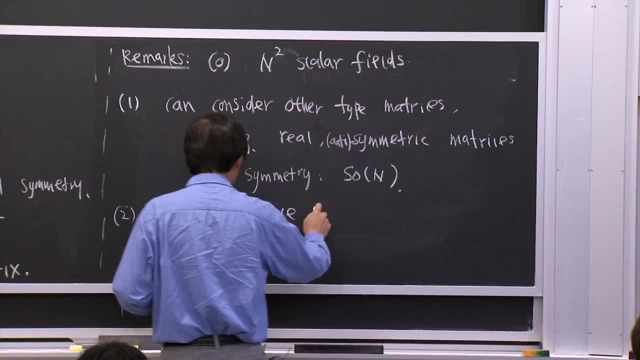 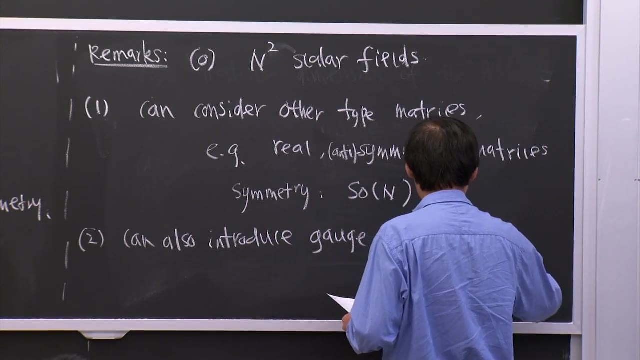 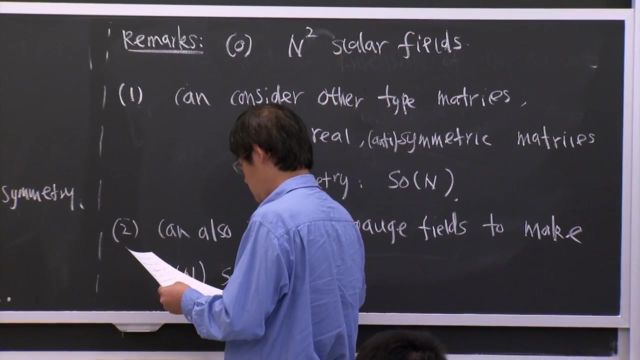 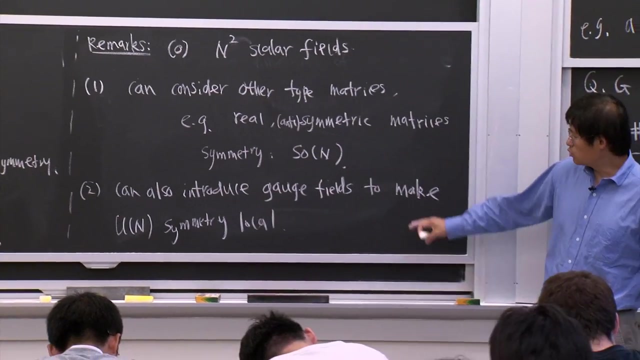 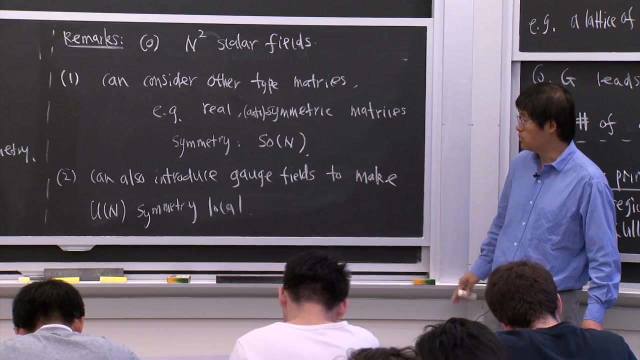 Cannot depend on x, But you can also. You can also introduce gauge fields to make this u n symmetry local. OK, So I will not do it now, but this will be important, OK, A little bit later. So later we will indeed make it into a local gauge symmetry. 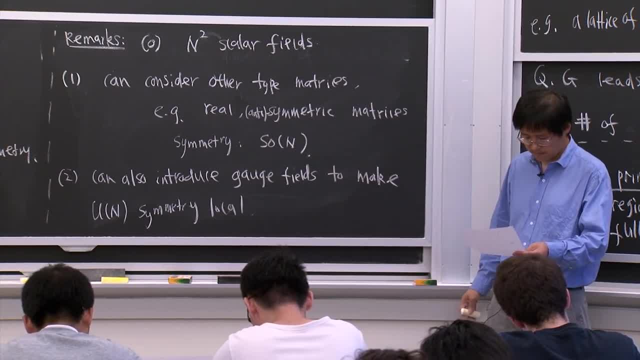 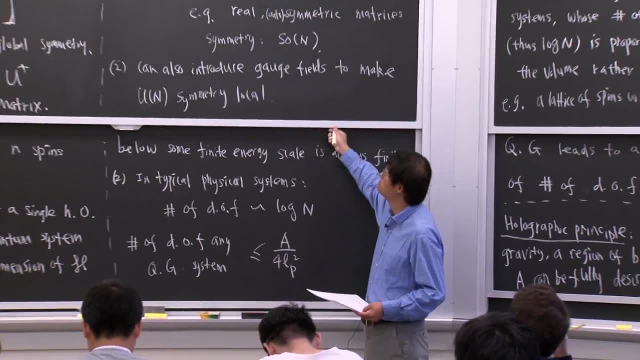 But for now let me just consider this simple example. OK, Because I don't want to introduce too many fields et cetera. So any questions regarding the set up of this theory? Yes, Can you explain the last point one more time? 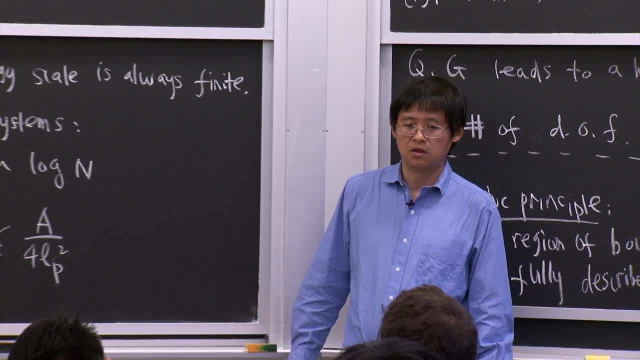 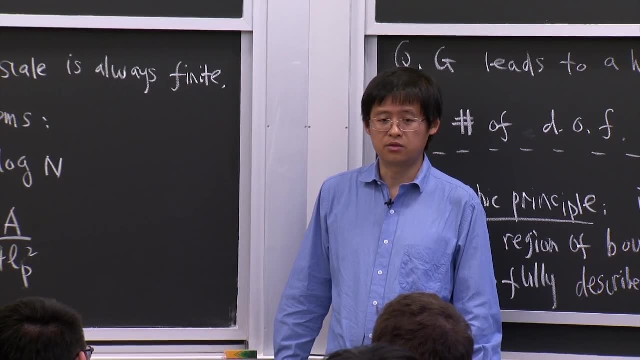 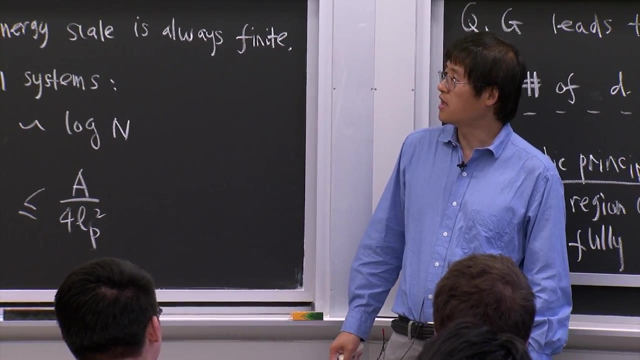 So what do you mean that? if you, How does introducing gauge fields make the symmetry local? Um Yeah, You have to take 8,, 3,, 2,, 4 to know that, But the simple way to explain it, yeah. 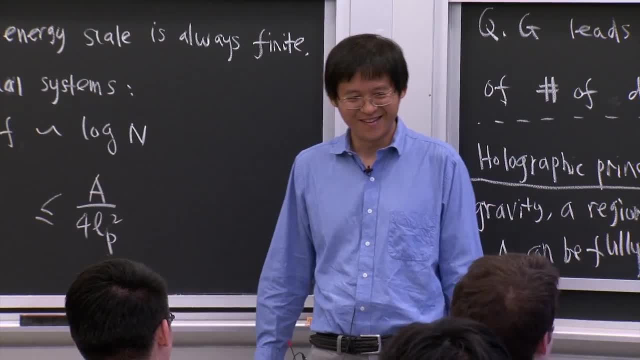 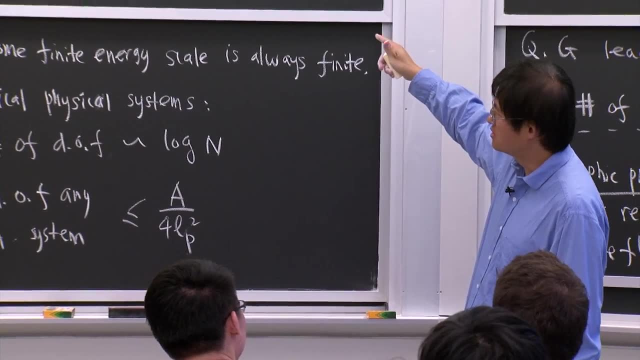 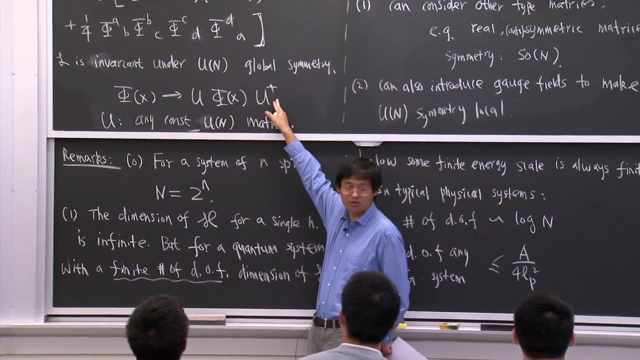 there's no simple way to explain it. Yeah, Yeah, Just say: let me just explain the statement. If you introduce some gauge fields, then you can make this u to be some arbitrary function of x rather than a constant. So that's the statement of a local. 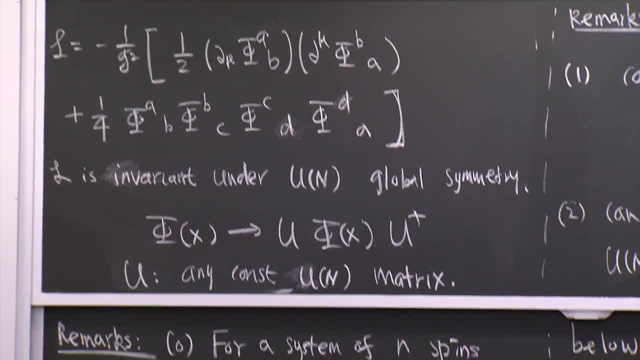 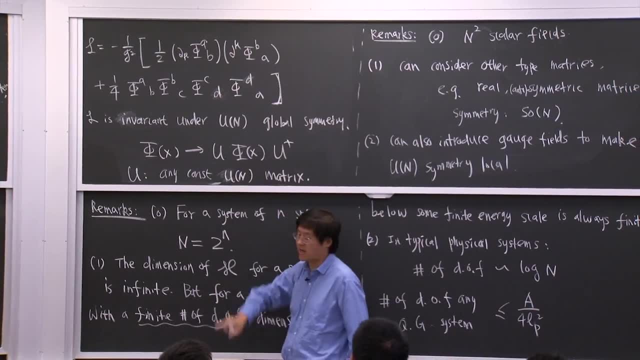 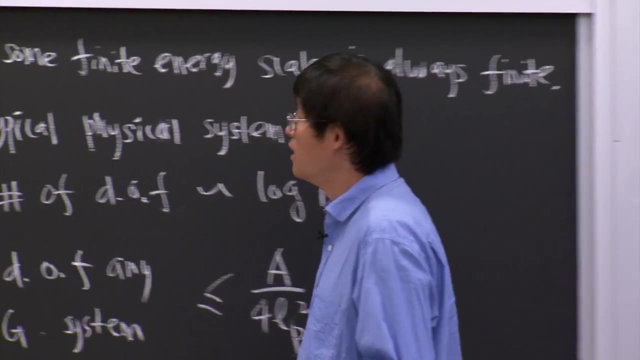 Yeah, Yeah, I just say I can generalize this theory so that this symmetry become a local, become a symmetry, so that u can have arbitrary x dependence, can have arbitrary space-time dependence. So right now u must be a constant. 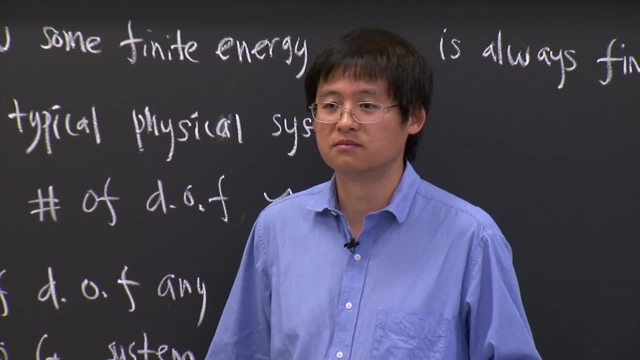 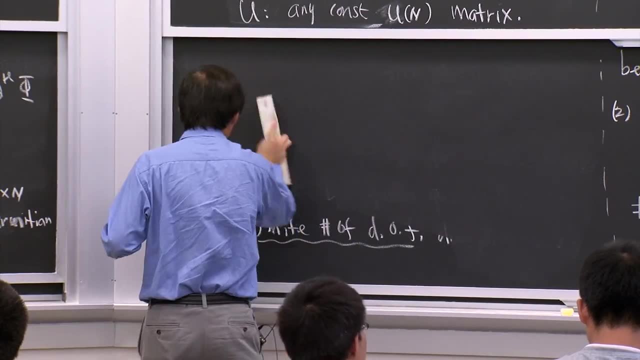 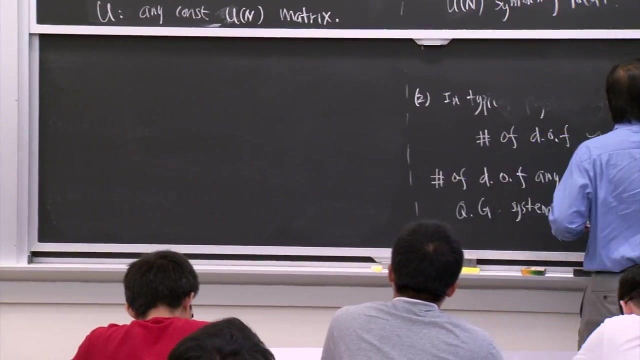 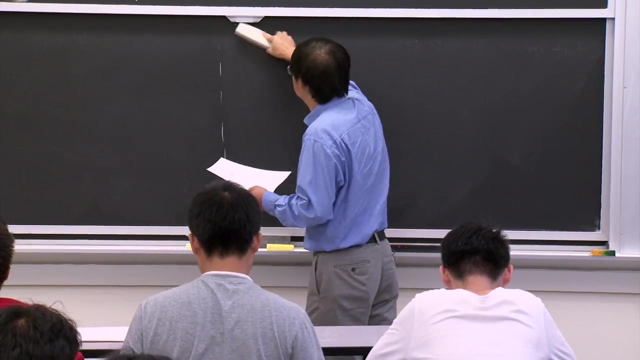 Any other questions? Good, OK, So now let's just try to do perturbation theory. Think g squared small. Try to do perturbation theory, OK. So the first thing you do, of course, is to write down the Feynman rules. 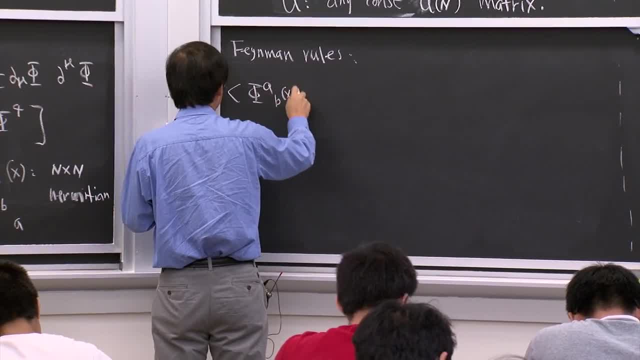 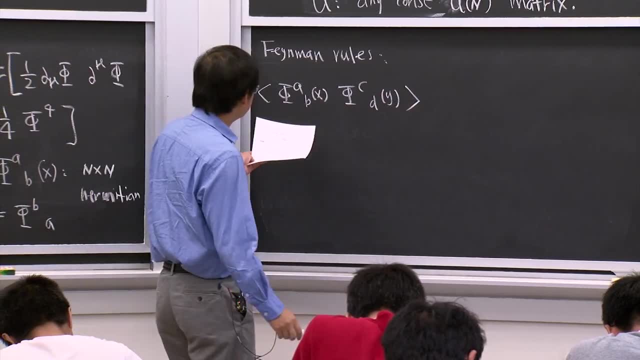 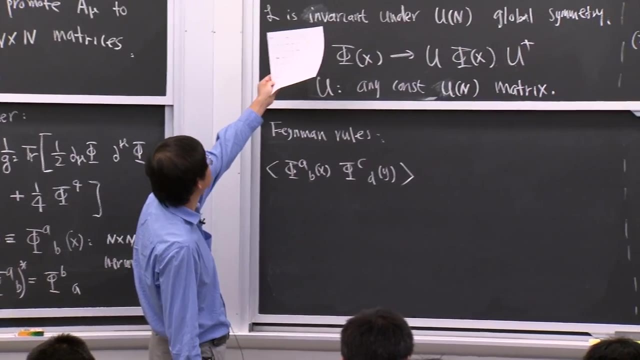 Say: first you have to look at the propagator. OK, look at the propagator, So you can. essentially you are all field theory experts, So just by looking at that Lagrangian then you can immediately write down this propagator. 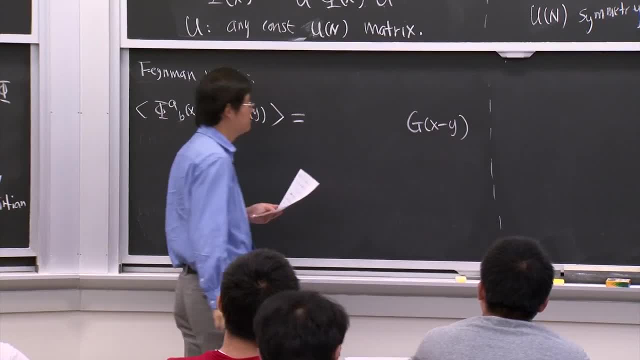 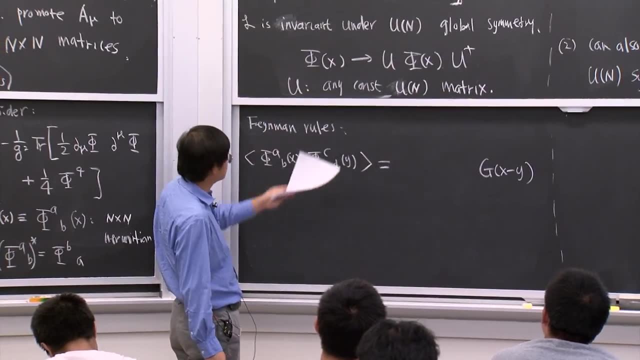 We can just write down x minus y, OK. So whatever propagator, Whatever space-time dependence, Let me just call it x minus y. But also there's a non-trivial index structure. First. there's also g squared, OK. 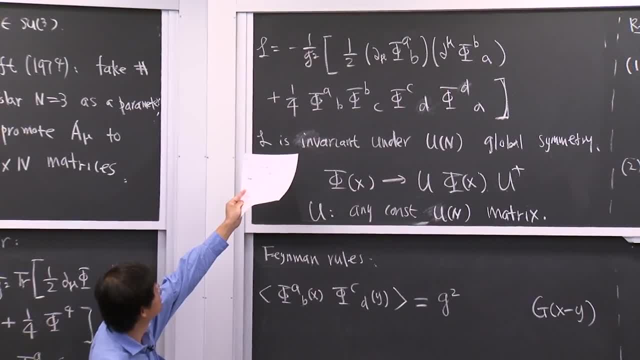 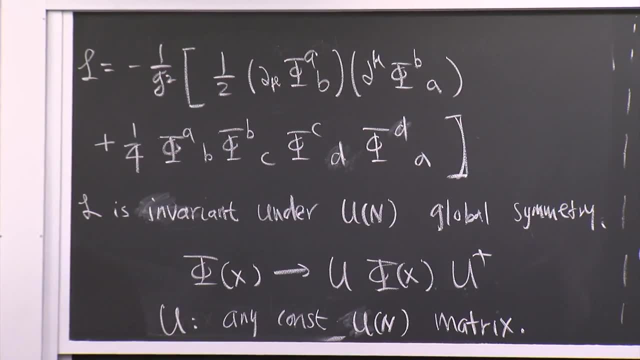 Because there's a prefactor 1 over g squared. So when you invert the kinetic term, there's a, g squared. And about the index structure, you said a, b, b, a, So that a must contract with d and b must be the same as c. 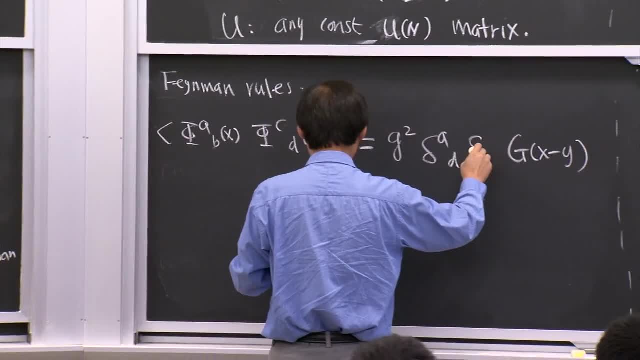 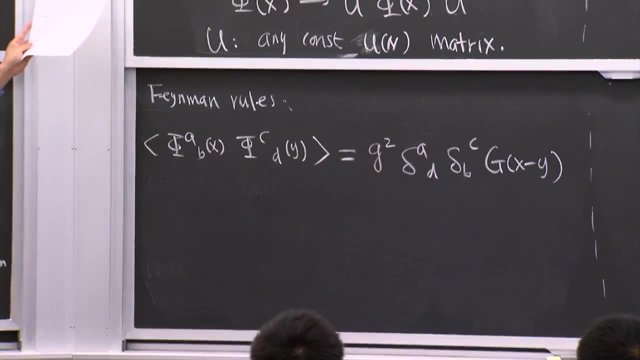 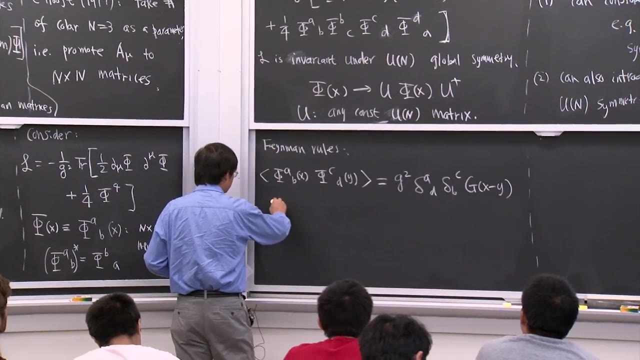 So that means you have delta ad: OK, OK, OK OK. And the delta cb, bc OK, Because in the Lagrangian only those fields are paired, So the propagator must have this structure. So similarly we can write down the: 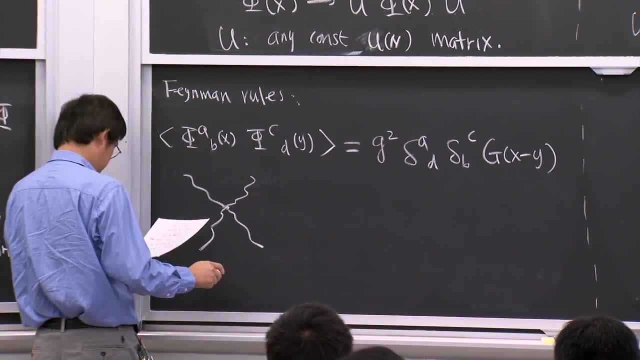 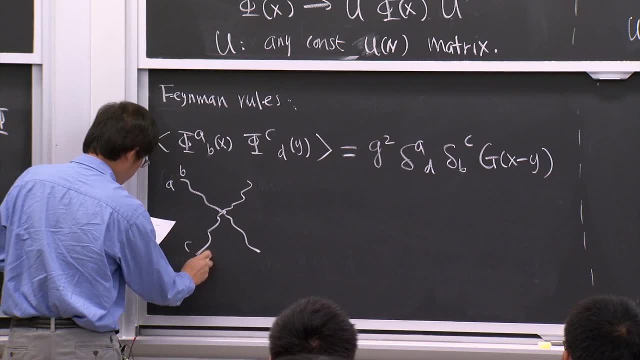 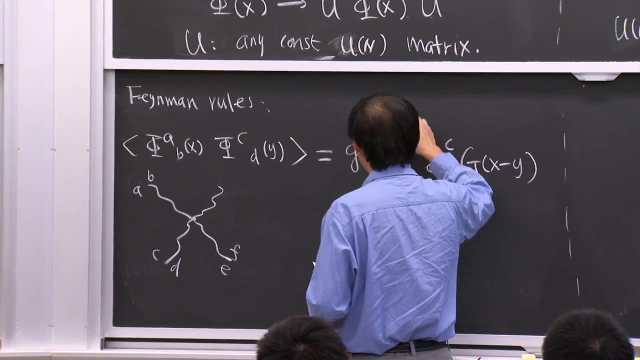 so there's four particle interaction vertex, So each particle have two index. So this is ab, cd, ef. Oh yeah, Right, Sorry, Let me add one more And then I can denote this diagrammatically just as ab cd. 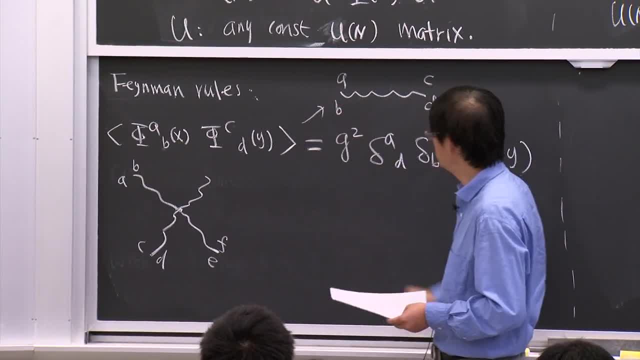 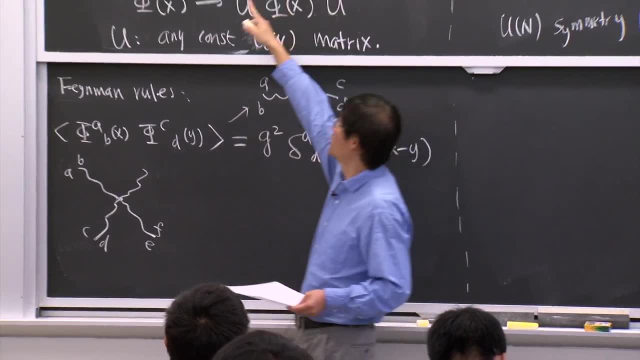 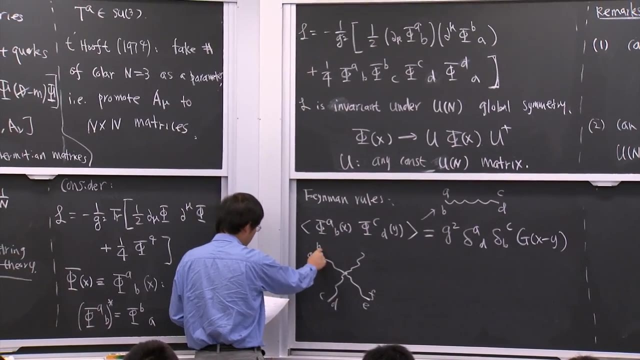 OK, Just denote this diagrammatically as the propagator, which is where we land: ab, cd. OK, And now also we have this quartic interaction vertices which involve in four fields. So each field have two index because ab. so ab, cd, ef, g, b. 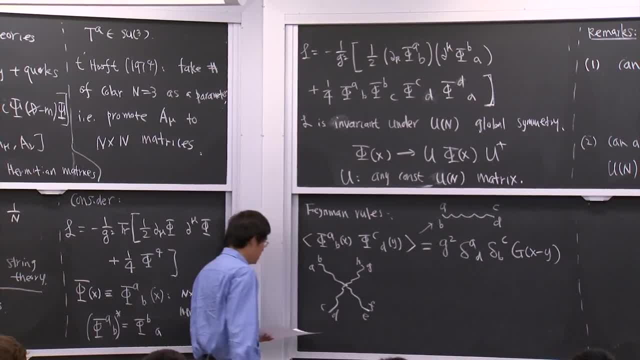 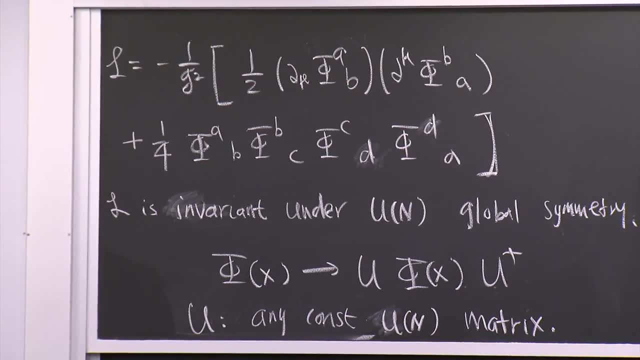 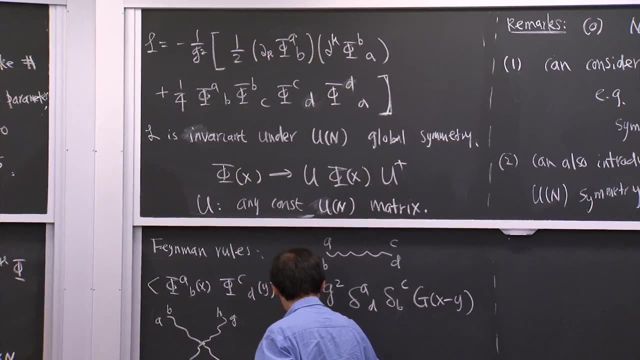 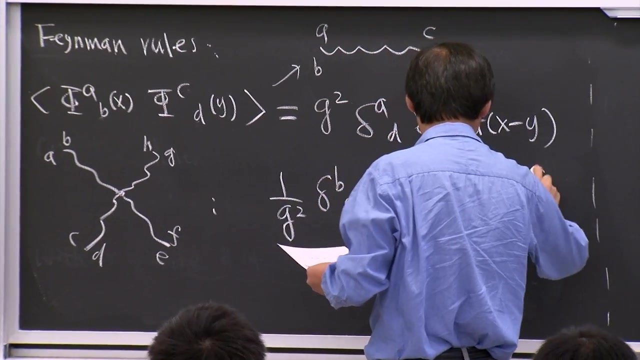 f, gh. But this is not arbitrary interaction. They have contracted In the interaction, they contract in a specific way. So you get 1 over g squared because of all factors g squared And then you have delta, bc, delta de, delta, fg, delta ha. 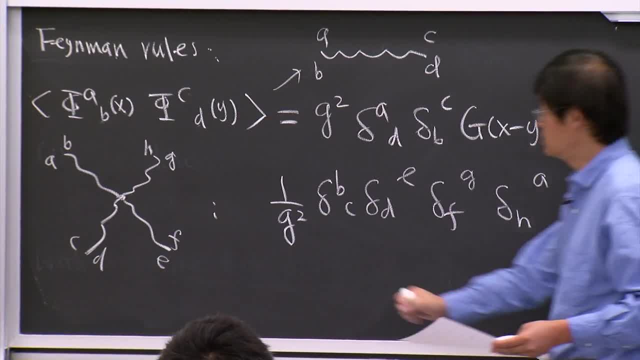 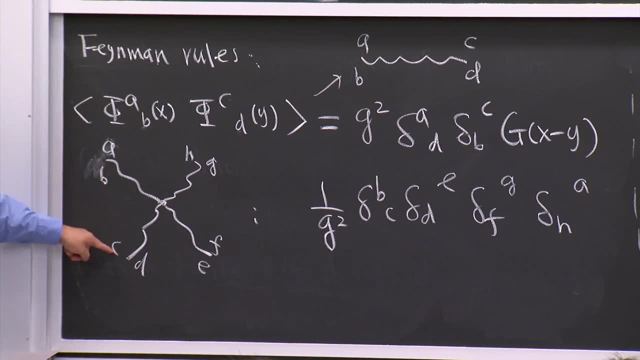 OK, Because they have to be contracted. OK, It's better, right, It's better to write it as ab this way, ab OK. So ab. b contracted with c. d contracted with e. e contracted with g. h contracted with a. 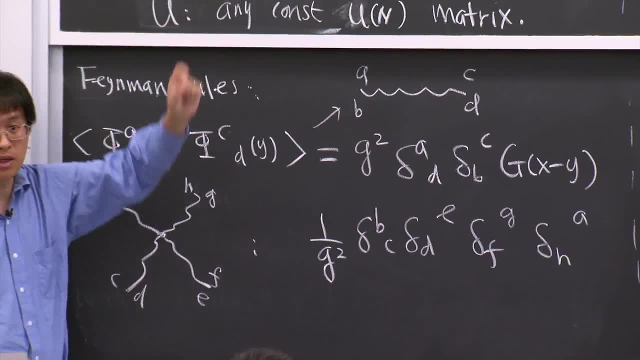 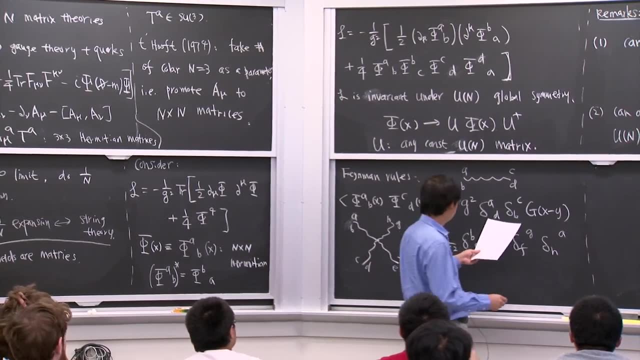 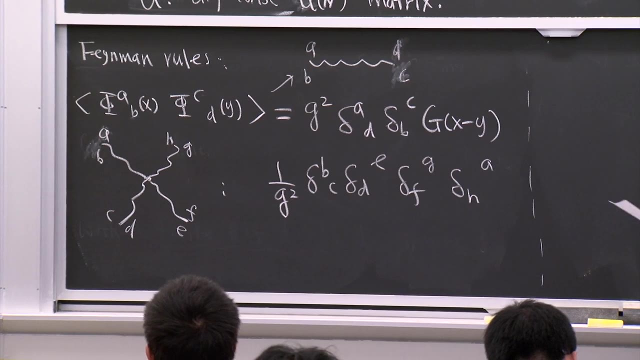 So this gives you a matrix product. So just like that. OK, So the propagator exchanges a and b, Hm ab contract with d. Yeah, let me just call dc, That's right. OK, So this is a Feynman rule. 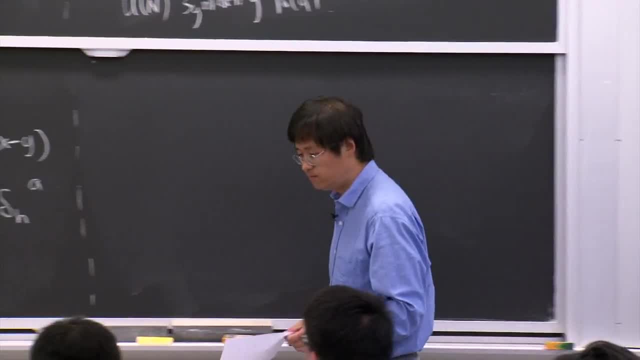 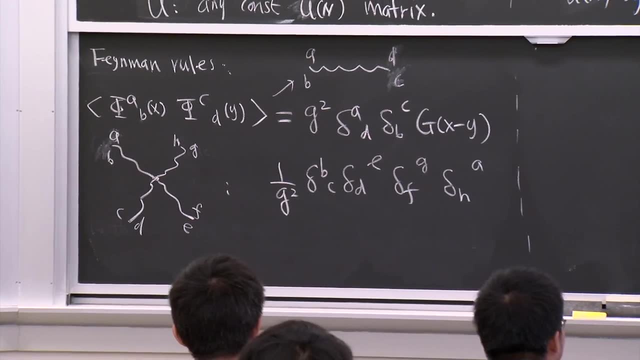 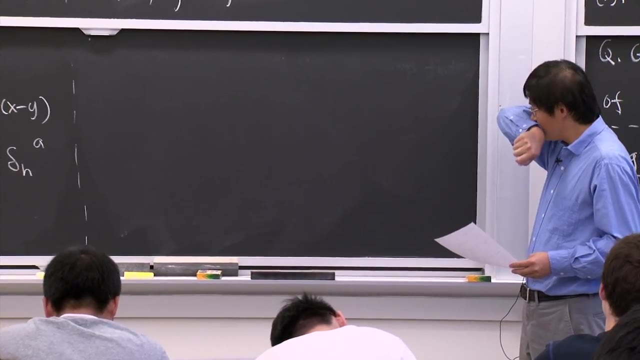 So now you can start calculating. OK, So if you have calculated this for a while, then you find this is a little bit tedious With all these indices. it's quite annoying, And but was a smart funnel. So you say, let me find a way so that I 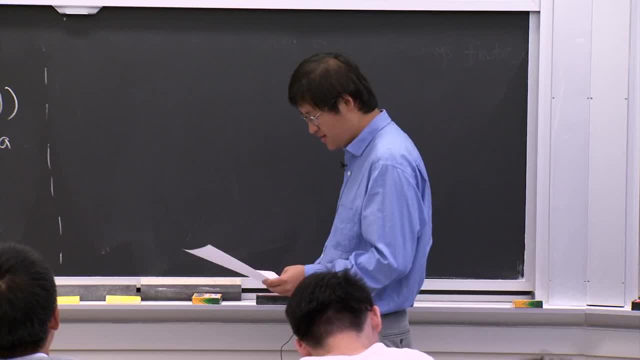 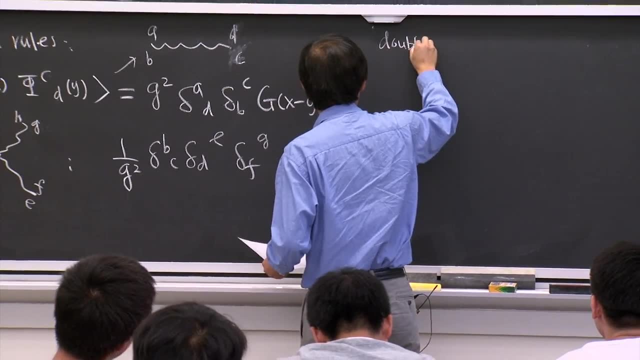 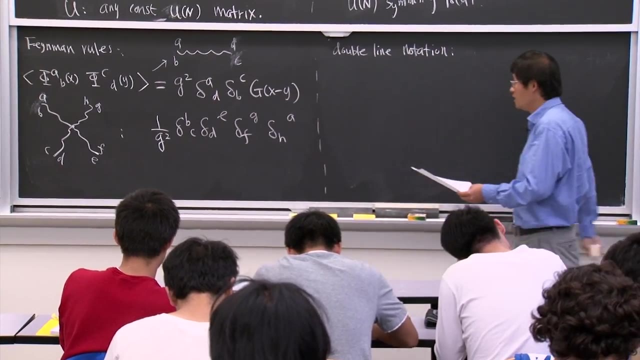 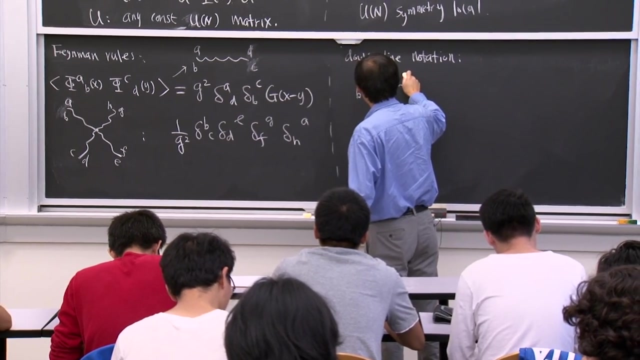 don't have to keep track of all these indices. OK, Then he invented a very nice way, So this is called double line notation. So first this propagator, ab, c, d, since that a is contracted with c, c is contracted with b. 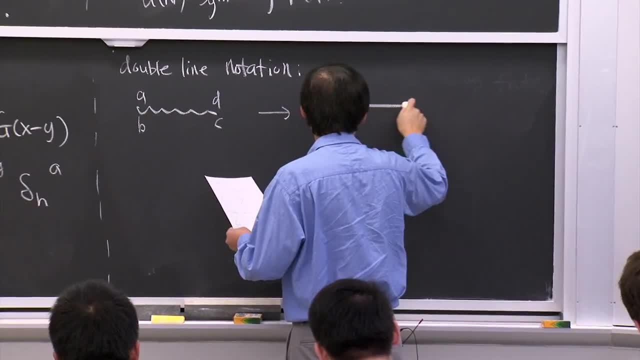 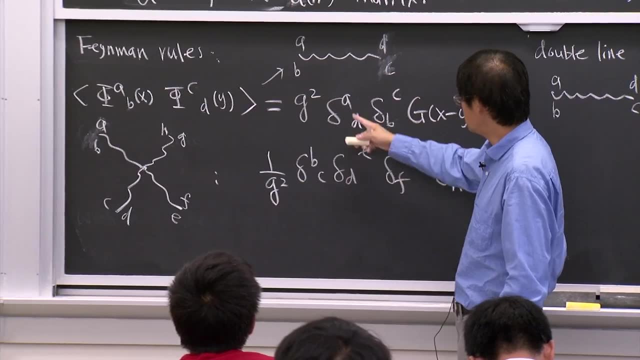 separately. he said: let's just write it as a double line, OK, But since there's a difference between the upper and the lower indices, so let's define a direction for this double line. So this should be go. so let's define the direction. 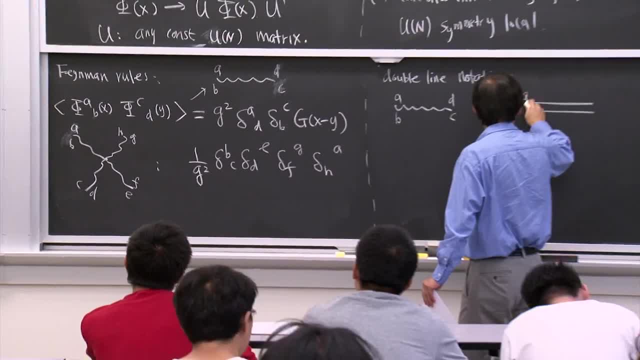 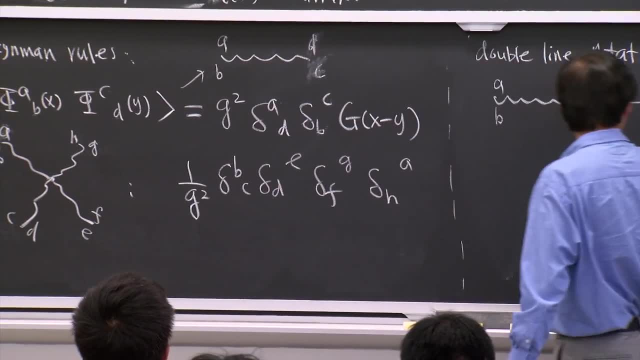 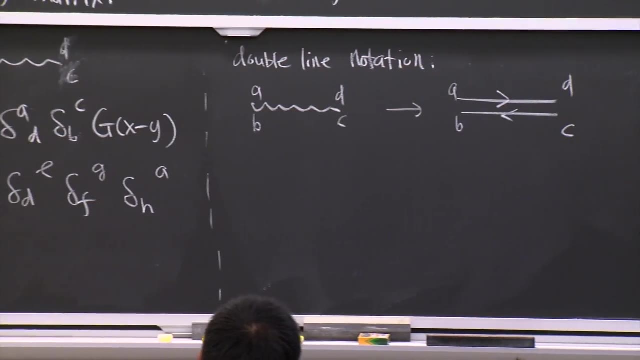 to go from the upper index to the lower index. Then you will have ab, then you have d, then c, b- OK, Because for c it's upper to lower index. You go from c, d- OK. So now you don't have to worry about this contraction. 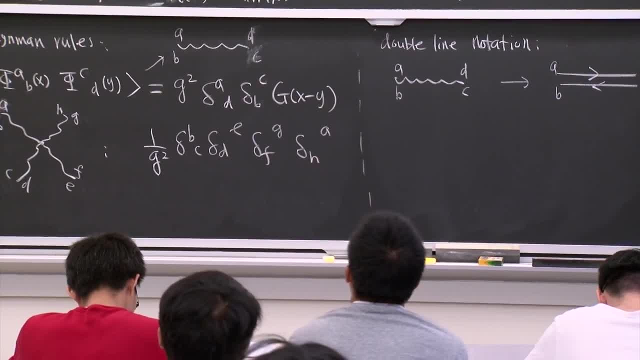 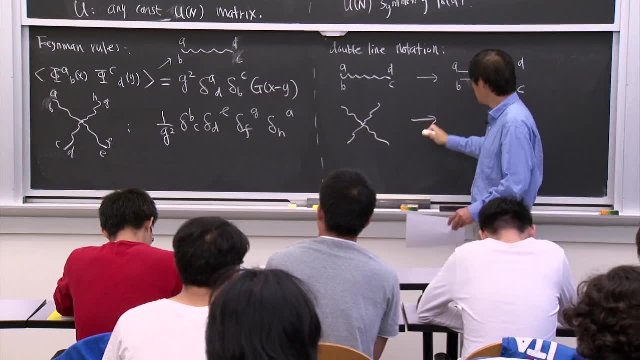 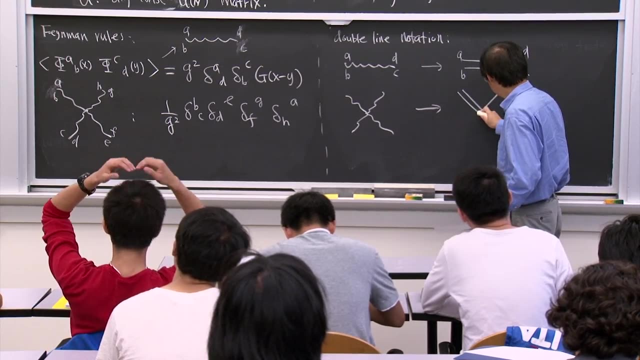 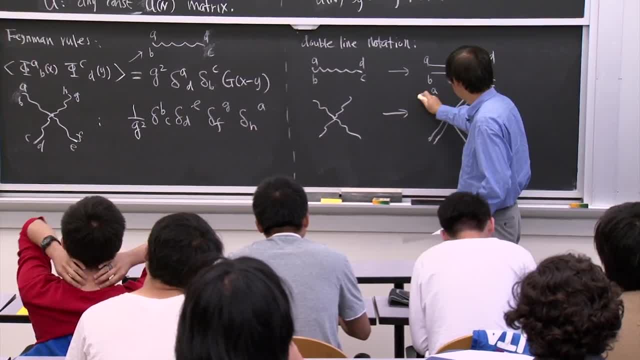 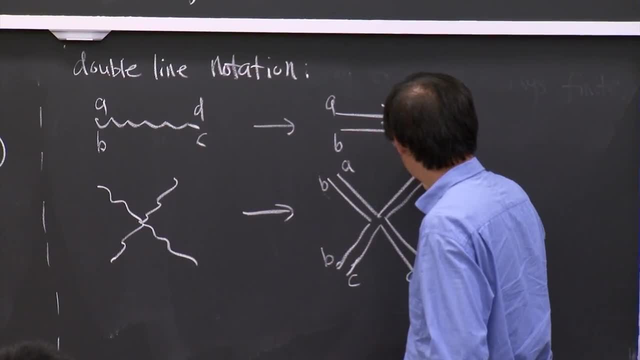 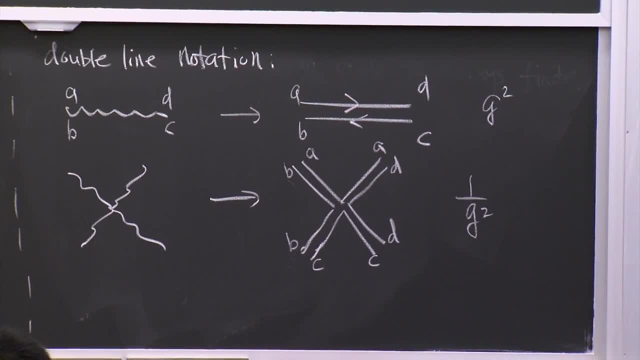 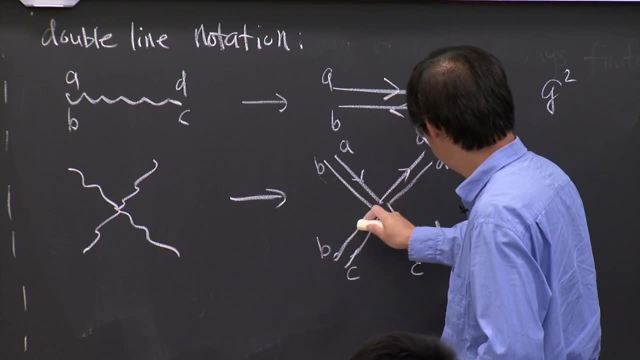 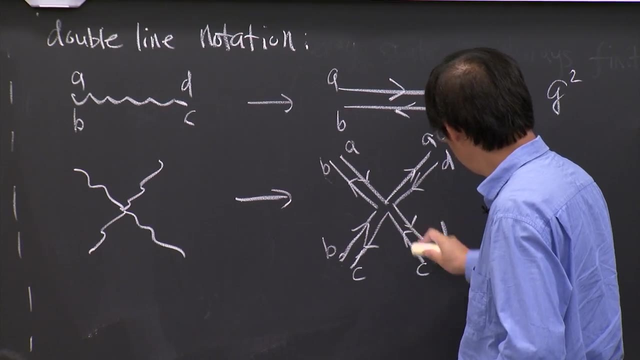 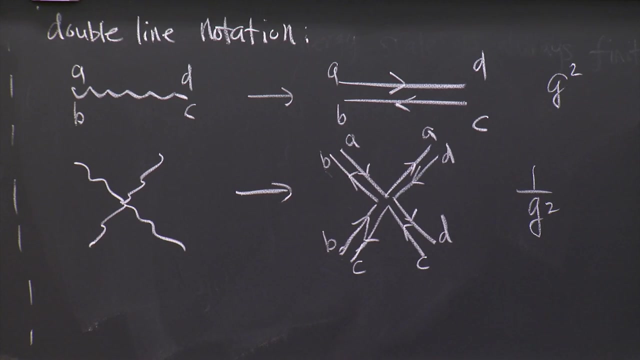 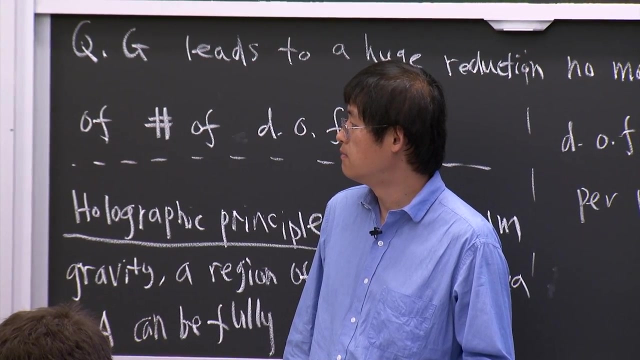 Here you have g squared, OK, So once you draw the double line notation, so let me also draw the arrow. Once you have a double line notation, then all those lowing deltas, they're automatically taken care of. OK, On the left left side is really delta c, d. 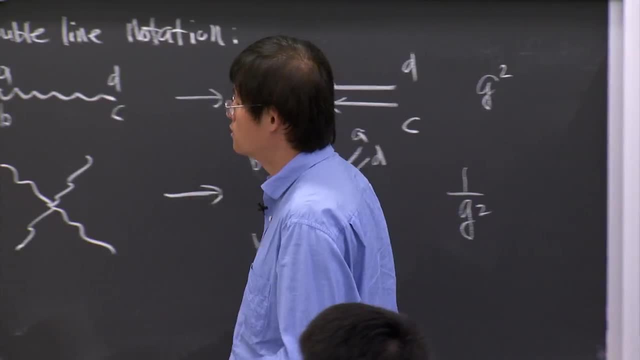 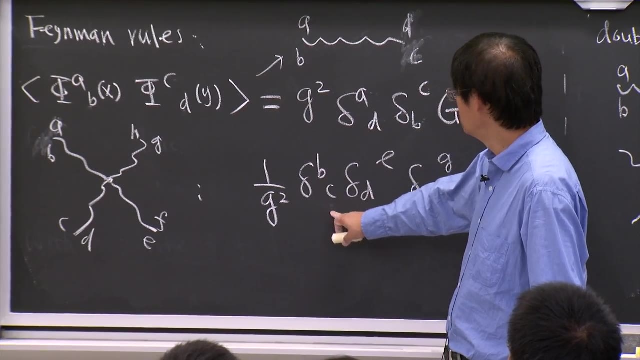 d is on the top of e. Sorry, which one? Delta f. yes, there's four vertices Here. Yeah, c is on the top Delta. Yeah, if you write it. Oh, OK, Delta bc. that's right. 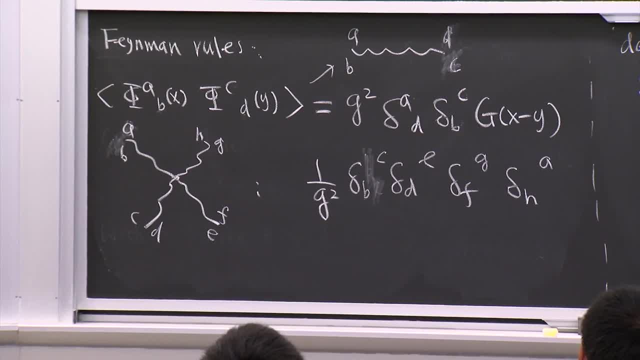 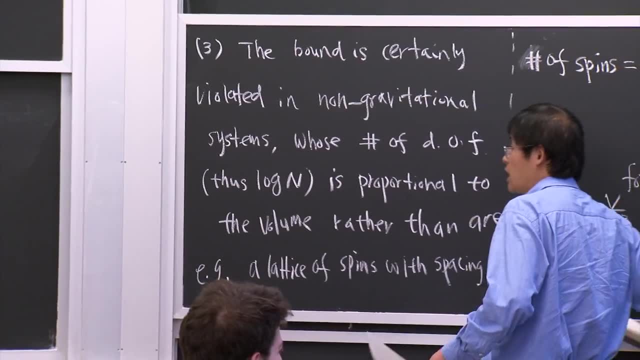 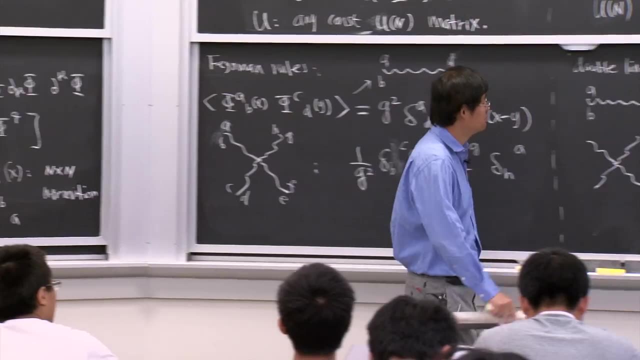 Good, Good, Good. So now let us give you some examples of using this diagram to calculate things, And also try to calculate the independence, Because you need to. Eventually, we want to take a large n limit, OK, So we want to keep track of the independence. 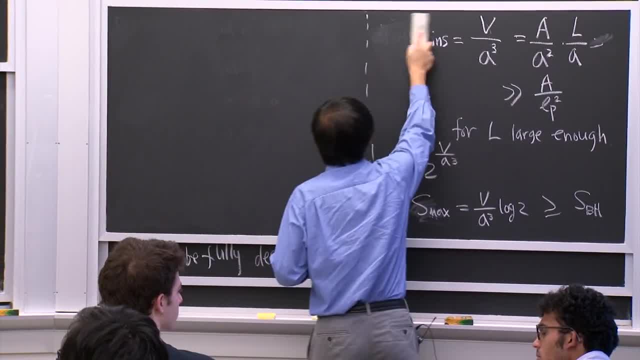 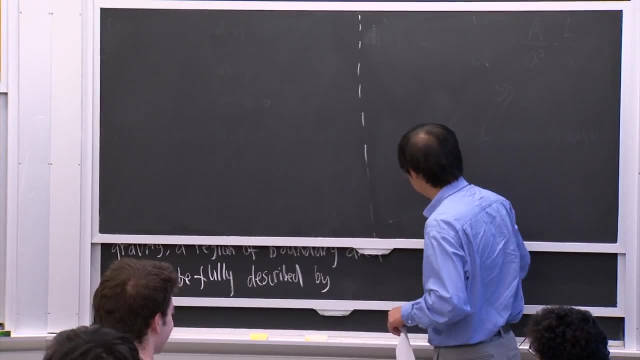 Yes, The four-point coupling. does that come from the commutator in the f menu on the gauge here? No, I just wrote it down by myself. OK, so it's an additional thing. Yeah, Yeah, it's actually. yeah, just arbitrary field theory. 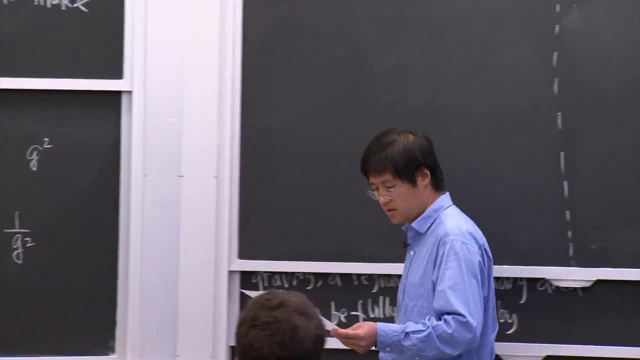 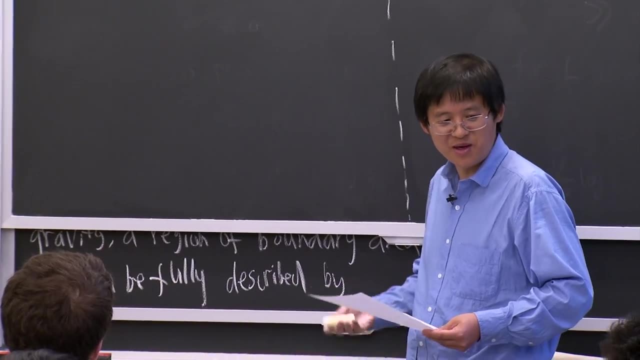 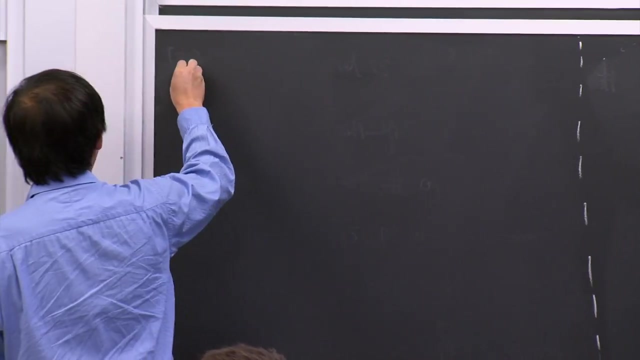 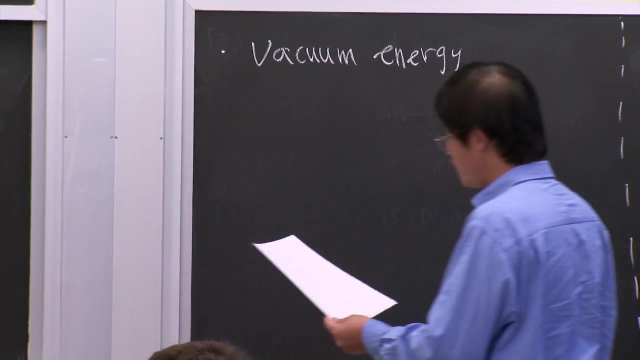 Yeah, Just an example. OK, so now let's start calculating. You already have the Feynman rule. what to wait for? So let's just calculate. So the first thing. let's look at the vacuum energy. OK, so that's the first thing to calculate. 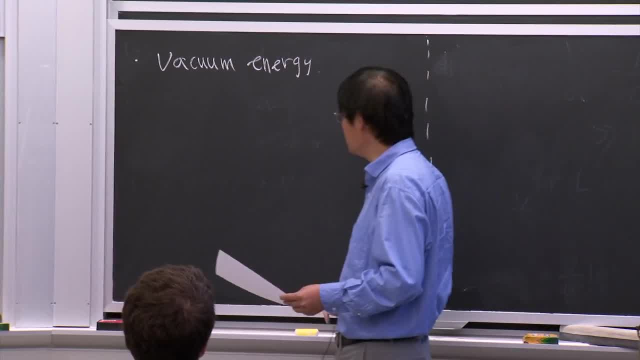 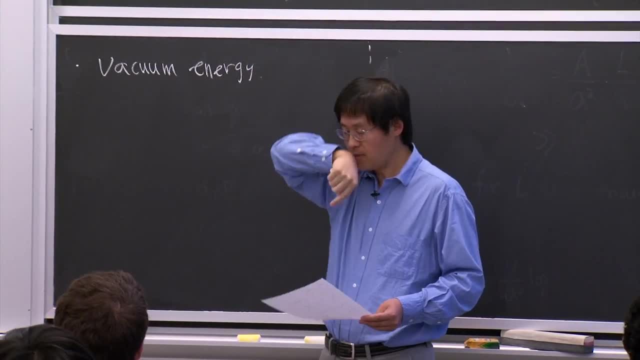 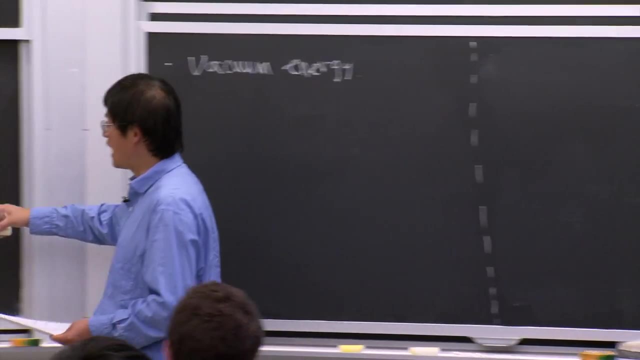 So what's the vacuum energy? Yeah, Yeah, Yeah, Yeah, Yeah, Yeah. So the diagrams. it's a summation of all the diagrams without external lags. OK, Yeah, let's just so. the simplest diagram is just with one vertex. 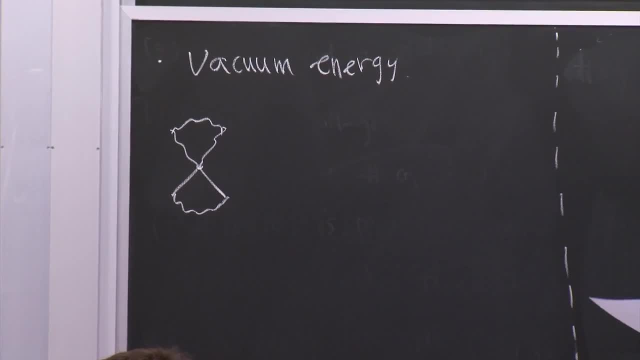 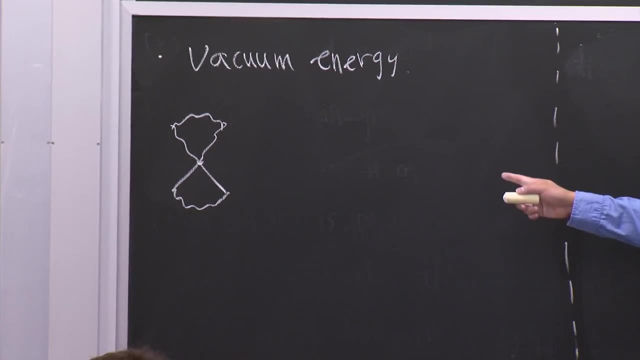 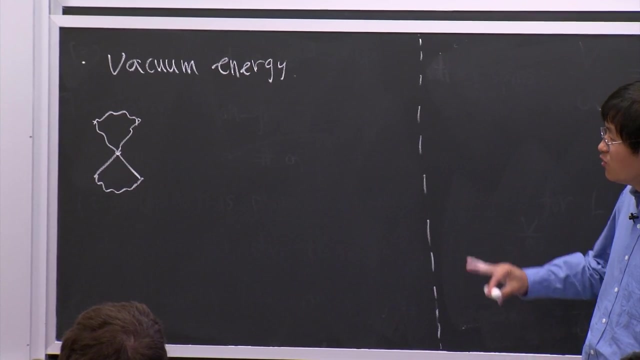 OK, So this is the simplest diagram. But now. so if you do lambda phi 4 theory, then that will be the end of the story. OK, You just contract with them. But now the matrix, because we are contracting matrices. OK, 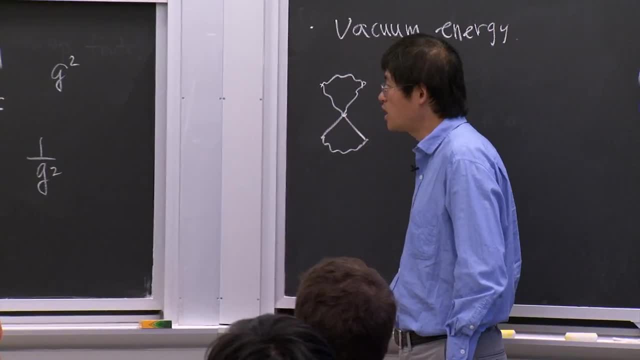 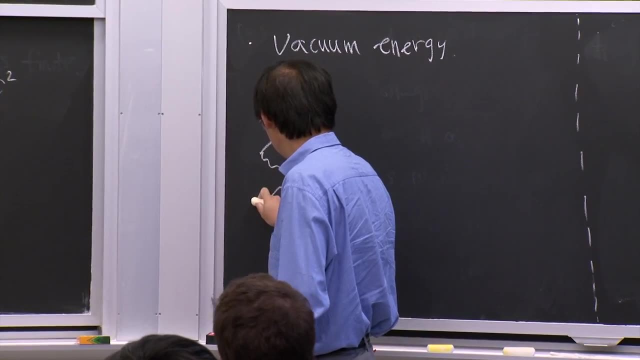 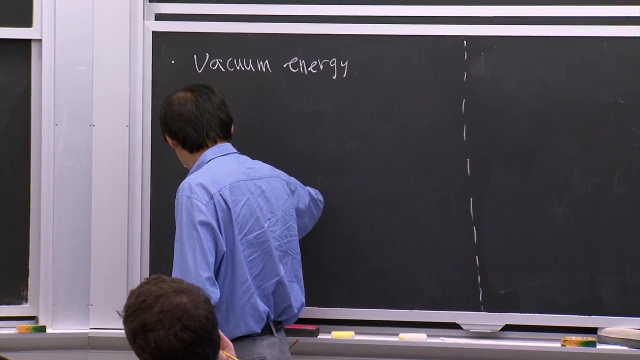 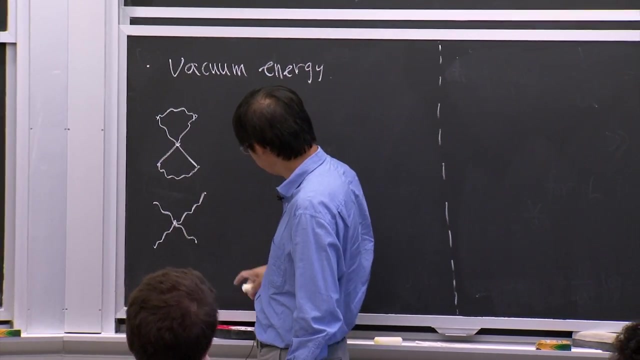 So this is like contracting to four matrices: We're contracting matrices, but matrices don't commute. So actually there's a difference. So you should convince yourself. There's a difference which I actually connect these two, from which I connect these two and these two. 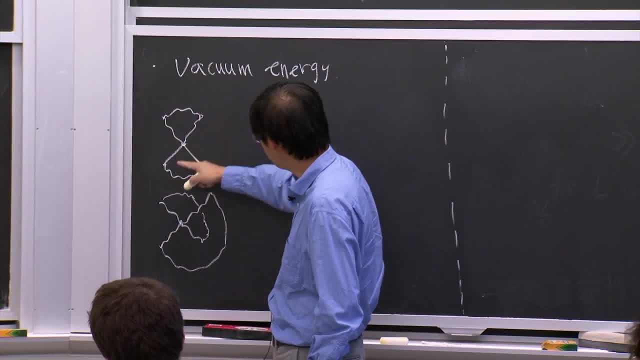 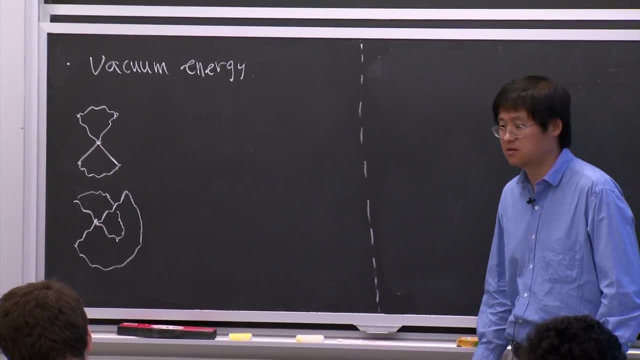 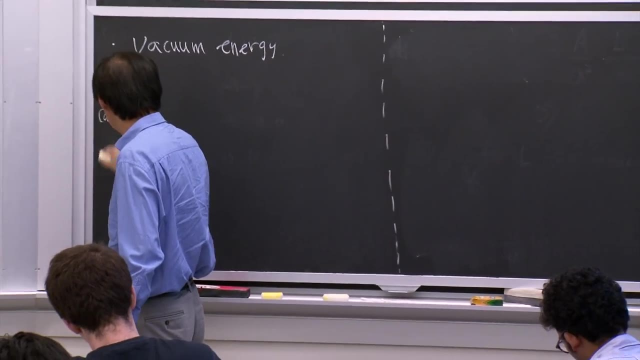 OK, Because this corresponding to: I connect the labeling ones And this one, I connect the diagonal ones And the order actually matters. OK, The order actually matters. It matters Because matrices don't commute. So if I call this a and b, then a not equal to b. 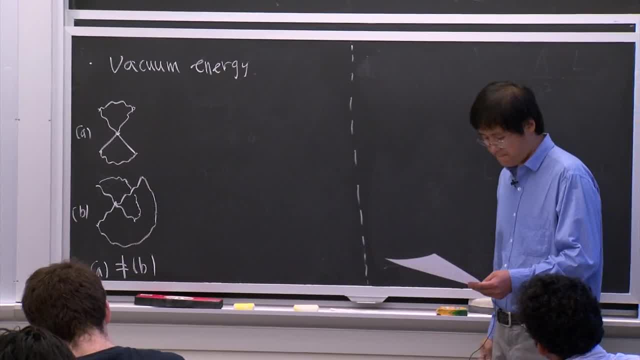 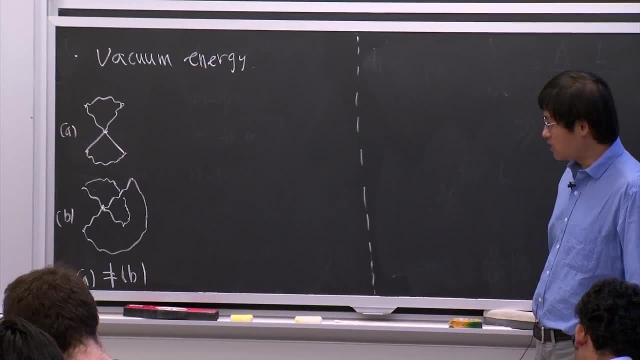 Because the matrices don't commute. OK, So now let's do the m counting. So do the m counting is actually much simpler. We use this double line notation. So let's now use the double line notation, Because all of these things, they're. 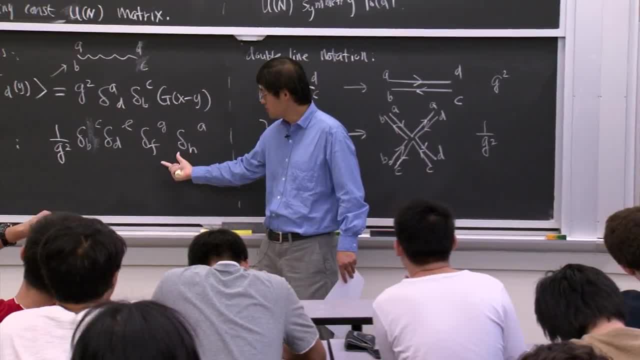 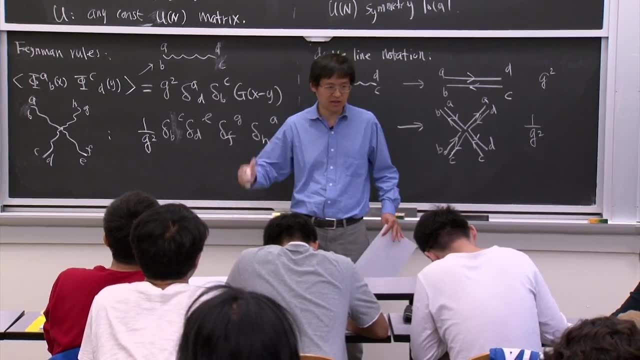 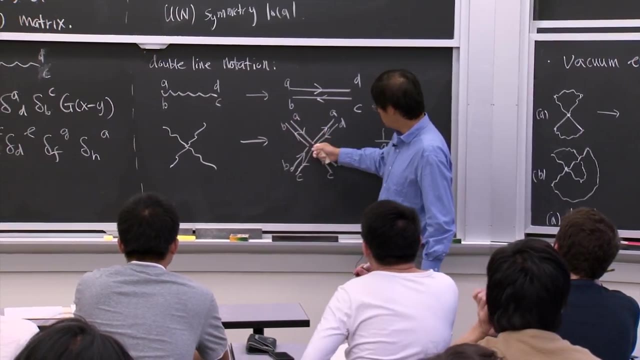 all these n. So when you do the contractions you have all these indices. You sum over all those indices. When you sum all those indices you get some factors of n. So that's how n will come into this theory. But double line notation makes the constraint all manifest. 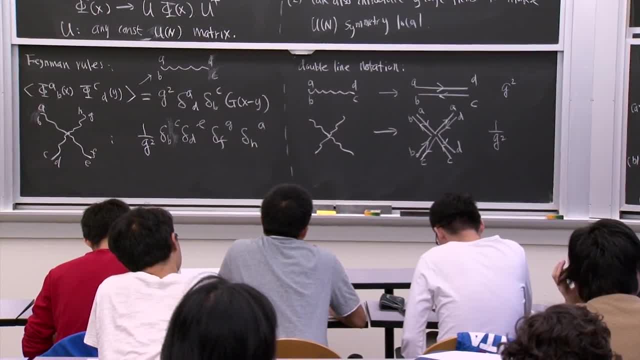 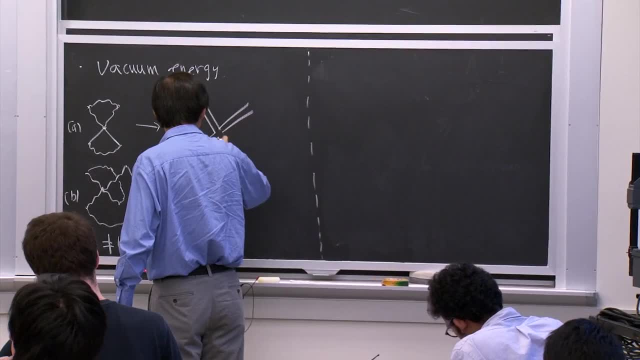 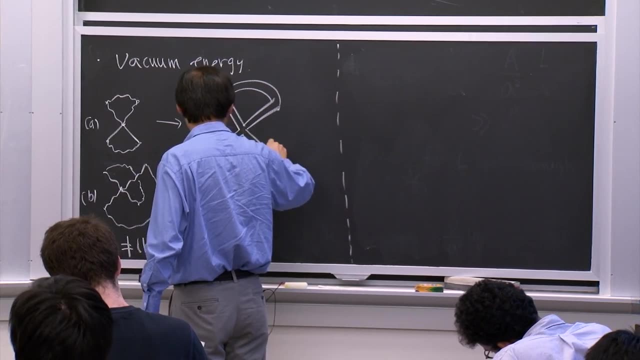 So the contraction will be automatic. You don't have to worry about all those deltas. So let's just do that. Let's draw this four point, Four point vertex. For this one, we just contract the neighboring ones. For this one, we do the same thing. 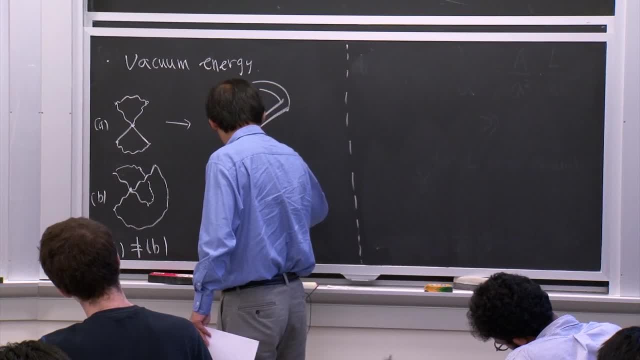 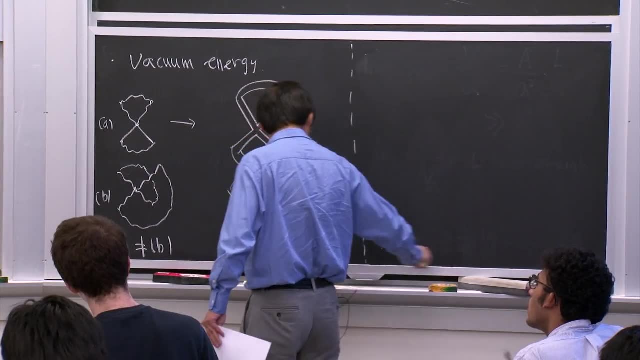 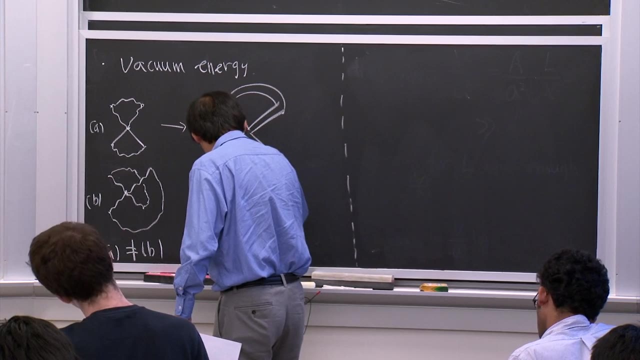 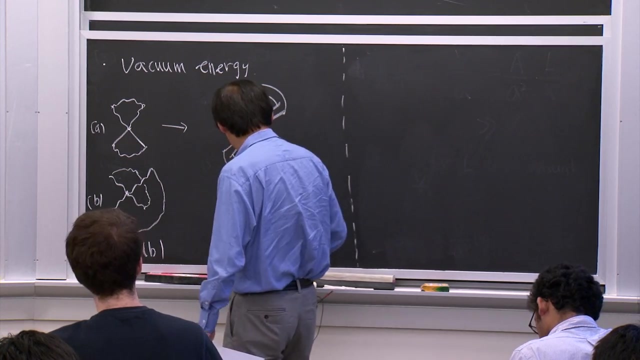 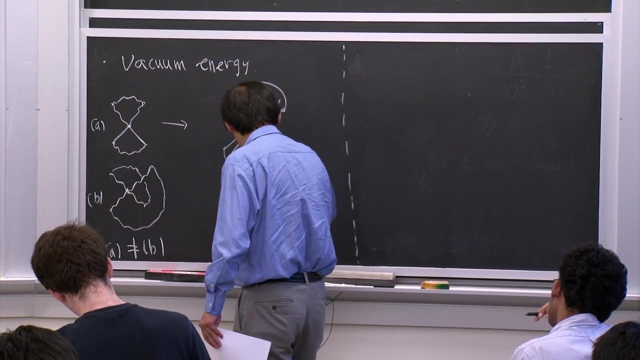 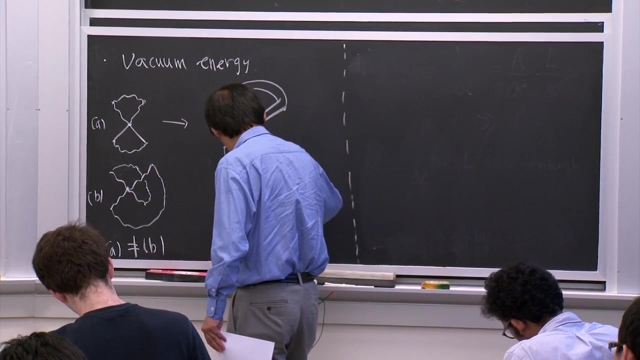 We contract non-labeling ones. Yeah, I did not draw very well, So let me OK. So this one should be contracted with this one, This one should be contracted with that one And this one contract with this one. This one is contracted with that one. 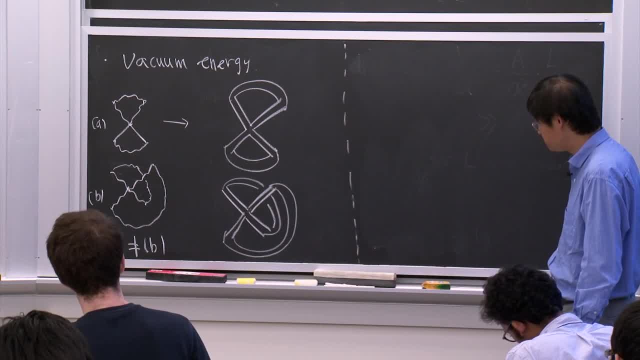 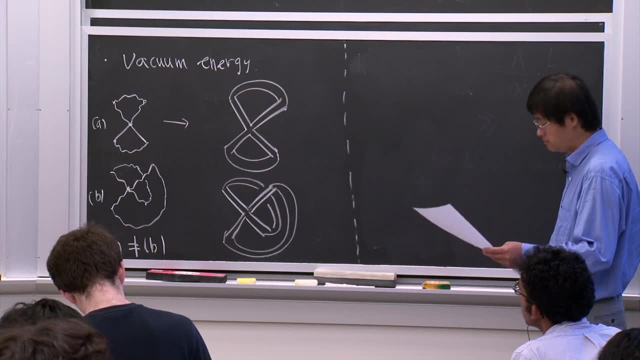 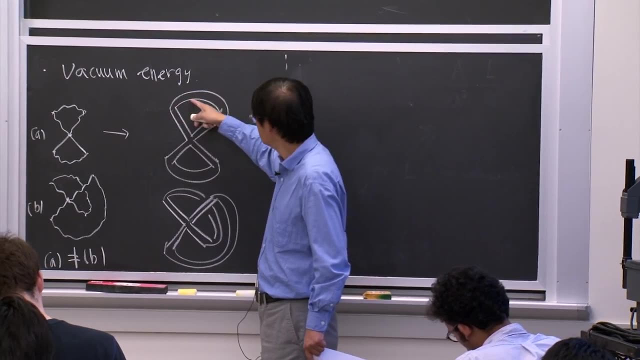 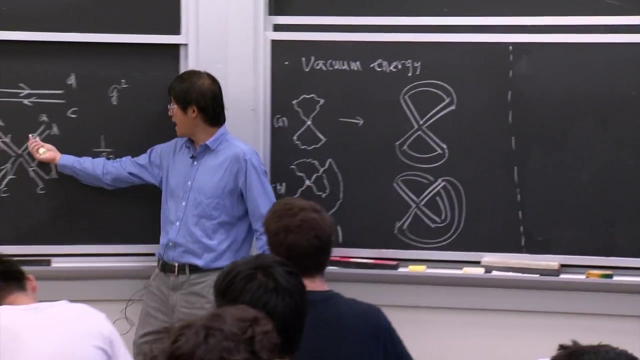 OK, So there's some intersection. So now let's come to the n. OK, So now here is the key, Each loop corresponding to a contracted indices. OK, So for example, in here this is already a and a, And then if you contract these two, then you sum over this a. 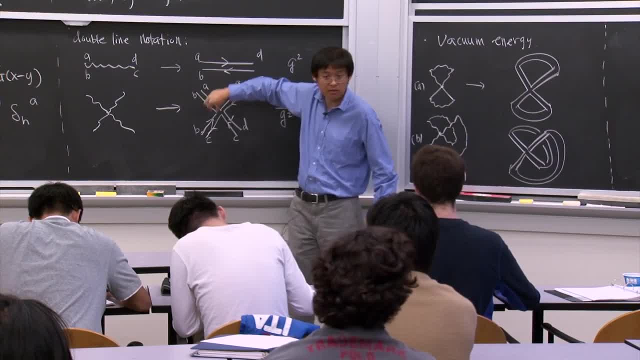 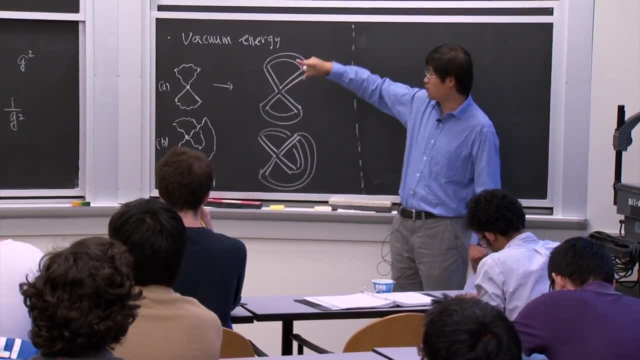 So you calculate the propagator And then that gives you a factor of n. So each contract, each closed loop essentially gives you a factor of n. OK, It's just because you contract. Yeah, So there's three loops here. 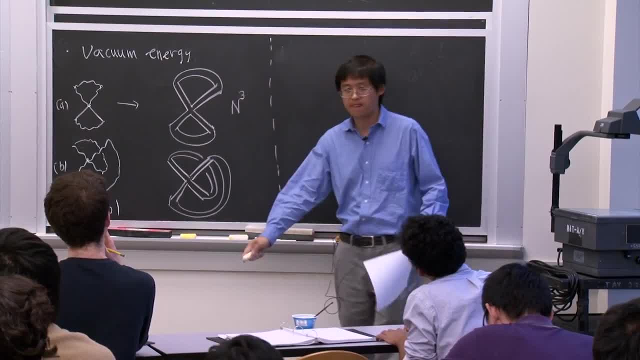 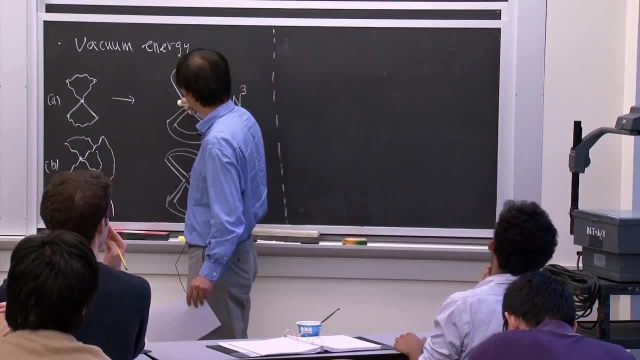 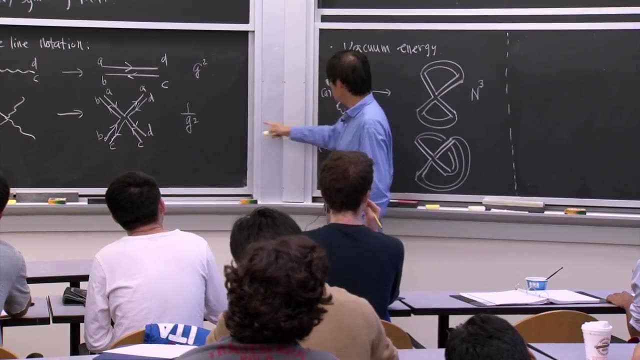 Three contracted loops. So this gives you nq. OK, And if you look at the g squared- dependence. so you have two propagators. here You have two propagators. Each propagator gives you a g, G squared. Then you have one vertex. 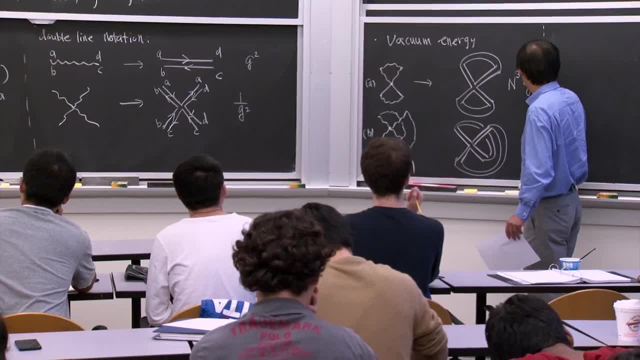 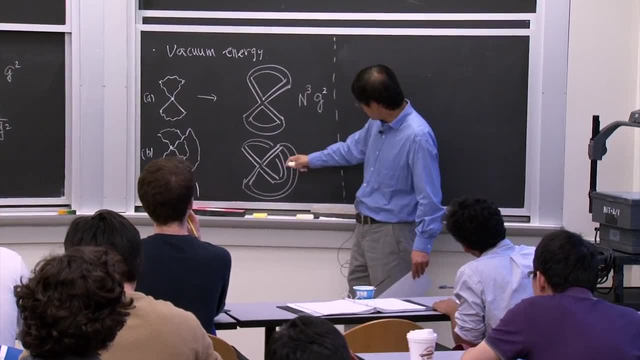 Each vertex gives you a 1 over g squared. So you have g squared, OK. So now let's look at this one, This one. let's just follow this line. You should also draw the arrow, because the arrow should follow. 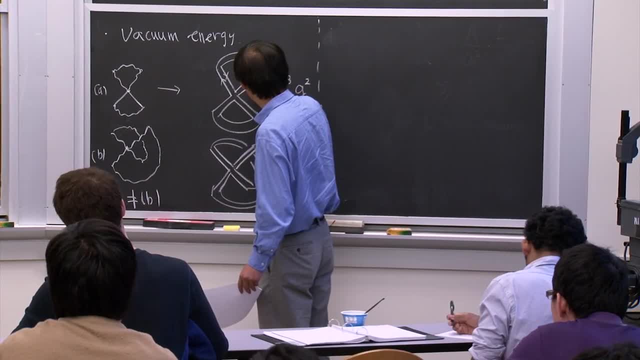 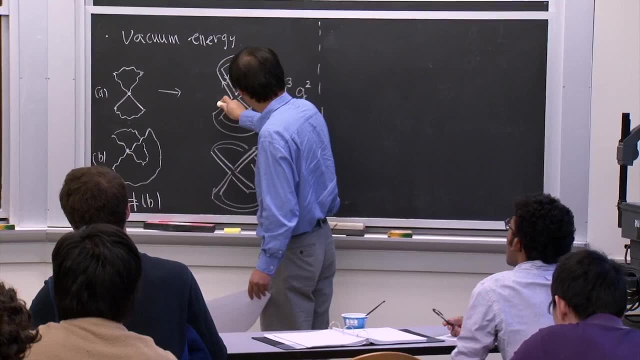 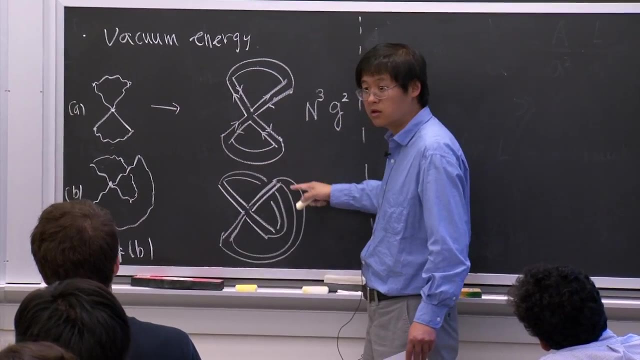 OK, I did not draw the arrow, but the arrow should all follow. OK, The arrow should be consistent. Similarly here. So here, if you go around, you find there's only a single contracted line. So this is only a factor of n. 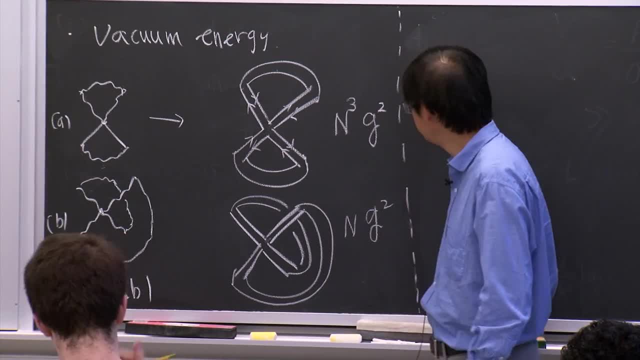 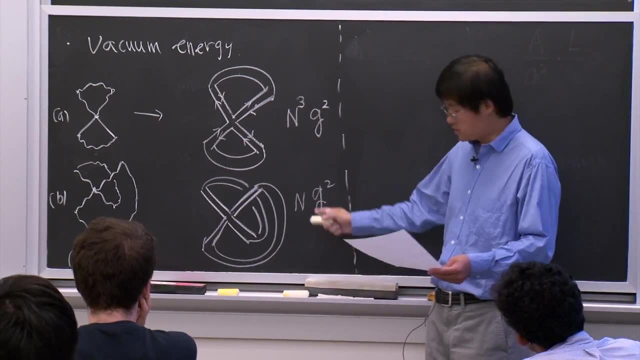 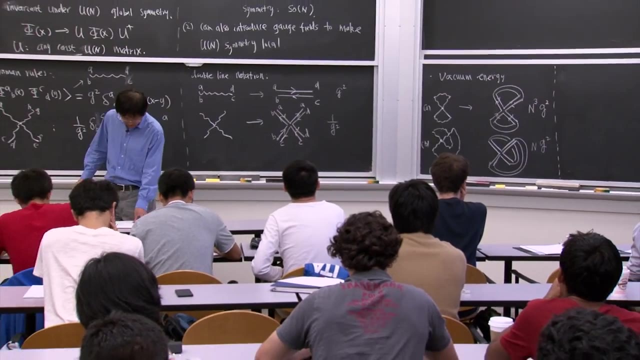 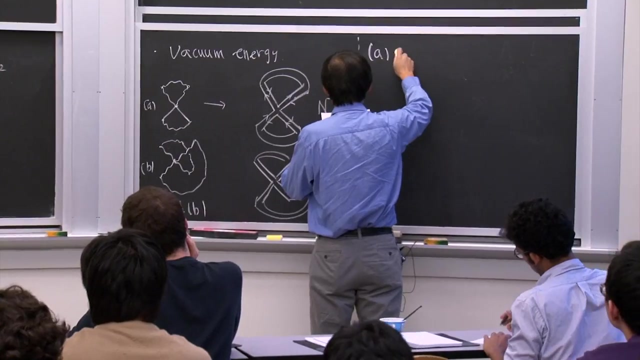 Of course g squared, dependence is the same. So you have g squared. OK, Now you already see the difference between these two diagrams, And one is proportional to n, One is proportional to nq, So a diagram a can be drawn on the plane. 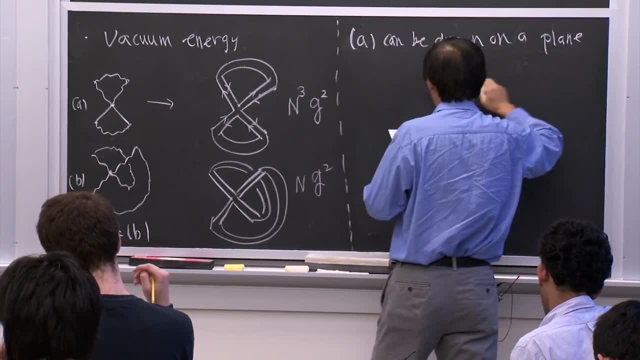 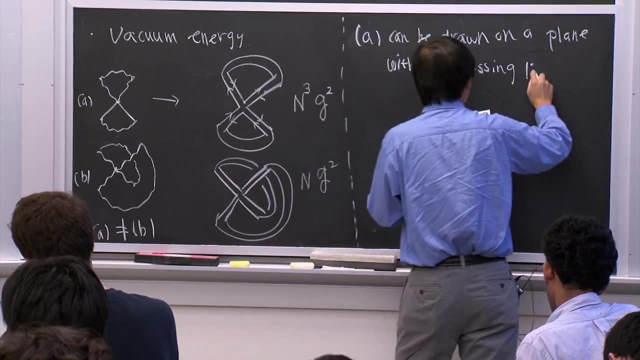 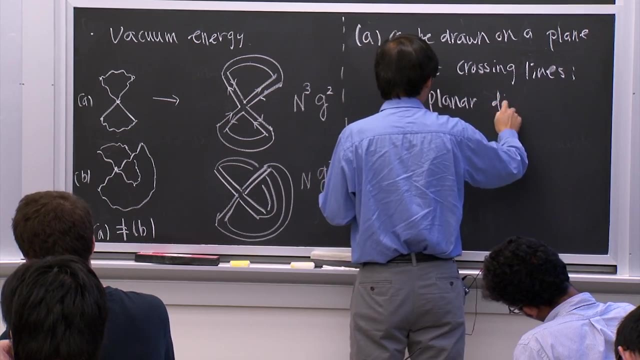 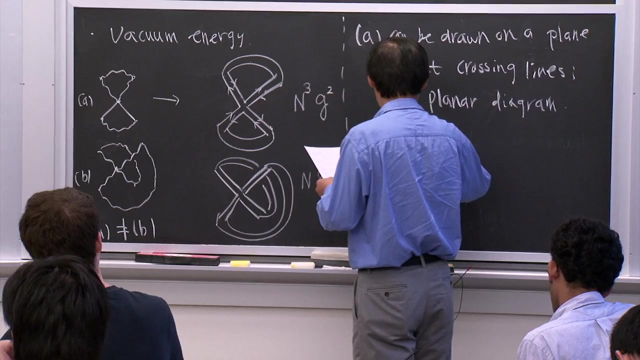 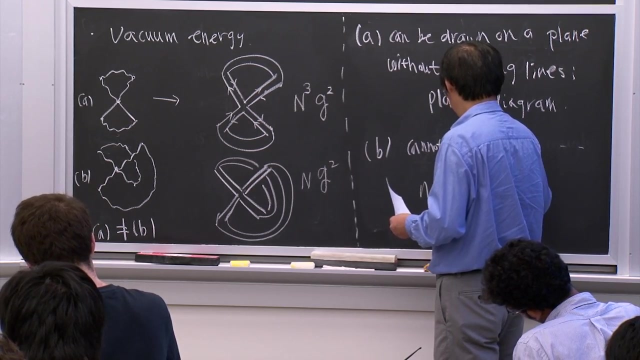 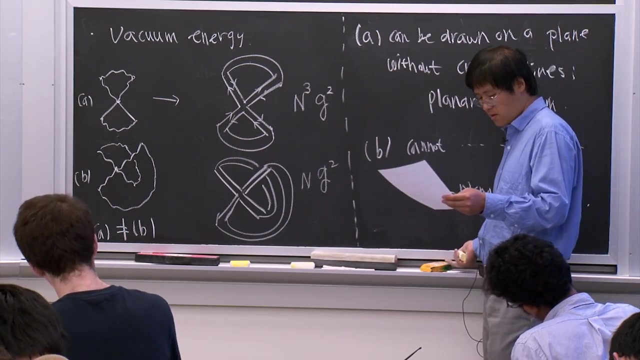 We are drawing it on the plane without crossing lines, So we call it a planar diagram. And b cannot be drawn on the plane without crossing lines, So we call it a non-planar diagram. OK, So let's do one more step. 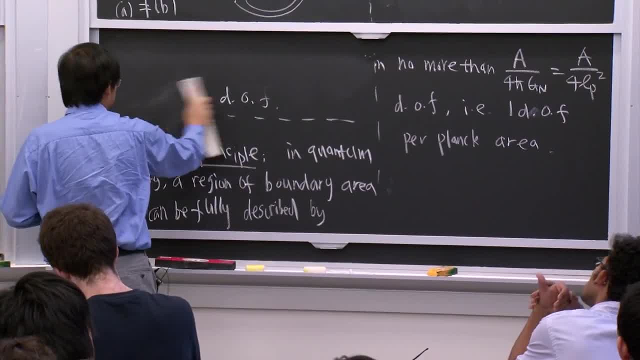 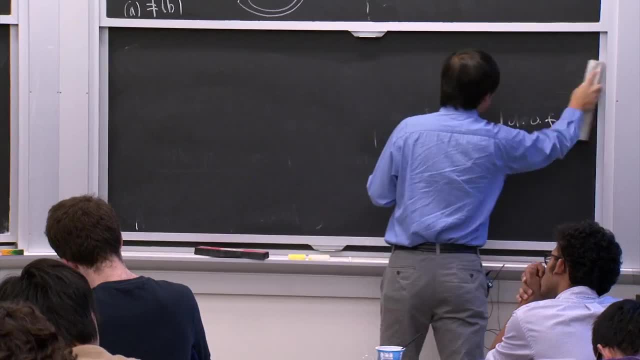 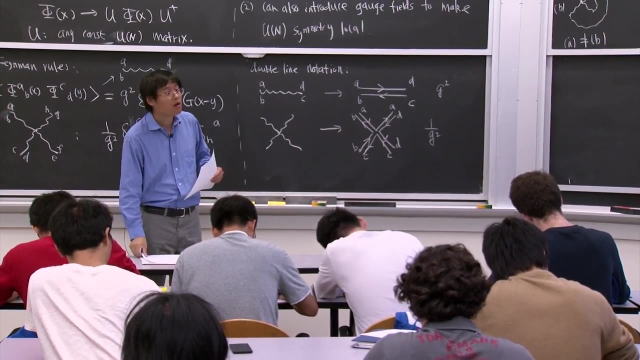 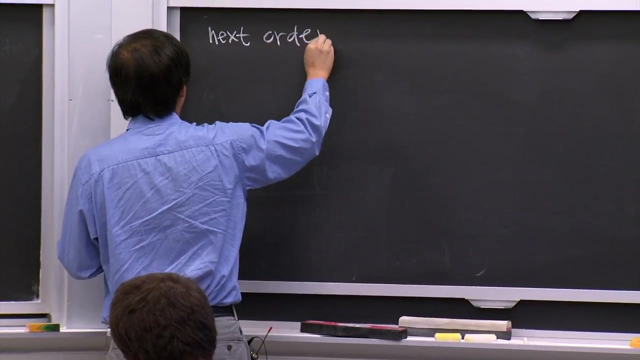 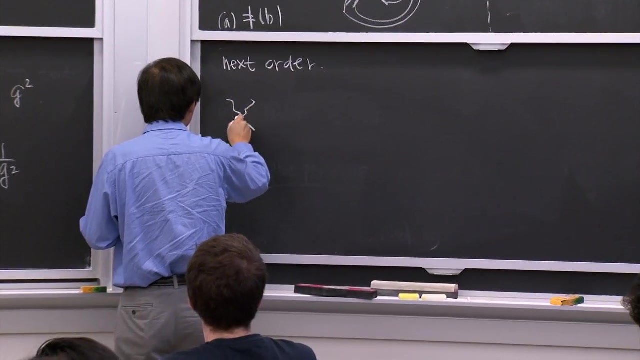 So let's do one more diagram. So let's do one more diagram. OK, So next order, you just get two. Next order: vacuum diagram. without any external lag. You have two vertices. OK, OK, OK, OK, OK. 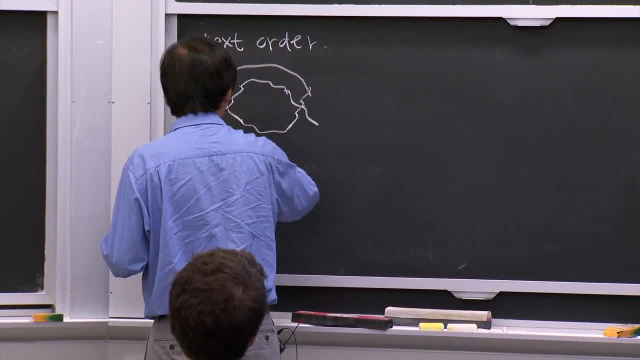 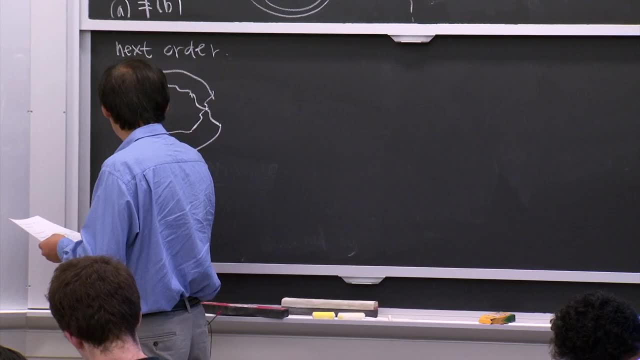 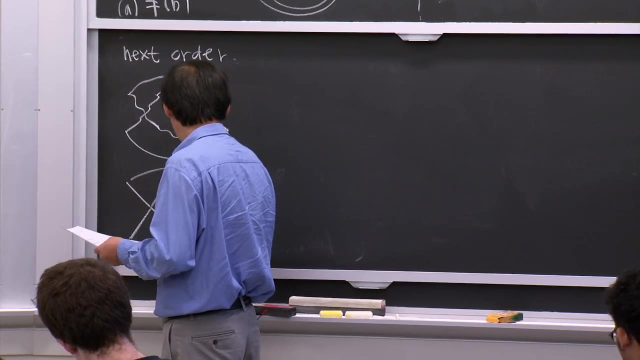 So you can connect this way. OK, So this is one diagram. You can also have a non-planar diagram. Yeah, Let me just draw the straight line rather than the wavy line, just to save trouble. You can, for example, you can draw like this: 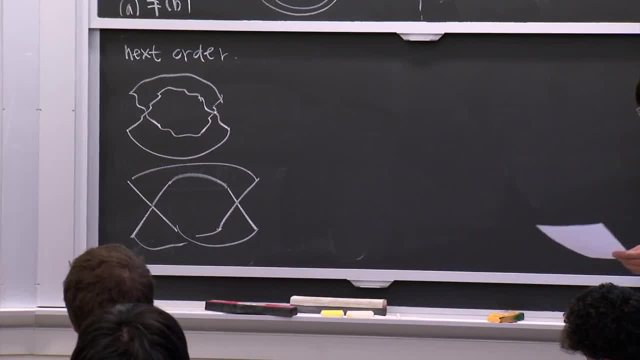 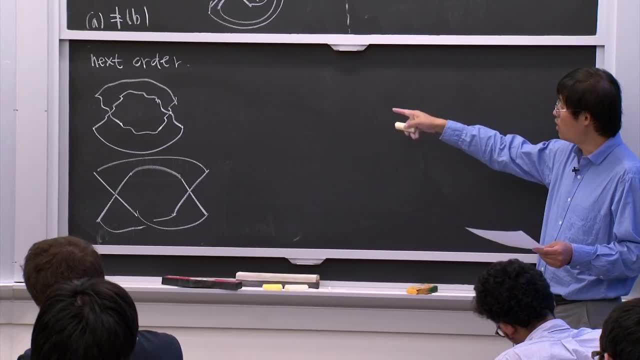 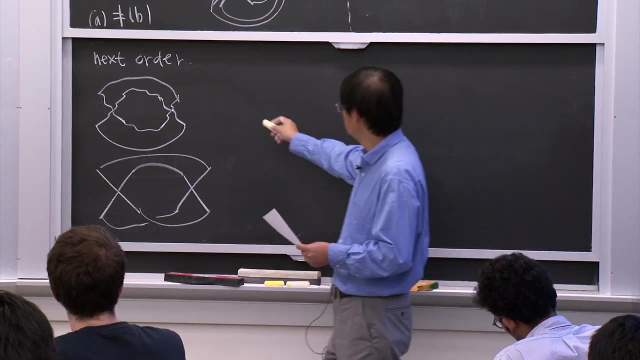 So this is a non-planar diagram. OK, So now I'll give you an exercise Today. when you go home, turn those into a double line diagrams. Then you should find yourself that this is n to the power 4.. Yeah, maybe I should do this. 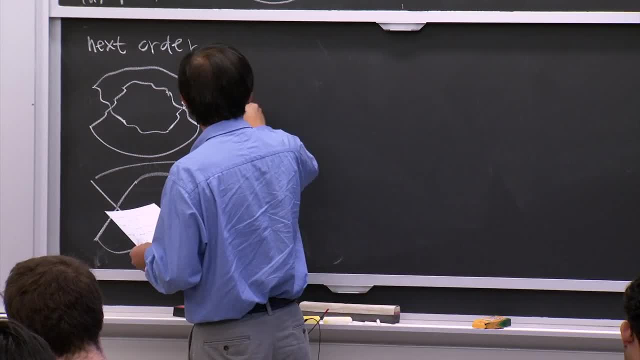 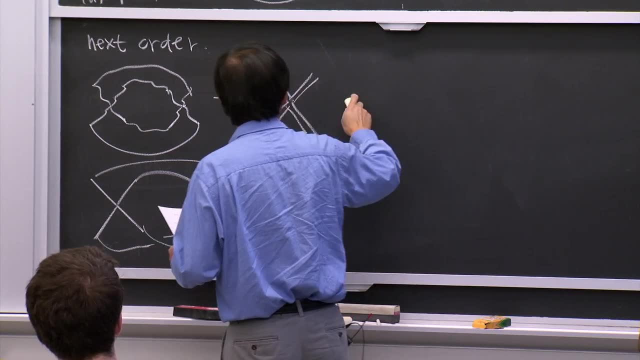 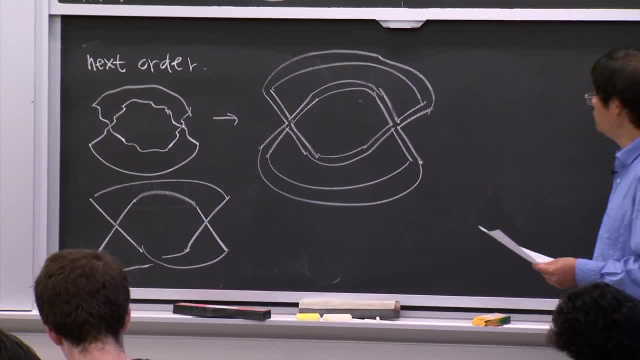 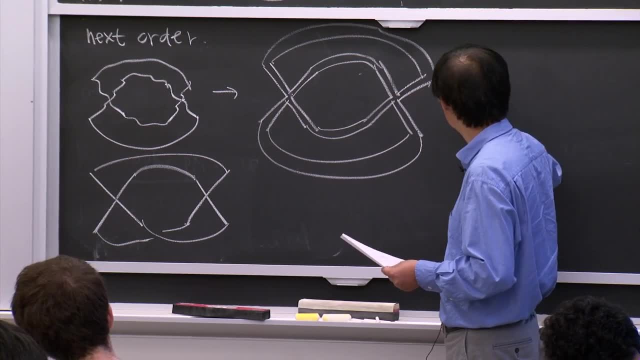 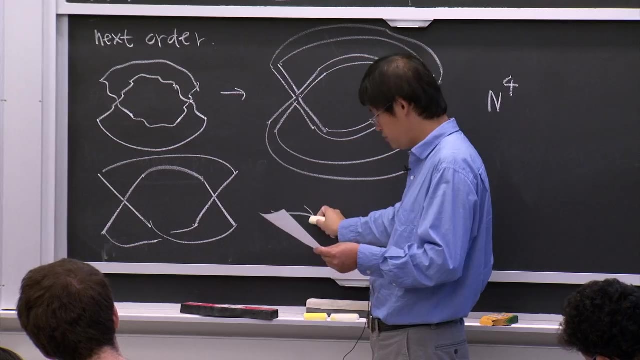 OK, So this one. you count how many contracted lines: One, two, three, four. So this gives you n fourth behavior, And this I will not do it now, You do it yourself. So also, if you count the g dependence: 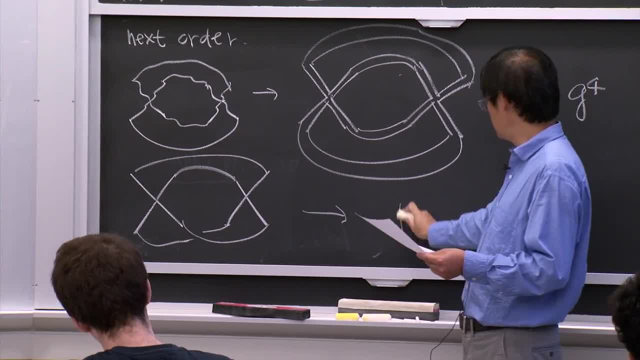 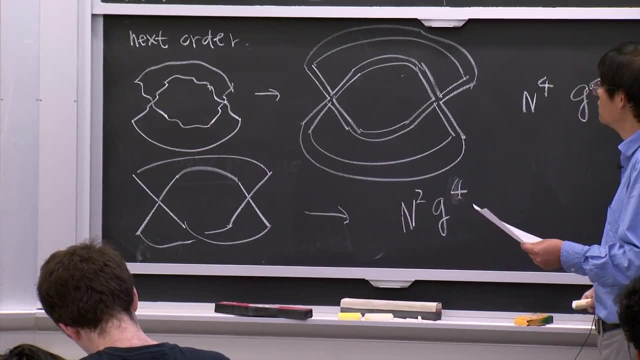 this gives you g to the power of 4.. And this gives you n squared g to the power of 4.. Is it g to the power of 4, or maybe I'm counting wrong- 1,, 2,, 3,, 4.. 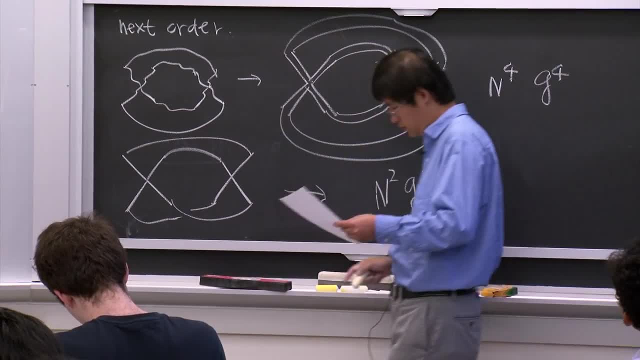 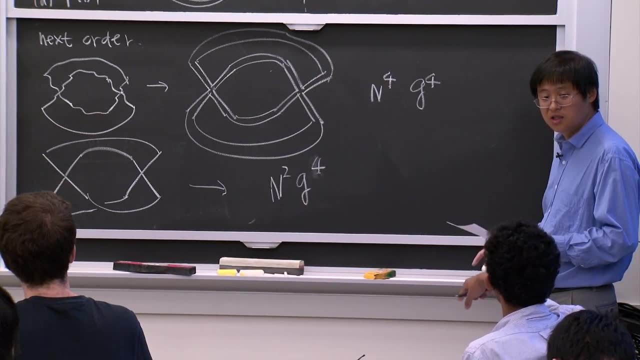 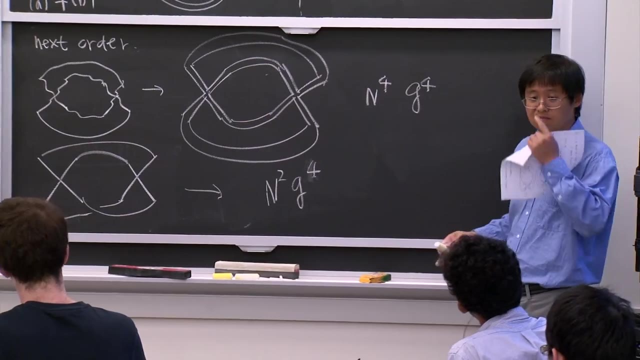 4 propagators is g to the power of 4.. Yes, So in general, the more is the more crossings with that decrease. n HONG LIUO- Yeah, that's right. OK, So now you can just continue with three vertices. 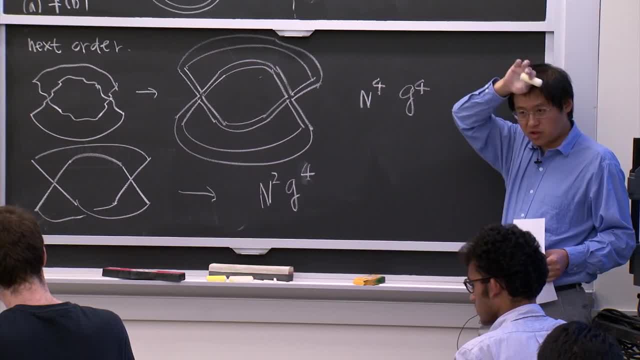 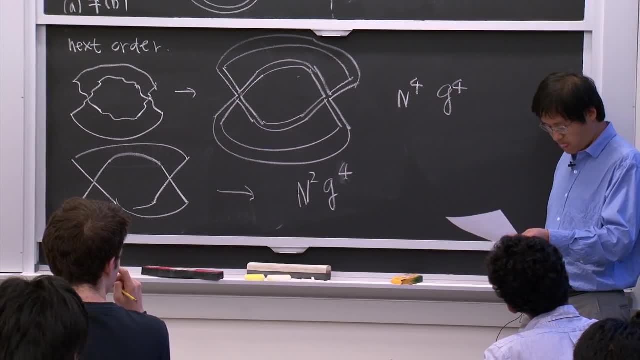 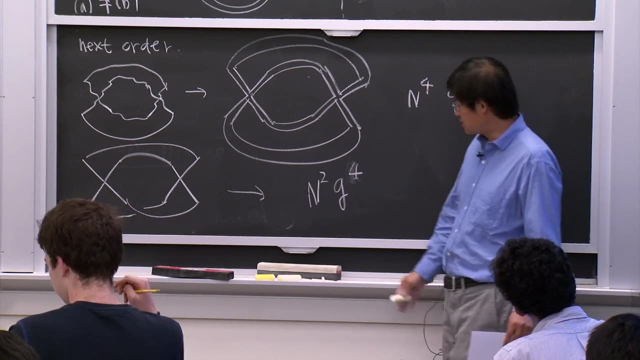 with four vertices, et cetera. But of course the smart fellows will now stop And they ask: can I find some rules in doing this? Say, how do you get the general n counting And whether does the all long planar diagram? 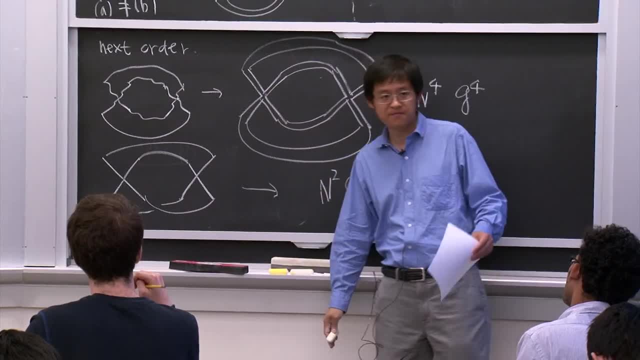 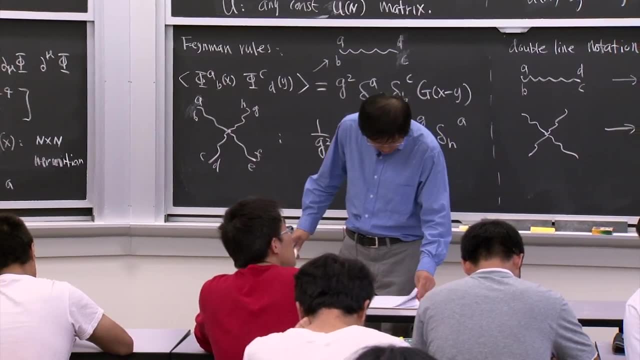 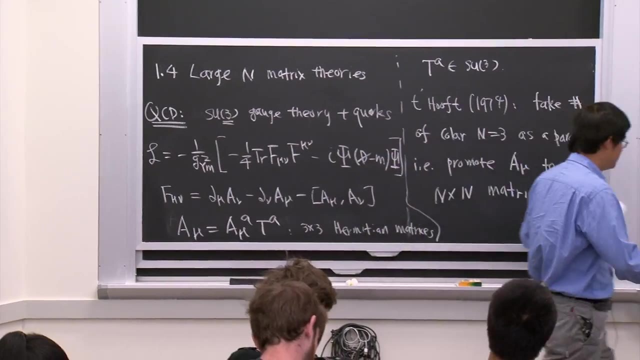 was the same, or do I need to classify them further? OK, So these are the obvious questions, And let me just tell you some observations, Then I will close for today. Then I will close for today. So the first observation. 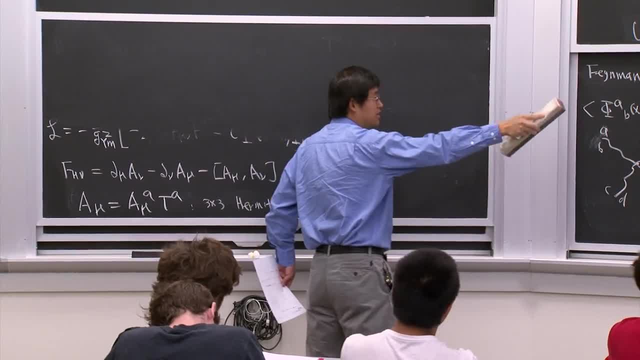 HONG LIUO- So just a little bit HONG LIUO- OK HONG LIUO- So just a little bit HONG LIUO- OK, HONG LIUO- So just from those examples. 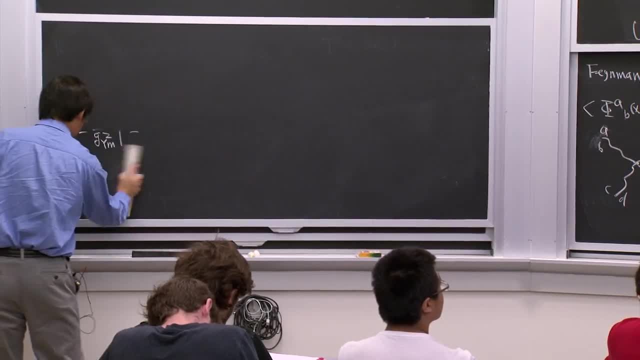 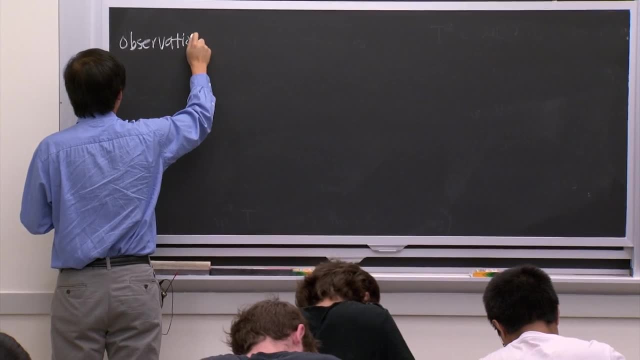 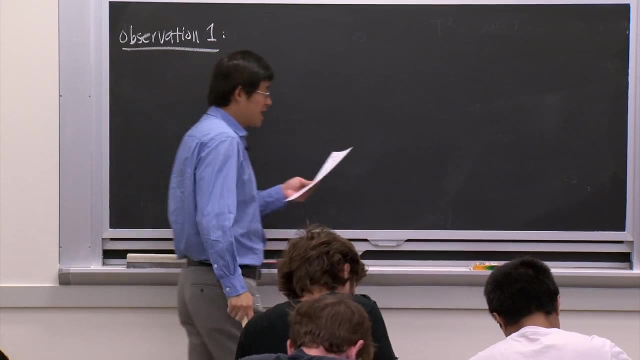 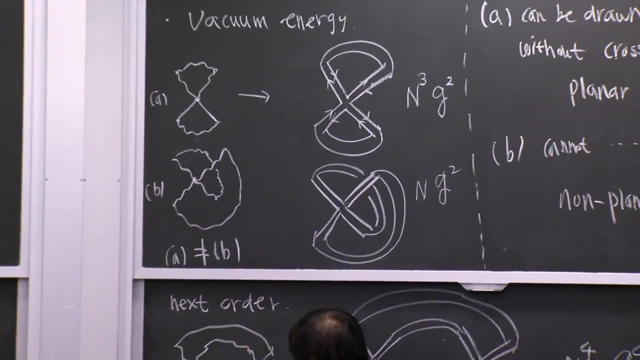 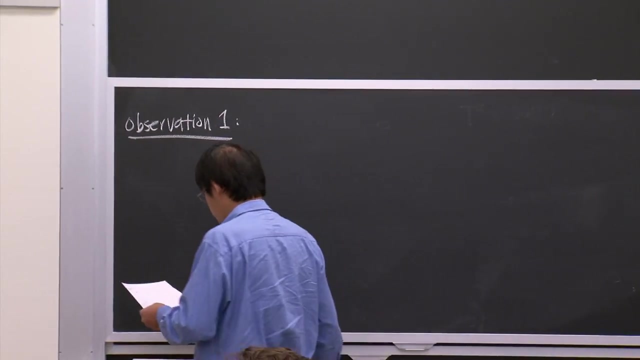 let me just draw some observations. Observation one- so this one requires a little bit ingenuity- is that even a and b. so this a and b, they cannot be drawn on the plane. They cannot be drawn on the plane without crossing lines. 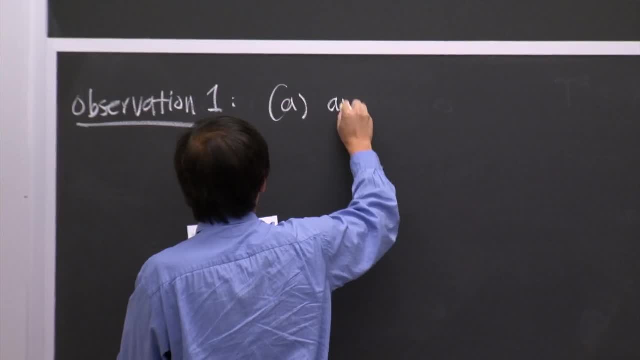 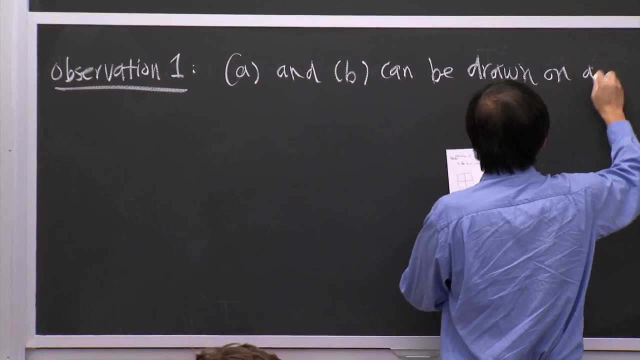 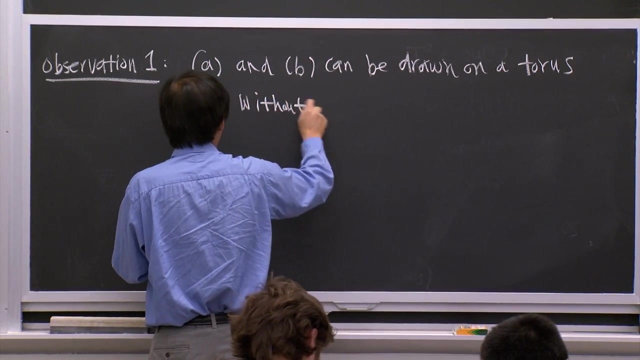 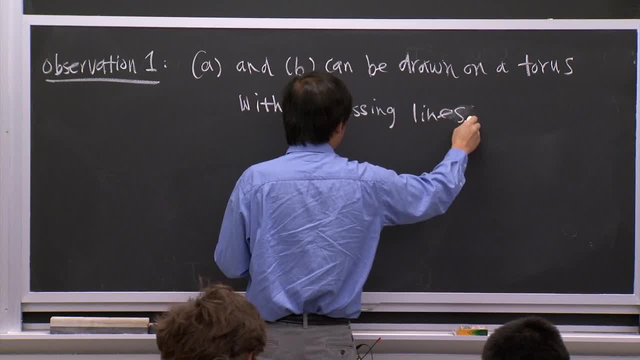 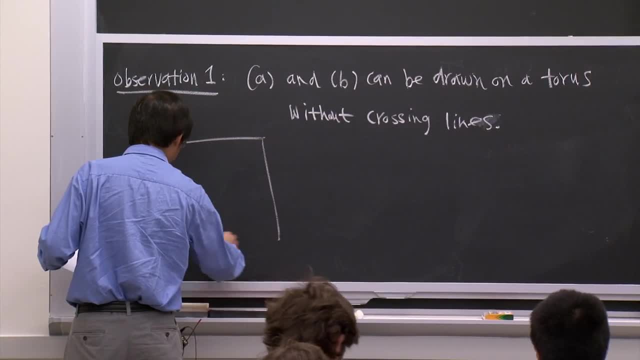 HONG LIUO- OK HONG LIUO- OK HONG LIUO- So now let me show it to you. So what is a torus? So we can draw a torus on the plane like follows: 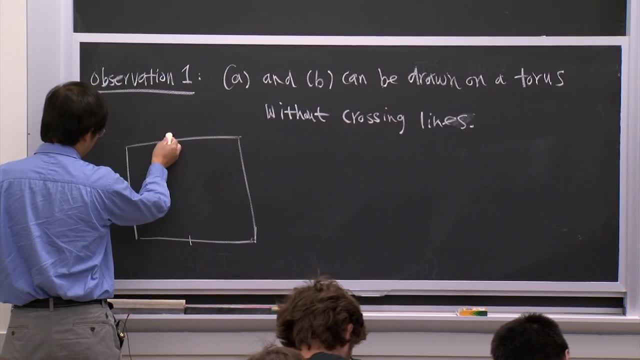 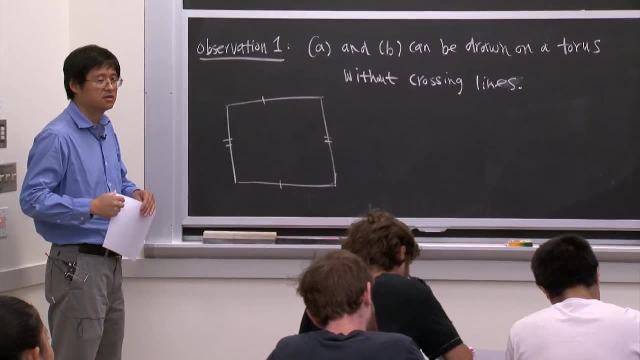 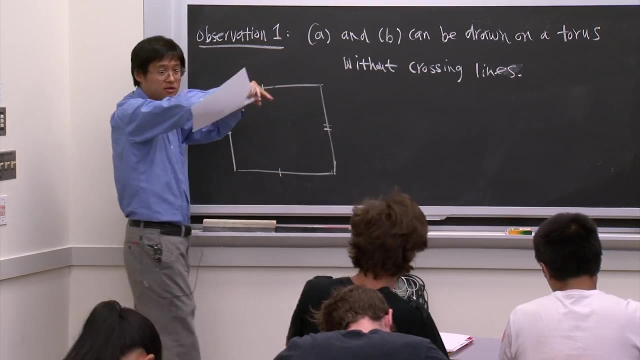 So we draw a square, Then we identify this side with that side, identify this side with that side, Then this give us a torus. OK, So, because when you do that, then give you a cylinder, And then you do that again, then give you a torus. 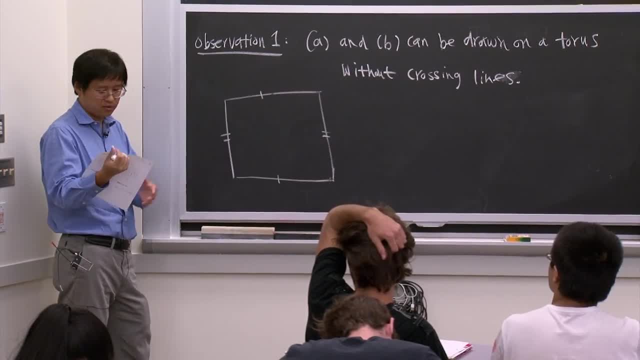 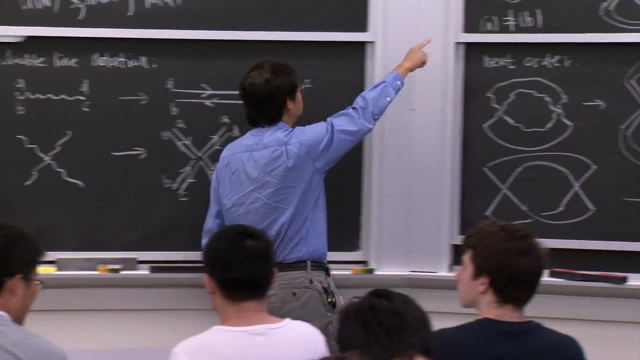 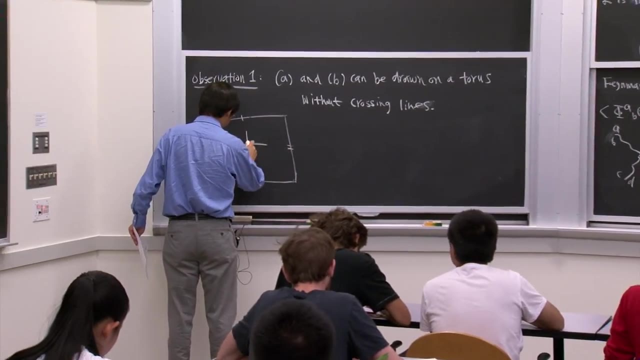 OK, So, but on the plane, just simple identification. So let's try to see this diagram. Now let me show. this diagram can be drawn on the torus without crossing, Because the vertex is like this: We want to contract this guy with that guy. 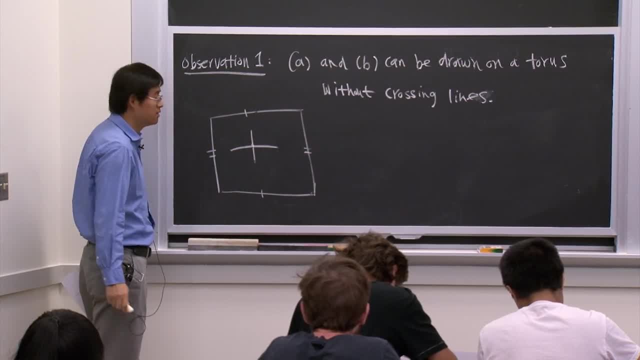 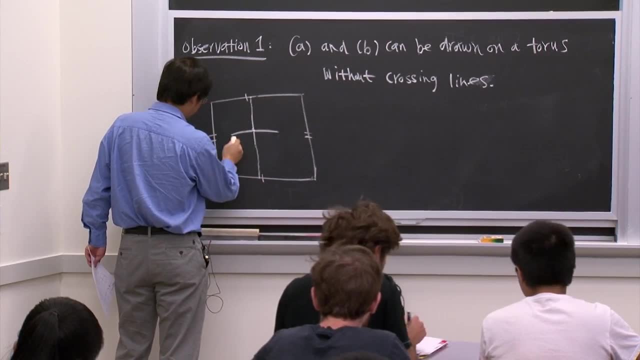 and that guy with that guy right Non-labeling ones. But now I can just go up And now this is identified: This guy is here, That can come back here, Can go here, come back here. OK, So this is contracted. 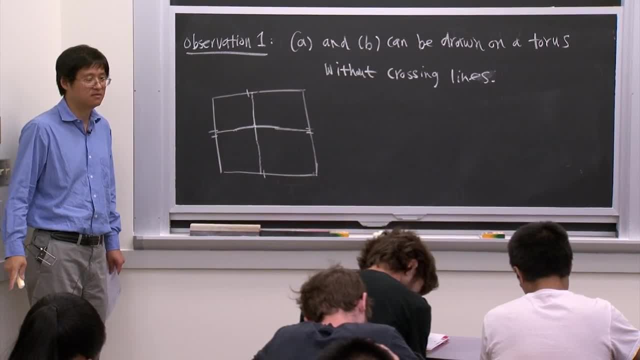 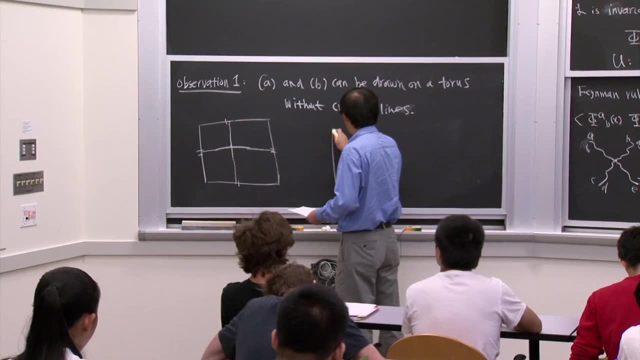 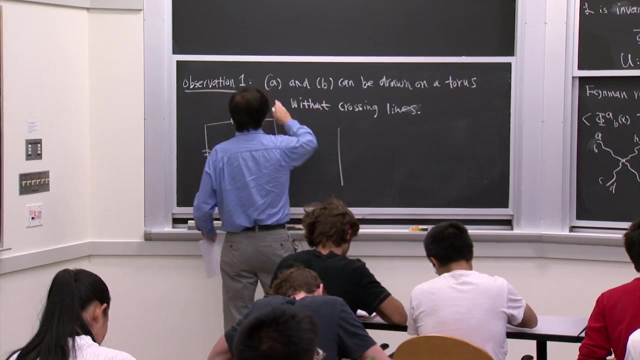 And I don't have to cross lines. Yes, Good. Similarly, let me do that one. Yeah, that one. maybe I will let you to do it yourself. So this is A. This is not A and B. This is B and D. Let me call. 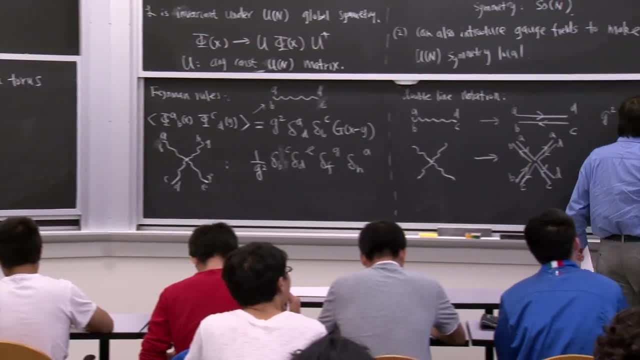 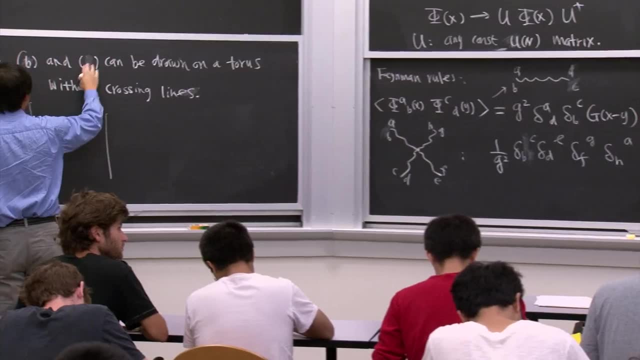 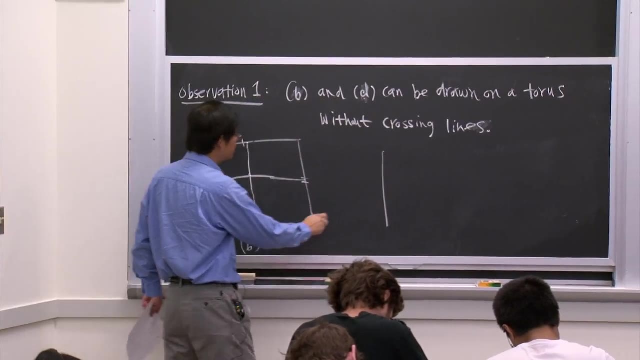 this B, This is, Let me call it C and D. So A and C are planar diagrams And B and D are non-planar diagrams. OK, So this is B, So try to do it yourself the D. So essentially you have two vertex. 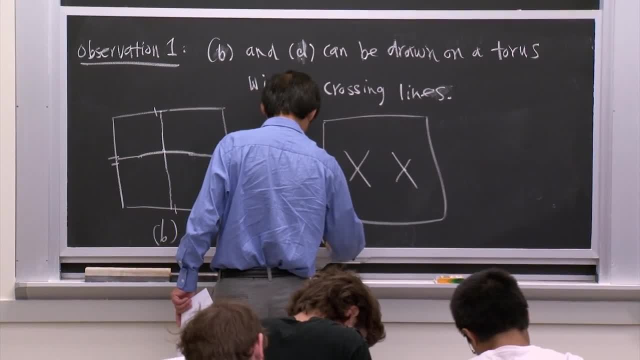 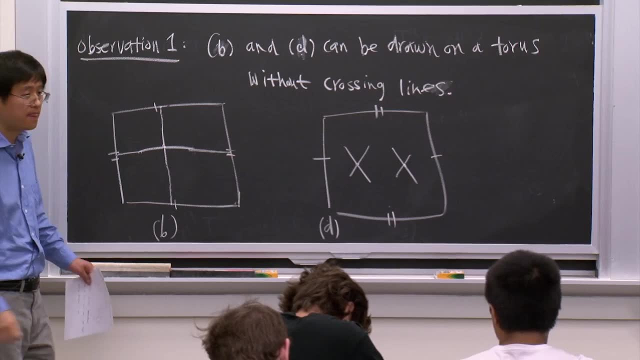 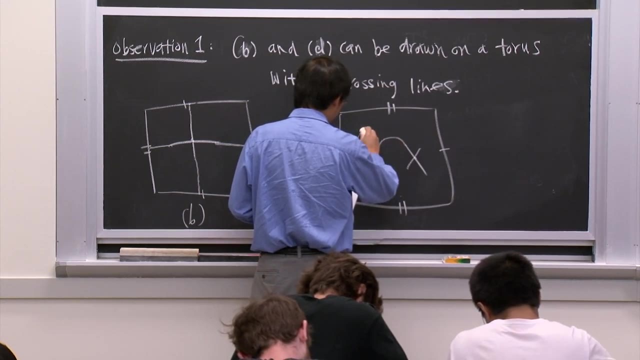 How to make that non-planar diagram to be planar on this torus when you identify here with there, there, It's there, OK. So this is observation one. Actually, let me just do it for you So we connect, because I need to do this. 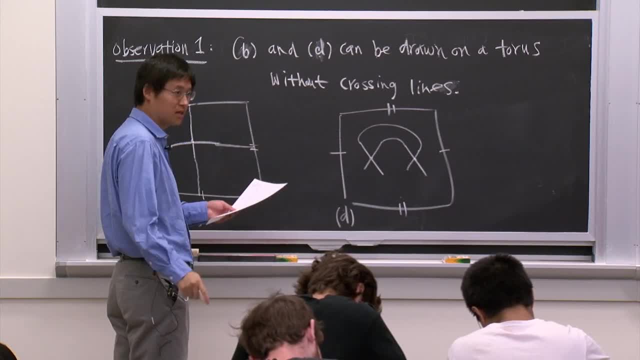 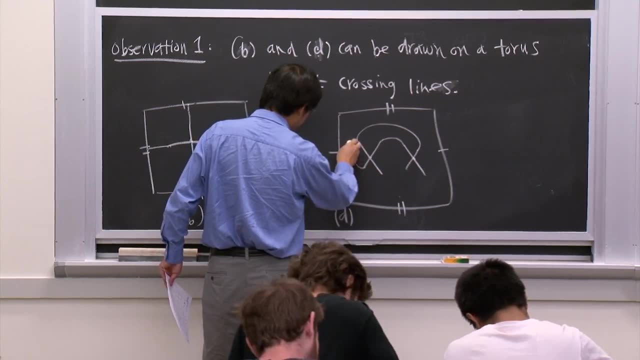 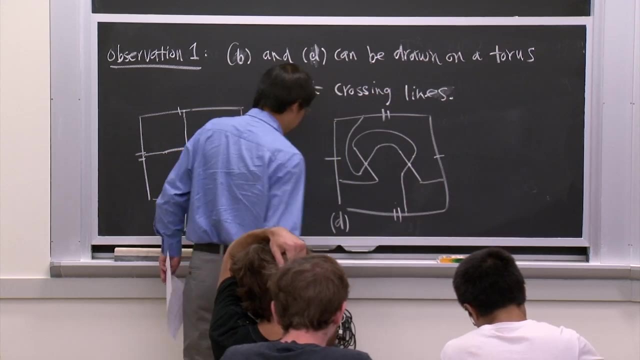 Because it's better. I have this example to make my second point. So now I need to connect this to that guy, But I can do it by going up. This guy can go here And then go there. Similar thing, OK. And then this is: I can connect them without crossing lines. 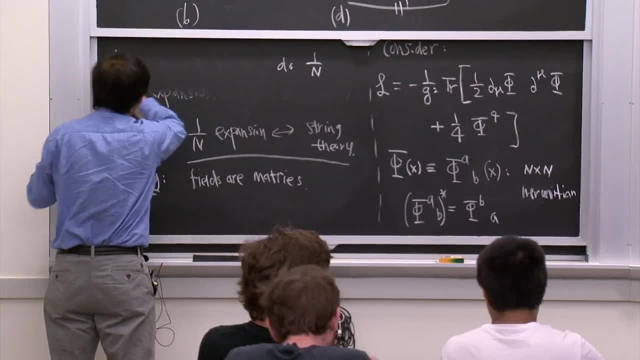 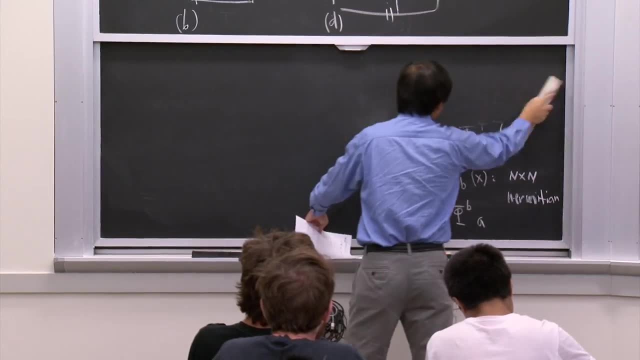 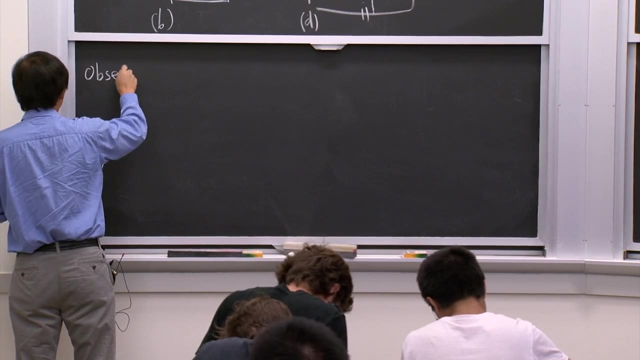 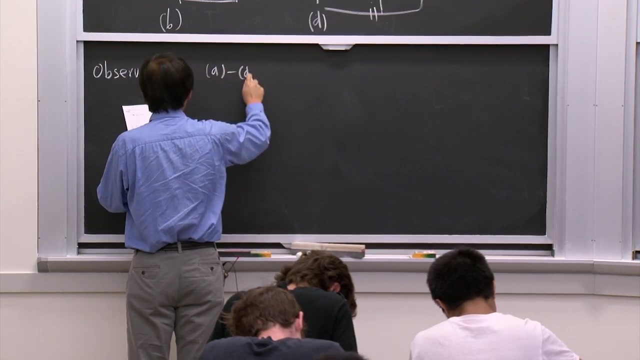 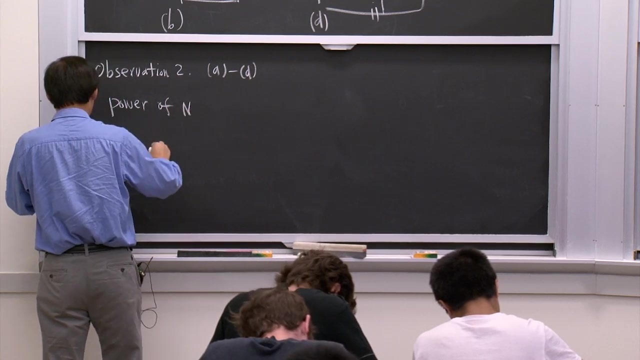 So this is observation one. So now the observation two again is a little bit ingenious, But maybe slightly easier if you have done it long enough. For all the A to D, This is B And D. The following rule is true: The power of n is equal to number of faces. 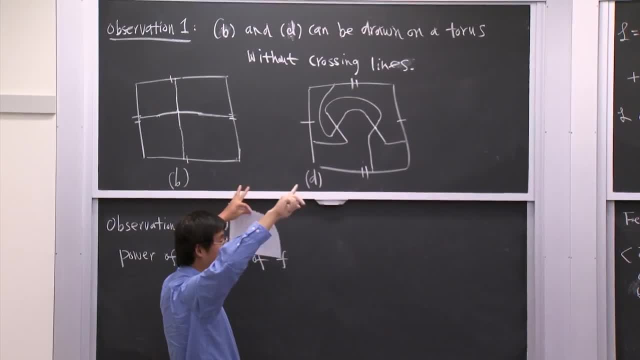 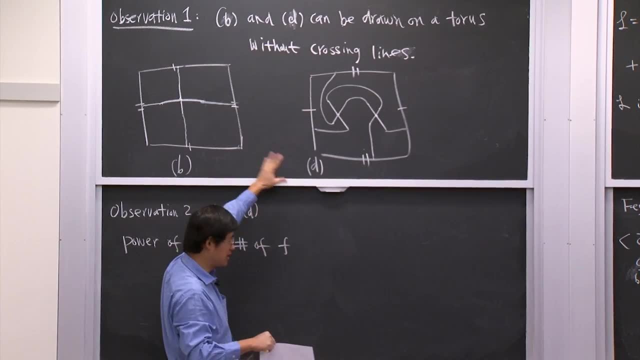 So this one we call. So, even though they cannot be crossed, they cross lines on the plane, but we can actually straighten them out on the torus. OK, So here we call: we can straighten them out on the torus. 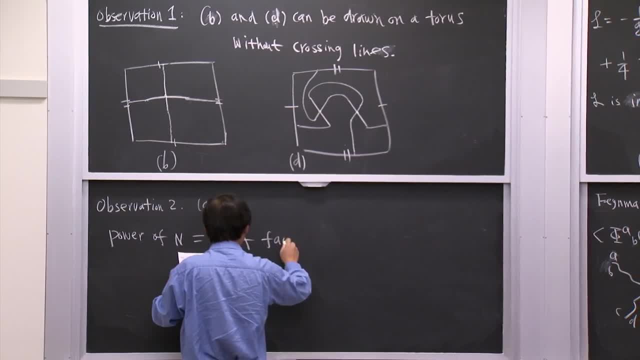 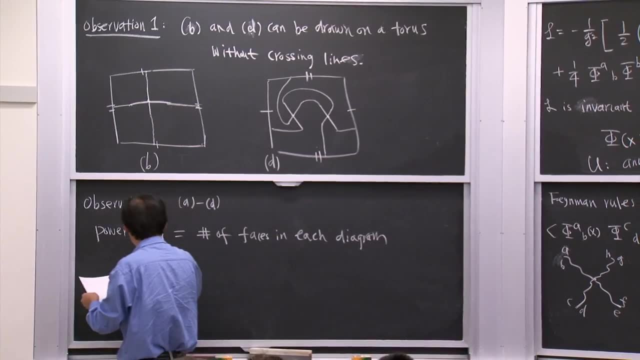 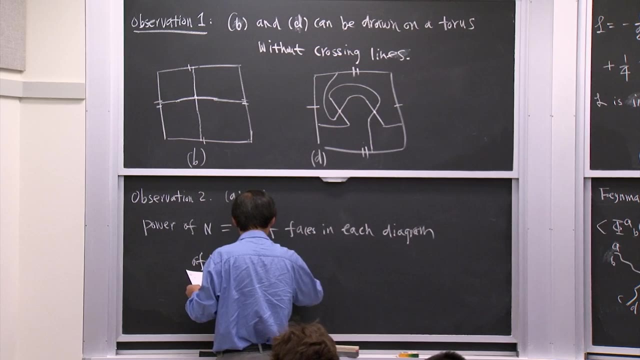 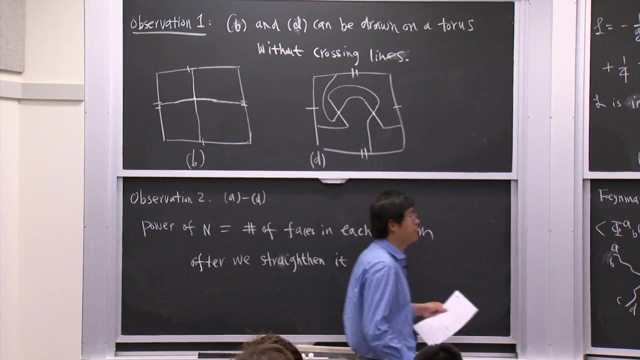 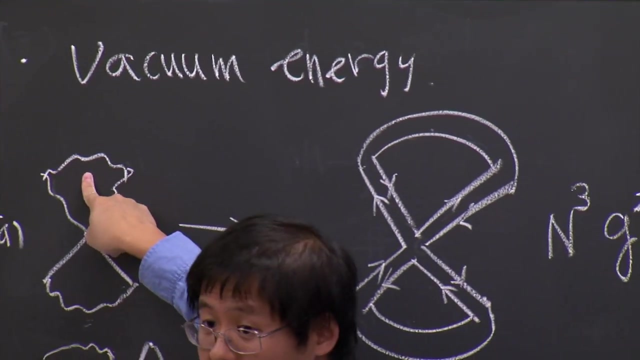 So the second is: the power of n is the number of faces in each diagram after we're stretching it out. OK, first let's look at this diagram. This is a planar diagram, So there's one face, there's two faces. 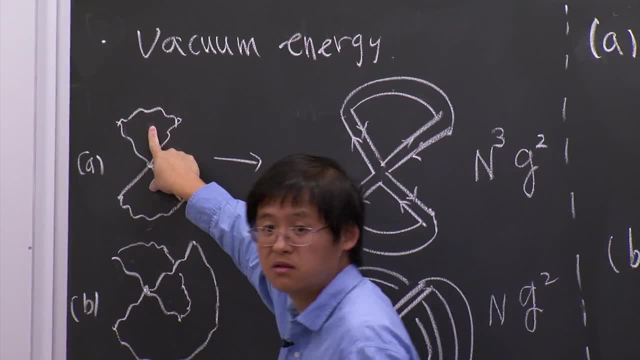 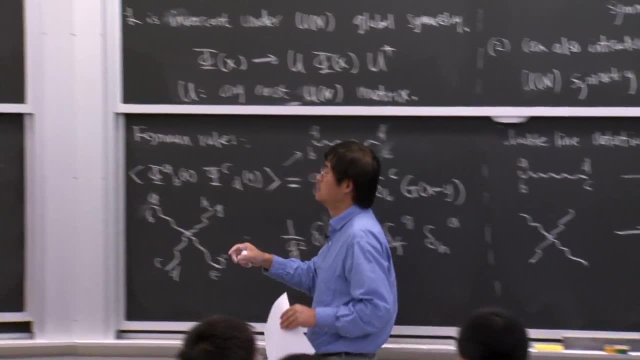 and then there's a face outside because it's a whole plane. So there's three faces. So this is n? cubed And the b on the torus. there's only one face because each region is connected to each other. OK.